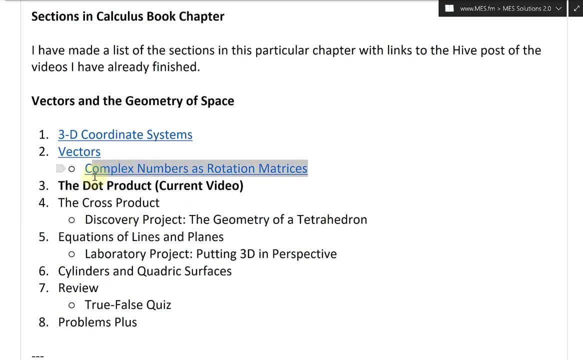 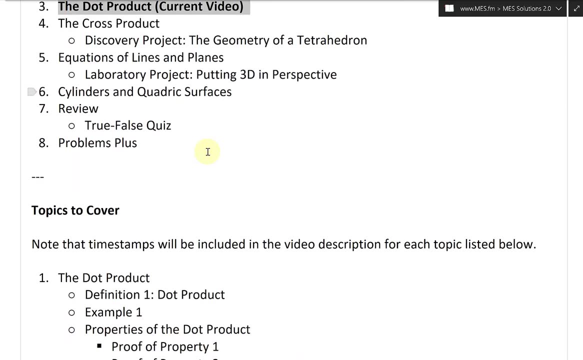 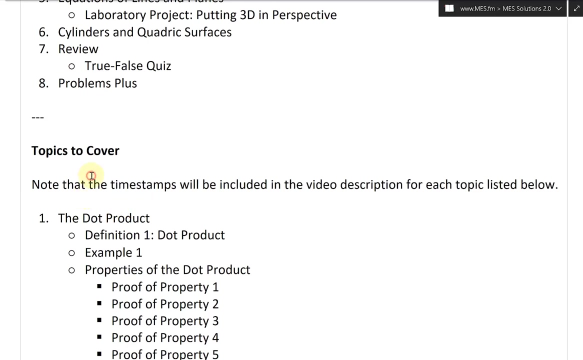 I did a video, very interesting one, on the complex numbers as rotation matrices are. highly recommend a diving into that one. And then all and now. the one we're doing right now is the dot product and that's the current video, And then later we'll go over these ones here as I go through. So let's jump right in. So, topics to cover. So a note that, yes, a note that the- yeah, the timestamps will be included in the video description for each topic list. 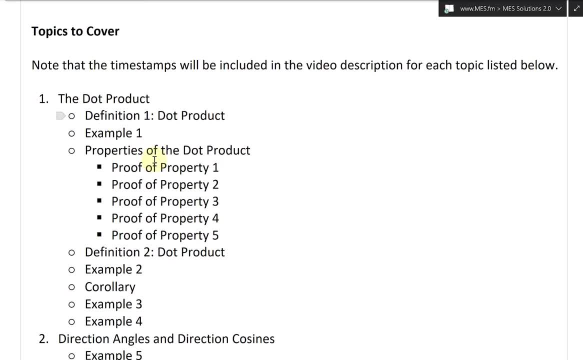 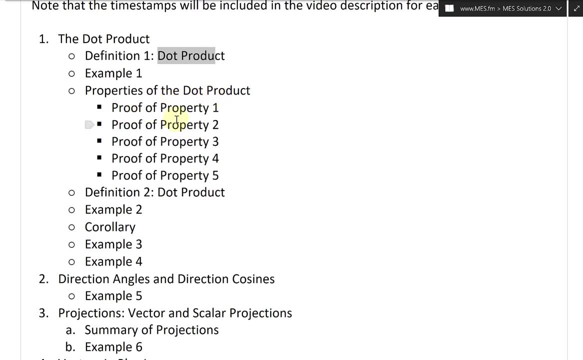 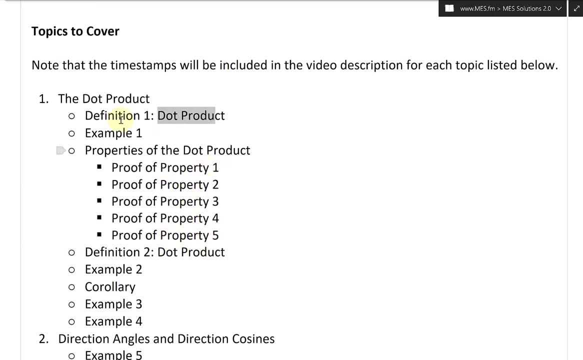 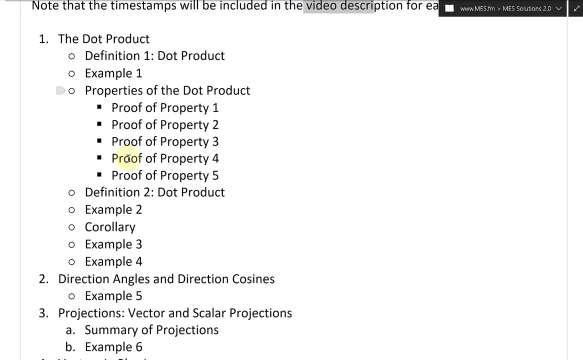 below. So the first part. we're going to go over the dot product, then definition one. it's on a dot product example, I mean example one- then go over properties of the dot product and I'll put proof of property one, proof of property to proof of property. three, proof of property for property, five, etc. And again I'm listing all this is. I'll put this in the description with links or with the timestamps to every single section here. then then go over definition to dot product example to corollary or a corollary. 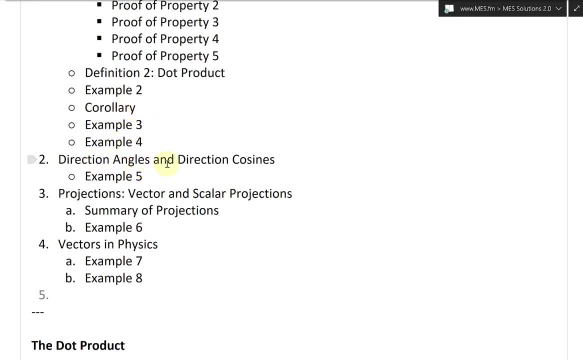 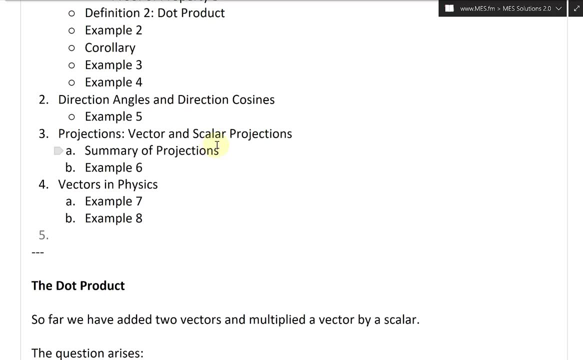 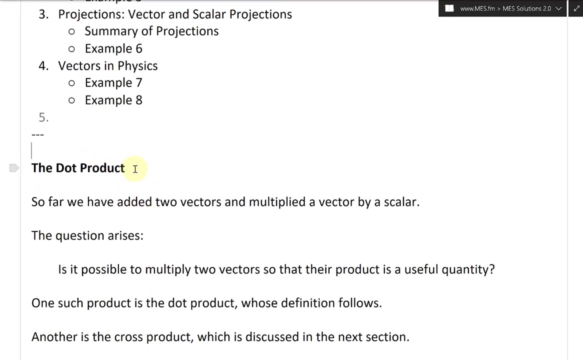 and then example three, example four, and then direction angles and direction cosigns and look at example five and then projections, and then, yeah, look at vector and scalar projections and then summary of projections and then example six. then then look at the next section of last section, vectors in physics, and go over two examples, example seven and example eight. All right, so now let's finally jump right in and look at the dot product. So so far we've added two. 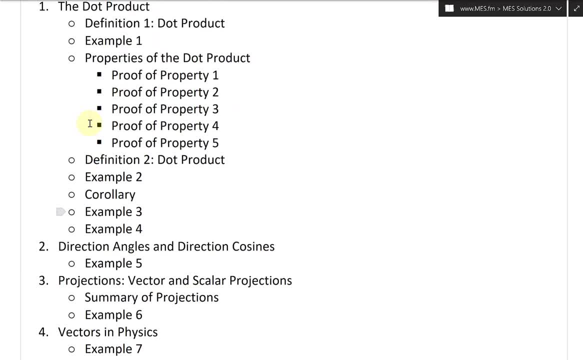 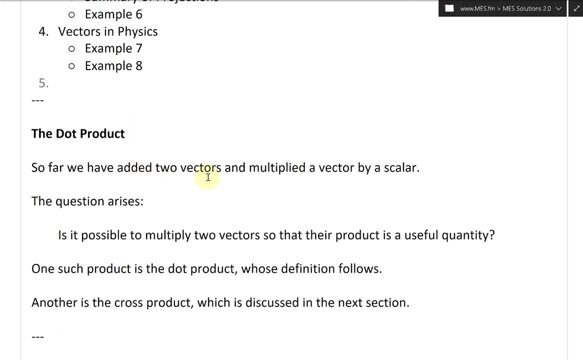 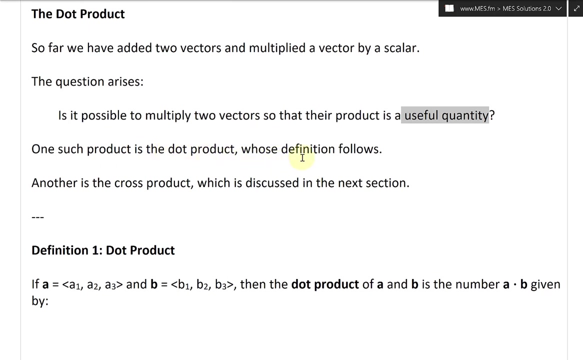 vectors and multiplied a vector by a scalar, And that's in the earlier videos on the on vectors and so on. we just added vectors and we multiplied and we multiplied vectors by a scalar. But then the question arises: is it possible to multiply two vectors so that, so that their product is a useful quantity? And one such product is the dot product, whose definition follows, And another is the cross product, which is discussed in the next section. 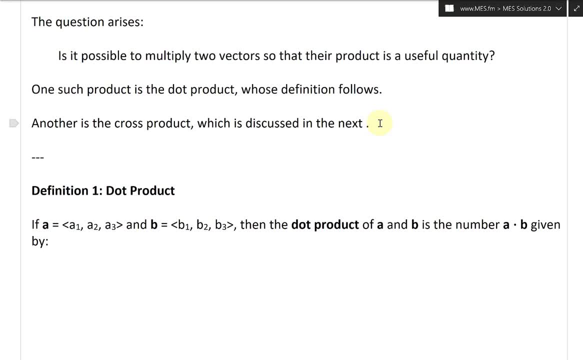 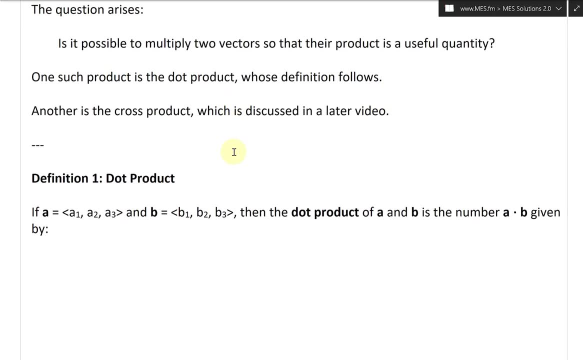 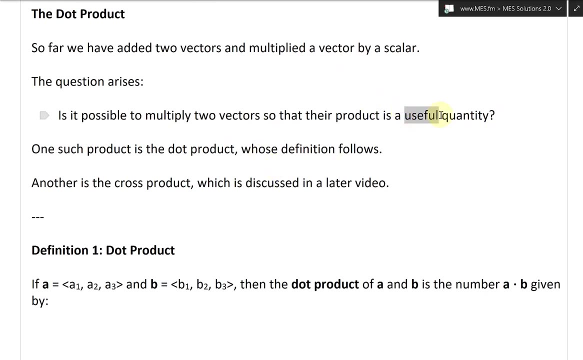 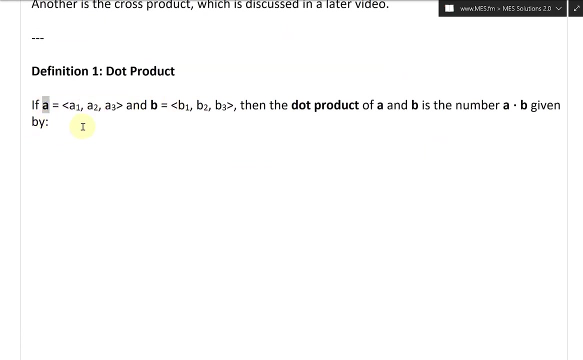 Or actually this is from my caucus book, So in a later video, in a later video, All right. so now let's continue further and look at now definition one. So we'll define dot product and we'll show how it is. we could utilize it to be basically a useful concept, a useful quantity. So if the vector a number, we bold them. if it's a vector as components a one, so you write these triangle brackets for indicating. 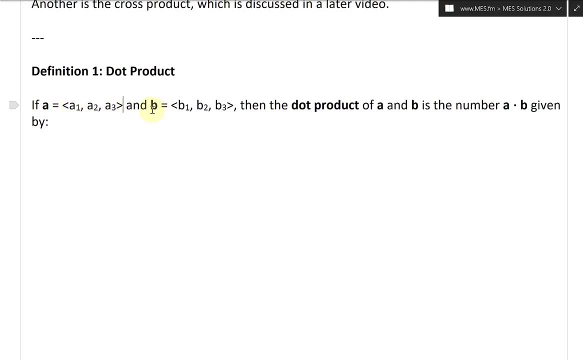 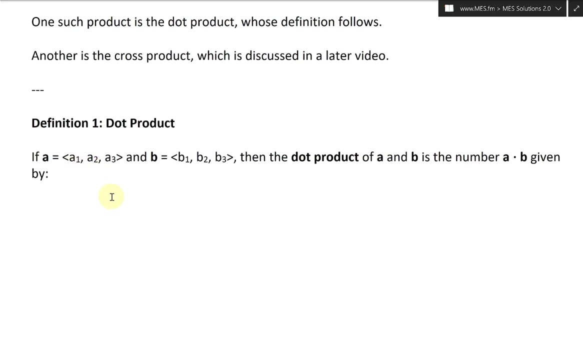 it's a vector, so a1, a2, a3, and this b vector has a component, b1, b2, b3. then the dot product of a and b vectors is the number a dot b. so you write: you have this dot there given by, yeah, given by, and we'll write this over here: this is a dot b and remember the notation you could. 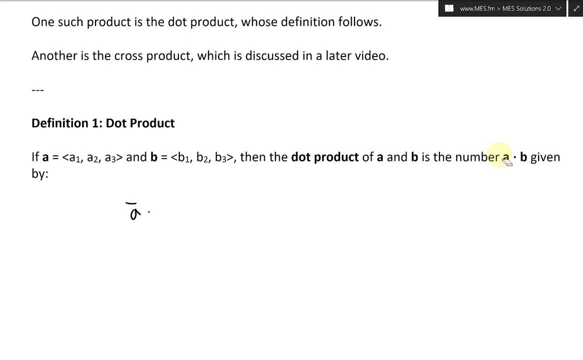 also write a vector with an arrow on top and i'll write it with arrows on top and i'm writing with my pen, just because it's hard to write with the bold set up here, because they all look the same: this one here, so that's bold. it's easy to bold when you type and not so easy when you're type. 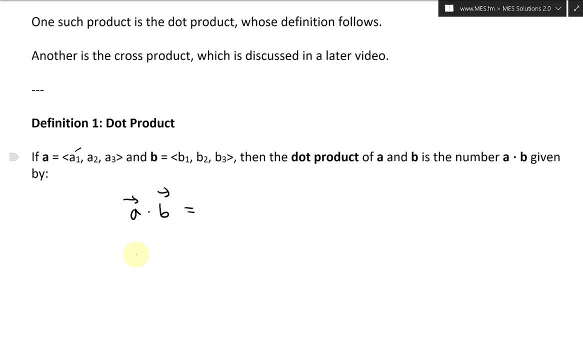 i mean when you're writing. so this is the definition. this one is: we're going to have the components, multiply the a1 by b1, then a2 by b2, then a3 by b3, and add all of them up and we're going to get this. so we're going to get a1, b1. this is, again, this is the definition, and then 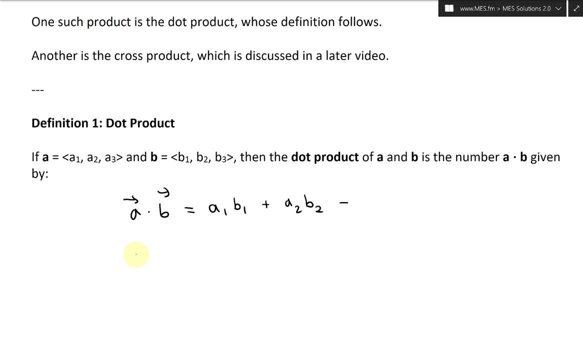 we're going to show that this is an actual useful quantity and this is going to be a3, b3. so notice we have. we have two vectors multiplying our dot product together. so the dot product of two vectors is just a summation of these two of these three. 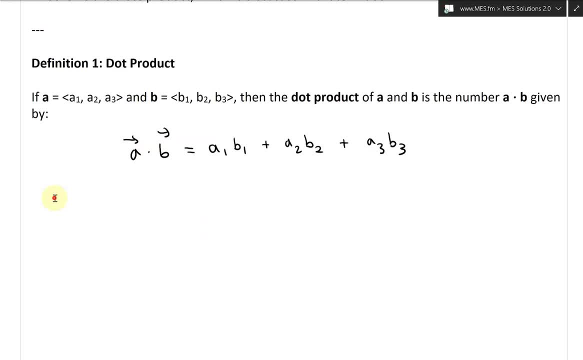 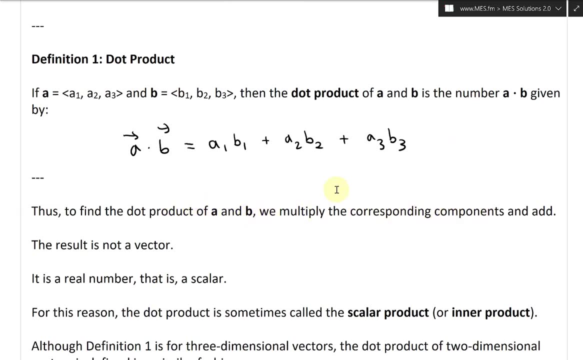 multiplications. in other words, these are: this is just a real number or a scalar, all right. so thus, to find the dot product of a and b, we multiply the corresponding components, as we did over here, and then we add them all together and again, as stated earlier, the result is not a vector, it is. 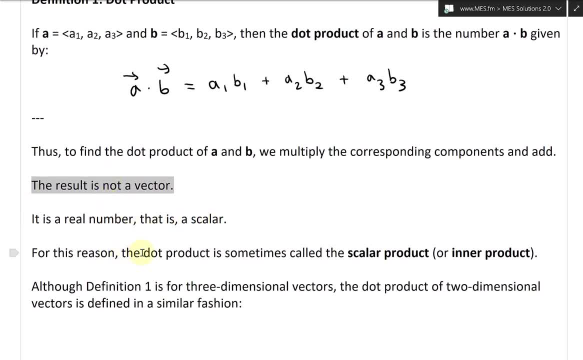 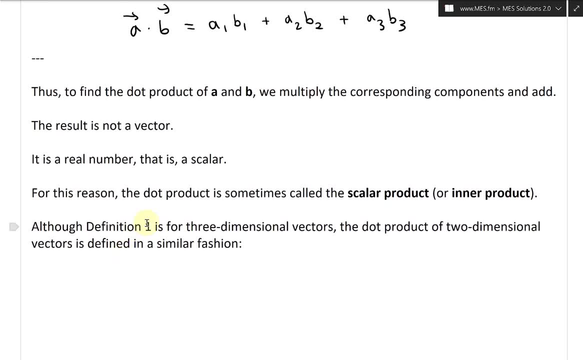 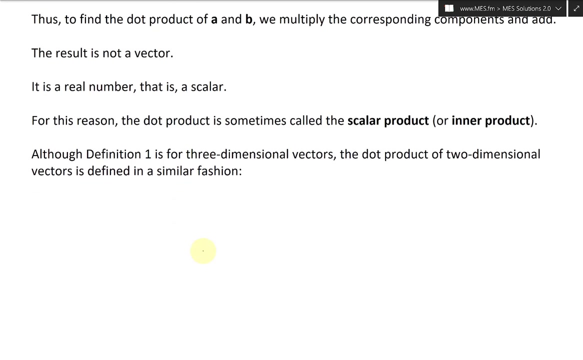 a real number, that is, a scalar. for this reason the dot product is sometimes called the scalar product or inner product, and although definition one here, so this definition one is for three dimensional vectors. the dot product of two dimensional vectors is defined in a similar fashion. so if you have two two-dimensional vectors, so a1, here's the components of them, just. 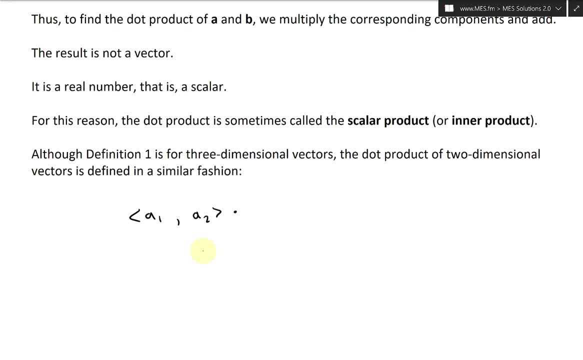 call this a1 and then this is a2, dot product of the second vector, b1, b2 is a two-dimensional one. this just becomes well a1, b1 plus a2, b2, so just the components and so on. you can do this for any number of dimensions. i. 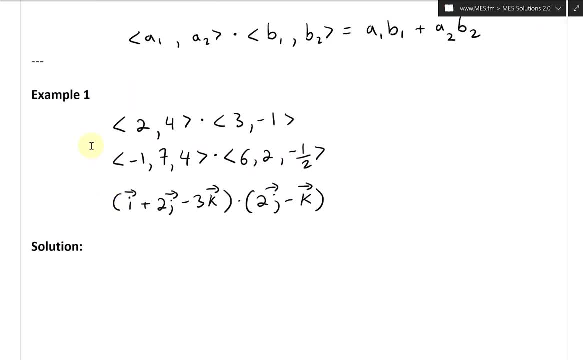 believe. all right. so now let's take a look at an example. so this example one, and this just has three different dot products. who for us to exercise? so we have this two: this vector is two-dimensional to vector 2, 4 dot product three times, and then three, and then 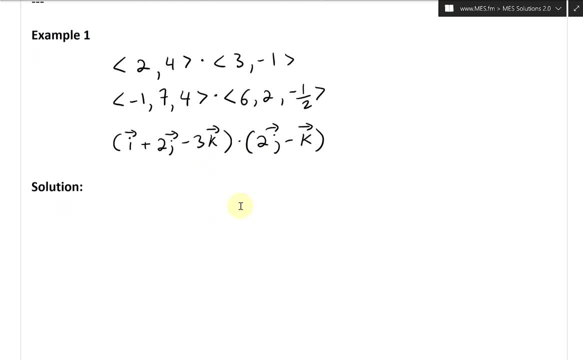 negative one. the other one is: uh, these ones over here, and let's go over each one. let's go over the first one here, which is 2, 4, all right, so let's look at the solution, let's go over it. so 2, 4. 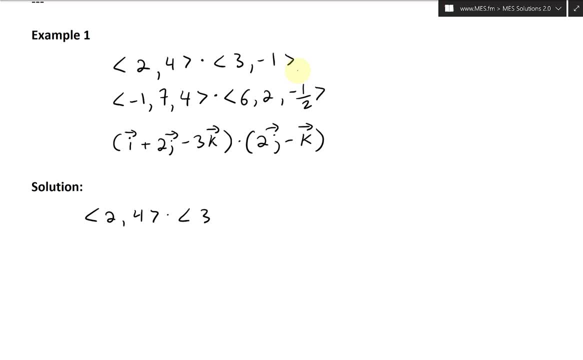 and then dot product three negative one, these two vectors. so this equals to well, two times three plus, and the next one's going to be 4 times negative 1, and this equals to well. this is going to be 6, and then 6 minus 4,, this equals to 2.. All right, now the next one. here let's write: 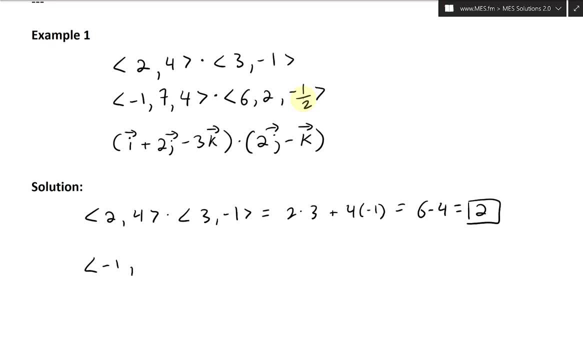 that down. that is going to be negative 7, I mean negative 1, 7, 4, dot product with the three. these are three-dimensional vectors: 6, 2, negative 1, 2, like that. All right, and then this is going to. 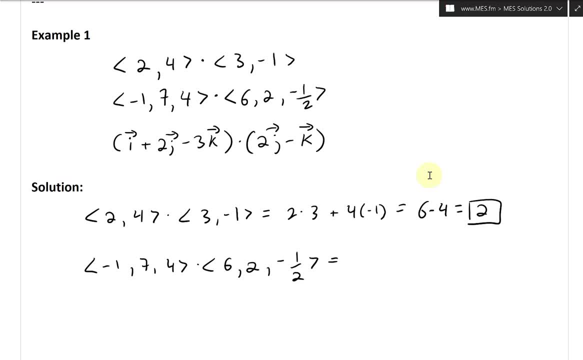 equal 2,. yeah, it's going to equal 2,. well, now we have a three-dimensional dot product, so we multiply this negative 1 times 6, so it's going to be negative 1, I'll put this in the bracket- negative 1. 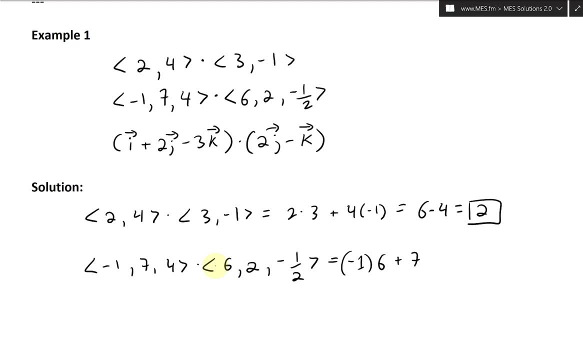 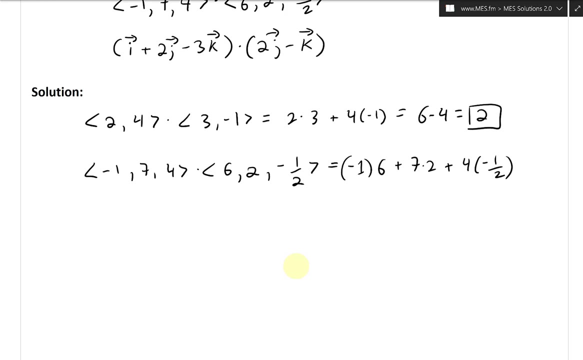 times 6, plus 7 times 2, 7, 2, and then 4, and then negative 1 half. it's going to be times 2.. Then plus 4, negative 1 half. let's add all these together so this equals to. let's put it here: 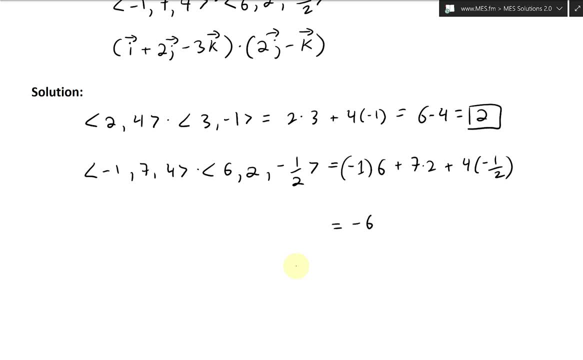 actually make it in line equals to negative 6 plus 14, and this cancels, well, the 2, or, yeah, that's going to be 2,. this cancels this is going to be well, yeah, 4 divided by 2 is 2, and then 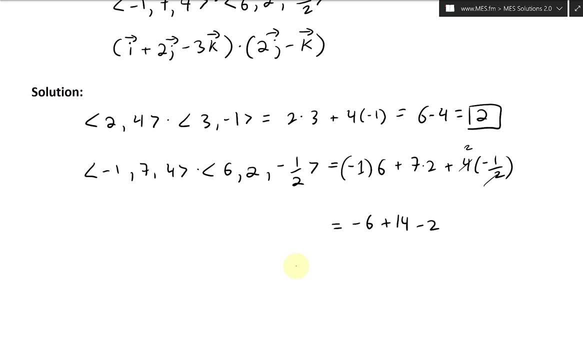 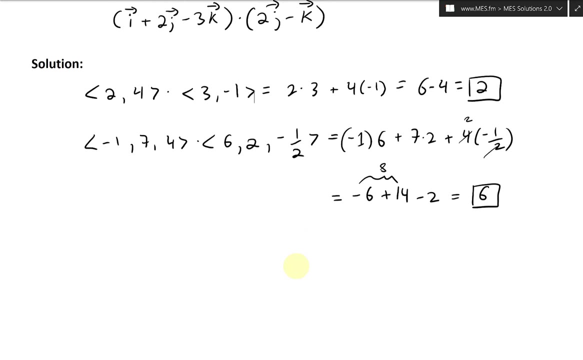 negative 1, so negative 2, like that It's going to be negative 8, or you could just look at this together: what are these together? negative 6 plus 14, or 14 minus 6 is 8,. 8 minus 2 is equal to 6, like that. All right, that's pretty. 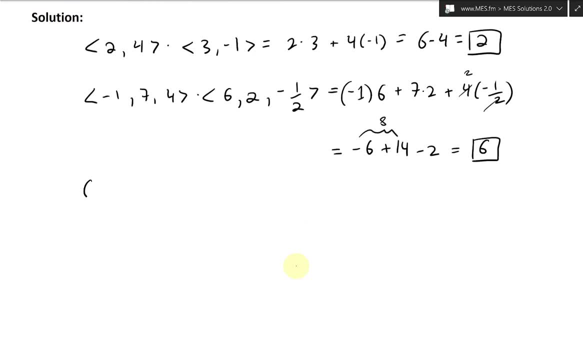 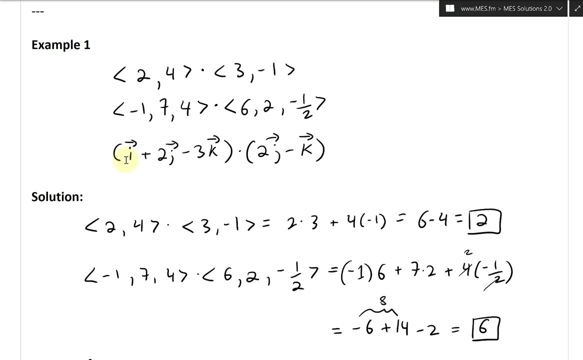 epic. so now let's take a look at the next one. this one is using this standard basis vector form and remember, recall from our earlier video, yeah, from the earlier video, these ones, each one of them, is going to be equal to 6,. so let's take a look at the next one. this one is: going to be equal to 6, so let's take a look at the next one. this one is going to be equal to 6,. so let's take a look at the next one. this one is going to be equal to 6, so let's take a look at. 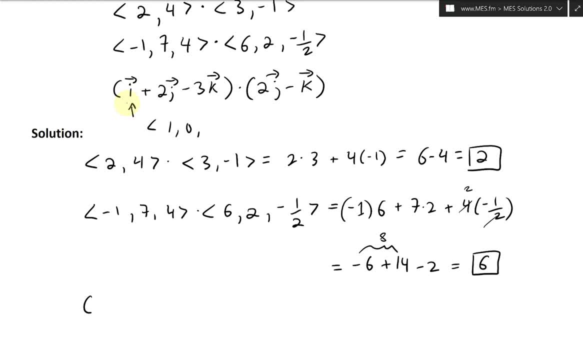 one of these. this, for example: this one here is just a 1,, 0,, 0 vector. the j1 is 0,, then you put a 1 in like that, and then similar for this one is be the k. this would be 0,, etc. so it's each. 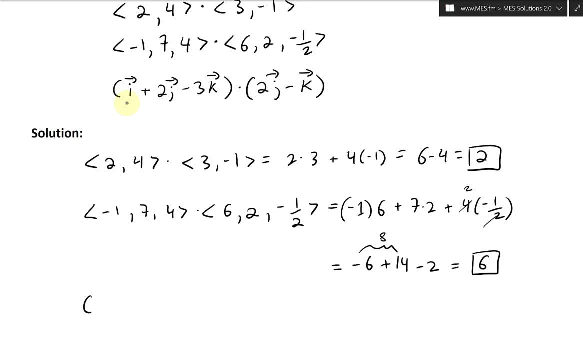 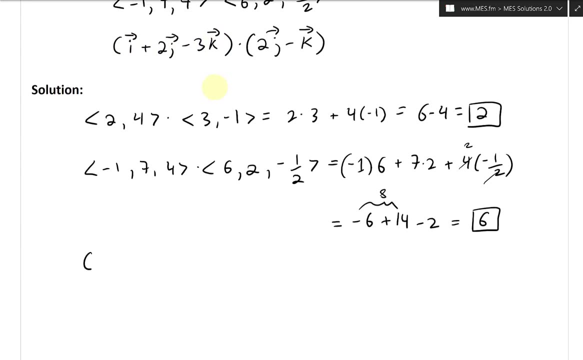 component of those, etc. what this essentially means is: this is the same as writing 1,, 2, negative 3 in this component, but you're writing it in a standard basis vector setup and notice the bracket change because we're writing it in these vectors setup. so what this? 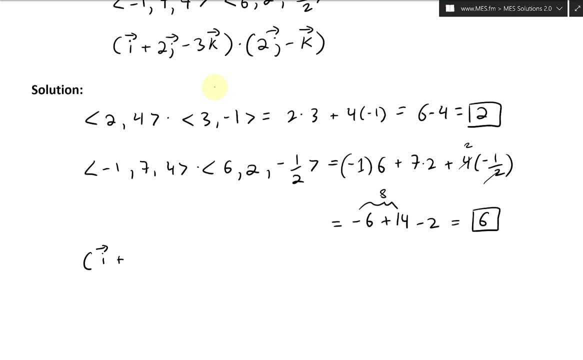 equals to. well, let's just write this out. so we have the vector there, the i vector plus 2 times j vector minus 3k vector. this times by 2j minus k vector, this equals 2, so now this is the. 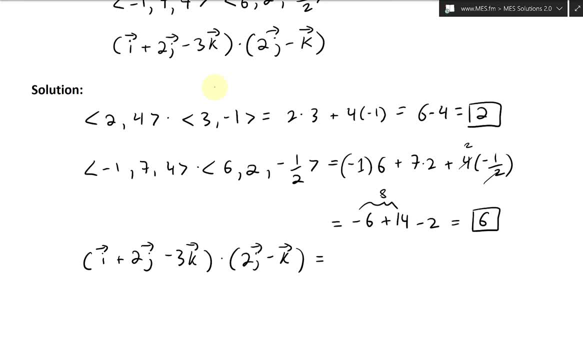 interesting part Here, because this one skipped the i one, and that's because it's assumed that the i is the 0 times by i. so, in other words, when we do the dot product of these two, this i, this is going to be. 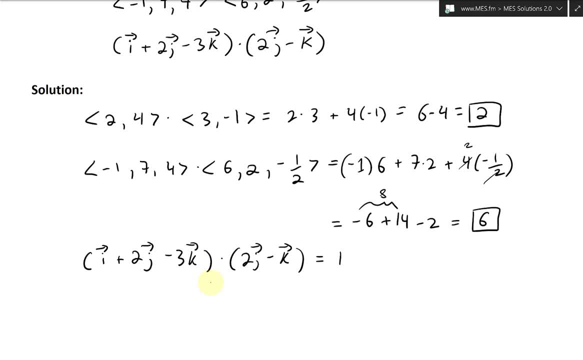 1 times by. well, there's, the 0 is gone there, so we'll have a 1 times by 0, and the next one is going to be plus 2 times by 2,. there's the j's matchup: 2 times 2, and the next one here. 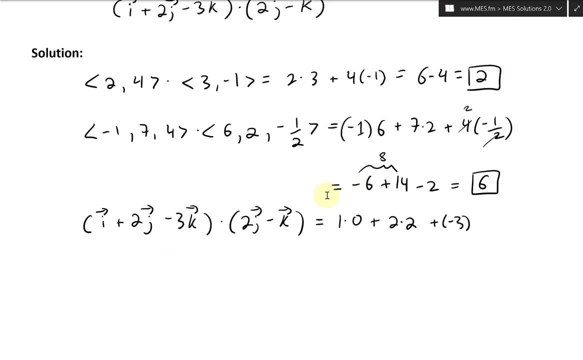 negative 3 times by. yeah, this one is just a negative 1 there, so we'll have a negative 1 like that. so this equals 2,. well, this is going to be 0, plus the next one is going to be 4,. 5 times 2 is 4, then the next one is going to be 2 negatives. 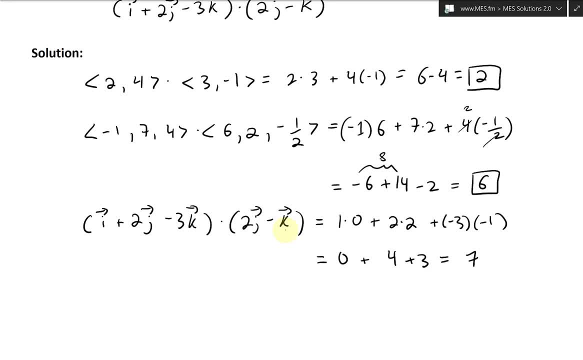 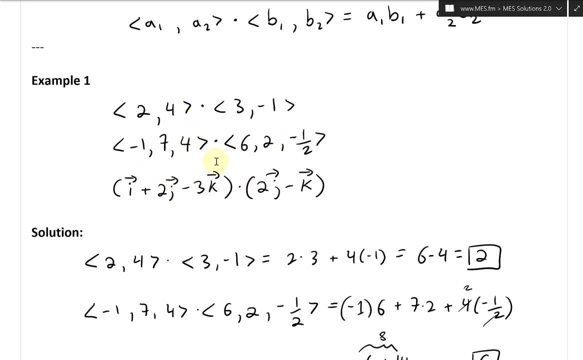 becomes positive plus 3, so in other words, this equals to 7,. so there's the dot products for all three of these. so all these vector multiplication or dot products, and then we get scalar numbers, just real numbers. 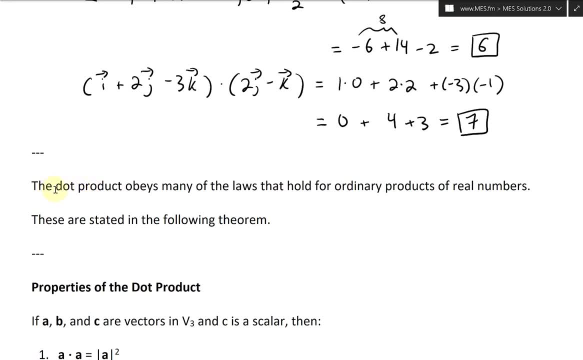 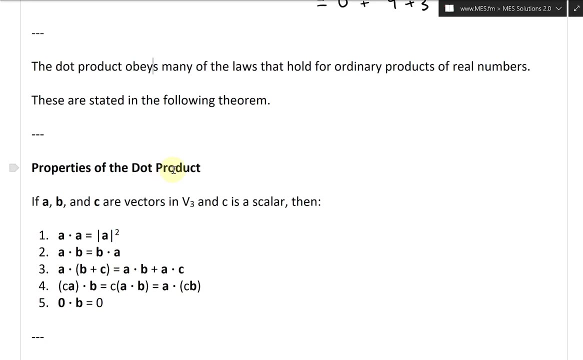 All right. so now let's continue further, and now I'll basically look at some properties of the dot product. So the dot product obeys many of the laws that hold for ordinary products of real numbers. These are stated in the following theorem. So, properties of the dot product. so if the vectors a, b and c are vectors in v3, or, 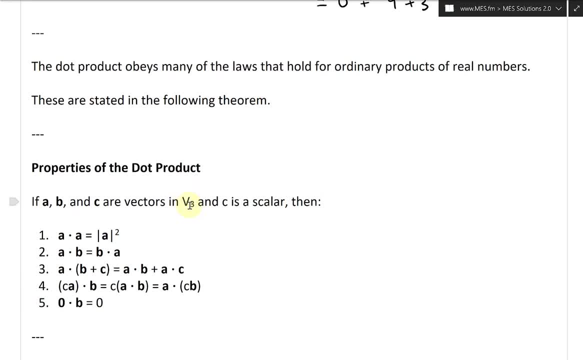 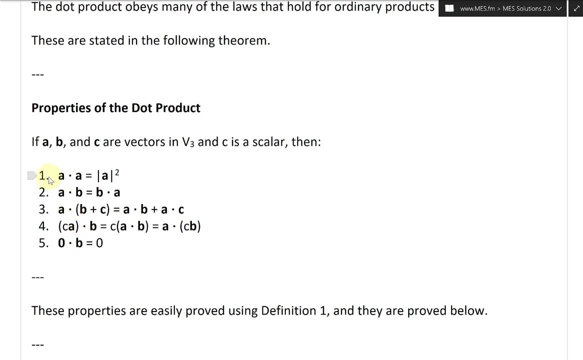 it's just a set of all three-dimensional vectors and c is a scalar. then you'll have these five properties and yeah, and these properties are listed as well. property one aa equals to the length a squared, so the 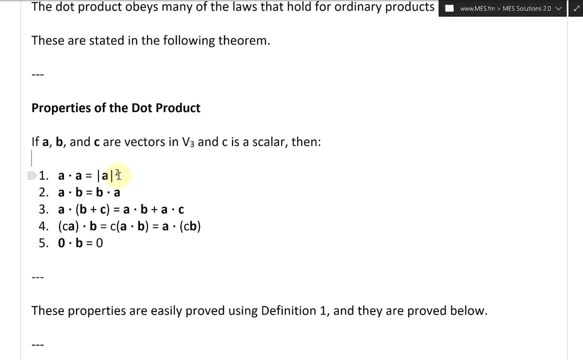 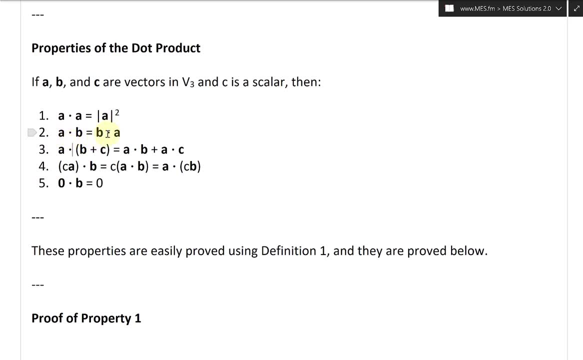 vector a, the distance or the length of it squared, is equal to, just when you have the dot of itself. so aa. and now this property two has ab equals to ba, so you can reverse the directions. you could switch up which one starts first and then property three is a and then b. 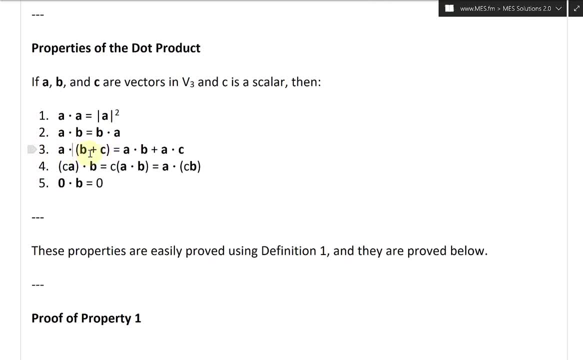 plus c is equal to ab, so you multiply this inside plus ac. And then property four is this again. this property three is just like a real number. you could just, or real products, you could just multiply this out and spread it out. 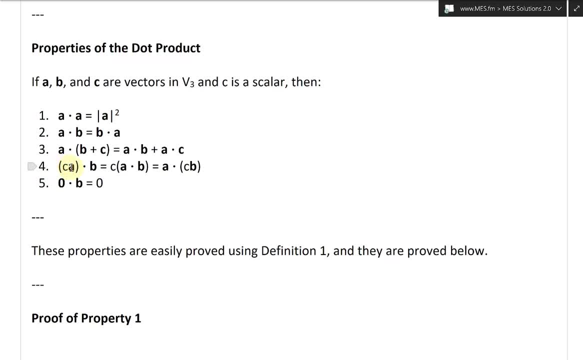 and so on. So property four scalar times a, and then the dot product with b is equal to, and you can just factor out: the c equals to c times by ab, which equals to. you could also put the c inside here, so you could have: 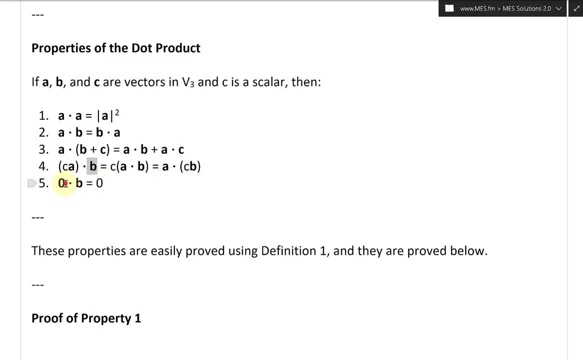 ac, times b. And property five is: if you have the, the, this zero vector dot b, this is equal to zero, a real number, so a scalar number. very interesting. And now these properties are easily proved using definition one, and they are proved below All right. 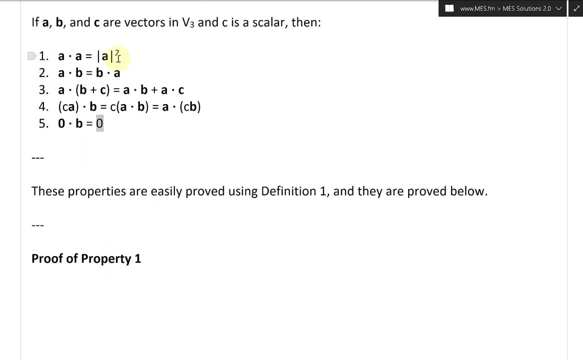 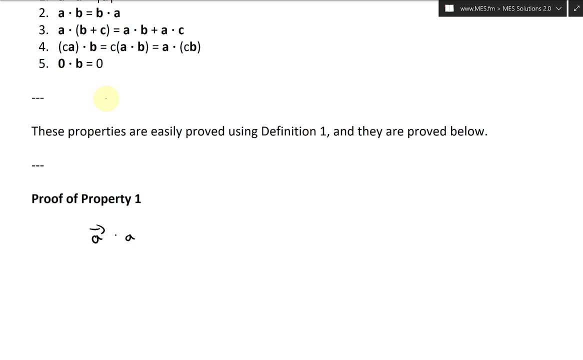 now let's take a look at proof of property, one that's. aa equals to the length, a squared. So let's take a look at that. So you have aa and we'll this in three dimensions. This equals to: well, this is the same thing as writing a1,. 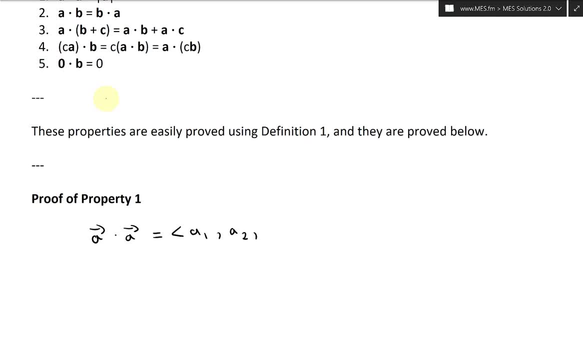 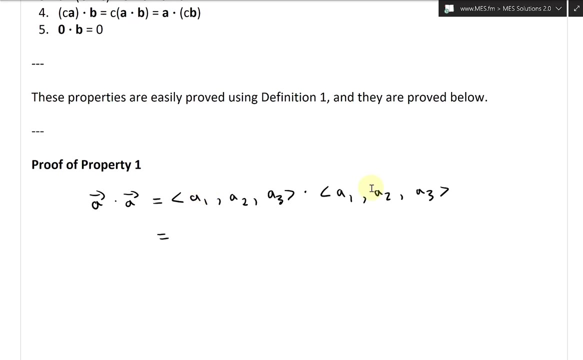 so it's three components: a2, a3, dot, and then it's going to be itself so a1, a2, a3, so we just apply the definition of a dot product. This just equals to well, a1 times a1, that's. 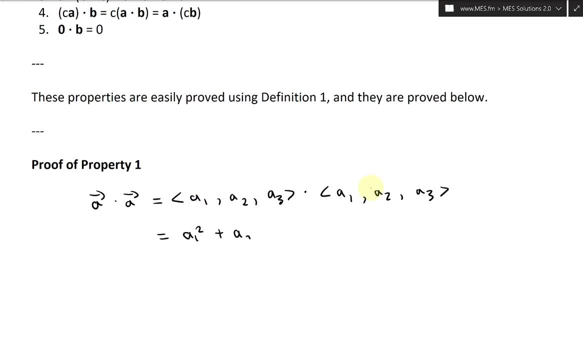 going to be a squared, Then the next one's, a2,, which is going to be a squared, plus a3, squared, and this just equals to. well, this is the length formula. This is just the components of a vector squared. In other words, that's just going to be our a vector length squared. This is 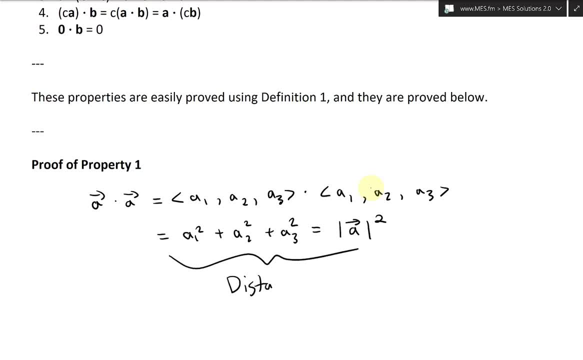 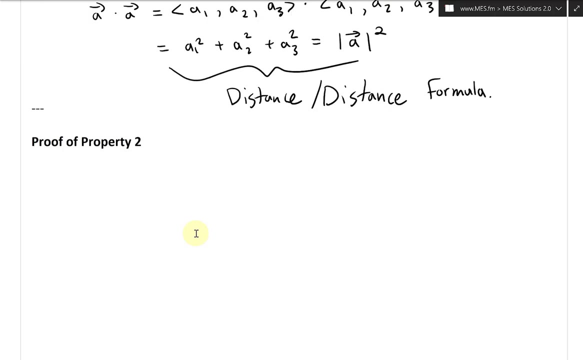 just the distance. yeah, the Pythagorean theorem in three dimensions, distance formula. I'll write formula. All right. so now let's take a look at the next one. Let's take a look at, well, proof of property 2, because, yeah, this is just a distance formula. 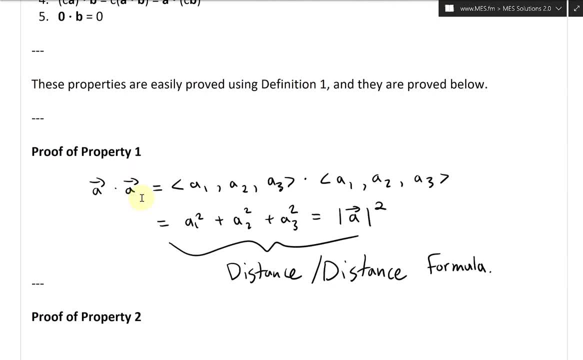 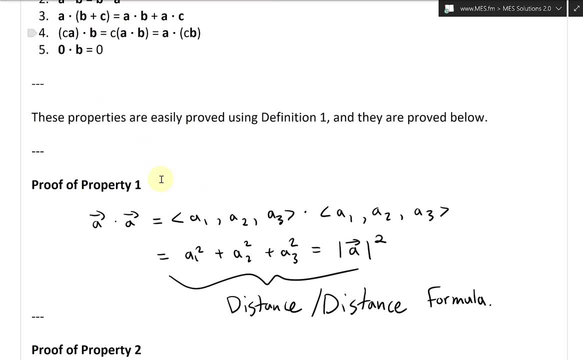 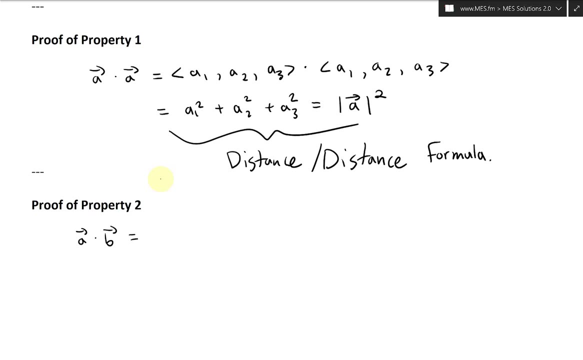 How do you prove that? You can see the earlier videos on that. So proof of property 2 right here. so a dot b equals to b dot a, and again, this is a straightforward one. so if we write a vector dot b vector, again write them in the components. just for completeness, write them all out. 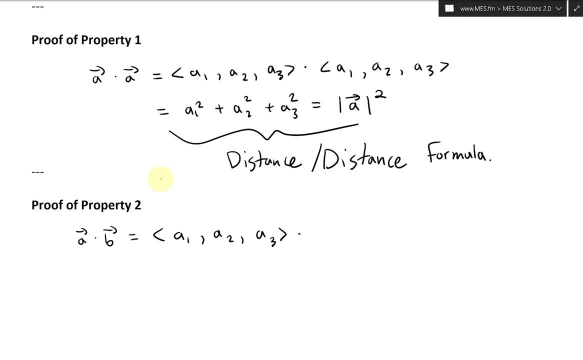 a1, a2, a3, dot b1, b1, b2, b3,. this equals to well, multiply these inside a1 times b1,, just using the definition of the dot product. The next one's going to be a2 times b2, and then plus a3, b3, and then basically. 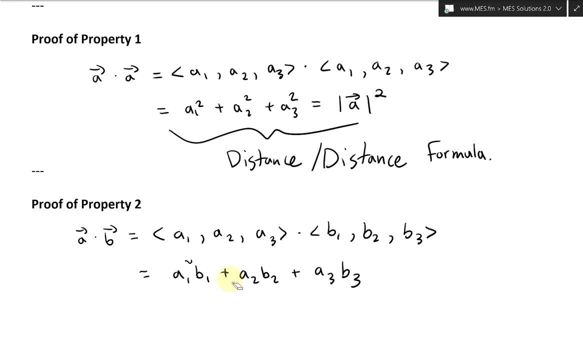 we can. now we could switch these around. You can move this back and forth. In other words, just use the regular multiplication properties and you can just switch them around. These are just real numbers. You can go two times three or three times two. Those are always going. 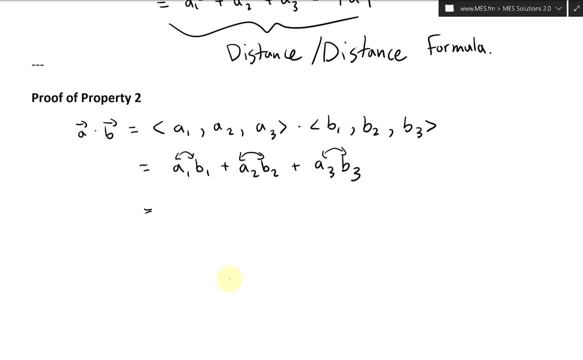 to be six, So we could switch these all around. So this equals to. this equals to b1, a1, plus b2, a2, plus b3, a3.. All right, and in other words, this is just the definition of a dot product. 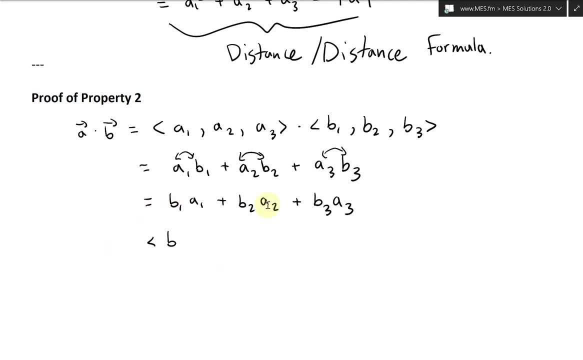 for the vector in the front. so b1, b2, b3, those components b1,. this just equals. I'll just move this equal sign there. this is going to be b1, a1,. oh, whoops, not a1,. 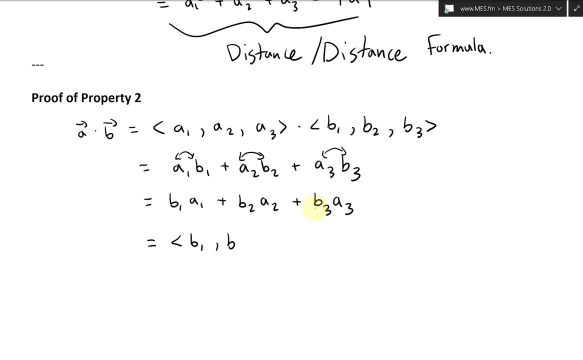 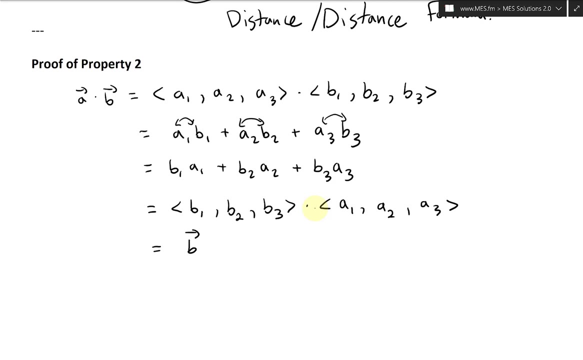 this is going to be b1, b2, b3, dot. a1, a2, a3, dot. yeah, bracket like that, Yeah, so in other words, this is just the b vector, dot, a vector Like that. Move this down here and scroll bracket. All right, so now let's take a look. 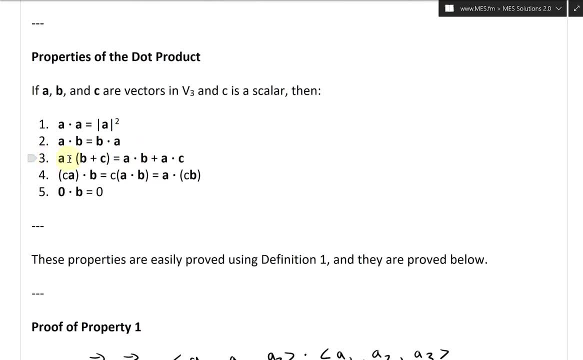 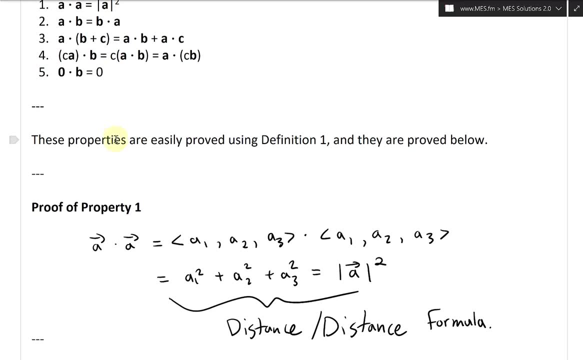 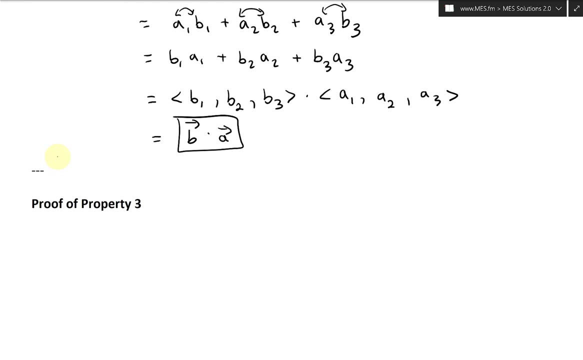 at proof of property three. This is one right here: a dot and then b plus c equals a dot, b plus a dot c, like that. All right. so let's just write this out again using the definition. So, proof of property three, we're going to write a vector dot and then it's going to be b plus c. 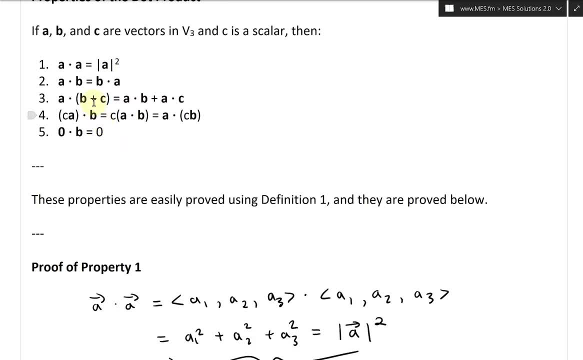 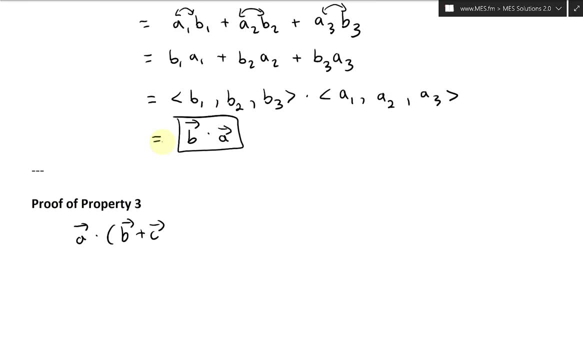 and show that we can multiply that inside. So again b plus c there, And we have to show that you can multiply this inside and foil it out. All right, so a vector times or dot b plus c vectors. this equals to in the component parts a1, a2, a3, like that. And then the next one. 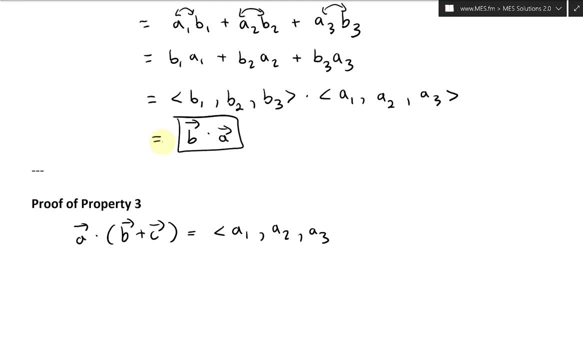 b plus c in their components. those are just adding vectors, And when you add vectors you add each component. So this can be b1 plus c1,, then b2 plus c2, and then b3 plus c3, like that. All right, and now we can just apply the definition. 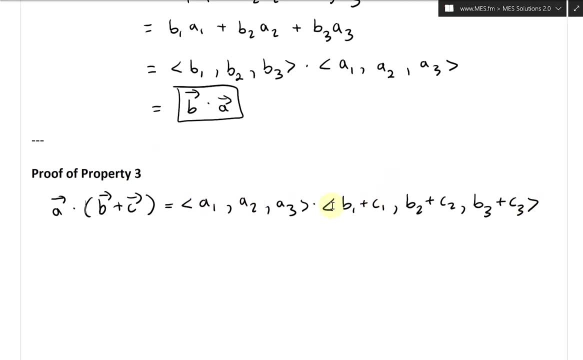 of the dot product. So multiply this a1 over here and then each component is multiplied and then add it all up, So this equals to a1 times by b1 plus c1, and then plus a2, and then b2,. fix this up: a2, b2 plus c2, plus a3, b3 plus c3, like that, And just fix this up like: 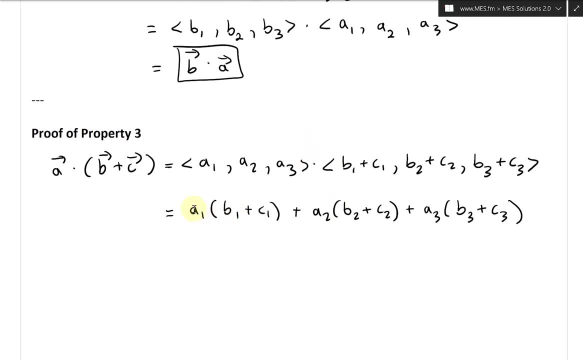 that That's what we have, And now what we can do is multiply this inside each one, just regular multiplication. So now we basically use a dot product, use a definition to get to the real numbers set up and now we can apply the regular product rule. 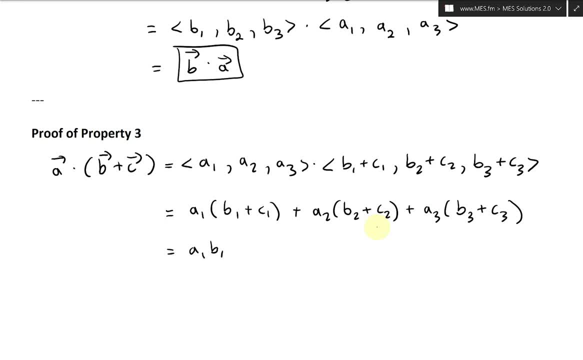 So a1 times b1.. So what I'll do is I'll write a1 times b1 here and then the a1 times c1 over here elsewhere. I'm going to write it over here: a1, c1, and then we'll have this a2, b2 over. 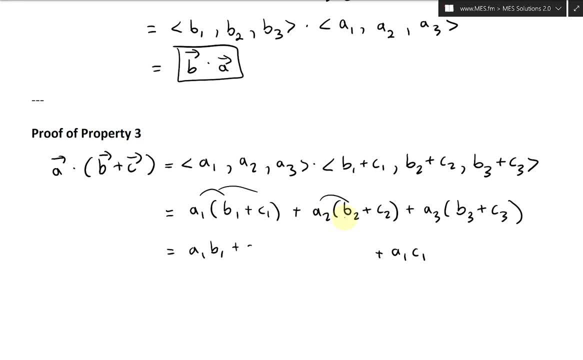 here and another one over at the side. This is going to be a2, b2, and then the next one, a3 plus b3.. Just so it's all together. Yeah, so we have those components, First plus, and now we'll do all these second terms: a1 plus c1.. a1 plus c1 plus a2 times c2. 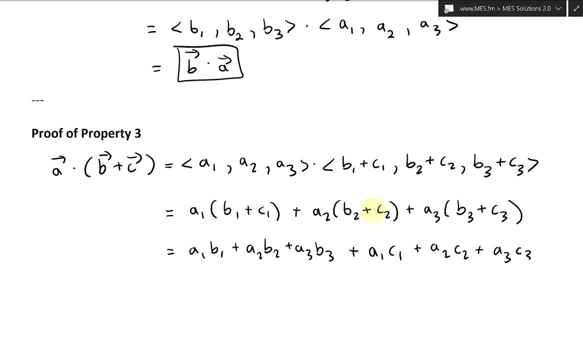 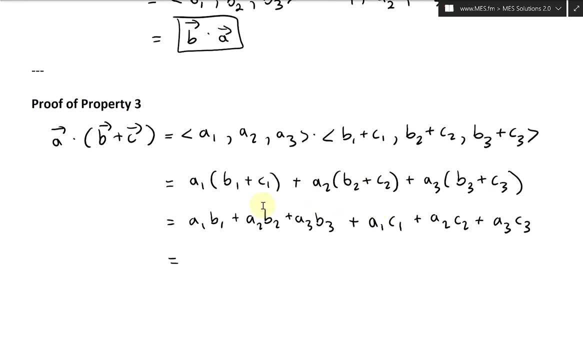 plus a3 times c3.. All right, and now this equals 2.. This is: yeah, this is just the. I'll put a bracket like this. So this is just the dot product for the a times b vector and this dot product from a times c vector. So this just. 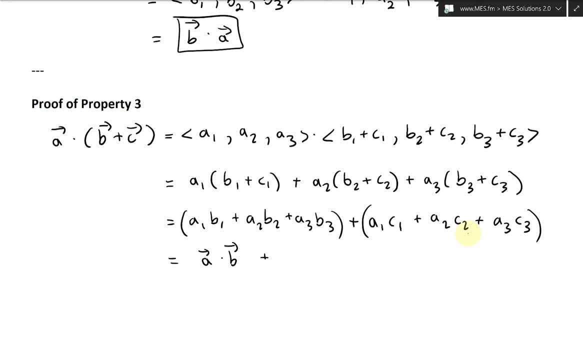 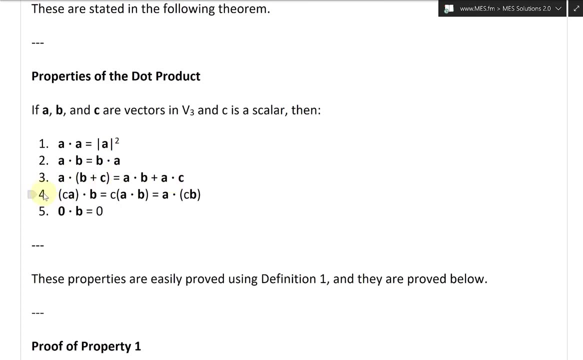 equals to a vector times b vector plus a vector dot c vector And yeah. so hence we've proven our property like that And yeah, so just scroll up here and yeah, there's the property we proved. And now the next one, property four: we'll look at c, the scalar c, times a, and then dot product. 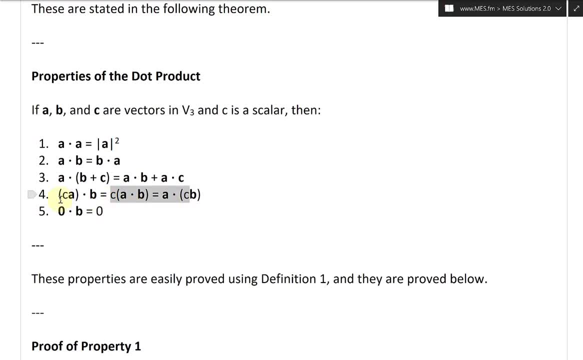 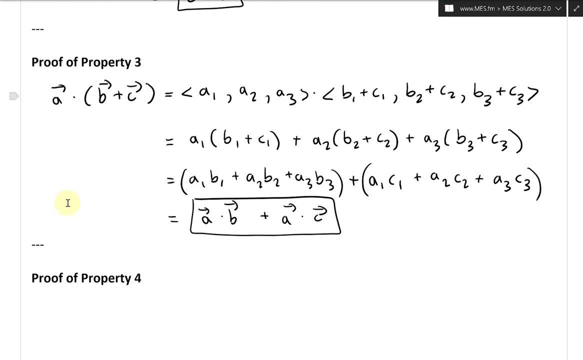 with b, But it equals these two. You could take the scalar out, or you can move it over to the b side, and so on. So that's property four. All right, so let's write this down here. This is property. 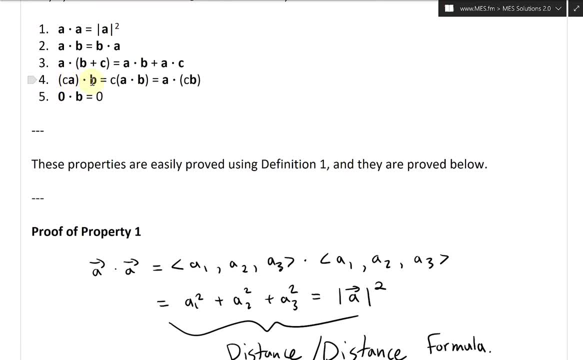 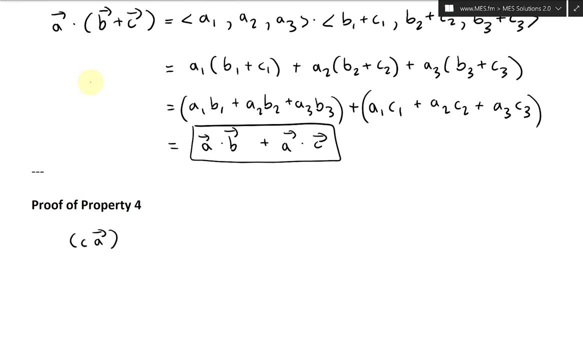 four. Again, that's the scalar c times a and then dot product with b. All right, so we have c a and then dot product with b, vector This equals 2, and write these in the components. This is scalar times it by. 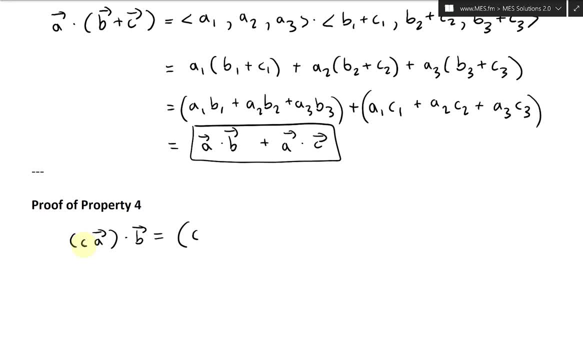 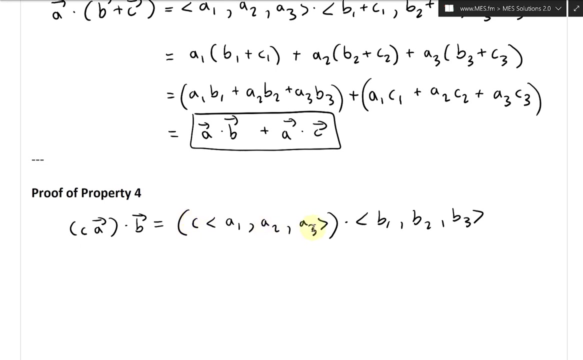 yeah, so we'll have this bracket like that: c times it by and then the components of those vector a1, or just write it in the component form a2, a3, like that, and then dot components b1, b2, b3, like that. And now what we could do is, well, the scalar, we can multiply that inside as. 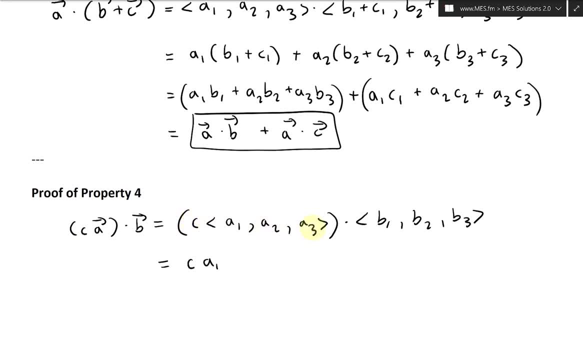 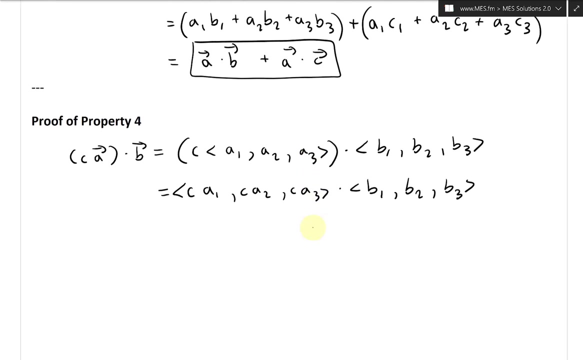 we showed in my earlier video: c a1,. put this bracket like that, and then we'll have this c a2, and then c a3, and then, yeah, just remove that out. then b1,, b2,, b3.. And now what we could do is, yeah, do the dot. product definition. 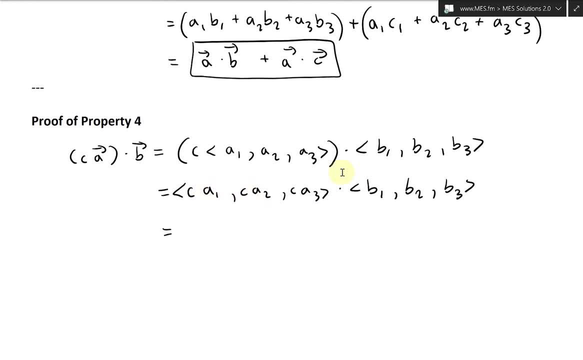 so c1 times c, a1 times b1, that becomes well c a1- b1, and then plus c a2, c a2, b2, plus c a3, b3. Like that. And yeah, that's what we have there. 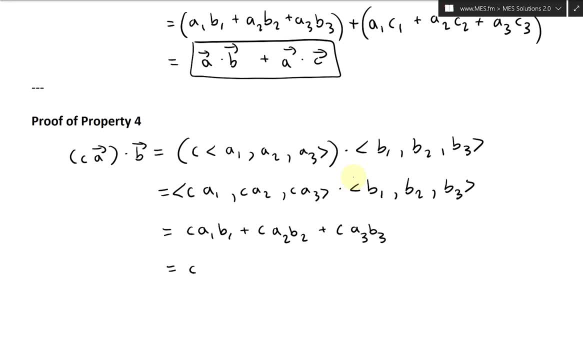 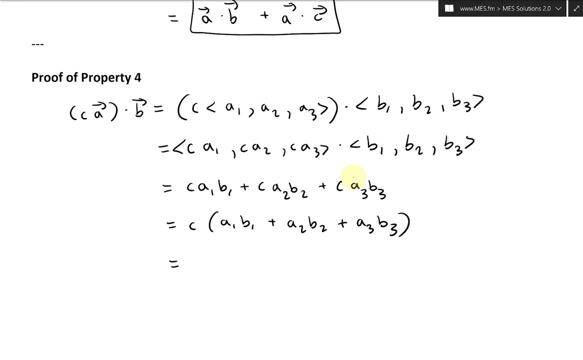 Now we can factor out the c and this just equals to c, and then a1, b1, plus a2, b2, plus a3, b3, and again, this is just this, is just basically. this is just C times, and this just becomes C times. well, the, this is the definition of the dot product for a. 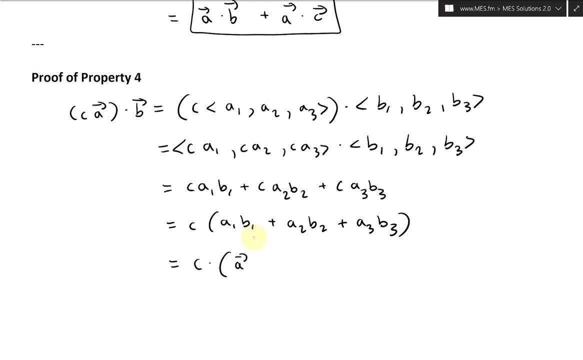 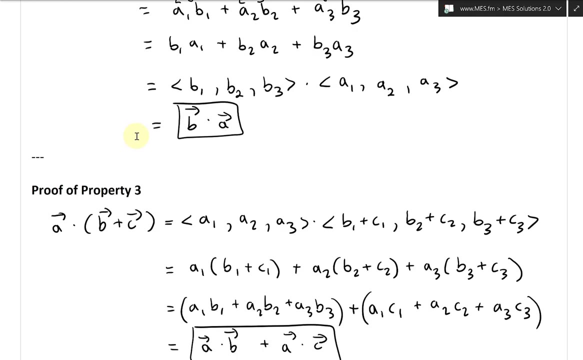 times or a dot B vectors. so a dot B, in other words, we factor out the C out of there. that's what we have, that's proof, those of the middle part of the property, that's this one right here. so we show that it's a scalar times. a dot B and or. 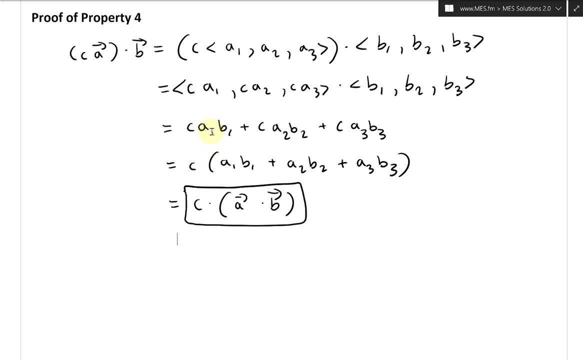 instead of doing this one, we can multiply the C, or going over here, yeah. or instead of here this one, here I'll move the C inside here, because these are all just real numbers. you can move the C over to inside there. so we could do, or I'll put an or sign, or this equals to a, 1, and then C, B, 1, just move those around. 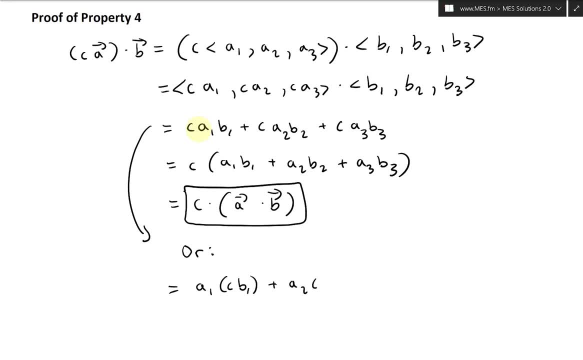 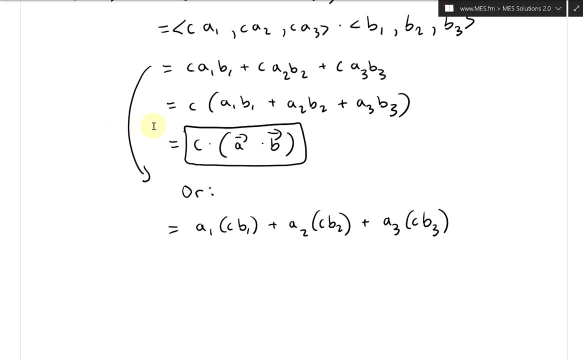 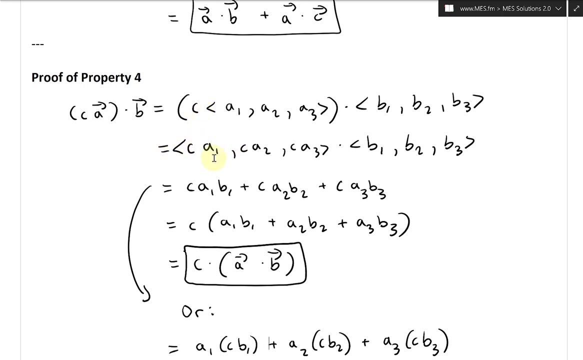 plus a 2, C that. or a 2- C, B 2 plus a 3 C, B 3. yeah, and this part right here. again, this is going backwards. this is the this part, right here. yeah, you could write it in this one in this form, except the C. 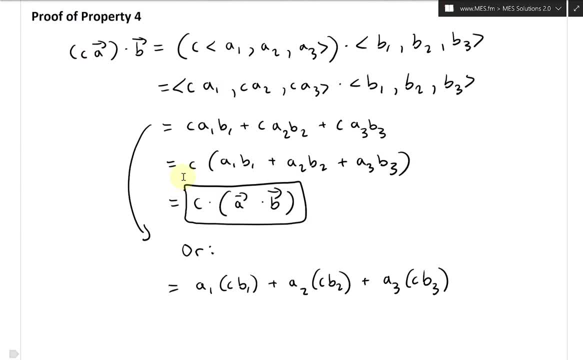 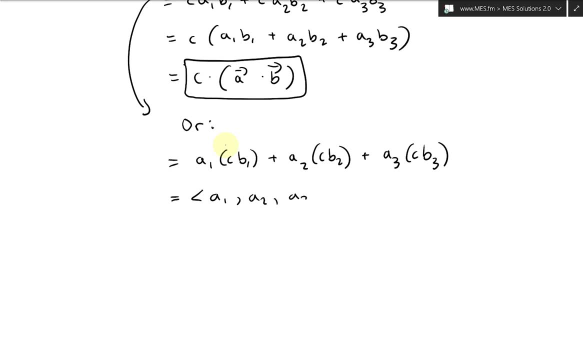 becomes on this side here. so in other words, yeah, just for completeness, doesn't make it match this set up here. this is equals to the vector with components a 1, a 2, a 3 and this is going be dot C. I'll put the C B 1, C B 2. 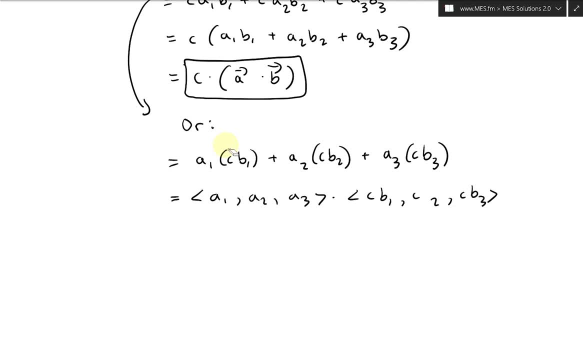 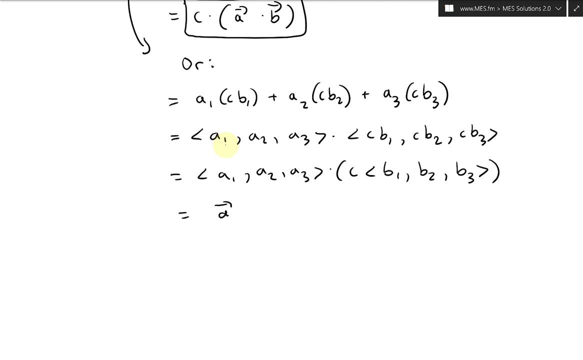 CB, 3, etc, like that. and again, just for completeness, I'll just write this: a 1, a, 2, a, 3, dot. and factor out the C and put a bracket here, so C bracket, B 1, B, 1, B, 2, B, 3, like that, and this is equals to a vector. 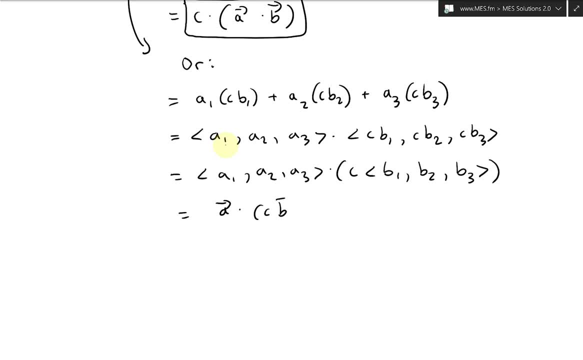 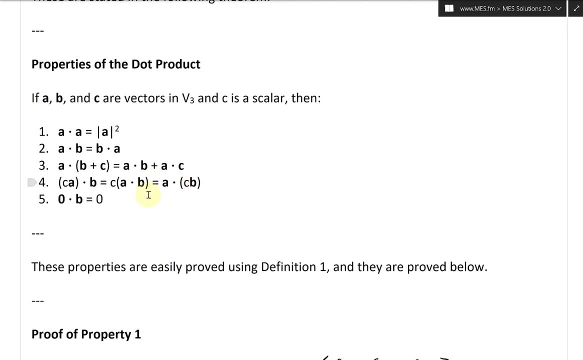 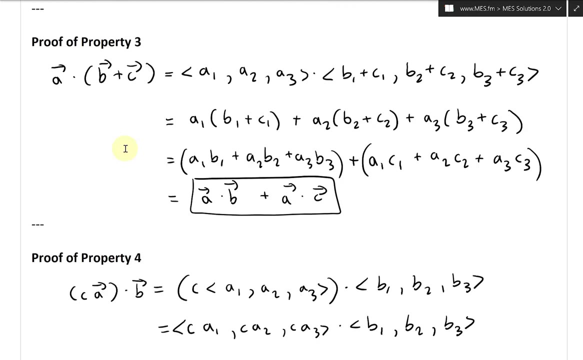 dot bracket C B vector like that. all right here. so we just proved this setup right there and that is property 4. all right. now let's take a look at property 5 and that is just a 0 vector, dot B, and let's show that it equals to 0. all right, 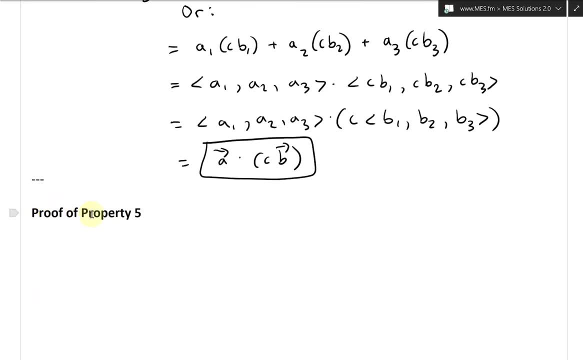 so let's jump right here. so proof of property 5. this one's pretty straightforward again: a 0 vector dot by a vector- this just equals to the component of 0 vectors- is 0, 0, 0 dot, and then we'll have 0. 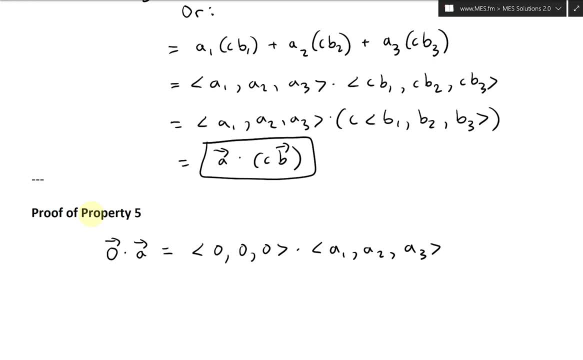 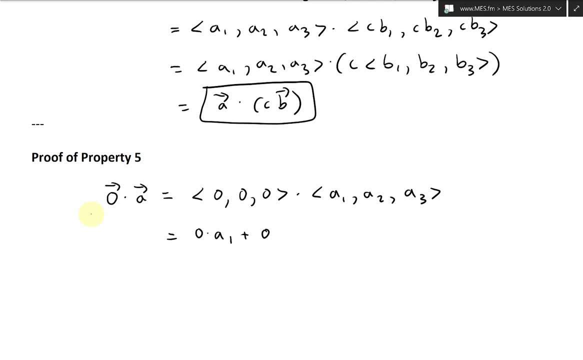 a 1, a 2, a 3, like that. in other words, just use the definition 0 times every single one, 0 times a 1 plus 0 times a 2 plus 0 times a 3, this is equals to 0. so real numbers. is your vector dot any of. 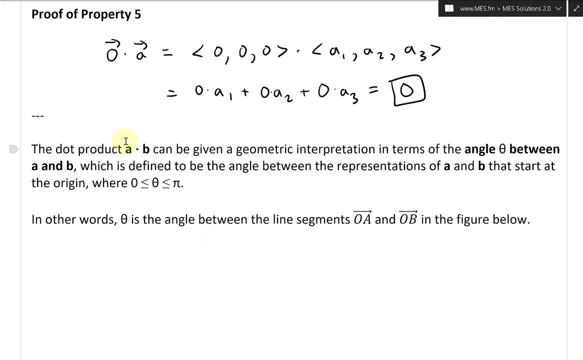 any vector just becomes here, all right. so now that we've covered all the properties, let's continue you further. so the dot product a, dot B, can be given a geometric interpretation in terms of the angle theta between a and B, which is which is defined to be the 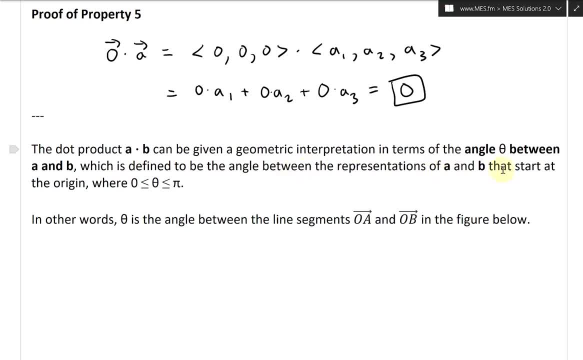 angle between the representations of A and B that start at the origin, where theta is between pi and 0. so it's greater than, equal to, greater than or equal to 0 and less than or equal to pi, in other words, when 180 degrees, all right. so in other words, theta is the angle between the line segments o, a. so 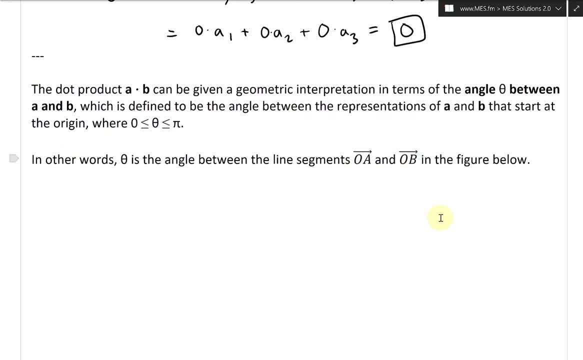 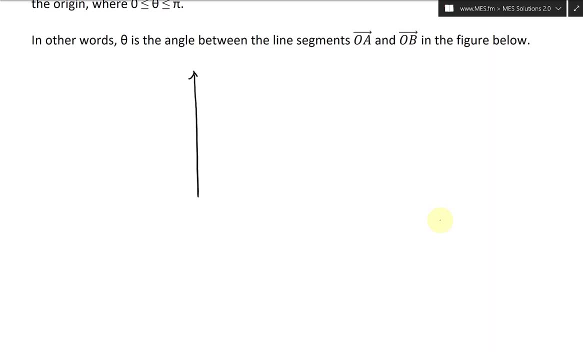 from the origin to a and o b in the figure below. so it will have is like this: all right, so let's draw this as the z axis, this is the y axis and this is the x axis. all right, it's the origin, and then this is going to be the b vector we'll go to, so i'll draw this first. this is the a. 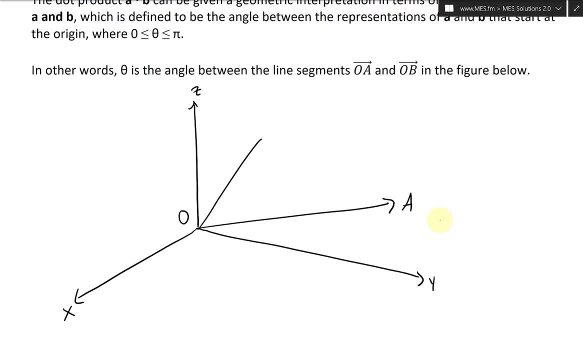 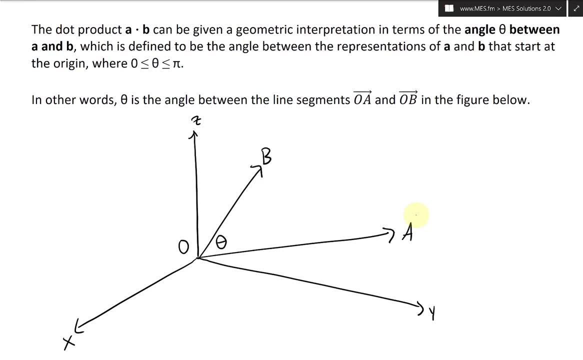 that's a, so we're going to a. uh, and then yeah, let's say that's the a, this is going to be all right. so there's the o, a, so this angle, theta is there. and if this is yeah, so this is going to a, let's say the origin: this is the vector a and this is the vector. 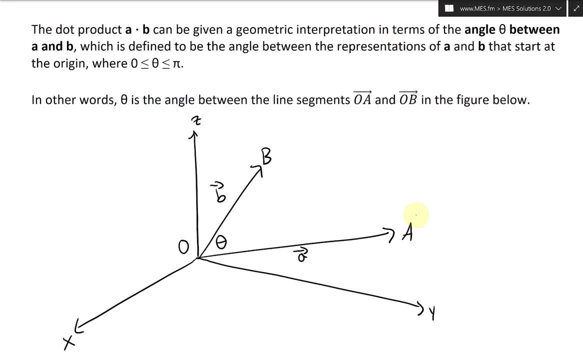 and this is the vector b: b. remember the vector there? a and the arrows definition. this is just a minus b, like that. and yeah, here if you add a plus a, minus b, we'll actually have the arrows the wrong way. so that's a, this is our a minus b, like that. and this is because when you have these vector the way it's. 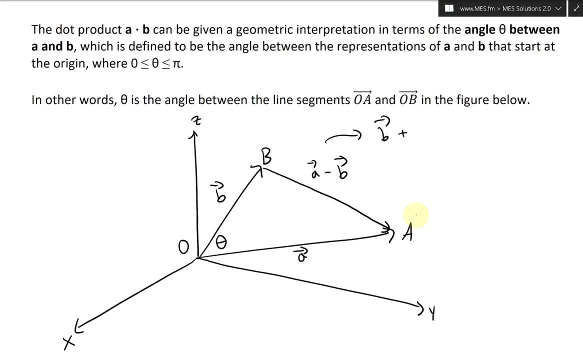 set up is: well, if you have a, if you have b plus, uh, this vector, a minus b, like that, this equals to well, this cancels, this cancels. we're just left with a. so that vector there, going all the way over, there is going to be a minus b, and here we will show that we can give this dot, product a. 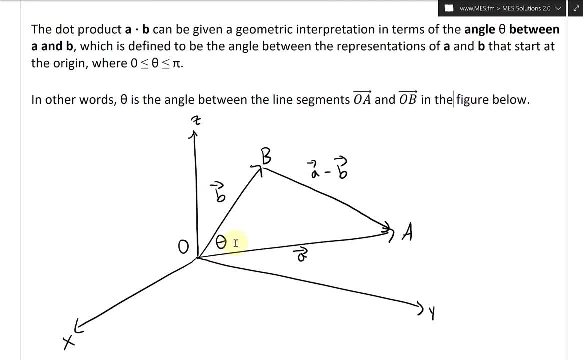 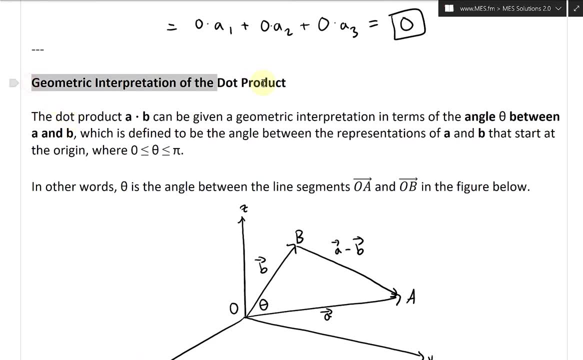 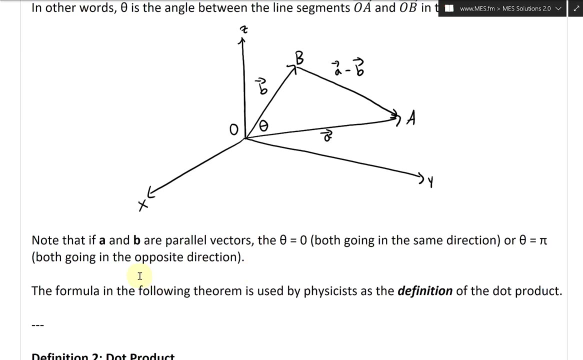 geometric uh interpretation using this setup, where that's the angle there between these two vectors, like that. all right, let's continue further and here's out of this uh heading there's a geometric interpretation of the dot product- and also include that in the topics to cover later, um or in the time stamp and 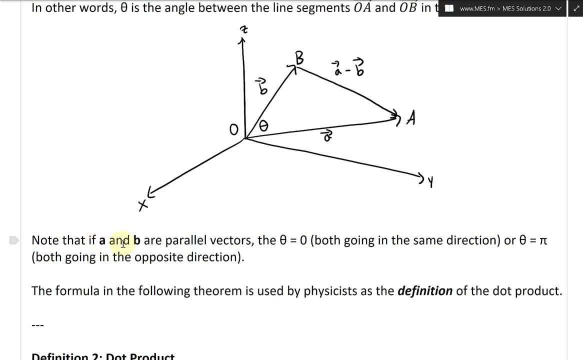 so on. so note that if the vector a and b are parallel vectors, that is, they're all going across the same way, like that, then the angle theta is equal to zero, so both are going in the same direction. but if it's uh, but if if theta is equal to pi, both going in the opposite, yeah, 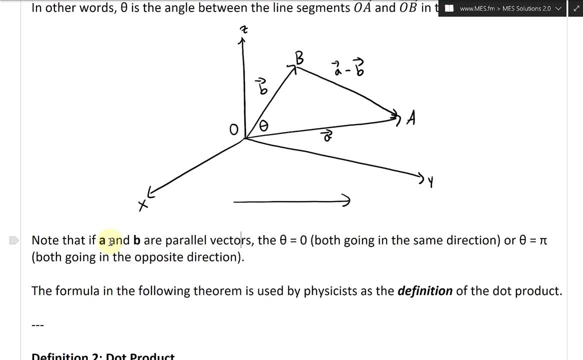 or opposite directions. or in other words, read this: probably so. if vectors a and b are parallel vectors, uh, the angles theta is equal zero, going in the same direction, or it's going in the reverse direction, and that is going to be. our theta equals to pi or 180 degrees. yeah, and it's going. 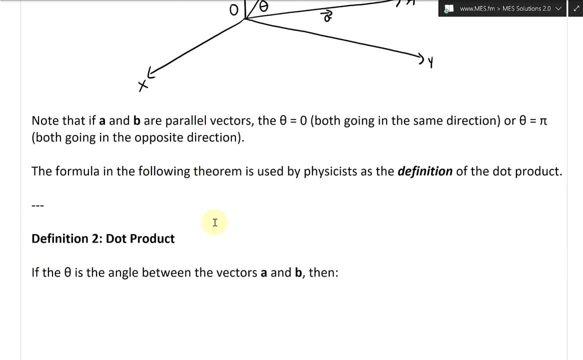 backwards and it's parallel nonetheless. all right. so the formula in the following theorem is used by physicists as the definition or quote definition: uh, or it's an intel italicized uh word here, uh, italicized definition or a definition in italics of the dot product. so this is typically how physicists define it: the definition two dot. 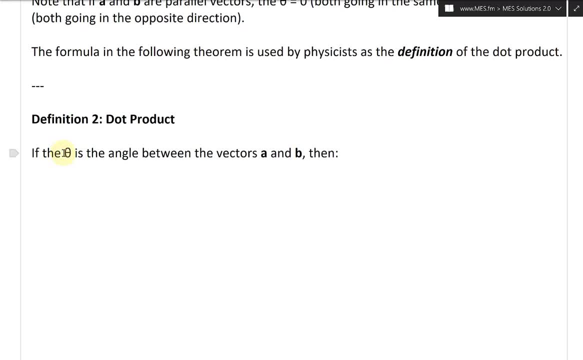 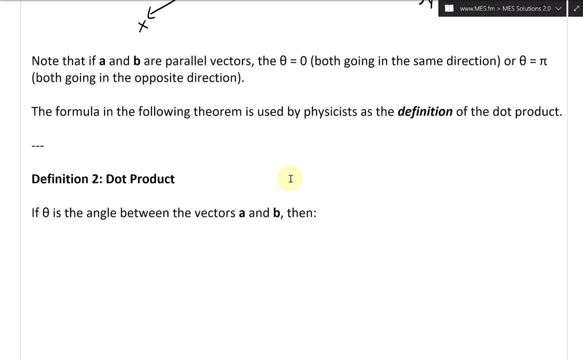 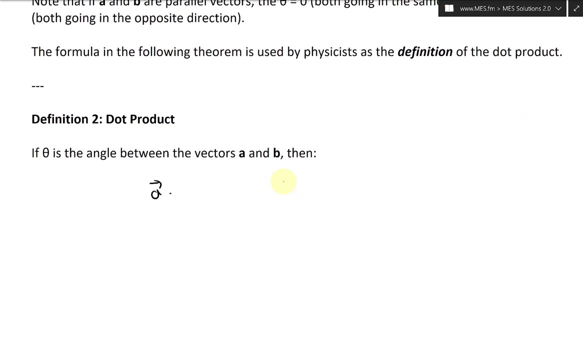 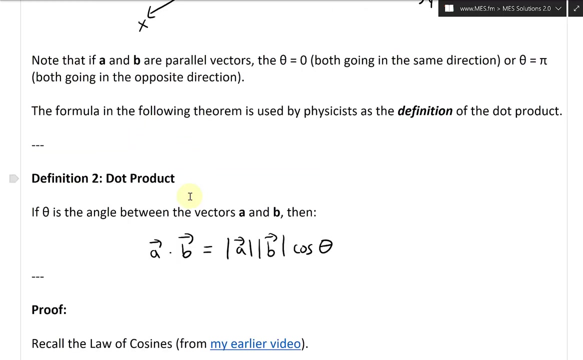 product, if the uh, if, if the angle theta or if theta, yes, so if theta is the angle between the vectors a and b, like this uh, then this is defined as a dot. product is defined as uh. a, B equals to the distance a or the length a times it by the length B as by cosine theta. all right, 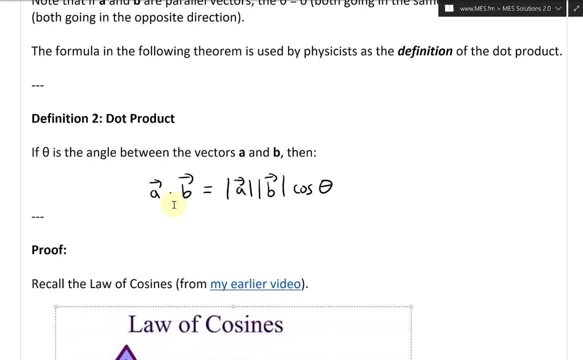 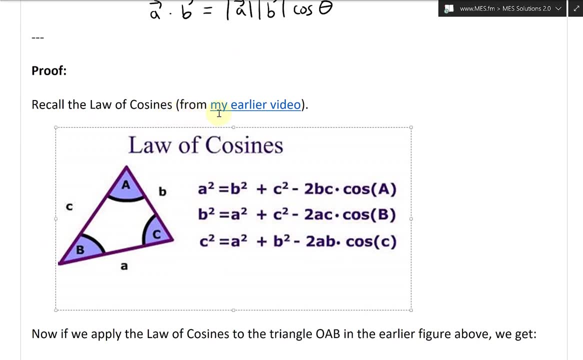 so that's the definition there, but we'll show that it. this is actually equal to the dog product as we defined earlier. so up proof here. so recall the law of cosines from my. this is sort of link from my earlier videos, the law of cosines, and you're just find this a random image online, so if you, 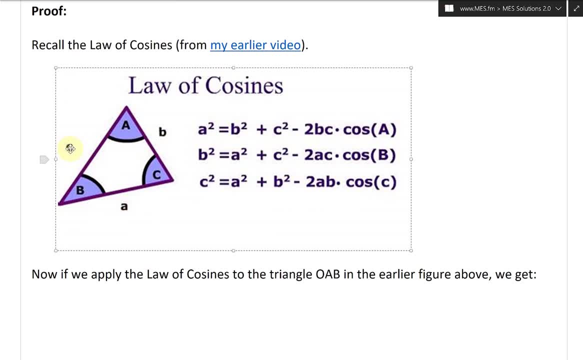 have a triangle, so as length, sides a, B and C, and then angles, capital a, capital B, capital C and so on, then you could plug in this formula for any of the three sides when you have one angle. so if you have this angle a, then you can determine a. well then, a squared plus B squared plus C, squared no. 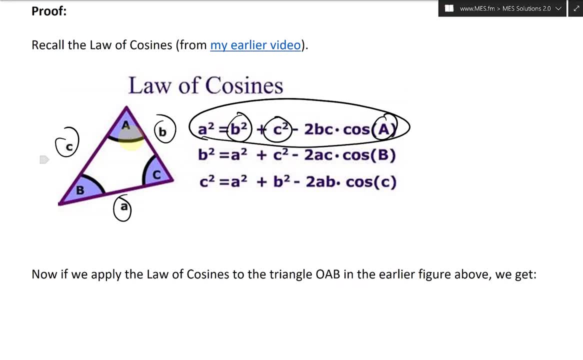 a squared equals to B squared plus C squared minus 2. a, B, C cos a, so and so on, and this, this applies for all of them. so for B, for the angle B, you're gonna have a. yeah, this is gonna be so, this is the B there. so you're gonna have a squared plus C squared, and 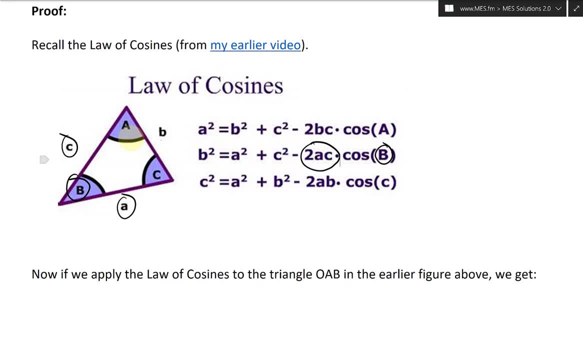 then 2 a, C, and yeah, that's what this B squared is equal to and like, and likewise for the angle C here. so you have C here. so C squared is this, and it goes to D squared, and then minus 2 a, B, these two, and then there's a C like that anyway. so that's. 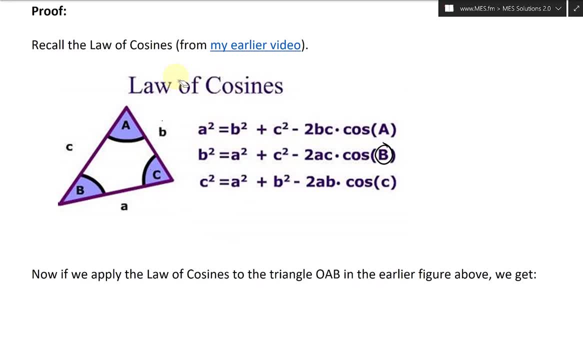 a law of cosine. so now, if we apply the law of cosines- and I'm gonna prove that in my earlier video- so now if we apply the law of cosines, yeah to the triangle o, a, B in the earlier figure above, we get. so this one right here. so we have this angle theta, and then we have these lengths side. 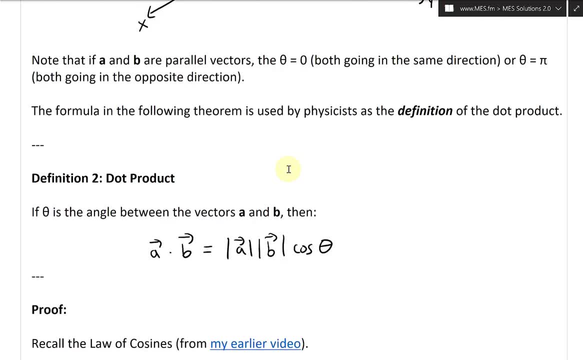 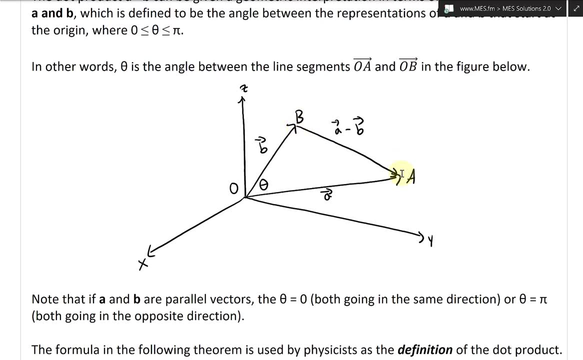 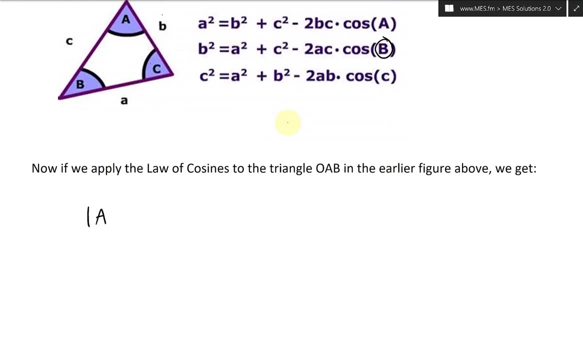 there there's this: o, a B set up there so we could apply the law of cosines. we know this is a angle, so we're gonna write this one squared, or I'll just write: write this as a B. I'll just call that a B, that length or that distance there. yeah, so I'll write it as a B. so we're without a vector. 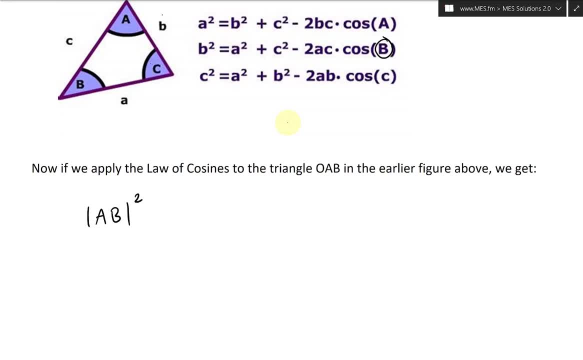 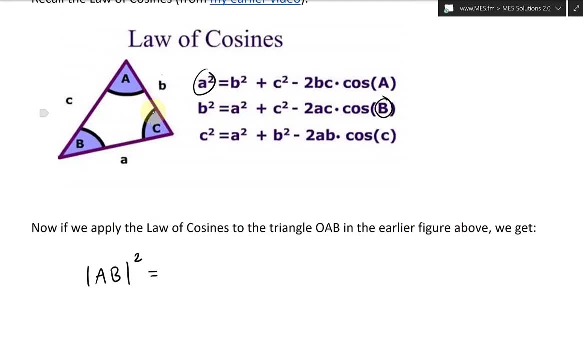 form, just me, the absolute value of the distance a, B squared is equal to. so when you have that, then so if this is a, B, for example a, let's do this one here you're gonna have. this is gonna be our a squared is over here, then these two sides squared, so we're gonna write this one squared, so we're gonna. 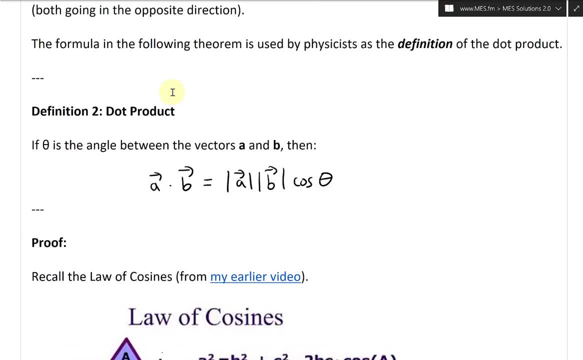 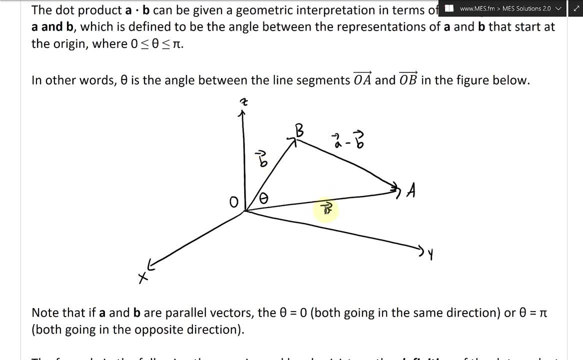 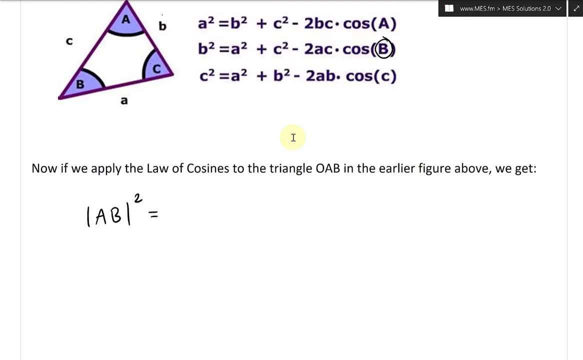 write this: one squared and then plus two to BC, etc. so this case, in this case we're gonna have, so this one squared is equal to a squared, and then, yes, so the length of a squared plus the length of B squared, or we'll call this o a and it's OB like that, so it's gonna be right here- o a squared. 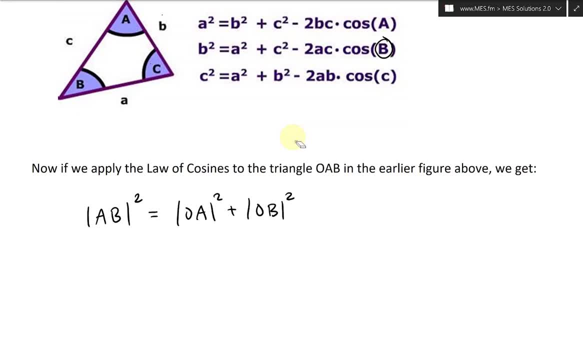 plus o, B squared. so this is the absolute values of the lengths there, those like line segments. then this is a, B and this is going to be two a, then this is going to be also o a, like that, and then this is going to be OB, like that, and then cosine theta, and again, we're just matching up this here. 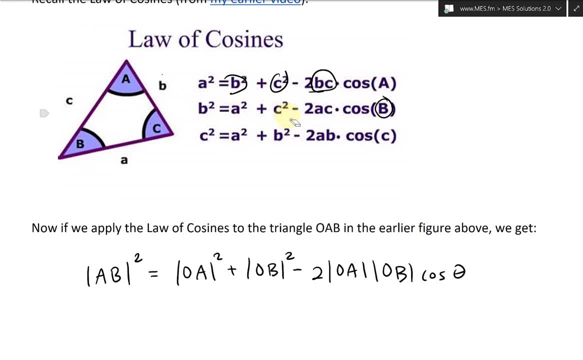 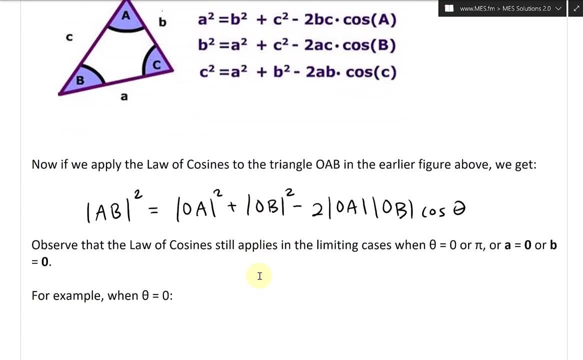 so if this is B squared, this is C squared, you're gonna have two BC and it's going to negative sign and then cosine that angle. all right, so that's what we have there, all right. so, now that we have this, and now, before we go over the proof, I'm just gonna look at these special cases here. uh, so, 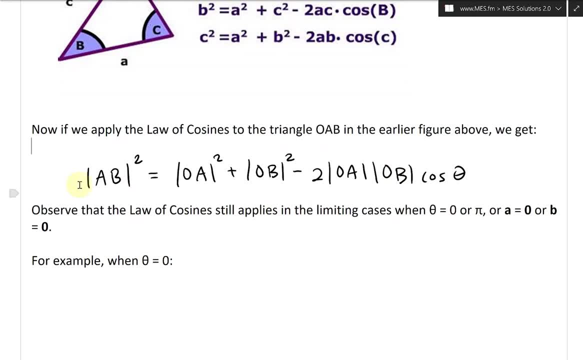 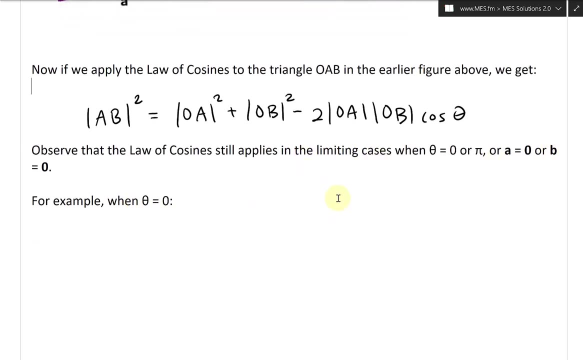 observe that the law of cosines that we wrote over here still applies in the limiting cases when theta equals zero or pi, when equals zero or pi, or a equals zero or B equals zero. and I'm not going to go through all them and they're pretty straightforward, because we're going to prove it. 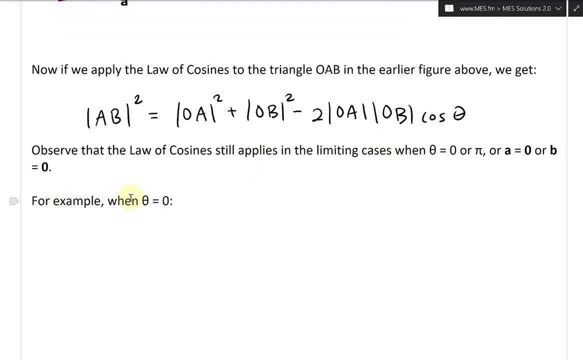 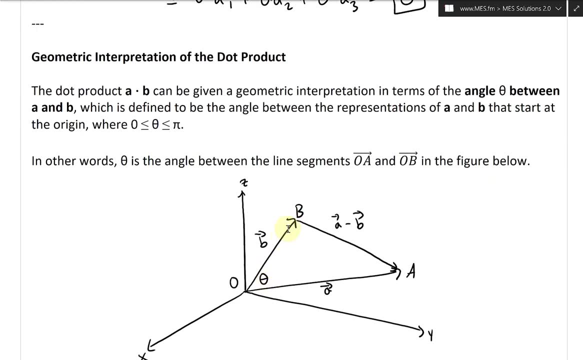 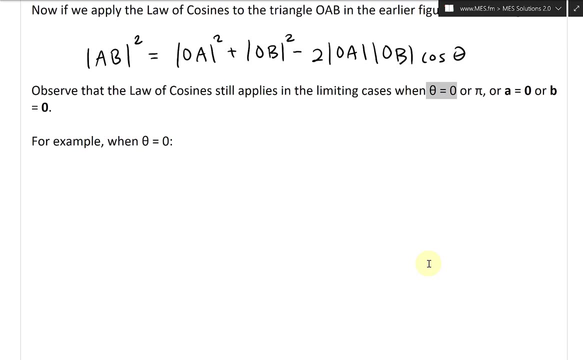 anyways, uh, in more rigidly this one just more graphically. for example: uh, we're just going to look at this case right here. so, when theta equals zero, so if you look at how this setup here, this vector B goes down, it's going to be parallel with a and in the same direction there. so, uh, for example, 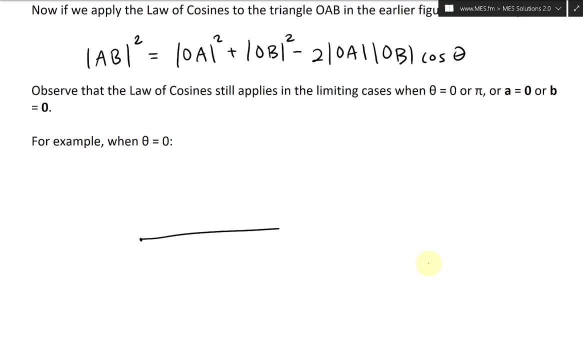 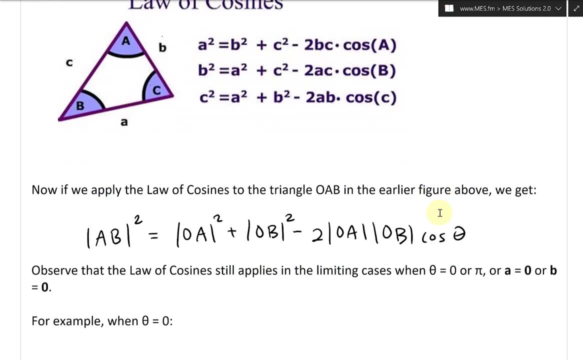 we're going to have. I'm going to write, I'm just going to write a straight line like this, because all we care about is the vector direction, so we just care about this one. here. we're going to make everything relative to this o, a there. so this is o, this is a. now the b is flattened, so the angles. 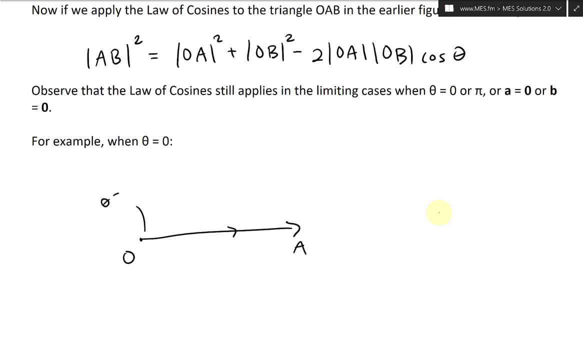 this angle zero, so, uh, theta is equal to zero. this distance right here, and this is the up to b and now. the distance between these two, these ones, is going to be our a, b, the absolute value there and this distance here. let's put this angle like that. and now this: 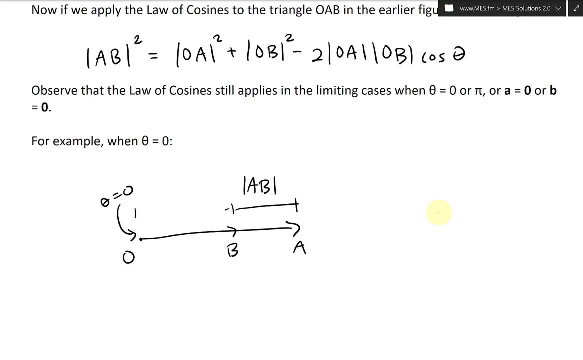 distance here to here. uh, this is ob, and now the full length is just o, a. so in other words, uh, if you want to find out, a b squared, a b squared, this equals two. well, we could have a put a bracket. this is going to be o, a minus ob. 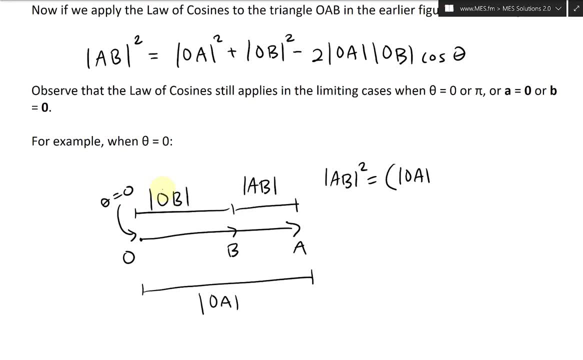 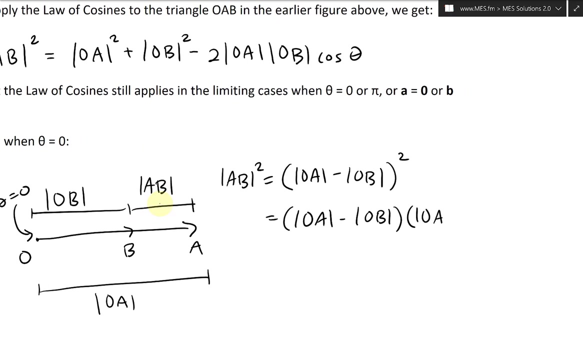 that's the value of o, a minus absolute value of ob, like that, then this is all squared. now, if you foil this out, uh, we'll just put this out for completeness: o, a, so value, ob, absolute value, and then uh, minus, uh, again ob, like that, and then foil it out: foil, foil, foil, foil. this equals two: uh, this is. 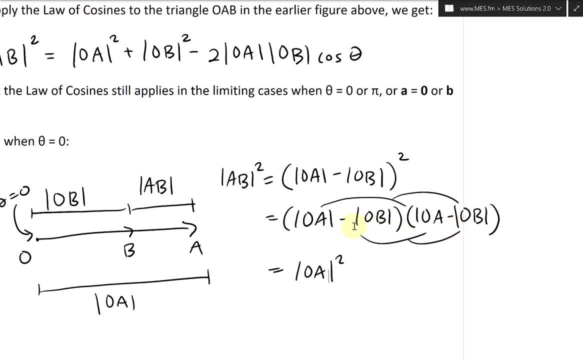 going to be o a squared and then, and then inside here is going to be negative two, because you're gonna, you're gonna have this one times by this, then this times this, you're gonna have o a times ob, and then we're gonna do the same thing: ob times, o o a. we're gonna have two. 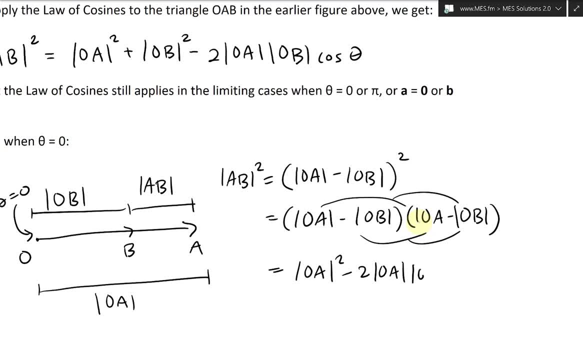 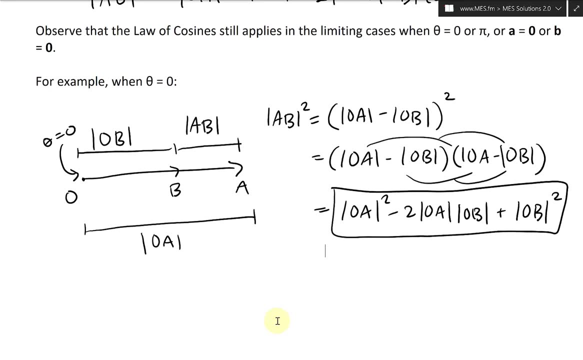 a times ob like that. and finally this one multiply with this negative cancel becomes plus ob squares again. this is basic foiling out, all right. so that's what we have there, that's what our a, a, b squared is. and now, if we look at this setup here: uh, this one here is uh, this is when. 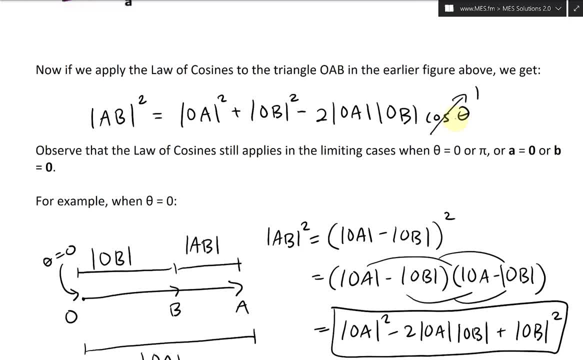 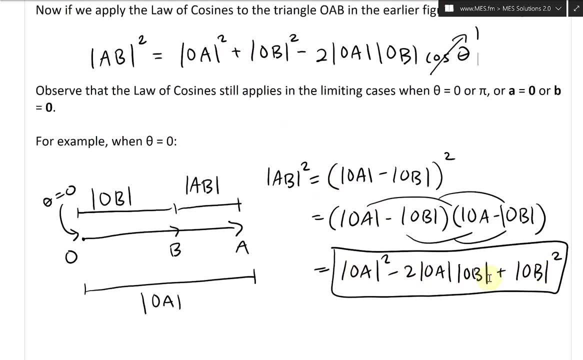 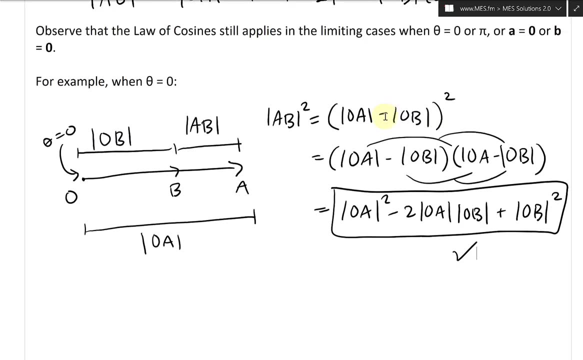 cosine is: uh is zero, this becomes one and in other words, this is matches. so you can see here that we see here oa squared, uh, then you have the ob squared, then you have a negative 2 o b there. so in other words, this is correct like that and i'll put: um, yeah, so in other words, i'll put it in. 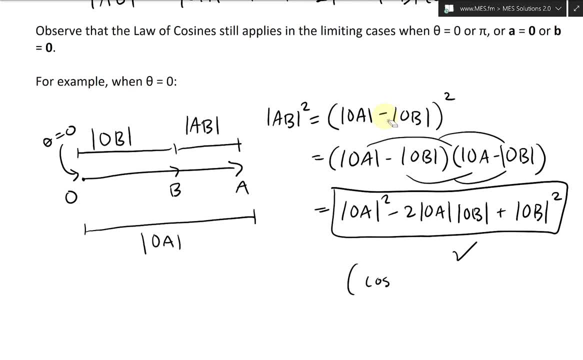 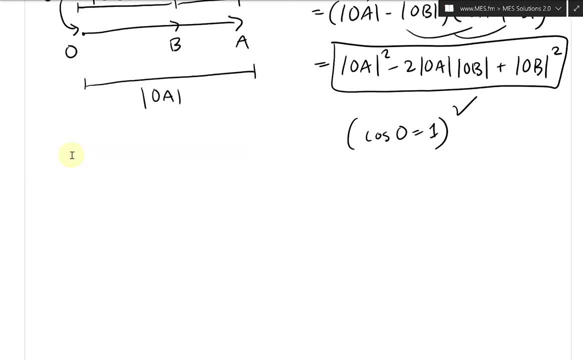 bracket cosine theta equals. i mean cosine zero equals to one. so anyways, we just proved this is correct. even when you have, theta is equal zero and it's just lines parallel. it's just very, very fascinating, all right, and uh, yeah, these, uh, these, this is i'm gonna go ahead and get all the way up to. 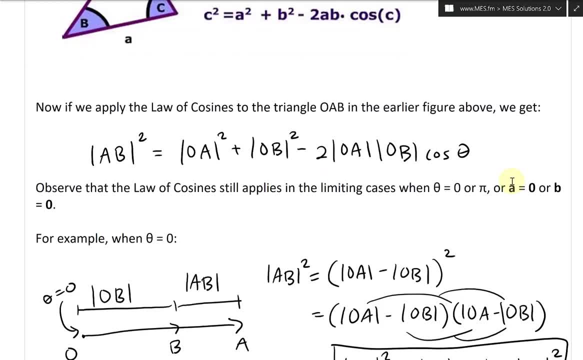 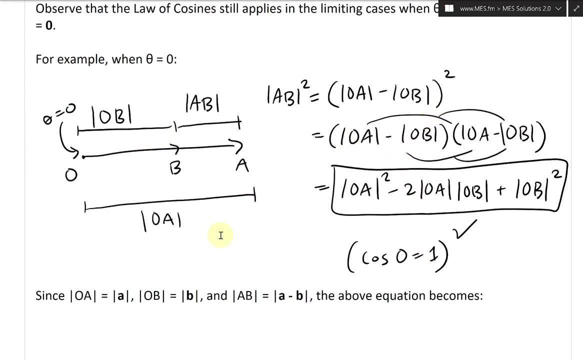 here so we can go ahead and get all these things and we'll go ahead and kind of define you know what other cases where theta equals pi or this, a equals zero, or b equals zero, vector, etc. those- uh, you could work on those yourself. it's pretty much. it could be very, very similar to this. 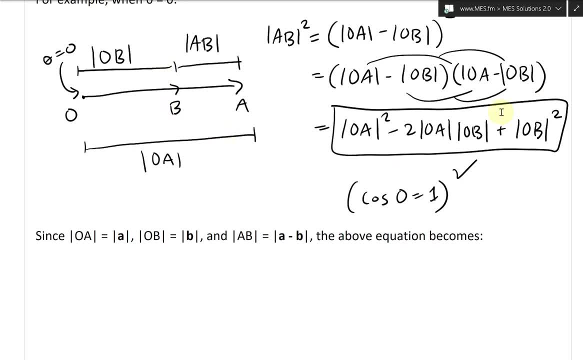 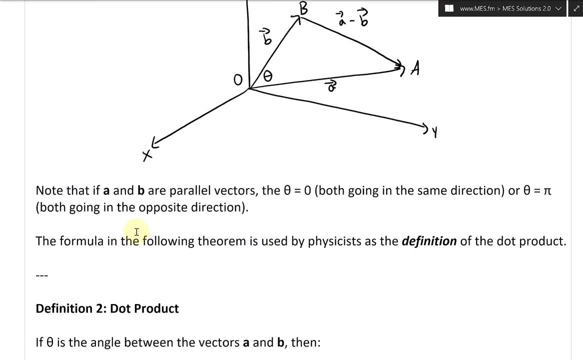 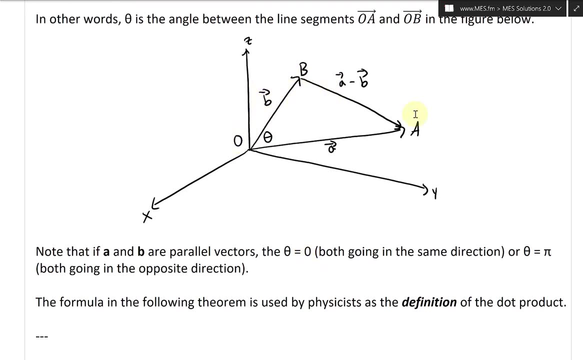 setup here. just do it algebraically. i mean uh, i mean graphically and then algebraically. so anyways, let's go back to here. so, since o, a equals to well, the length of this a vector, and ob is just this b vector, so we're going to write this all in vector form and then a b here is just going to be a minus. 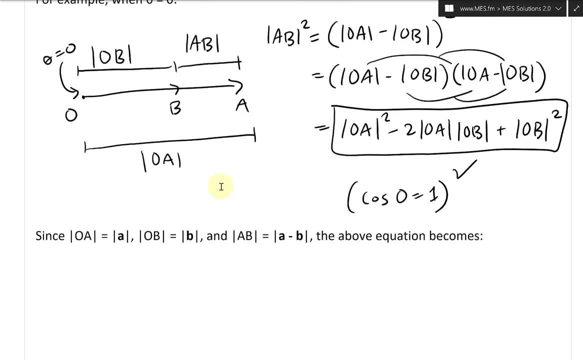 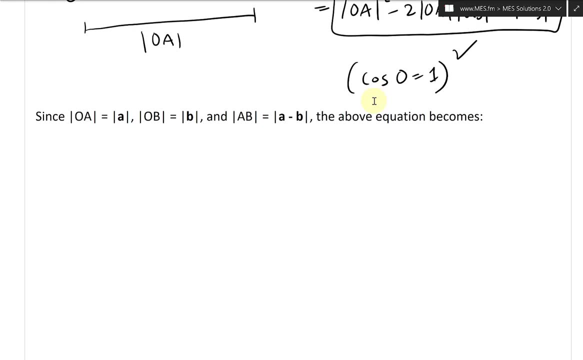 b, like that, yeah, or the length of the a minus b, yeah. so here, so: o, a, the absolute value of the line segment is equal to the length of the a vector, ob is the length of the b vector, and then a, b is the length of the a minus b vector. the above equation, this one here, becomes and this: 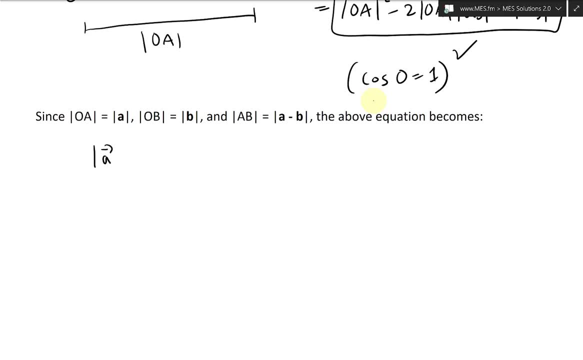 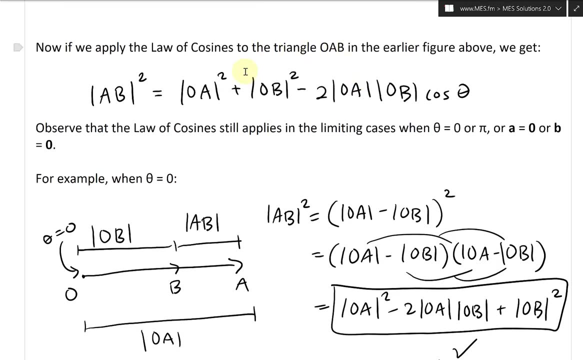 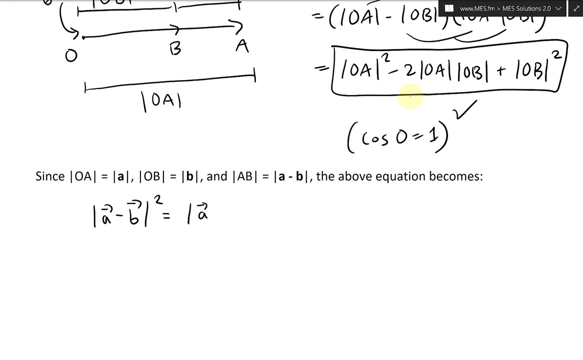 becomes, uh, a vector minus b. vector squared is equal to the o a. oh, a becomes a and then vector: this one's b squared and this one's going to be negative 2ab cosine theta. this can be a vector squared plus a, b vector squared minus 2 and this can be a vector length and not squared. 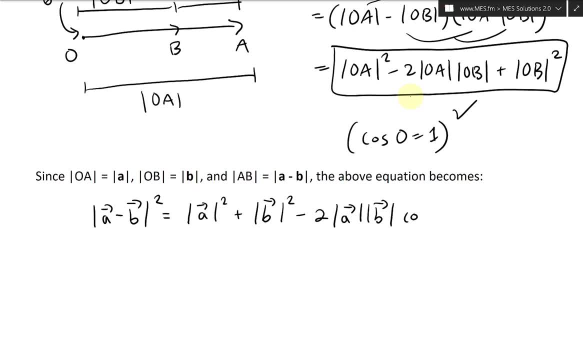 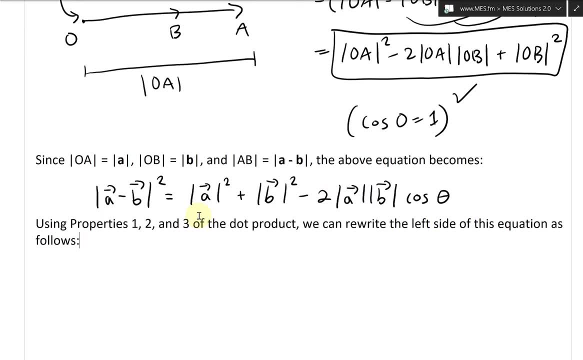 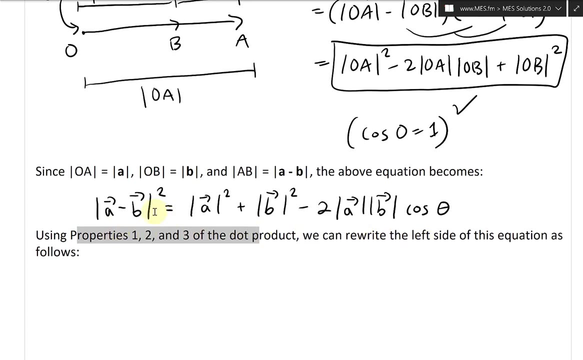 and then the next one's going to be b, like that length, and then cosine, theta, like that. all right, so now that we have this set up here and now, what we're going to do is, well, we're going to use properties one, two and three of the dot product or, using it, we can rewrite the left side, so this: 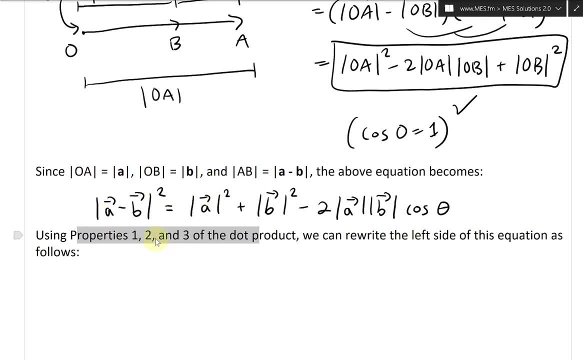 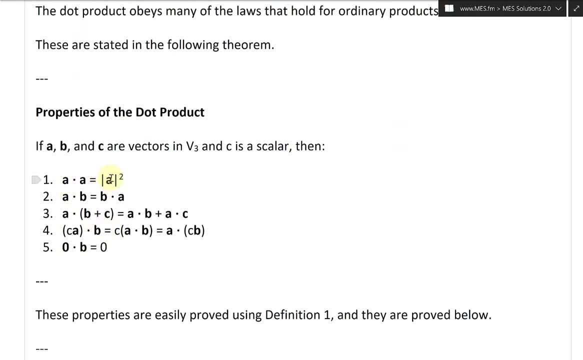 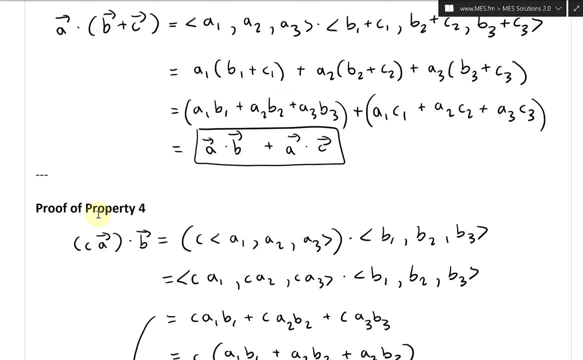 part right here of this equation as follows: or so let's just look, recolor properties. so we have property this one. here, a dot a is equal to well, this length a squared, then this one, the next one, you could rearrange the sides and then this is the foiling one. out is the property three. so let's. 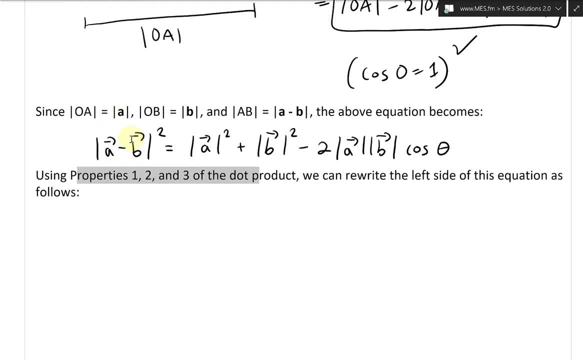 take a look at it here. we're going to try to rewrite this part right here, so let's try this: a vector minus b vector, uh squared, or the length of it all squared, and this is going to be equal to a minus b squared. so length, magnitude, whatever. 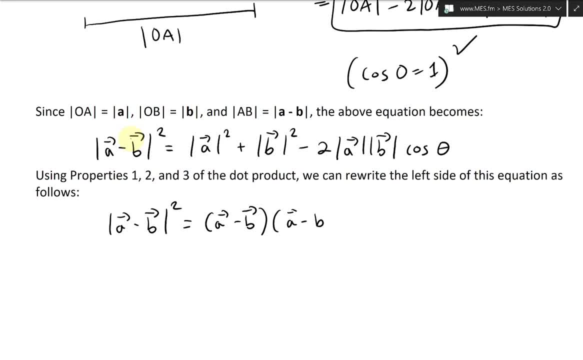 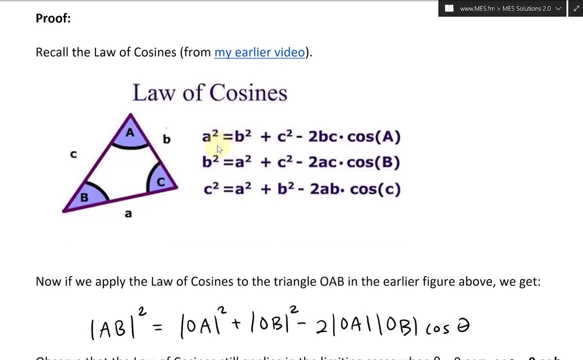 you want to call it distance and just write this as a minus b, like that. in other words, we're just going to be foiling this all out, but i'm going to go step by step, just so we match the properties as listed here and just do it this way. 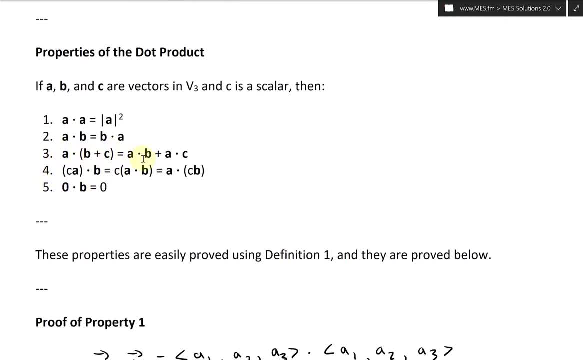 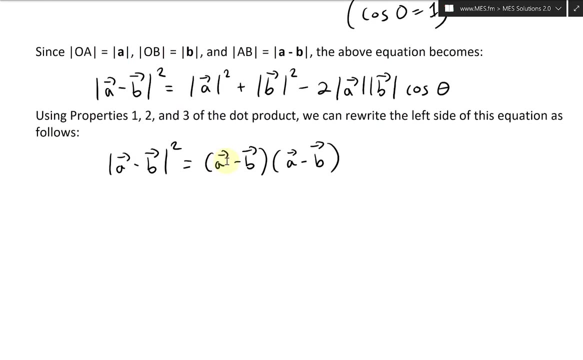 slowly and methodically. so we're going to do, yeah, this property here, and then later we're going to do the reverse one, and then also this one right here later. let's just do this slowly, let's do. i grasp it. so what i'll do is: yeah, so multiply this: uh, a minus b times by a and or multiple. 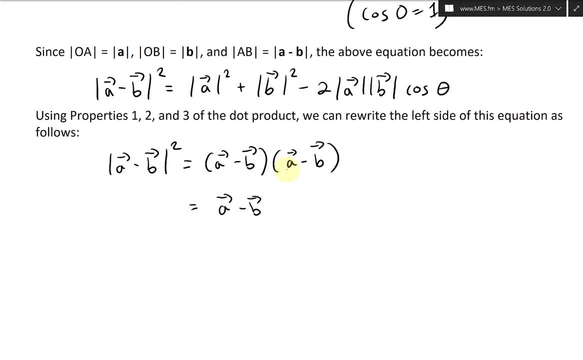 dot product, good. so a minus b dot, a dot like that, and then minus, and now this times the by the b one thus becomes a minus b like that, a vector, dot, b vector. and then multiply this: now inside here, inside here, etc. this inside here and this side, again, again. this is just basic foiling. i just wanted to do that step by step. 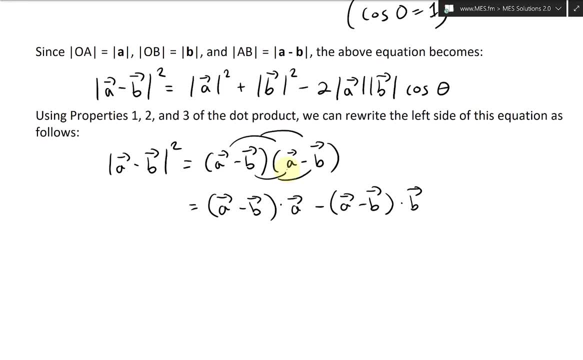 but later you could just do foiling this times this, this times this, exactly like real numbers. so you just do that and so on, and then we're going to do this here, and then we're going to do this and we're going to get: uh is a squared, i mean, uh, this is a yeah, a times this one here, a dot a. 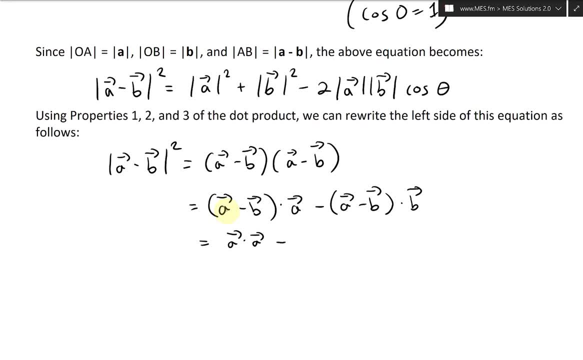 and then we're going to have minus uh a, dot b, yeah, minus a, yeah. so we're going to have it here. i'll just write this as uh, just as it is, and we'll do the property uh two later: a b, dot a, and the next one here, this one, multiply inside, multiply inside, and so on. so what we get is: 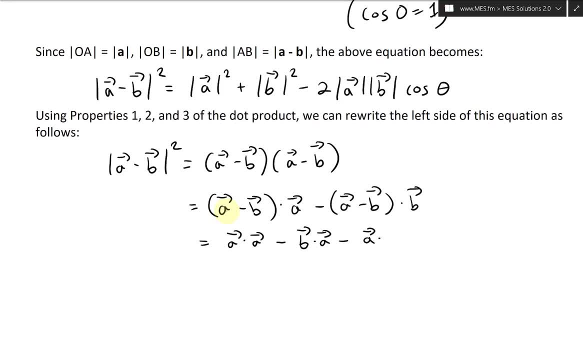 is minus a dot, b, and then this minus becomes a positive plus: b, dot, b, dot. i mean uh, b, dot, uh, b. all right, and again, this is exactly as we expected. so this is going to be now. this is property one. this is equal to the length squared. the next one: here we can just uh add: yeah, this one, we. 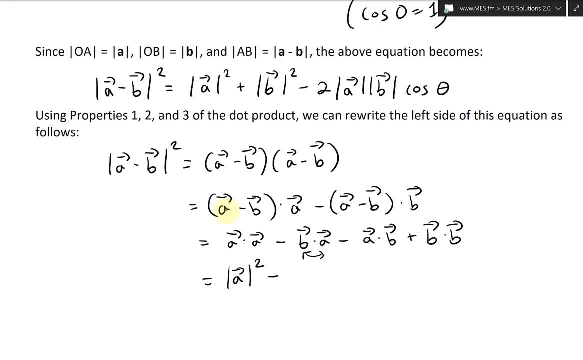 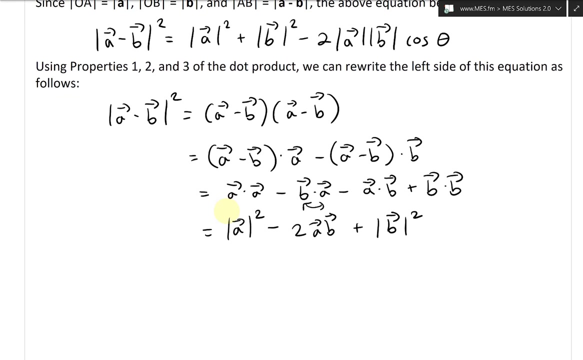 just rearrange, this becomes a, b using property uh two, and then add these up, this becomes two, a, c- i mean a, b like that, a b. and the next one here is plus this one right here, using the property one, uh b, length of the b or magnitude and square like that. that is fascinating stuff here we can. 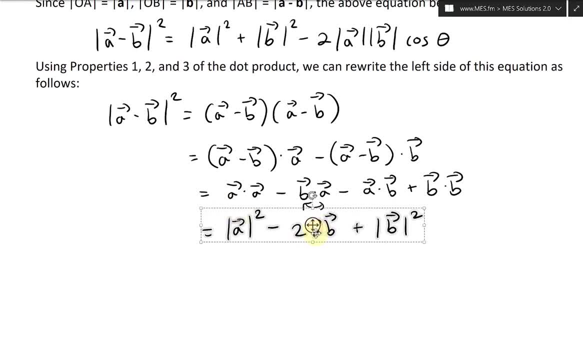 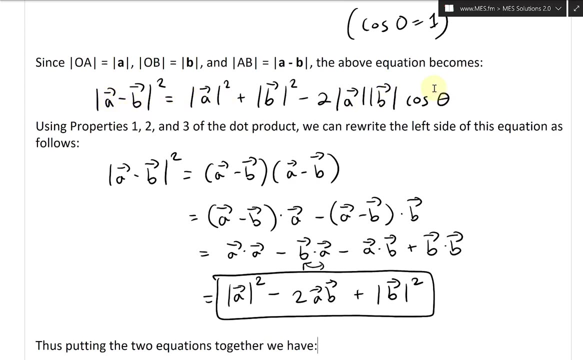 box this in, we'll box this all in, like that, like this, all right, so now thus uh, putting the two equations together. we have, so we have. this is the left side, and now we have this cosine law set up there to put them together. we have, or i'll just uh put it out for completeness: 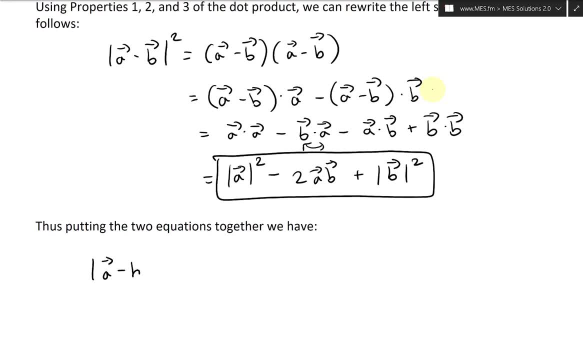 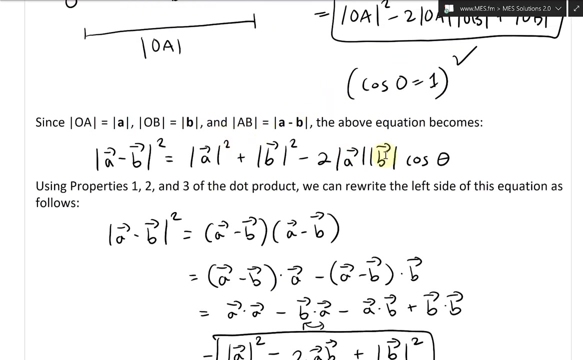 first. so a, uh, yeah, so a minus b vectors squared equals to using the cosine law setup: a vector, uh, the magnitude, uh squared plus b, squared minus two: a, b, magnitude, cosine theta. so that's these, uh, this setup right here, and now we have this one right here. so we have this and we have this, and and, uh, equate them. let's put those together and 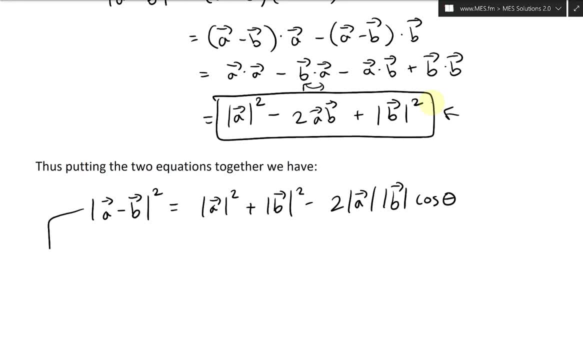 i'll do that right here. so this, uh equals two and uh, let's write this all down here. so a squared minus 2, a b squared plus b squared like that. and now this equals to this. and i'm going to do here, i'm going to copy this, copy and paste. oops, i'm going to copy this, i'm going to paste. 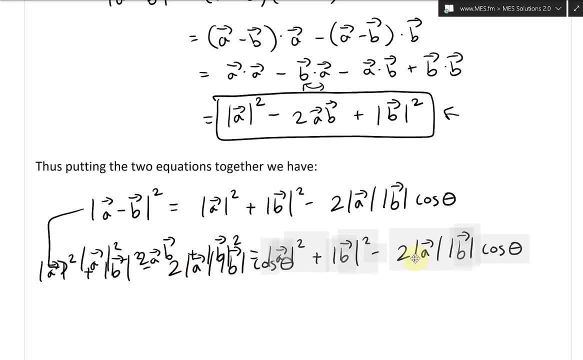 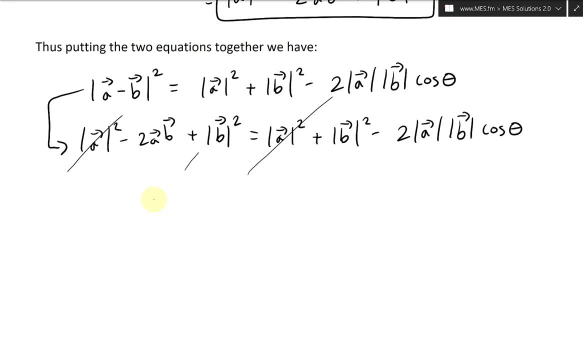 it here, save time and move this all the way across here. all right, so that equals to that. and now we can just do some simplification. while this cancels, this cancels, i'm going to just men's- this cancels, this cancels, and what we're left with is: well, this and this in other. 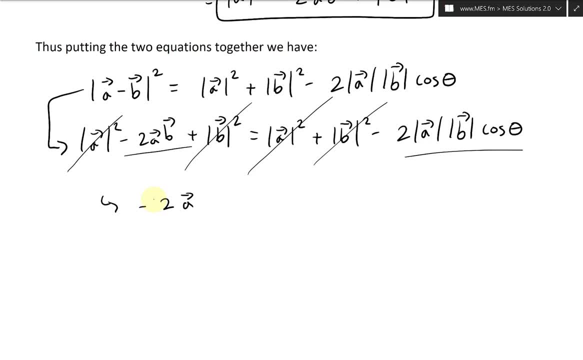 words, we get negative 2, a, the a and B. this is a dot number. there's a dot product there. so a dot B equals to negative 2, absolute value of a or the magnitude of vector a, magnitude vector B, cosine theta like that, all right. so as we have negative, those are negatives. 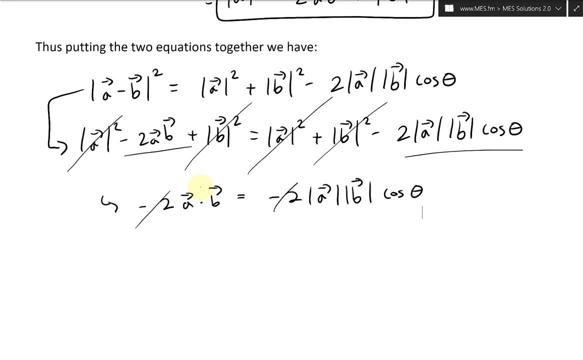 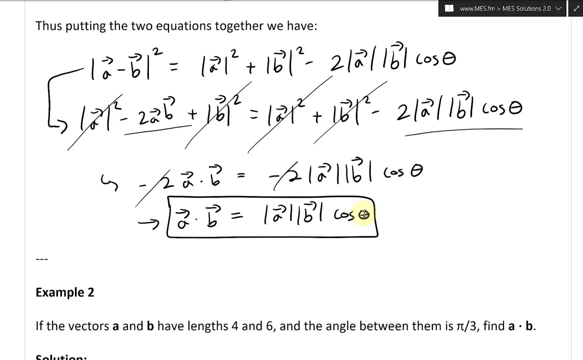 and the negatives cancel, of course. and what do you know? we have a dot B. dot equals to the magnitude a times by magnitude B, cosine theta. absolutely magic, yeah. so in other words, we prove that a dot product is equal to all this geometric view with a cosine angle there. 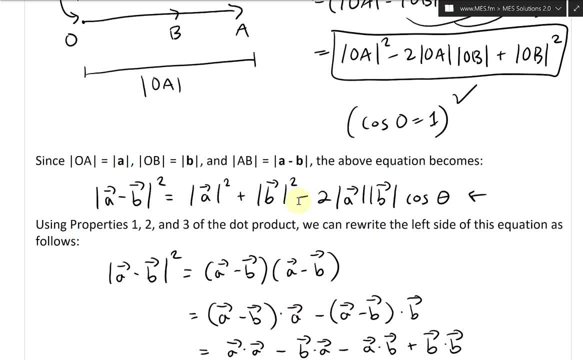 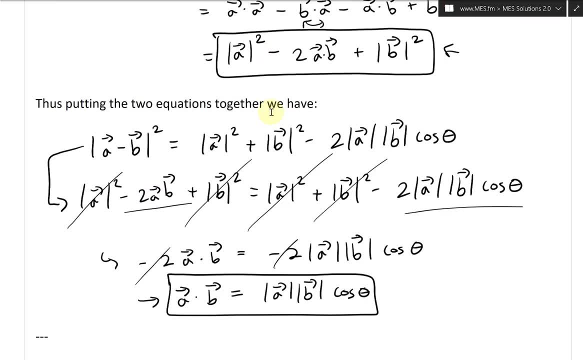 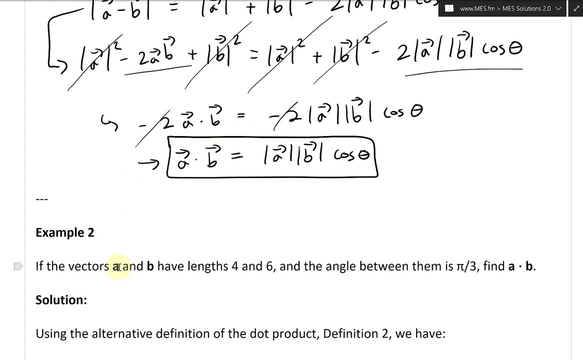 and is also equal to earlier definition. and yes, it's pretty fascinating. and we just started with the cosine law and then also this squaring using the dot, product properties and so on. so it's very, very fascinating. so now let's go take a look at example 2. so if the vectors a and B have lengths 4 and 6 and 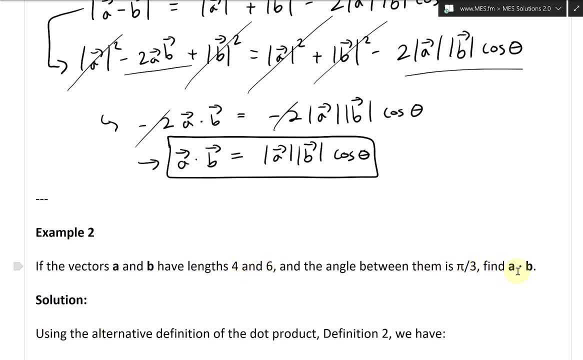 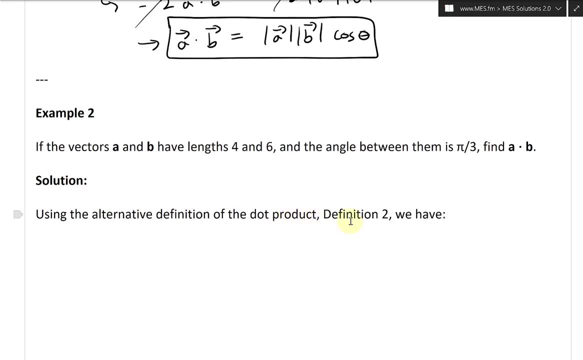 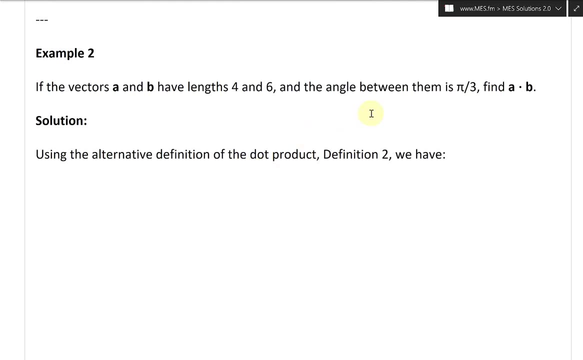 the angle between them is pi over 3. find a dot B. all right. so solution: using the alternative definition of the dot product, in other words definition to the physics definition we have. so again, we are asked to find a dot B. so we know that. well, a dot B is equal. 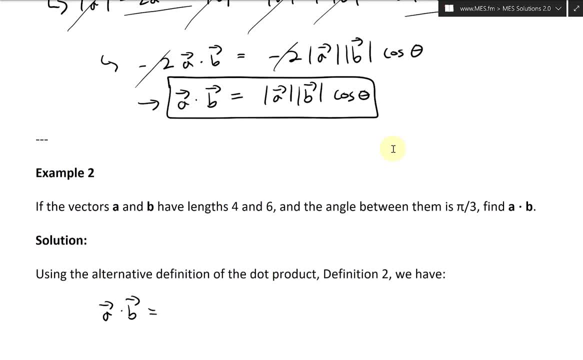 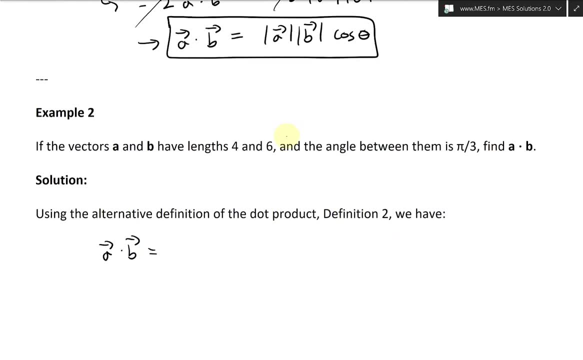 to, and all we're given is lengths and the angle. we don't have the actual components. what we could do, though, is what we know. it's this, so we know that is the definition, so we could go: a the length, a of the length, times by length b. 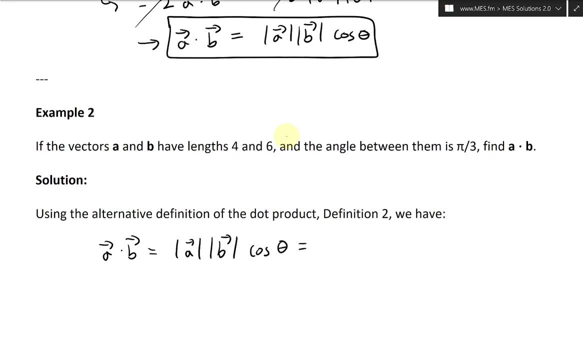 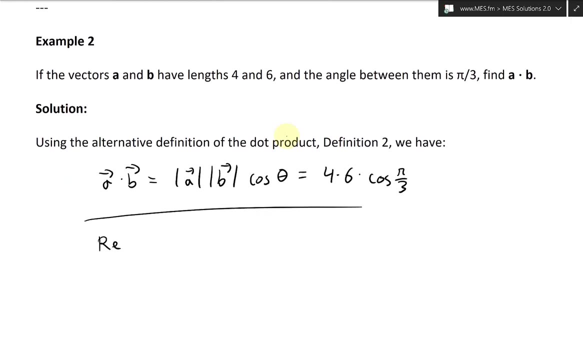 b, cosine theta. in other words, in this case we're going to have lengths 4 times, 6 times by cosine, pi over 3.. like that, another question is: well, what is pi over 3? and if we recall from my earlier videos, or just recall trig identities, uh and, and the way i do it for this, pi over 3, that's just. 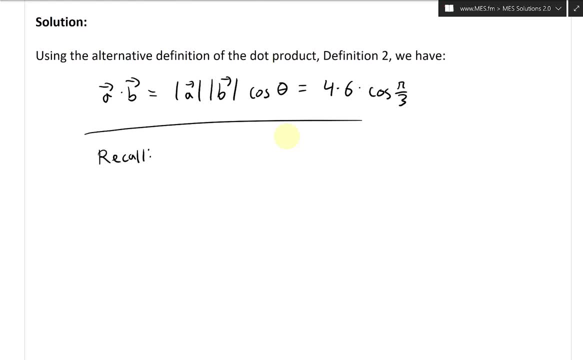 uh, 60 degrees, because number pi is 180 divided by 3, 60.. so what i'll do is i'm going to draw a equilateral triangle like this: all the sides are length two, two and this one. i'm going to split this in half so that this length is one one, so there's all two. so, in other words, all these angles. 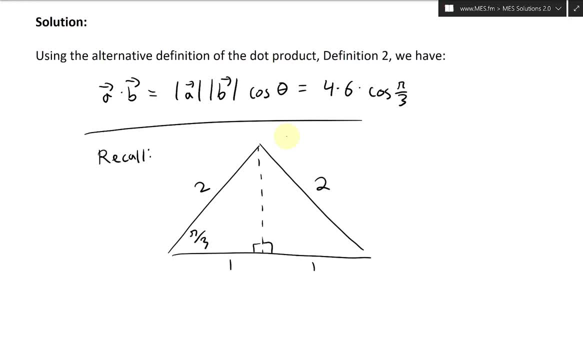 are going to be a good way of memorizing it. pi over three, let me pi over three. so all of them are, uh, 60 degrees, and then this one here is splitting in half, so it's gonna be pi over six, pi over six, and we're looking at cosine. 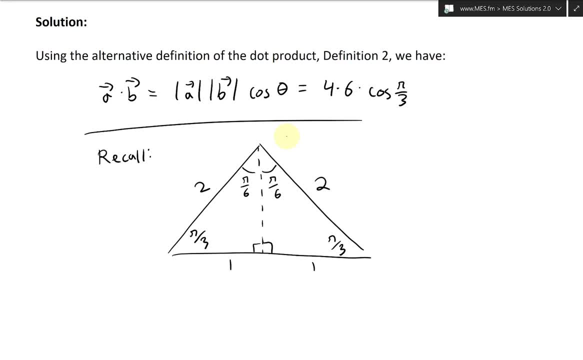 sine of pi over three. in other words, cosine is adjacent of our hypotenuse. uh, cosine, pi over three, is this equal to well, one over two, one over two like that. so in other words, this equals two. so that, over top just the end of this and this little recall thingy, let's put a line: uh equals to. 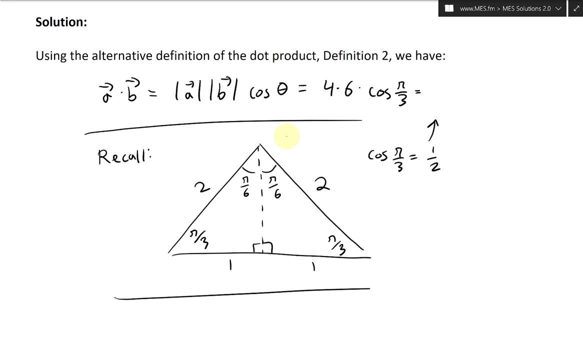 four times six is 24, or actually, before i even get to that, i will just do: um, yeah, actually, i'll just leave it that like that. so four times six is 24.. i'll just leave it that like that. so four times six is 24.. 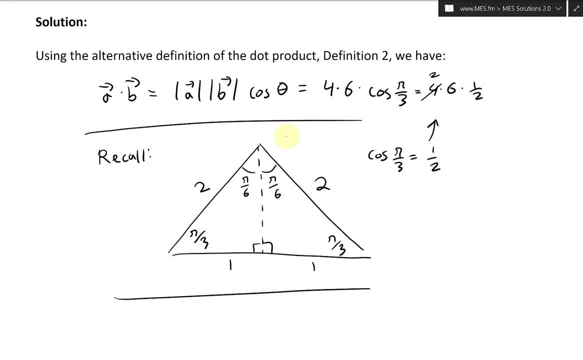 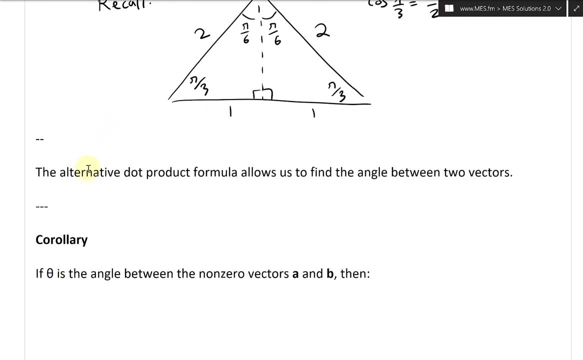 times six, times it by one half, this is two. this cancels and we're left with two times six is twelve, so in other words, the dot product is twelve, which is quite fascinating. all right, so now let's continue further. so, uh, the alternative dot product formula or definition do allows us to find the 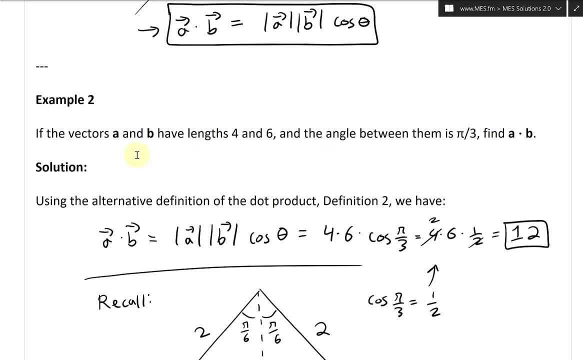 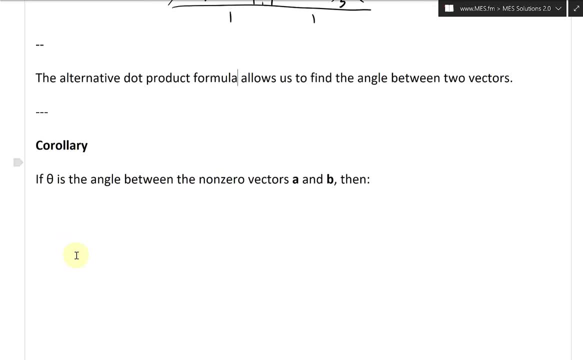 angle between two vectors. so if we have the length and uh and the dot product, we could just find the angle so corollarily or corollary, in other words, this is the theorem that follows from another one. so if theta is the angle between the non-zero vectors a and b, then and we could just rearrange. 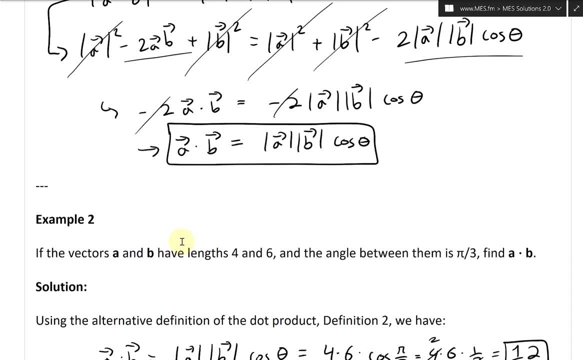 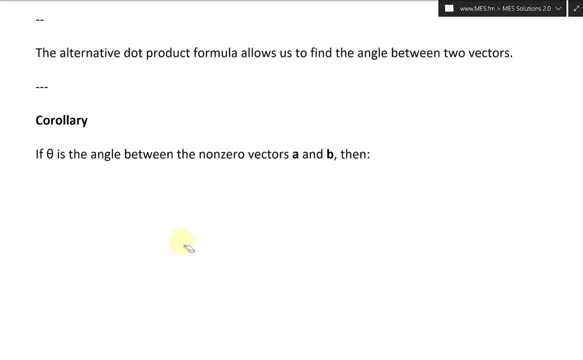 uh, this formula here: cosine, remove these, or just move these across here to the other side. so we're just left with the cosine. so what we get is, well, cosine theta. oh, let's write this neater: cosine theta is equal to a vector, dot b, vector over a vector. uh, the other length, a, b, like that: 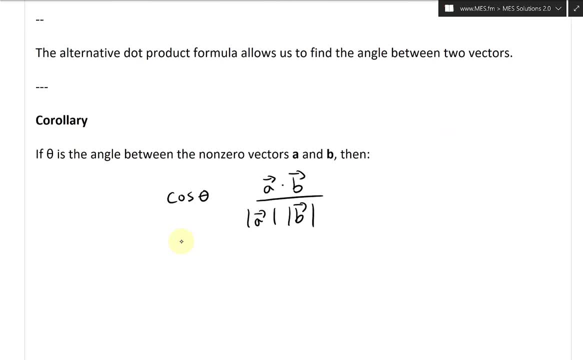 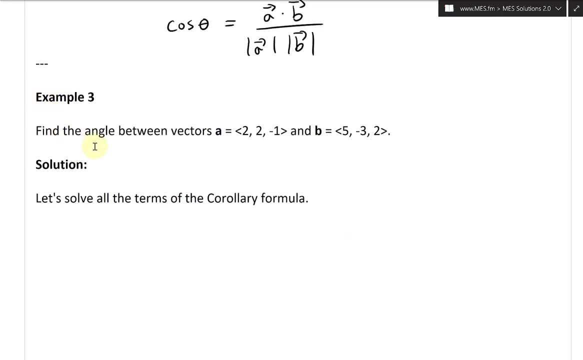 so just move those over to the other side. just very fascinating stuff there, all right. so now that we have this uh corollary, uh, let's go over example three. so example three states: find the angle between vectors uh or between the vectors uh a, which has components two, two and negative one, and b, which has components five, negative, three. 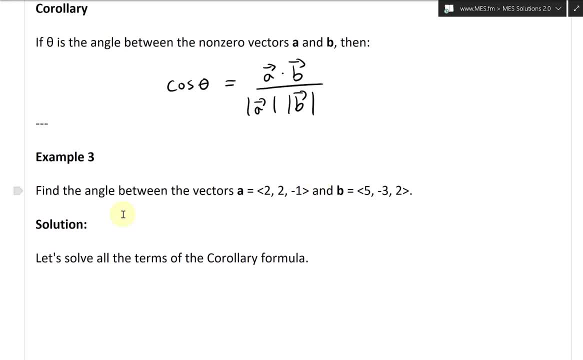 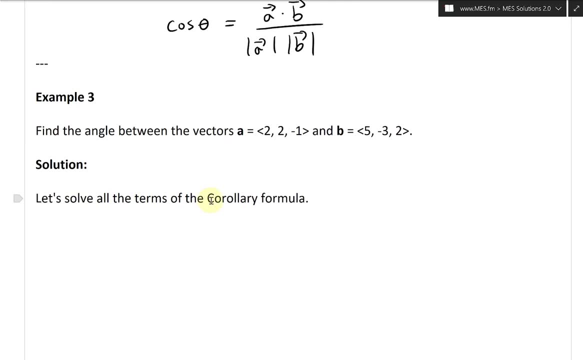 and two and let's take a look at the solution now. all right, so we're basically finding the angle between these two vectors. so, solution: let's solve all the terms of the corollary formula, because we're gonna need the angle there. so we have to do the dot product and then we do the 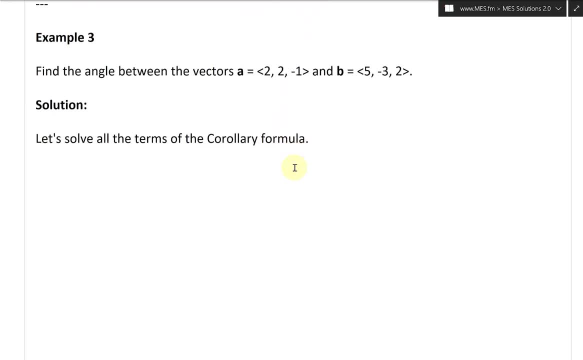 lengths there. so let's just do. uh, let's do the lengths first again. uh, the length is just 3d. uh, trick formula, or the distance formula, so let's get the lengths here. so, uh, the length of a is equal to all the positive square root of. and this is going to be well, um, this is i'll. 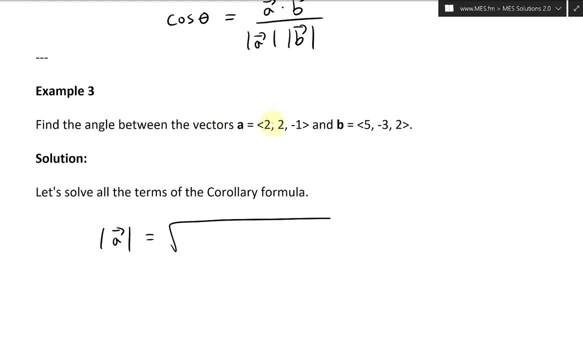 write this here and just skip it. yeah, this is going to be 2 squared. so square root of all this, plus 2 squared, all the components squared plus negative 1 squared, negative 1 squared, this equals 2 like this: so this equals 2. so 2 squared is going to be. 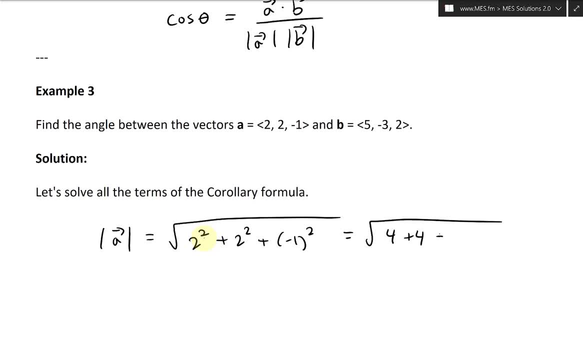 equals to 4 plus 4, and then this one's going to be plus 1.. so 8 plus 1 is 9.. so that's going to be 9. yeah, equals square root. 9 equals to 3.. all right, that's that one. and then the uh, the length of the b. 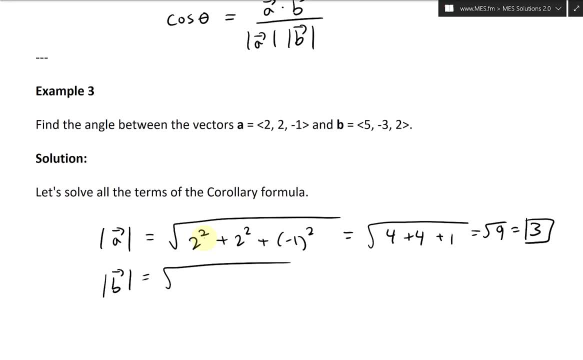 is equal to: like this: it's going to be 5 negative 3, 2, 5 squared, plus negative 3 squared plus 2 squared. this equals to 25 plus negative 3 squared. it's gonna be well, nine negatives cancel plus four like that. 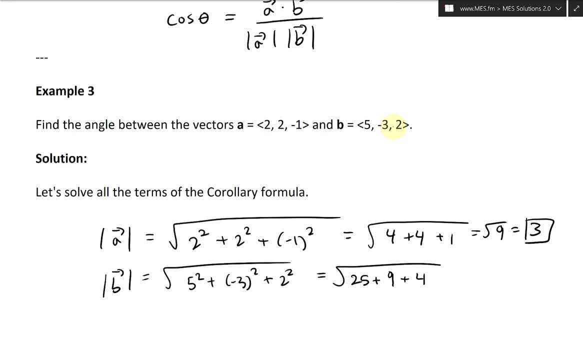 all right, so what? this is equal to well, 25 plus 4 is 29, or actually, let's go here: 25 plus ten is 35.. so minus one, so 34. then 34 plus 4 is equal to square root 38, and we're not gonna solve that. 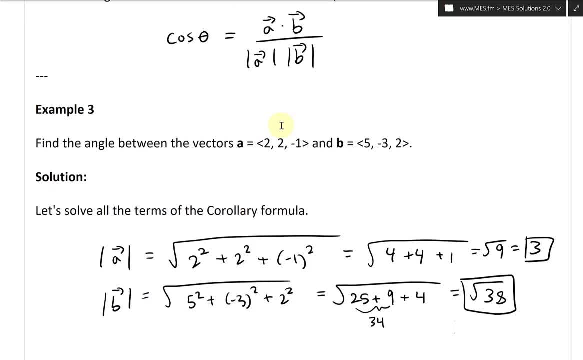 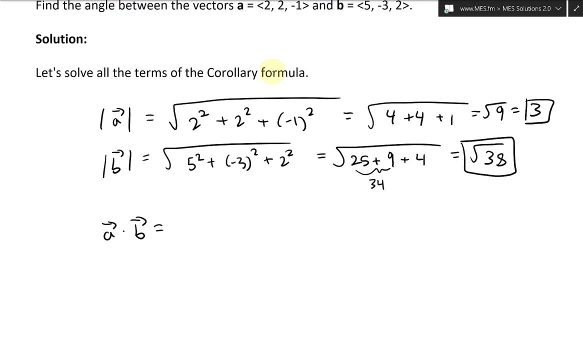 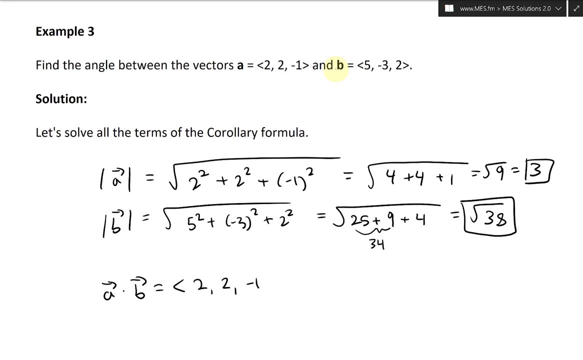 just leave it like that. all right, so we have the length. so now let's look at the dot product there: a dot b. so a dot b is equal to all the components. uh, so two times two- let's put this all for the plainest: two, two negative, one dot, five negative, three negative, uh, and then two leg up and then. 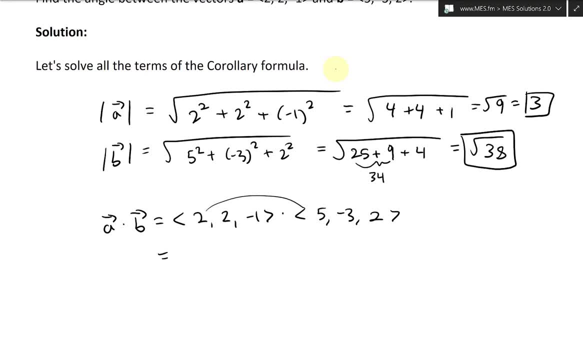 this equals two. well, this is going to be multiplied this. and then- uh, yeah, it's multiple components- this equals two and it's gonna be a real number, so we don't have the bracket. so, two times five plus two- uh, negative three, and then uh plus uh- negative one. 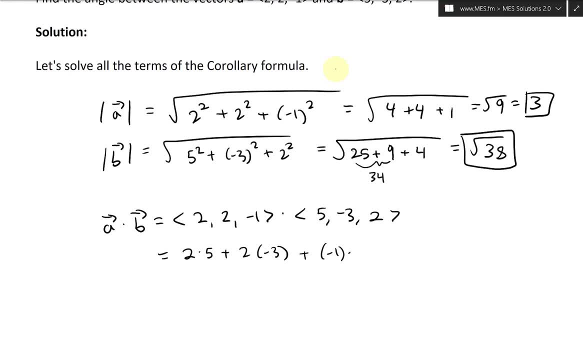 times by two, and this equals two. well, that's gonna be ten. two times five is ten, and then two, not times negative. three is six. negative six, then negative. one times two is negative two. this equals two. well, negative eight, and this becomes: uh, yeah, this is negative eight. so ten minus eight is equal to two, like that. 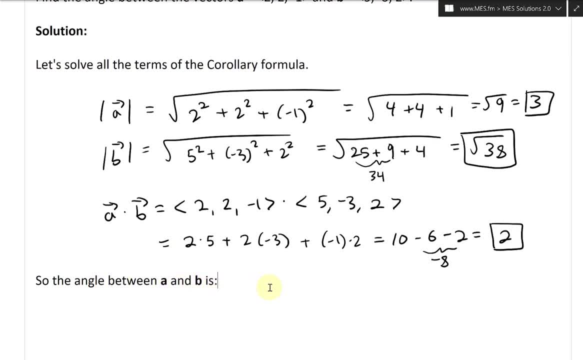 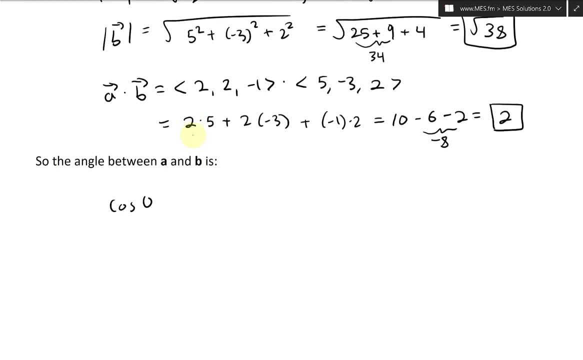 all right. so, uh, the angle between point a and dot product a, dot b, divided by length a, uh, length b, like that, this equals two. well, dot products two, and then divided by uh, three for a, and then um, square root, 13,, 3,, then square root, I mean 38,, like that. all right, so that's the cosine. 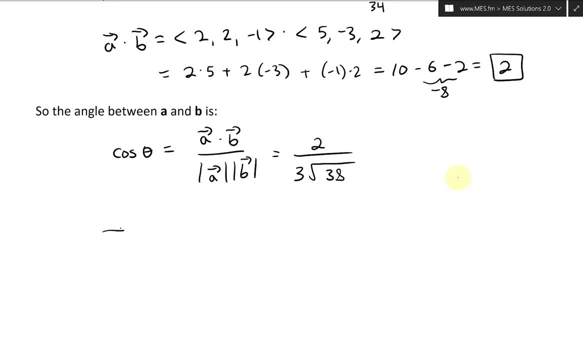 and we just take the inverse. so theta is equal to a tangent. I mean arc cosine or a cosine or cosine inverse, like that, and 2,, and then 3,, 38, like that. if you plug this into the calculator, what you end up getting is 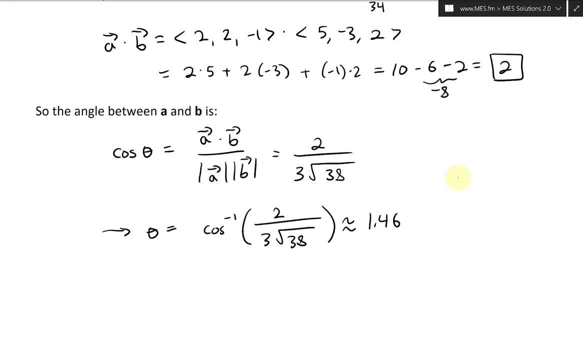 this is going to be roughly equal to 1.46 radians, radians and, or you know, or I'll box this just for completeness or and degrees. this is equal to: yeah, this is going to be, or it's going to be. 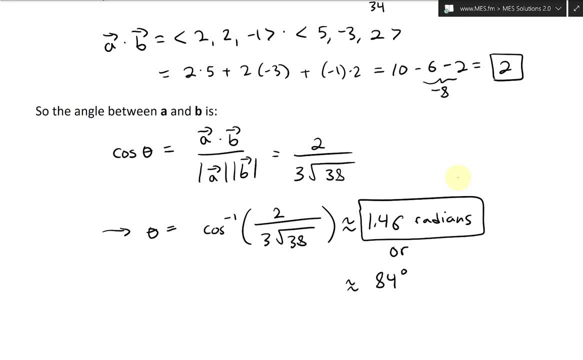 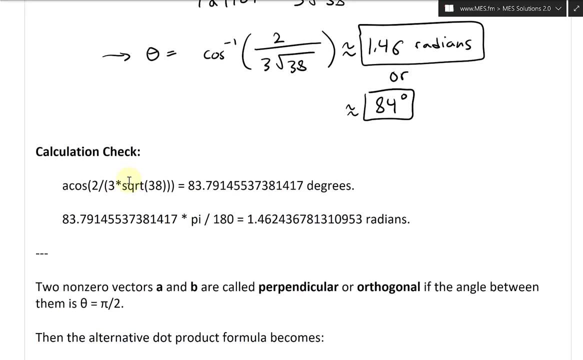 84 degrees or 84 degrees. and now let's do a quick calculation check. so my OneNote, the OneNote program that I'm using, has a built-in calculator. so if you write a cosine, yes, a cos, and then bracket 2 divided by 3, then you can write squared or sqrt for square. 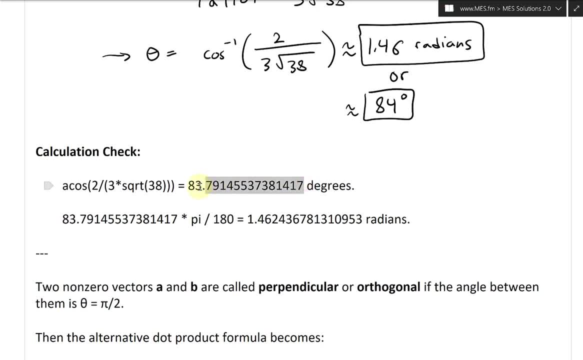 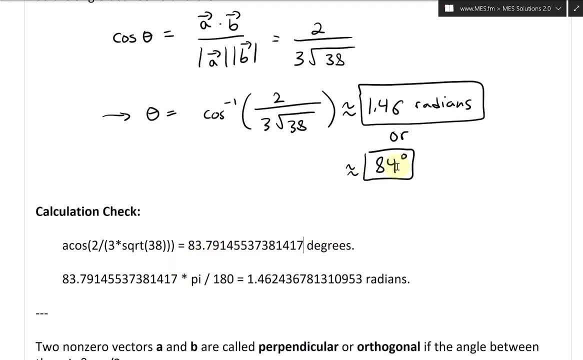 root 38 for the corresponding correct brackets. delete this. the thing is, default is in in degrees like that, and you get 83.79, et cetera, round it up to 84, and then, if you plug. 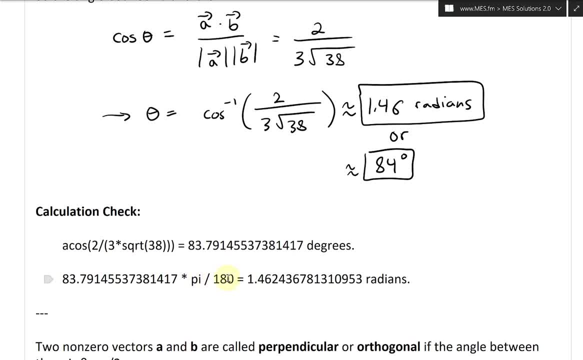 that inside here and times it by pi divided by 180, because pi radians for one for every 180 degrees, and then you get erase and press space and you get 1.462, et cetera. this fascinating 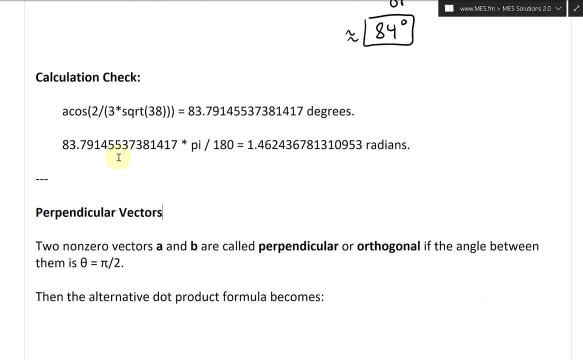 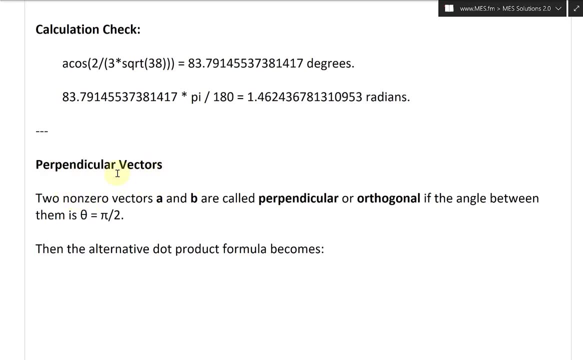 stuff all right. so now let's continue further and now look at perpendicular vectors. so, and yeah, here this heading, I'll put this in the topics to coverage that it is right now. so anyways, two non-zero vectors, a and b, are perpendicular or orthogonal, again basically the 90 degrees. 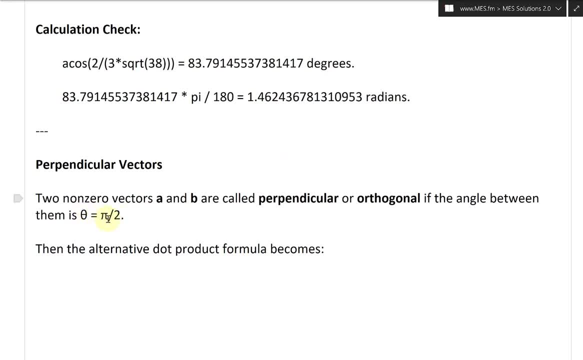 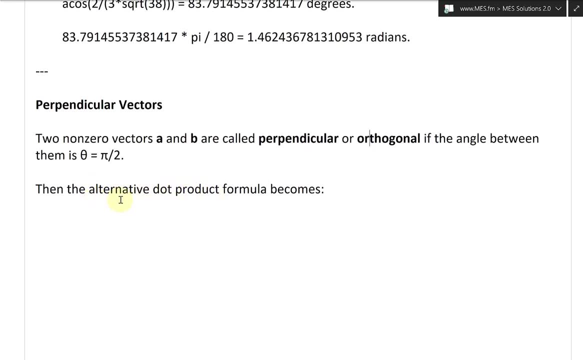 set up like that: if the angle between them is theta equals to pi over 2 radians or 90 degrees, then the alternative dot product formula becomes or definition of 2, this just becomes a dot b for the angles. for the angle, theta is equal to pi over 2,. 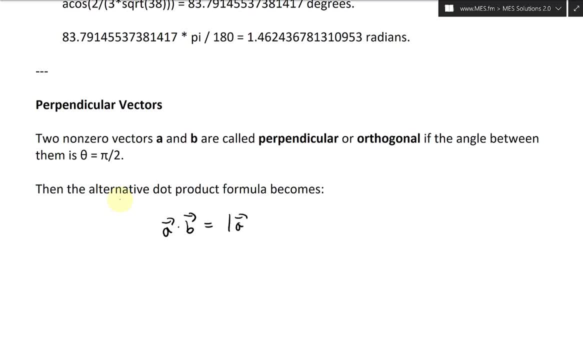 this is equal to 2, like this, a like that: yes, this becomes. and then the cosine, cosine pi over 2,, in other words, this becomes: well, this is 0, actually. so this equals to 0, and we'll illustrate this later. this is cosine pi over 2, and I'll graph: 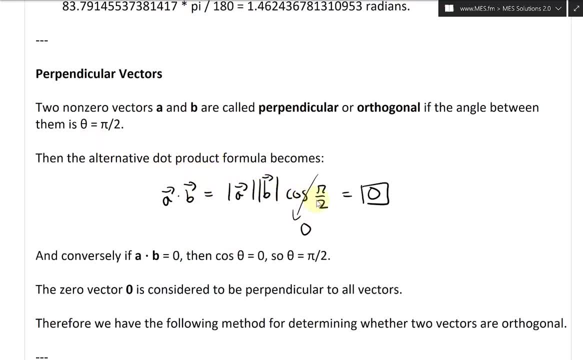 this out later for cosine, just to recall it later. but yeah, so cosine, pi over 2 is 0, so this whole thing vanishes. and that's when it's orthogonal or perpendicular, when the non-zero vectors a and b are perpendicular. 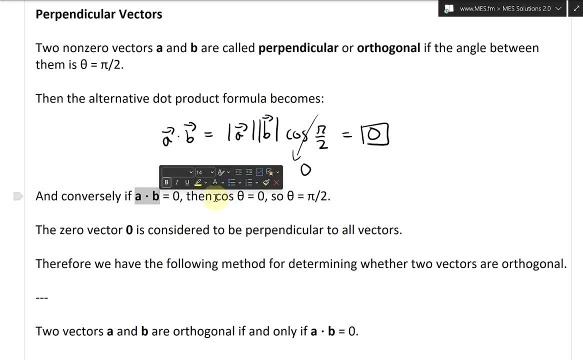 and conversely, if the dot product a, dot b is equal to 0,, then cosine theta is also going to equal to 0, and hence cosine. yeah, so this cosine right here, so this dot product is 0,. 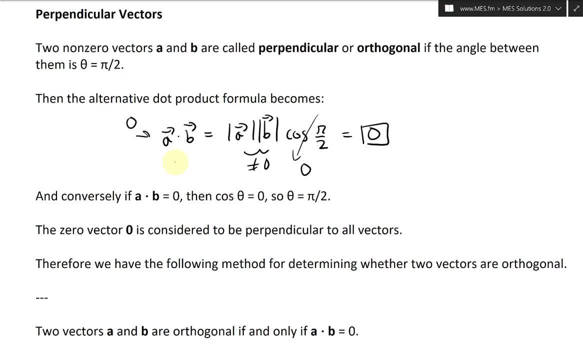 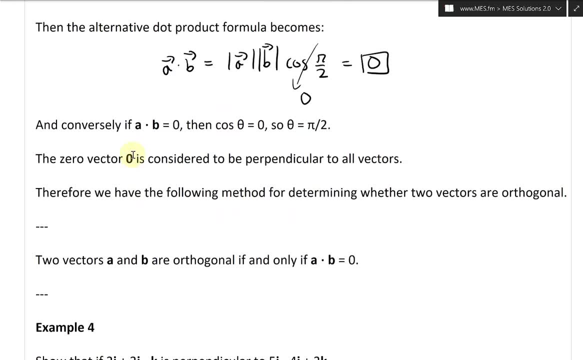 then this one has to be 0 too, if these ones are non-zero. so then you have, the cosines can be 0, so then the angles can be: theta is equal to pi over 2, and yeah, so the zero vector. 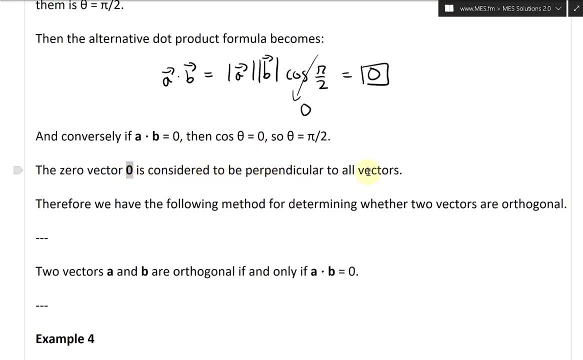 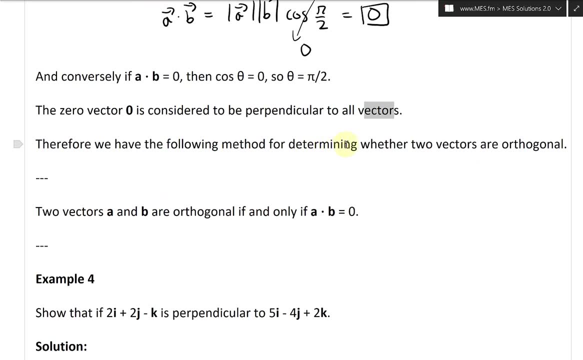 this right here: zero vector is considered to be perpendicular to all vectors. so, yes, very interesting. so zero vector is always perpendicular, just by definition. therefore, we have the following method for determining whether two vectors are orthogonal. two vectors, a and b, are orthogonal or perpendicular if, and only if, the dot product. 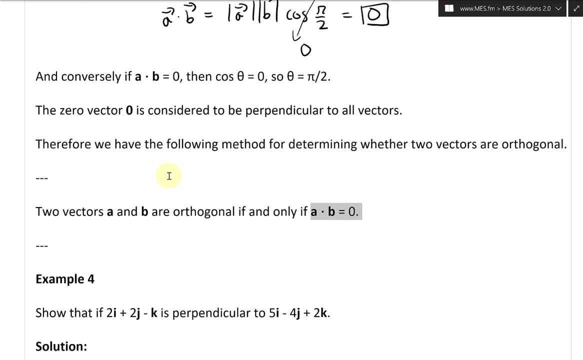 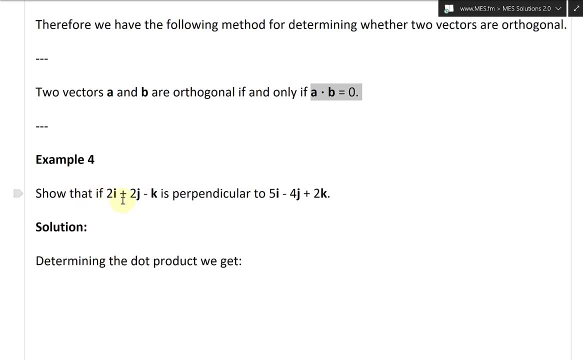 is equal to 0, absolutely, yeah, fascinating stuff there. now let's take a look at example 4, and this one states: show that if 2i, the standard basis vector, 2i, vector plus 2j minus k, is perpendicular to 5i minus 4j plus 2k, 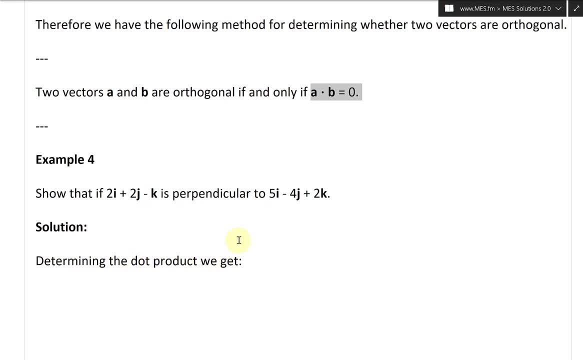 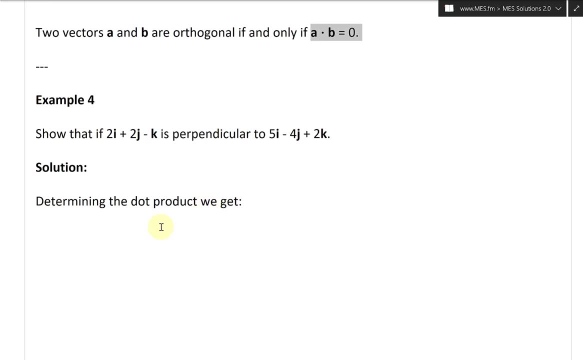 so show that this is perpendicular. so solution: determining the dot product. so all we got to do is determine dot product. if it's 0, then it's perpendicular. all right, let's take a look at this dot product. all right, so we get. I'm just going to write this. 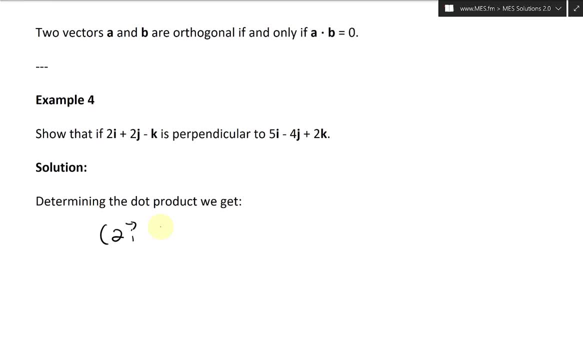 like this: 2, and put as regular bracket because the vectors are already inside: plus 2i, plus 2j minus k vector, at least on top, and then dot 5i vector minus 4j vector plus 2k vector. 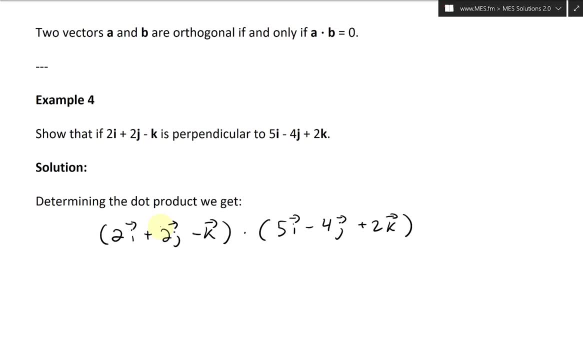 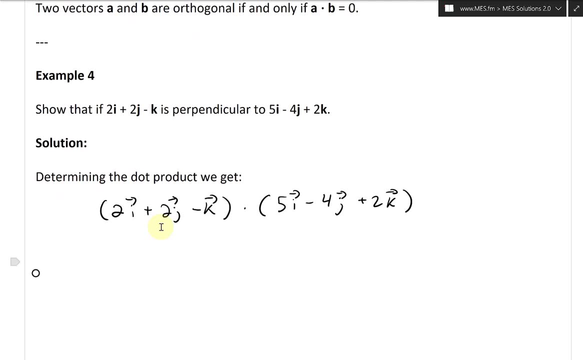 like this: and then, yeah, the dot product, all the component parts here. I'm going to write this, actually, I'm going to write this: move it to the left, okay, so move it over there. this equals 2, and I'm going to put it over here. 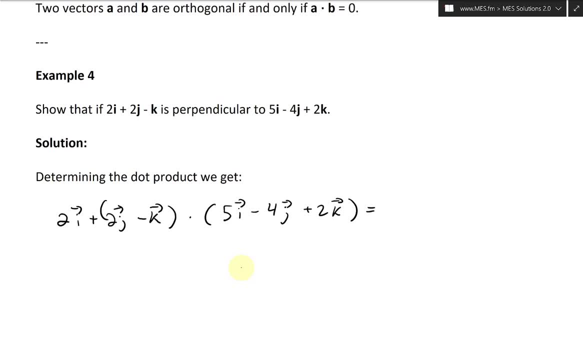 let's put it here. where should we put it? right here? see, all right, and then this is 2 times 5, yeah, this is going to be 2 times 5, plus, yeah, 2 times negative 4,. 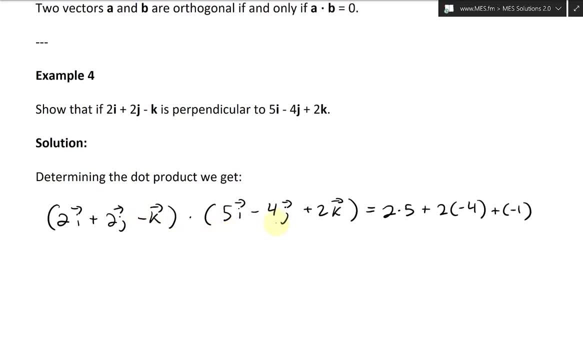 and then plus negative 1, and then 2,, like that this equals to 10, minus 8, minus 2, and yeah, that's just 10,. so this equals to 0,. yeah, so it is orthogonal or perpendicular, or a better box, perfect. 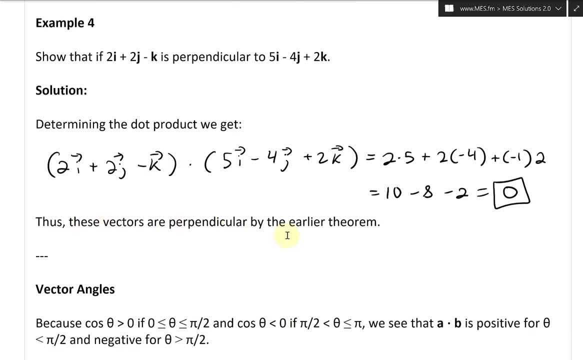 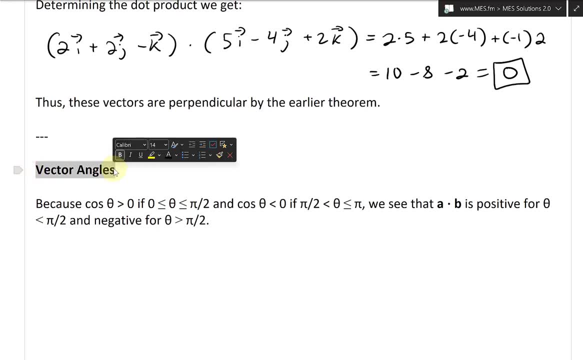 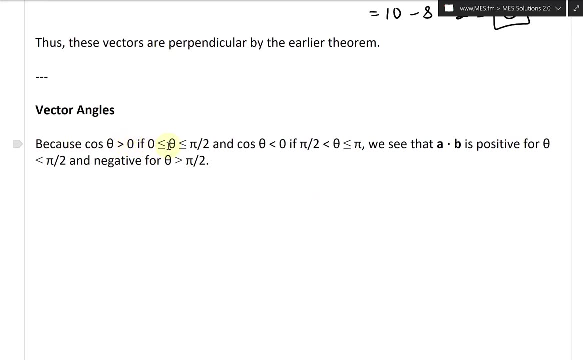 all right, yeah, so finish off example 4, so thus these vectors are perpendicular by the earlier theorem. that's fascinating. and now here's another section. I just added the heading on this one here, vector angle. so because cosine theta is greater than 0, if, if the angle theta is between 0 and pi, 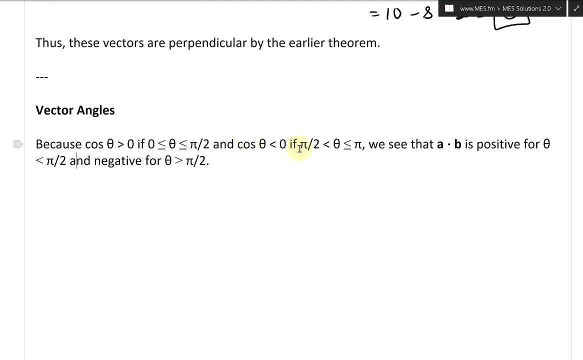 over 2, and cosine theta is less than 0,. if, if theta is is less than pi over 2, and less than equal to pi, we see that a dot b is positive is positive for theta is less than pi over 2,. 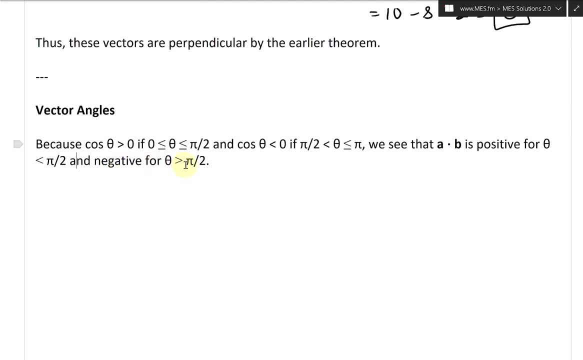 and negative for theta is greater than pi over 2, and here's a graph it all the components of it. so let's say: we have this angle, theta is the x-axis. now we have the cosine, theta is the y-axis also. I'll just put a y like that, all right. 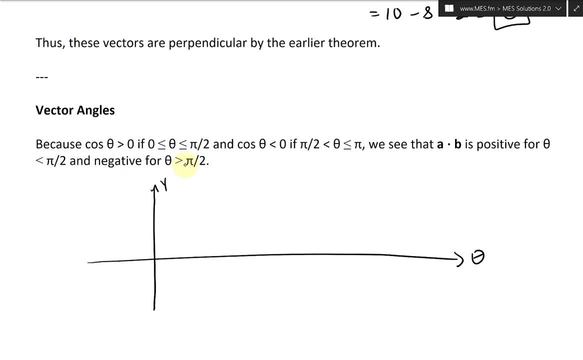 so now we have- I'll do this a bit better, all right, so that is pretty decent, actually. all right, that's pretty good. all right here, I just fixed it up. so basically, here's the cosine theta. 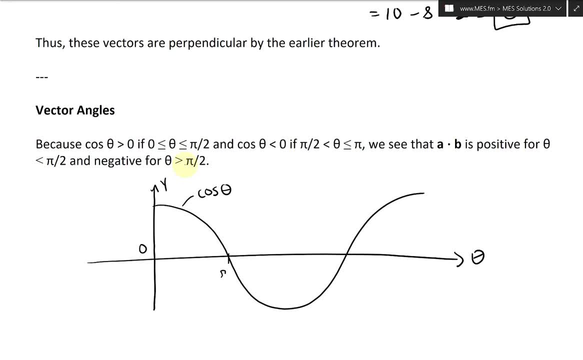 graph like this, and this is at pi over 2, just recall it. and here's at pi like that, and notice here, because we're only considering from 0 to pi, from 0 to 180 degrees. so then this is positive and then I'll put this on top. 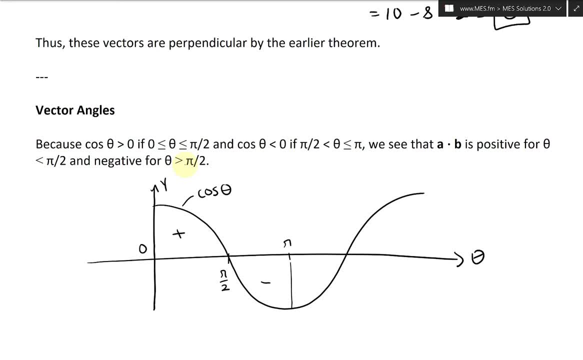 pi and then over here. this is negative. so because cosine theta is greater than 0, if if theta is between here and cosine theta is less than 0,, if it's between here, we see that a dot b is positive. 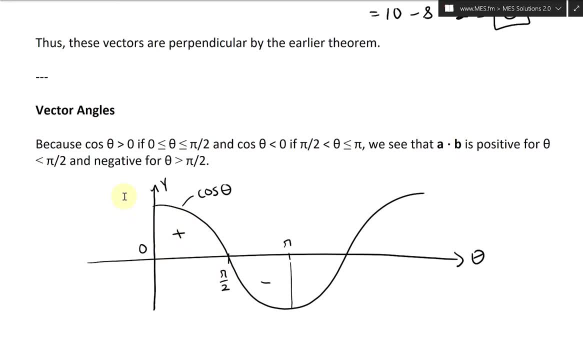 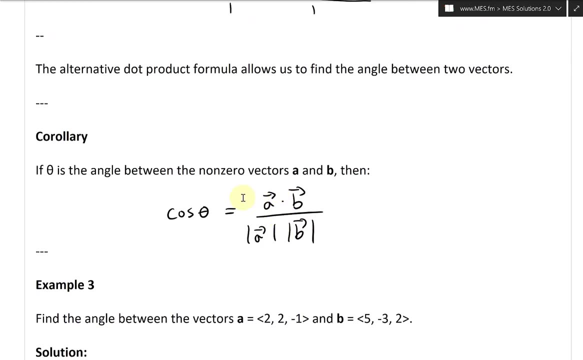 for angles less than pi over 2, and negative for theta is greater than 2,. so the cosine theta is going to be, or the dot particle will be positive or negative, because it is dependent on the cosine of the theta of the angle. so there's dot product and it's dependent on it. 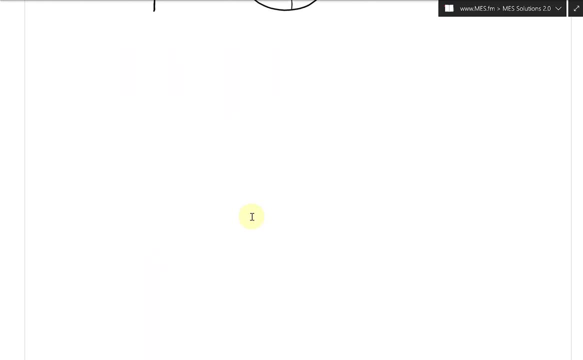 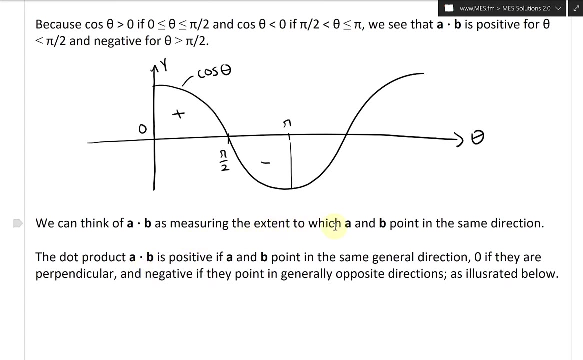 yeah. so it depends on the angle. it could be negative or positive. all right. going further, we can think of the dot product a, dot b- as measuring the extent to which a, yeah, a and b vectors point in the same general direction. so it's 0 if they are perpendicular and negative if 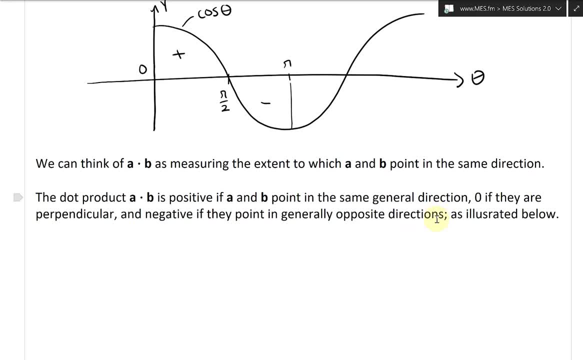 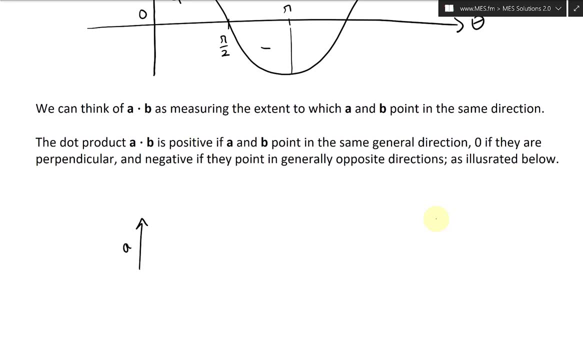 they point in generally opposite directions, as illustrated below. all right, so for example, let's say you had vectors a- this, this is a. you had a vector B like this: and this is a theta. let's put a data in between here. right, here is fix that up. so this is our B vector. there's. 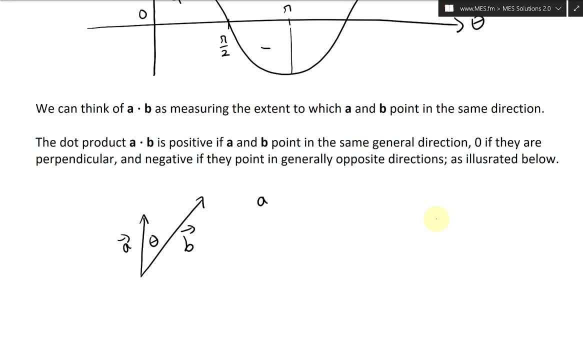 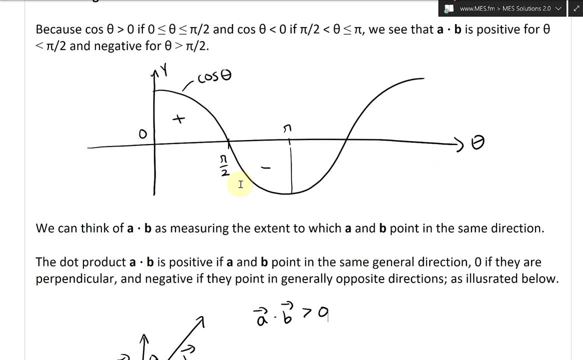 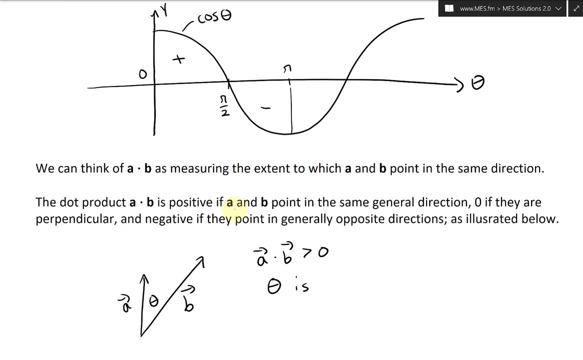 our angle between them is theta, so this is a small angle, this one here, a dot B would be greater than zero, because this angle is between here, so this angle is between there, so it's less than 90 degrees and in other words, A theta is acute like that, or less than less than pi over 2. 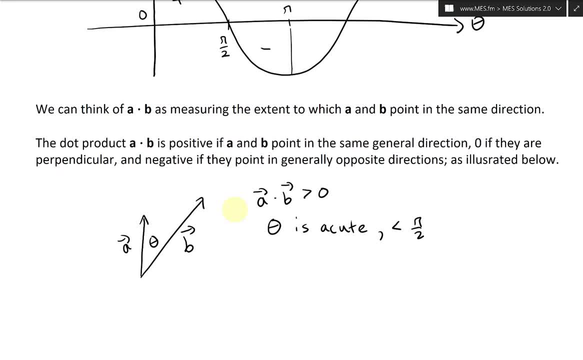 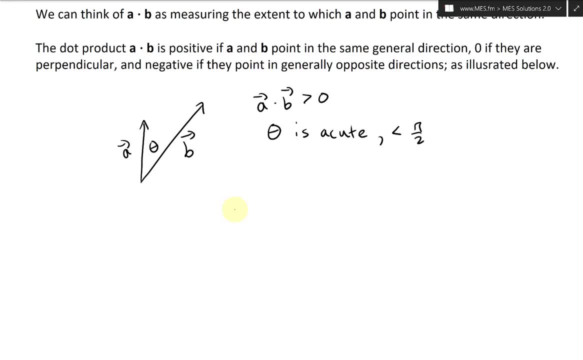 plus less than pi over 2, like that. and then if it equals to pi over 2, then that's going to be a 0 dot product and it's gonna be perpendicular like this. and this, this is a particular going to be our b vector, it's our a vector and as our angle is going to be, well, yeah, this angle. 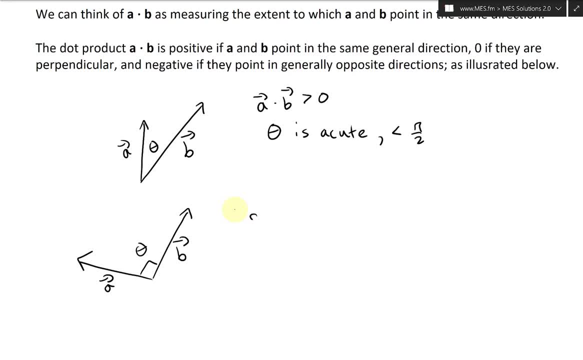 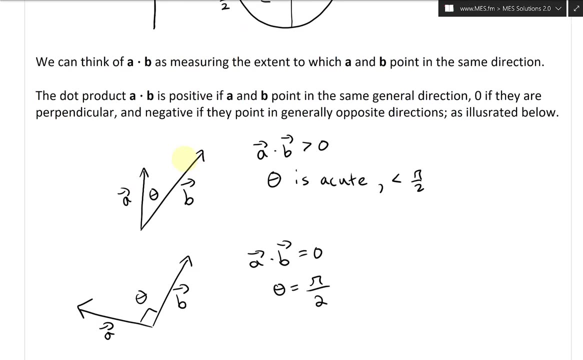 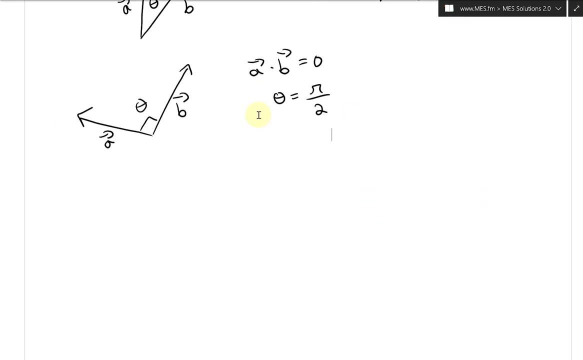 right here is uh 90 degrees, so a dot b equals to zero and theta equals to pi over two. or uh 90 degrees, pi over two radians. and then finally here, because uh, we show that it's negative for the angle is greater than pi over two. in other words, uh, if it is uh obtuse, so greater than 90. 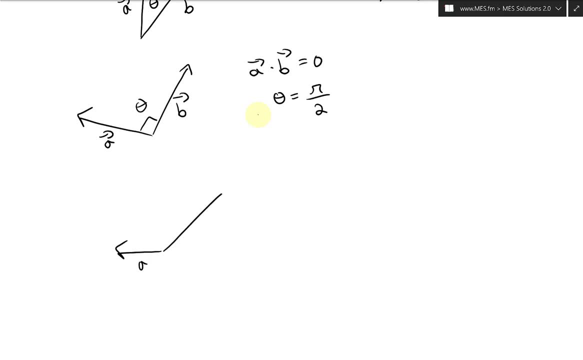 degrees. so let's say you had uh angle a and then this is angle b, i mean vector b, and there's the angle theta, like that, and that's very large. so we'll have a dot. b. vector is greater, i mean it's going to be less than zero, i mean negative. so this is uh. this theta is obtuse. 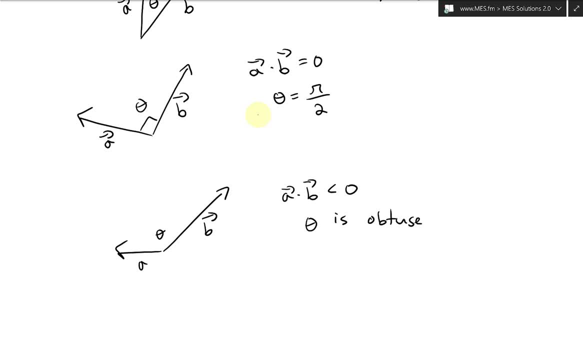 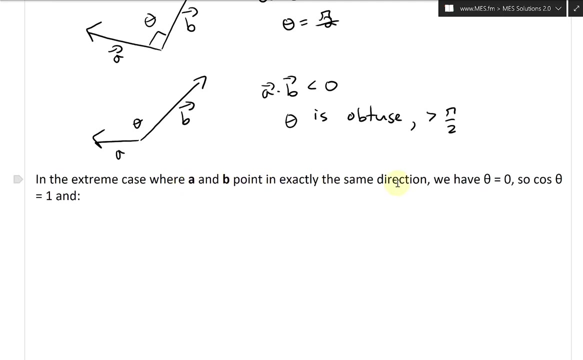 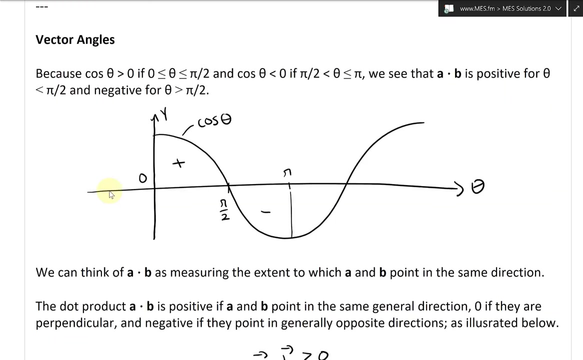 in other words, um, we'll have it as greater than pi over two. i guess it's a very, very fascinating stuff here. all right, and going further. so in the extreme case where a and d point in exactly the same direction, we have the angle, theta is equal to zero. so, cosine theta is equal to one because 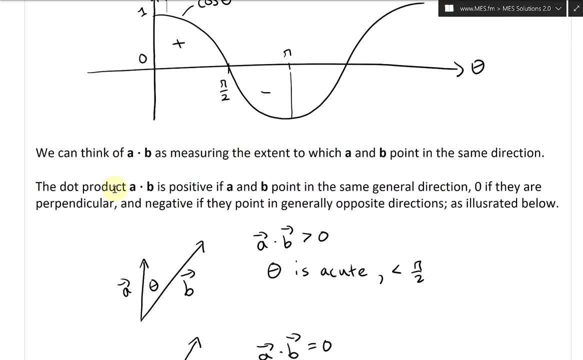 remember, this is just one there. so when a zero, it gets one, and then also when it's a positive, it gets a negative. so that's a positive, so that's a positive, so that's a positive. and then also when it's a positive, it gets a negative. so that's a positive, so that's a positive. 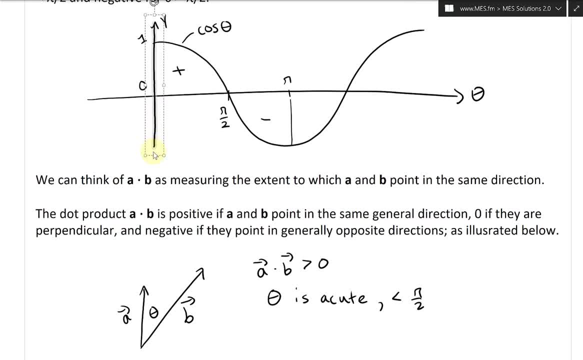 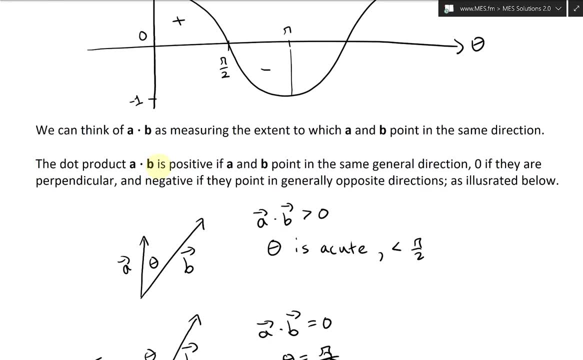 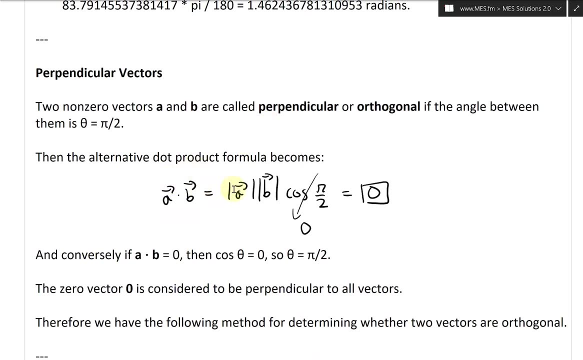 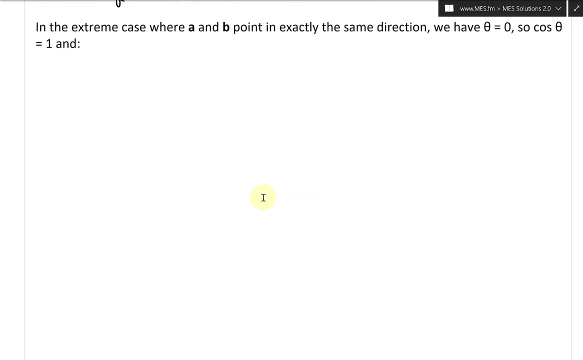 becomes negative one, just for reference, because we'll do this here soon and this is like, this is a negative one, like that. so the cosine theta is equal to one, in other words, a dot product. let's go that theorem right here. this is becomes one. this is equals to a dot B. equals to right here. equals the lengths times each. 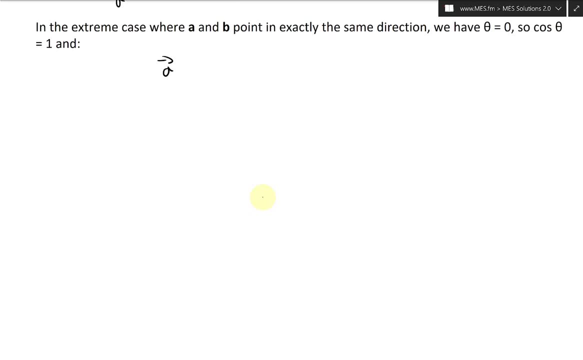 other. so in other words, we'll have a dot. B is equal to the lengths multiplied by each other, and yeah, so that's, that's. it is cos. cosine 0 is equal to, this is goes to 1 now, so I'll just leave it like that. 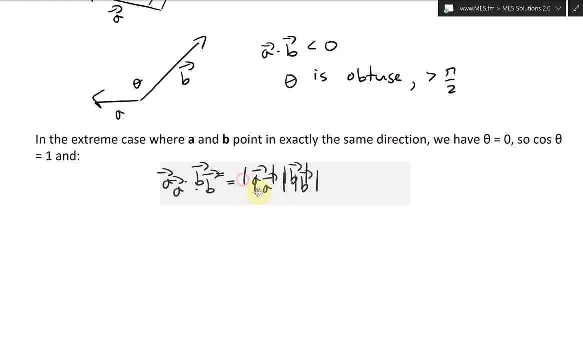 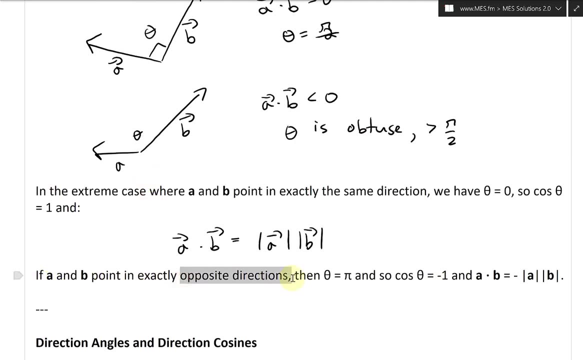 because we just wrote it all right. so that's what we have. that's fascinating stuff. all right, I don't know. lastly, if a and B point in exactly opposite directions, then the angle theta is equal to pi, so cosine theta is equal to negative 1 and a dot B. 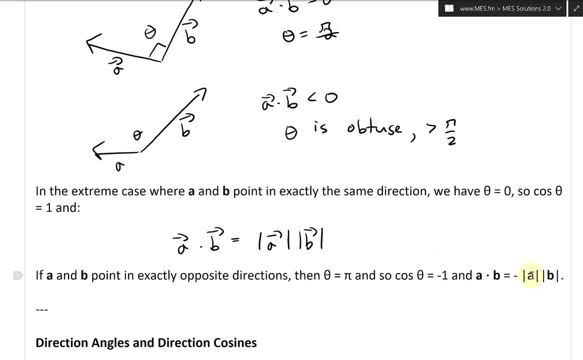 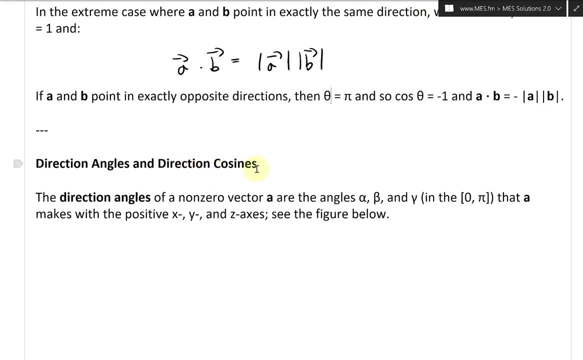 is going to equal to negative, a negative length, a times lengthy, yes, very faster, all right. so now let's go to the next section, that's on direction angles and direction cosines. so the direction angles of a non zero vector a are the angles alpha, beta and gamma. 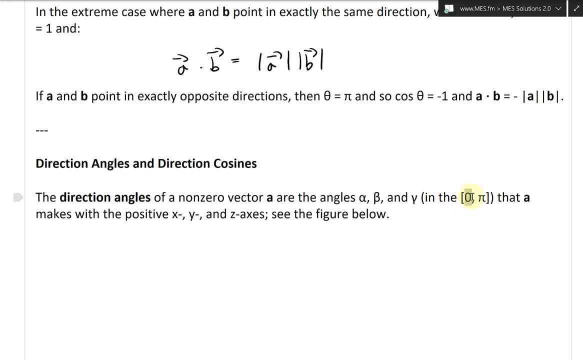 in the. this is in the again the domain from 0 to pi or an interval from 0 to pi, and this is a closed, this is closed bracket, so includes them. and yeah, and this is the direction angles that a makes with the positive x, y and Z axis. 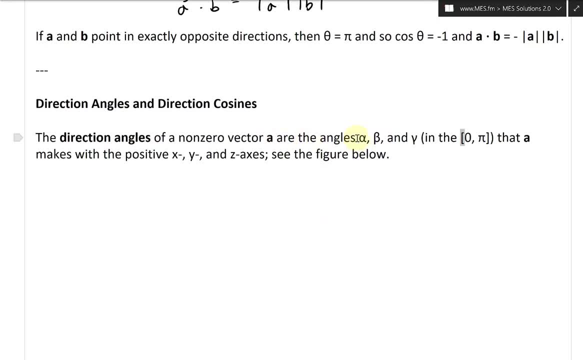 and see the figure below. so now we're looking at a three-dimensional and have all of these yeah angles. these are, yeah, these are the considered unit angles or whatnot, and this is based on the axis of the coordinate shrimp 체계 and the coordinate. 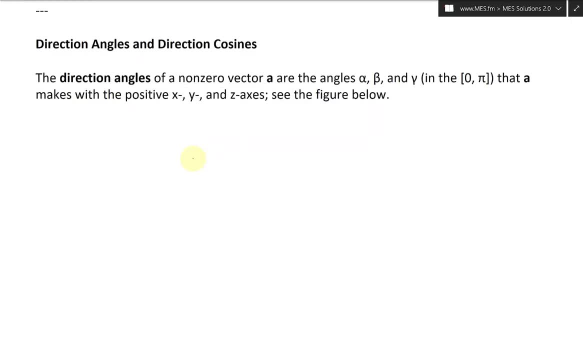 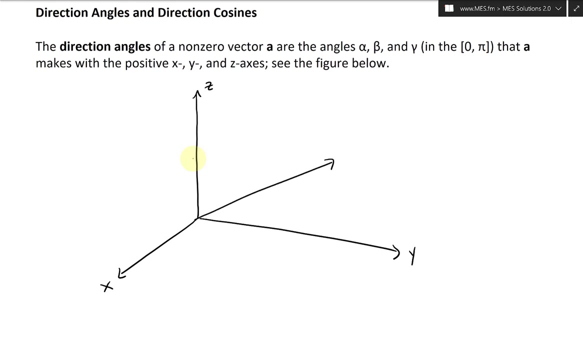 the system. so yeah, for example, if you let's just graph this out in 3d, so we have here, we have this is our z axis, let's draw our y axis and then this is our x axis, like that, all right, so as we have, and let's say we have a vector goes out here in 3d space, like that, and we're gonna do what i'm. 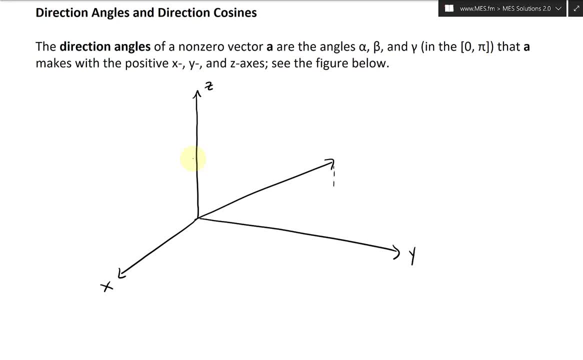 going to do is: yeah, let's just draw the components of this. i'm going to draw this 3d and the dash lines across down here, so it goes down like that and then it goes like this: all right, let's fix that up, and i'm going to draw it across here, perpendicular across there, and likewise for the vertical side. 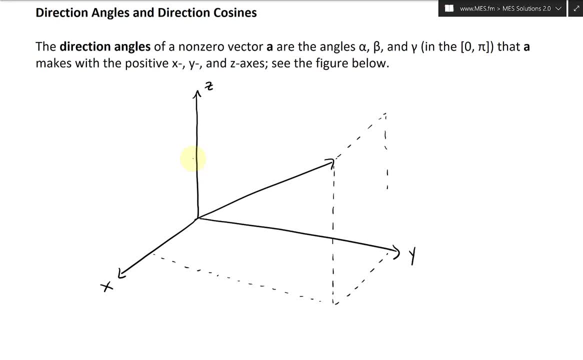 goes like that high part goes all the way down. so we try to draw a 3d rectangle, show it in 3d space and put this up as well, and then down here, and then down here, this across there, and let's fix it up like that: 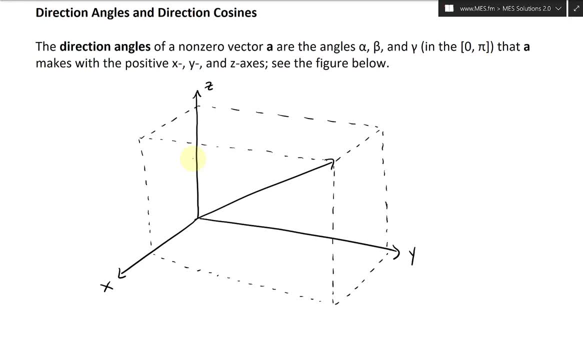 and uh, all right. so we drew, uh, this. there's the vector as fix the box up like that, all right, so now let's draw the angle. so this is the angles. uh, alpha is going to go from the x-axis to this angle, i mean to this vector. it's going to look like this: this is the alpha. 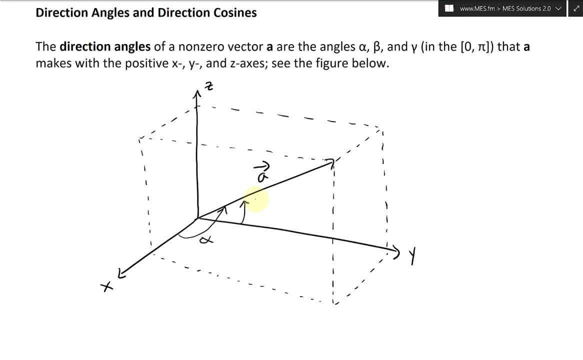 and then the y one is the beta that's going from the y-axis, that's beta, like that. and then, uh, and then the z-axis is the gamma going over to here, and this one is gamma. i got very fascinating stuff and i'm also going to draw a line here, this segment. 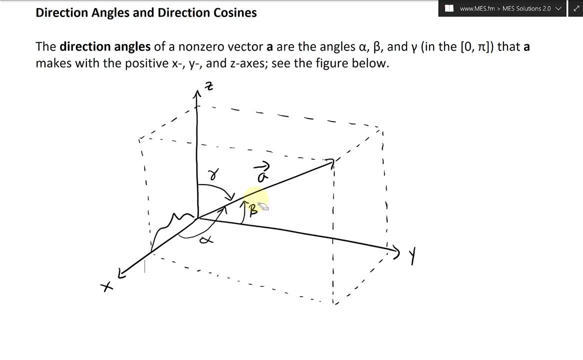 is a component, because we're going to use this. i'm going to point this out later. put this a bit better: this is a1, i got that distance a1, and the corresponding here is a2, and then the vertical is a3, and so on. all right, now what we have here is, uh, something very interesting. 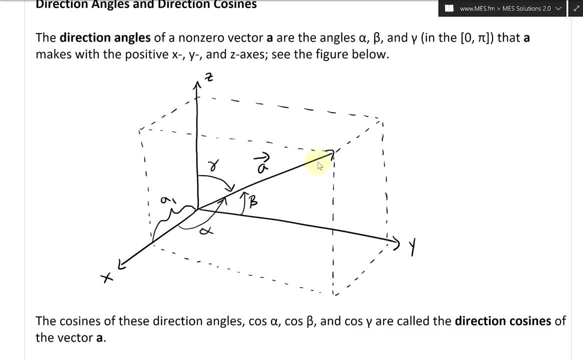 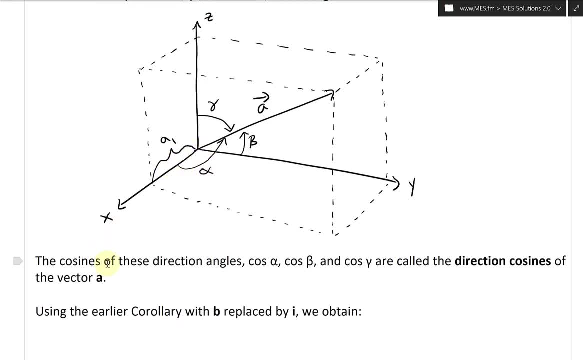 because if we take the cosines of every single one, notice we'll have the adjacent of every single one and the hypotenuse is the length of this vector a. so we take the cosines of every single one, yeah, the cosines of these uh direction angles, cosine um, alpha cosine, beta cosine. 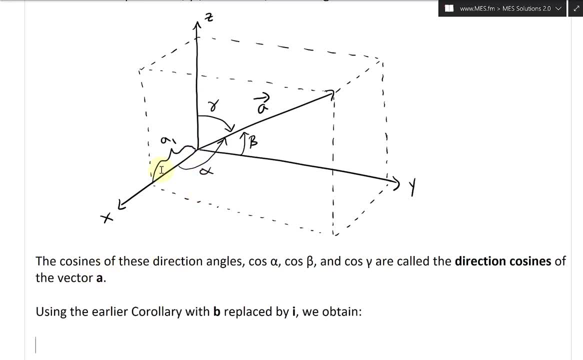 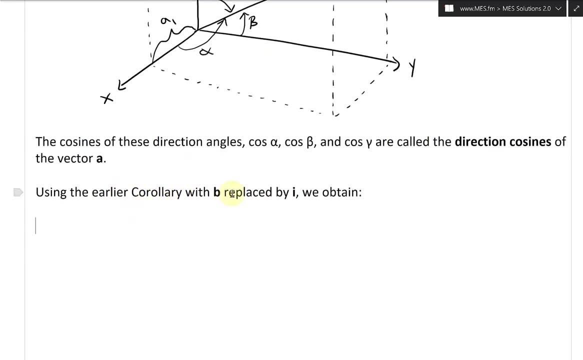 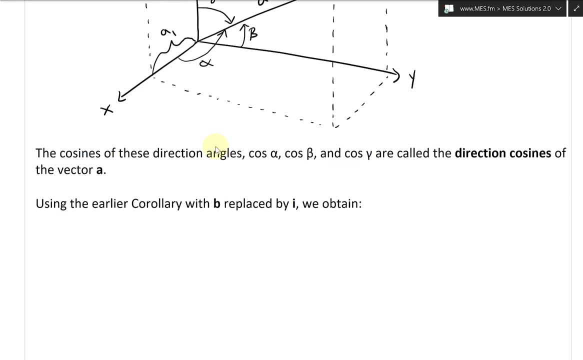 gamma are called the direction cosines of the vector a and those are just going to be the components of it. well, cosine times it by the length across it. so, using the earlier corollary with b replaced by i, which is the um, the x, uh, the x vector there, or just a unit vector in a. 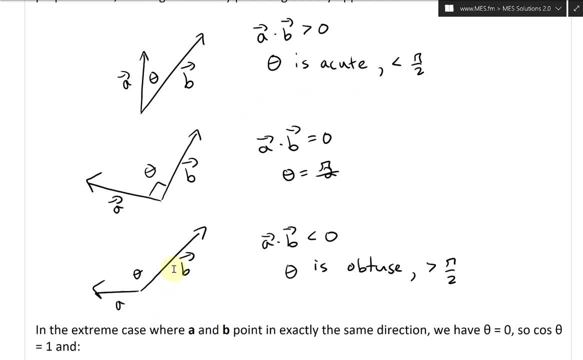 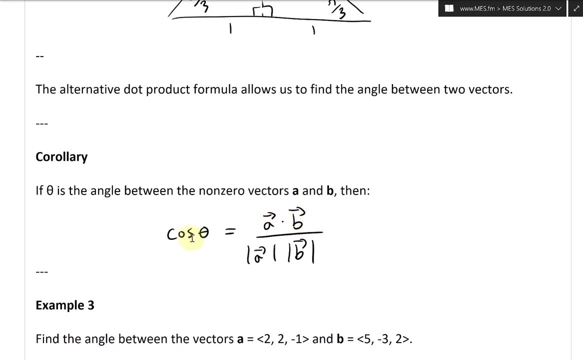 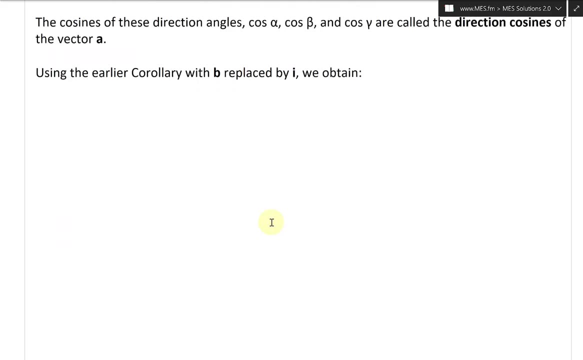 direction of x-axis we obtain. and then the corollary is just a cosine set up here. let's go back here. that's just this one, right here. we're going to replace b with i, so cosine theta equals to a dot dot b. instead of that we'll do dot i, all right. so let's write this down. so cosine alpha. 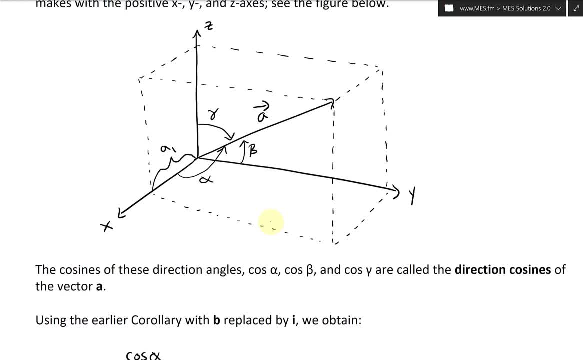 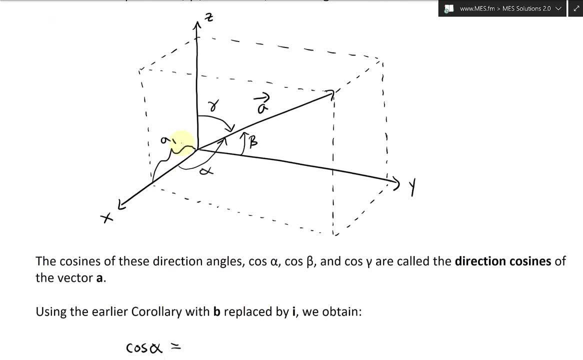 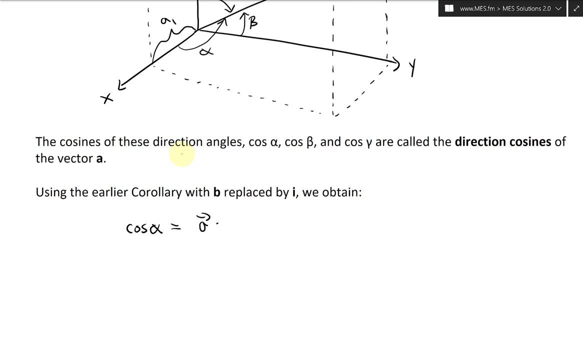 so we're going to replace that and we're going to write cosine alpha instead of cosine theta. we're going to: cosine alpha, here is equal to, and then we're going to use uh, the i, this part, right here. uh, it's going to be the i vector. let's put this here: uh, a, the, a vector, dot, the i vector, and then this is going to be: 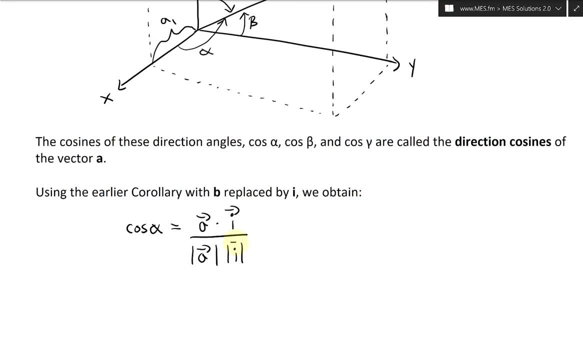 divided by a and then divided by b length. i'm going to divide it by the a length and then the b and then the i length. all right, all right here. i just thought, yeah, fix it all up. so a dot i divided by a length, and then the i length, and again the i is. uh, this is the i. 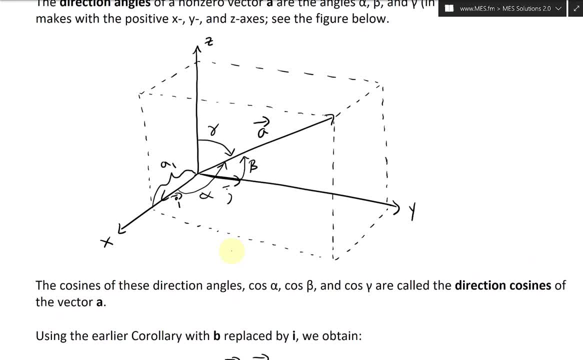 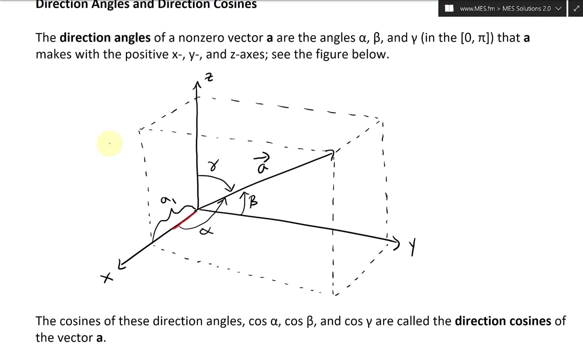 like that just over there, the i is there, this is the j and this is the uh z, etc. this is the k, uh k is going top, etc. and i'm just going to erase all these just for neatness. all right, yeah, although, however, it is important to include this either. 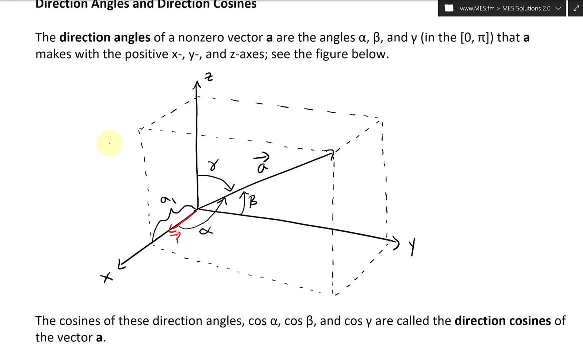 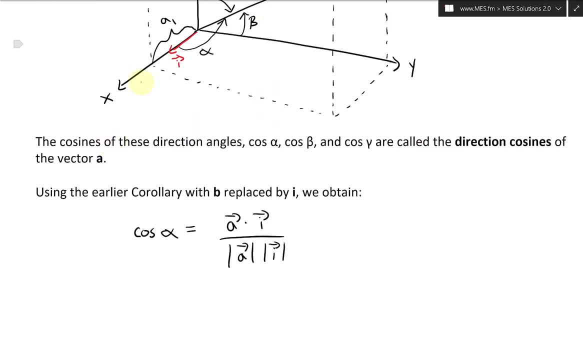 it's gonna be the I unit vector for the I standard basis vector I got. so let's say either- and it's a length, is one all right now, before I solve this- or simplified, I'm gonna do a recall again, recall from earlier video: what this all? 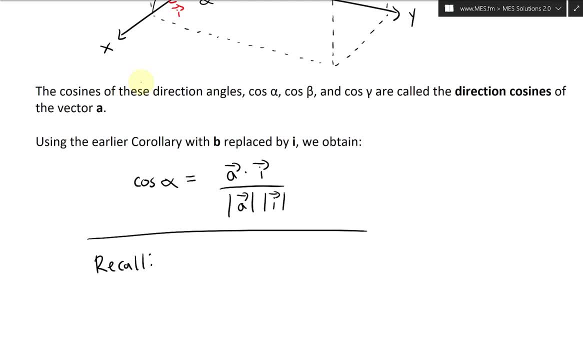 means the unit vector or the standard basis vector. I so I dot this just equals to one zero, zero like that. this here is zero, zero. yeah, so that's, that's just a how, its components of this vector and the length of it is just a unit. one is. 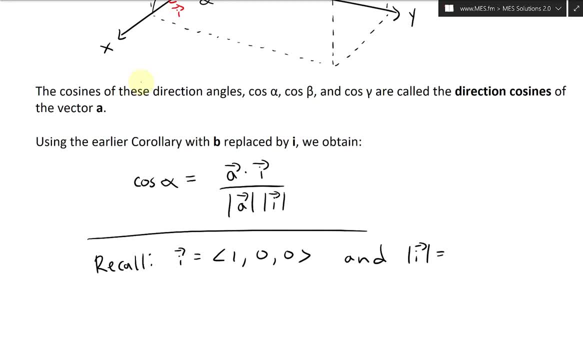 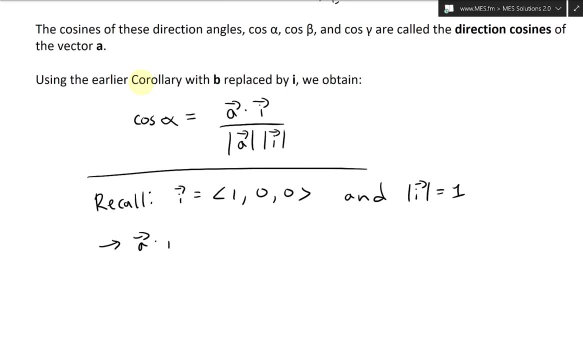 just one is equal to one, like that. so we have that in that. thus a, a, a, a dot I, or else, but recall that, well, I got. thus I'll leave that line out of there, all right, so thus a dot I is equal to well a one, a two, a three, dot one, zero, zero. 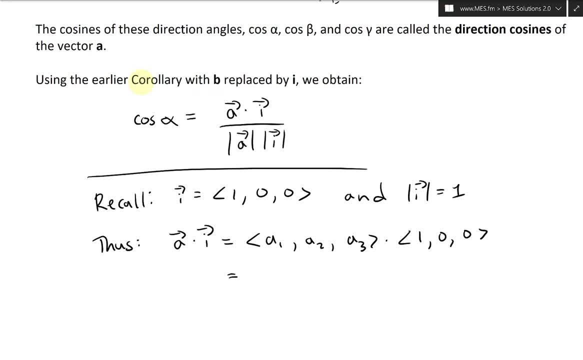 a two, a three dot one zero. this all equals to well the a ones times by one. this all equals to well the a ones times by one. this all equals to well the a ones times by one times of one plus the next one is times of one plus the next one is: 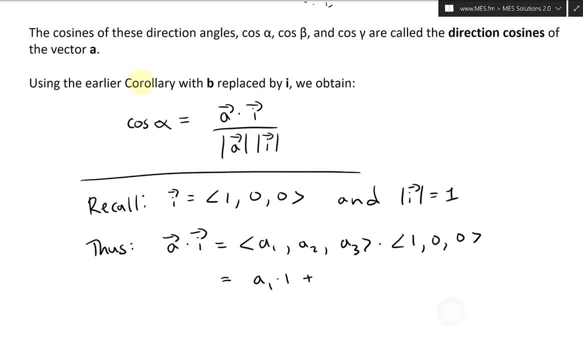 times of one plus the next one is going to be: well zero times a two times zero. going to be well zero times a two times zero going to be well zero times a two times zero, and so on. so, in other words, me zero, and so on. so, in other words, me zero. 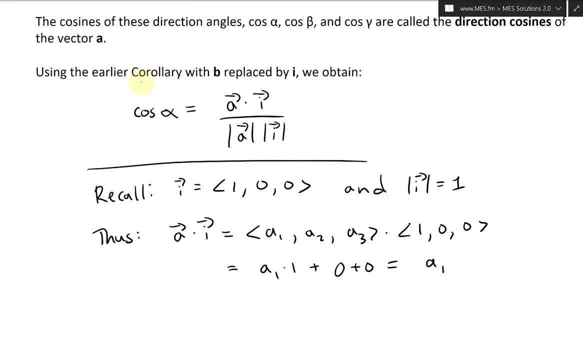 and so on. so, in other words, me, zero plus zero. this all equals to a one plus zero. this all equals to a one plus zero. this all equals to a one like that. yes, in other words, this equals like that. yes, in other words, this equals like that. yes, in other words, this equals to one. and then the a dot I is equal to. 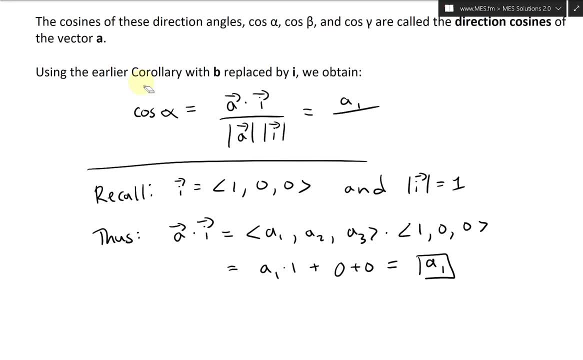 to one, and then the a dot I is equal to to one, and then the a dot I is equal to a one. this equals to a one over a one. a one. this equals to a one over a one. a one. this equals to a one over a one. oh yeah, the length: a like that where a one. 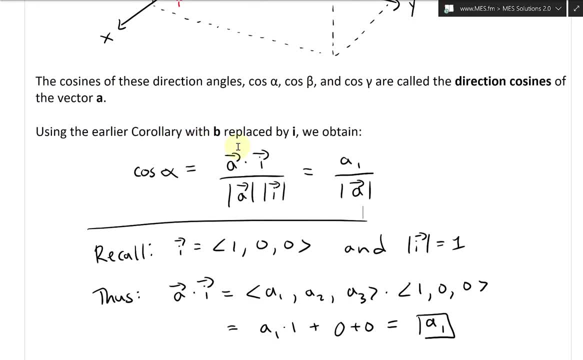 oh yeah, the length a like that where a one. oh yeah, the length, a like that where a one again. is it here? that's why I wrote again. is it here? that's why I wrote again. is it here? that's why I wrote it down there. there's a one, there's a this. 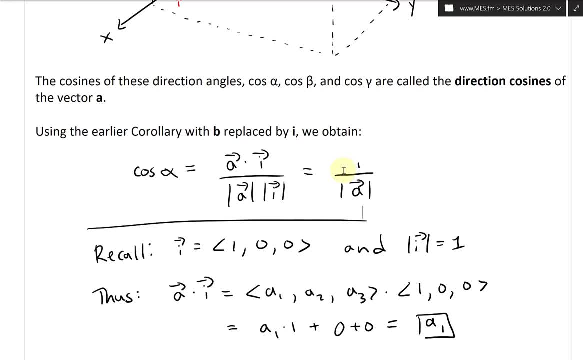 it down there there's a one, there's a this. it down there there's a this is this is actually some pretty fascinating stuff, is actually some pretty fascinating stuff, is actually some pretty fascinating stuff once you grasp it, because then you can. once you grasp it, because then you can. 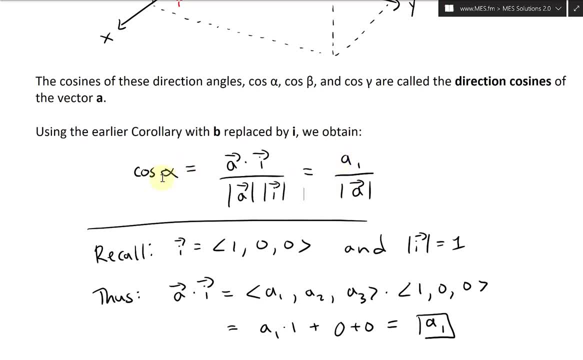 once you grasp it, because then you can move this a1 over to here. so this is move this a1 over to here. so this is move this a1 over to here. so this is gonna be cosine of this alpha times. by gonna be cosine of this alpha times by. 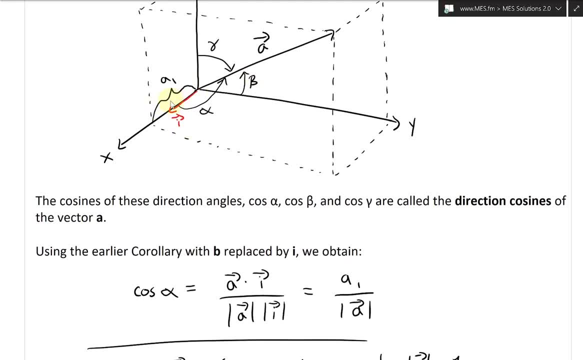 gonna be cosine of this alpha times by the length is equal to a1, so that's just. the length is equal to a1, so that's just. the length is equal to a1, so that's just the code direction: cosines passing stuff. the code direction: cosines passing stuff. 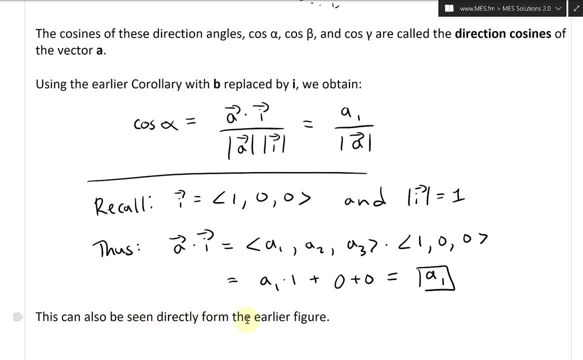 the code direction, cosines, passing stuff, and, as I just stated, this can also be, and, as I just stated, this can also be, and, as I just stated, this can also be seen directly from the earlier figure. so seen directly from the earlier figure. so seen directly from the earlier figure. so, if this is the angle, that's the 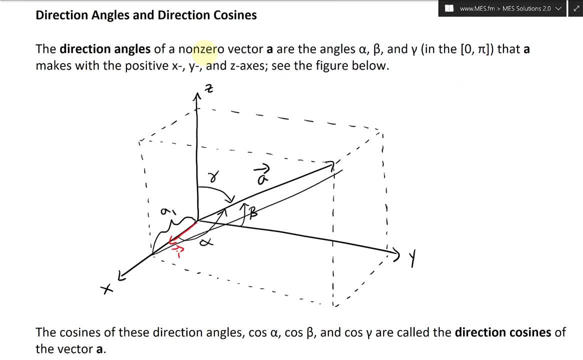 if this is the angle, that's the, if this is the angle, that's the component there then this, this triangle component there, then this, this triangle component, there, then this, this triangle. like that you draw this triangle way. like that you draw this triangle way, like that you draw this triangle way across there. I'll make this fit like: 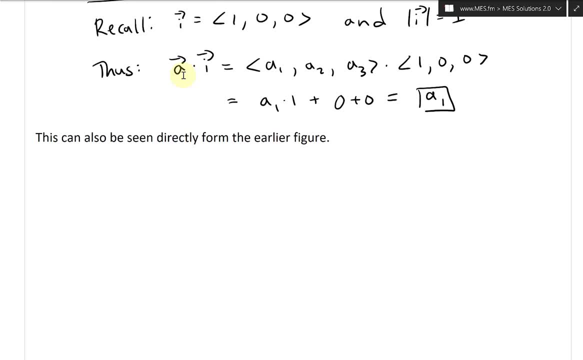 across there. I'll make this fit like across there. I'll make this fit like that. if you draw it all the way across that, if you draw it all the way across that, if you draw it all the way across there, we can end up getting is it'll have. 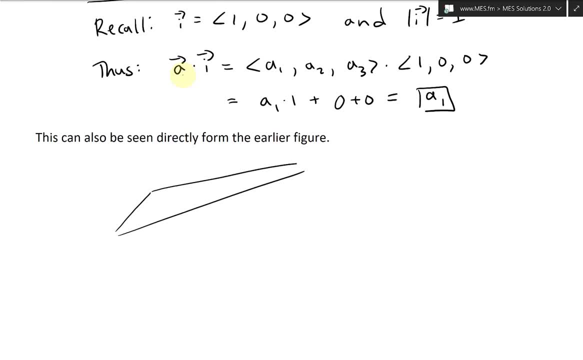 there we can end up getting. is it'll have there we can end up getting, is it'll have something like this? I'll just draw it something like this. I'll just draw it something like this. I'll just draw it only without that component, only without that component. 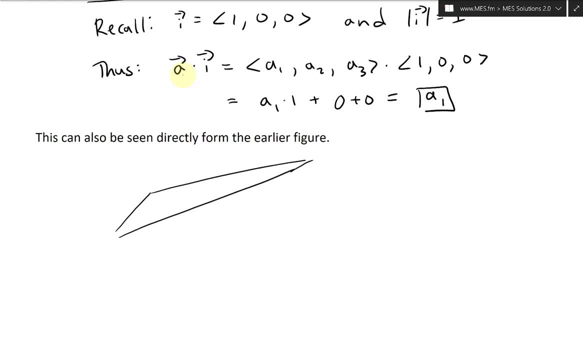 only without that component. oh my god, flat set up like this. oh my god, flat set up like this. oh my god, flat set up like this. and as this is a1, this is, this angle is, and as this is a1, this is, this angle is, and as this is, this angle is going to be our alpha, this length is going. 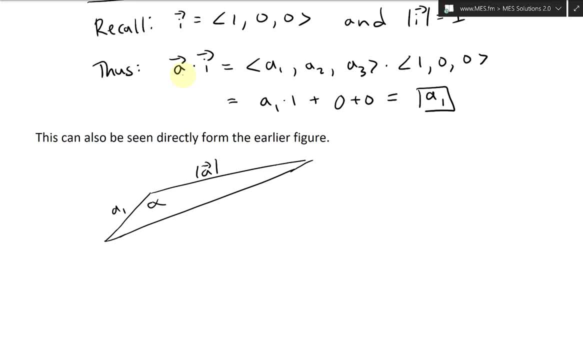 going to be our alpha. this length is going going to be our alpha. this length is going to be a1 like that, and yeah, this is to be a1 like that, and yeah, this is to be a1 like that and yeah, this is just. yeah, this is a bit skewed, but it that. 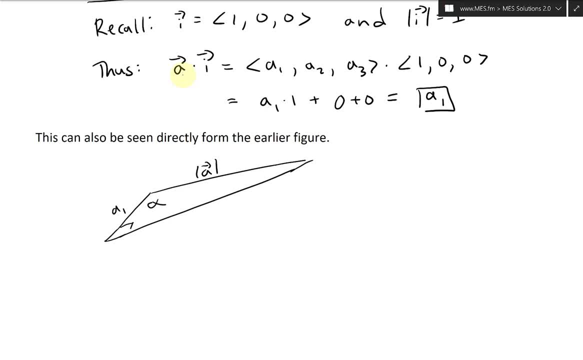 just yeah, this is a bit skewed, but it that just yeah, this is a bit skewed, but it that is the right angle there. because is the right angle there, because is the right angle there, because it's um, so yeah, so we have this going. it's um, so yeah, so we have this going. 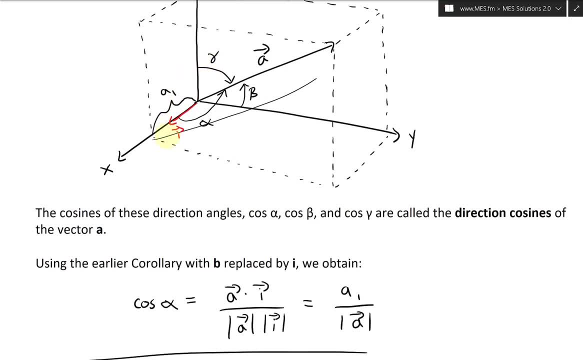 it's: um, so, yeah, so we have this going across from here to here, all the way to across from here to here, all the way to across from here to here, all the way to cross there. this is gonna be a perfect cross there. this is gonna be a perfect. 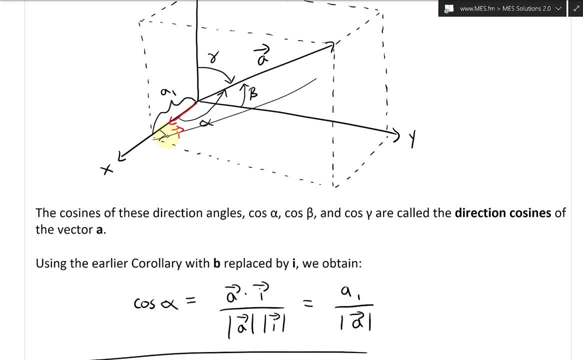 cross there. this is gonna be a perfect right angle across there, but uh, tilt it right angle across there. but uh, tilt it right angle across there. but uh, tilt it upwards, upwards, upwards, which is uh quite fascinating. so we got, which is uh quite fascinating, so we got. 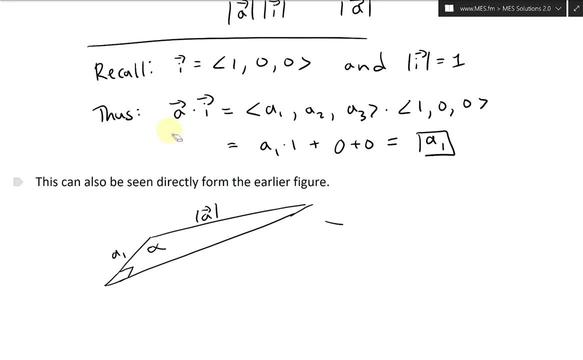 which is uh quite fascinating. so we got rid of that this right angle, and that is rid of that, this right angle, and that is rid of that, this right angle, and that is a yeah, that's just uh basic trigonometry. a yeah, that's just uh basic trigonometry. 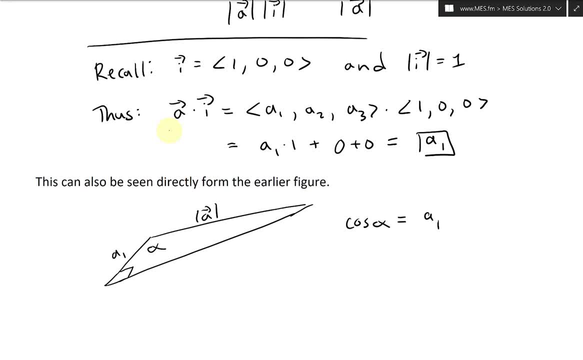 a yeah, that's just uh, basic trigonometry. and cosine theta equal to adjacent over, and cosine theta equal to adjacent over, and cosine theta equal to adjacent over hypotenuse, over, over, over a one length. we got a one length. we got a one length. we got yes, which is quite fascinating. all right, 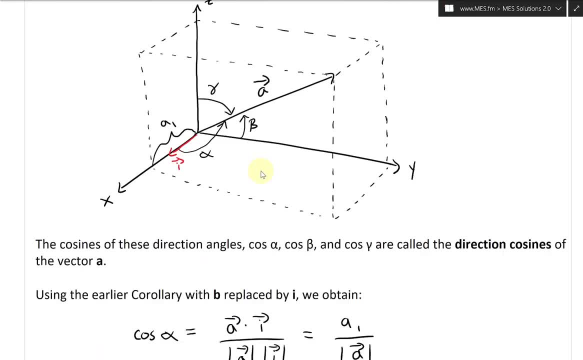 yes, which is quite fascinating. all right, yes, which is quite fascinating. all right, and uh. similarly, if we do the same thing and uh. similarly, if we do the same thing and uh. similarly, if we do the same thing for the other ones we use instead of i, for the other ones we use instead of i. 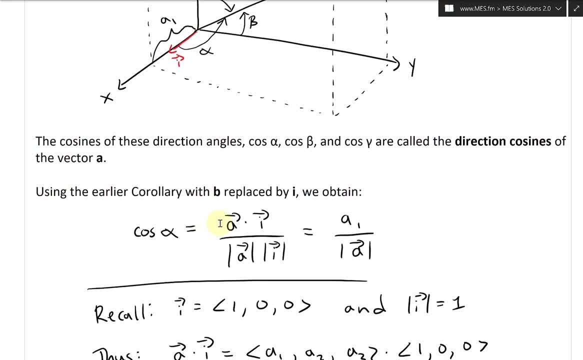 for the other ones we use instead of i, we use j, we use j, we use j, uh, we use k, etc. and because number this, uh, we use k, etc. and because number this, uh, we use k, etc. and because number this one's going to be one, zero, zero, j is. one's going to be one zero, zero j is one's going to be one zero, zero j is going to be zero one zero k is going to going to be zero one zero k is going to going to be zero one zero k is going to be zero, zero one. 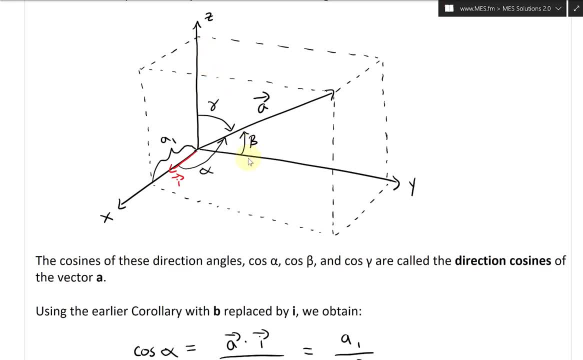 be zero zero one, be zero, zero one. and you're basically just gonna be using and you're basically just gonna be using, and you're basically just gonna be using different angle, but to meet exactly the different angle, but to meet exactly the different angle, but to meet exactly the same. 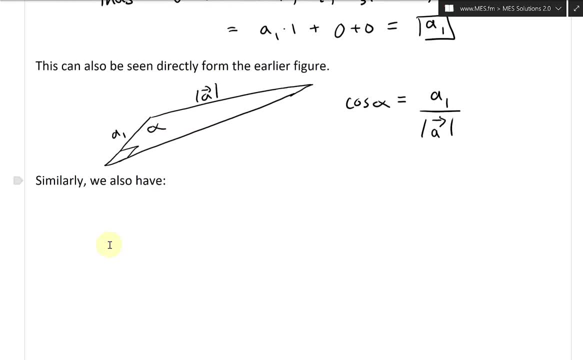 same same setup. similarly. we also have setup similarly. we also have setup similarly we also have for the y component cosine. for the y component cosine. for the y component cosine, beta is equal to a2. beta is equal to a2. beta is equal to a2 over the length of the a vector. 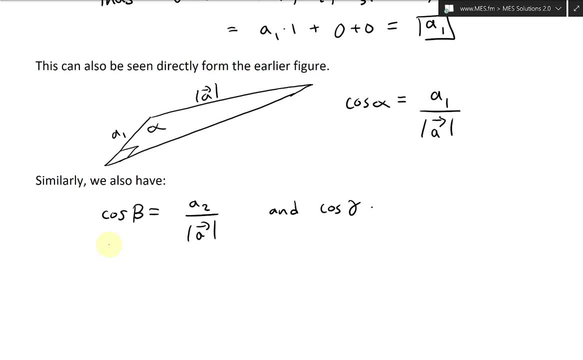 over the length of the a vector. over the length of the a vector, and cosine gamma is going to equal to, and cosine gamma is going to equal to, and cosine gamma is going to equal to. a3 component, because i know everything. a3 component, because i know everything. 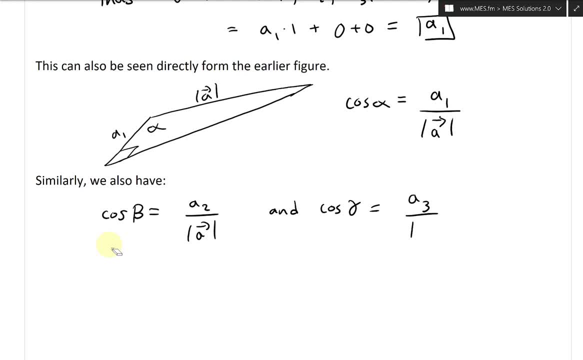 a3 component, because i know everything else cancels when you're multiplying by else. cancels when you're multiplying by else. cancels when you're multiplying by the the, the k vector, but the last one there, so a3 k vector, but the last one there, so a3. 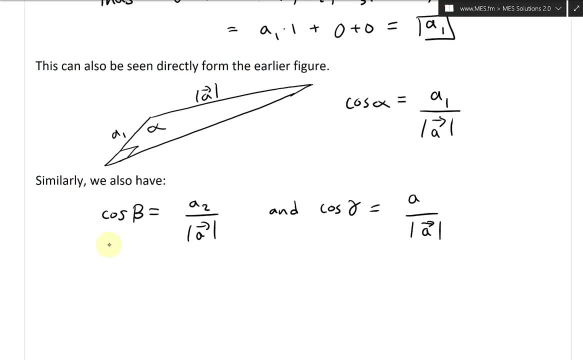 k vector, but the last one there, so a3, and this is going to be, and this is going to be, and this is going to be vector like that vector like that vector like that. all right, so now going further, uh by. all right, so now going further, uh by. 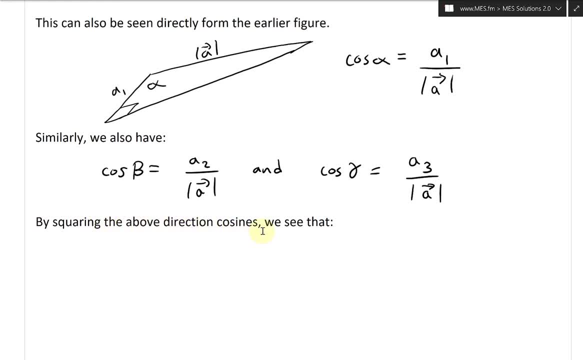 all right, so now going further. uh, by squaring the above direction, cosines, we squaring the above direction, cosines, we squaring the above direction, cosines. we see that, see that, see that. i mean i mean squaring and adding. so, i mean i mean squaring and adding so. 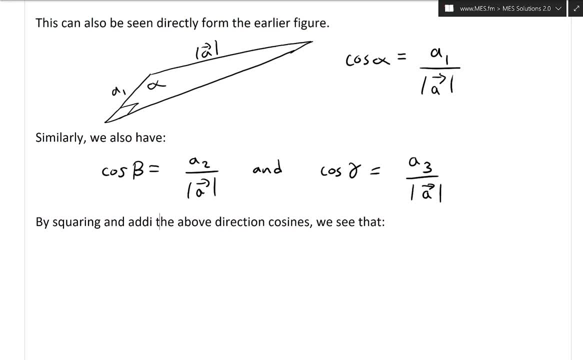 i mean, i mean squaring and adding, so squaring, squaring, squaring and adding and adding and adding. the above direction cosines, we see that, the above direction cosines, we see that, the above direction cosines, we see that, well, if we take every single one cosine, 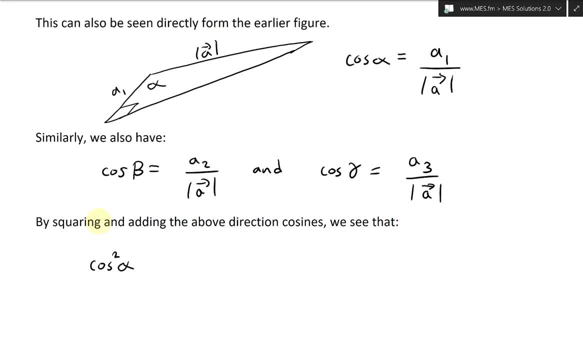 well, if we take every single one cosine. well, if we take every single one cosine alpha- yeah. cosine squared alpha- alpha- yeah. cosine squared alpha- alpha- yeah. cosine squared alpha. or cosine alpha squared plus, or cosine alpha squared plus, or cosine alpha squared plus cosine squared of the beta one plus. 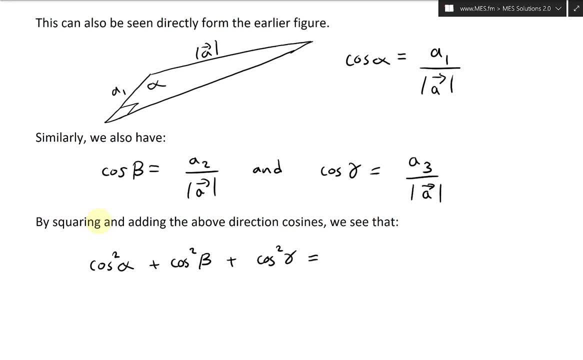 cosine squared of the beta one plus cosine squared of the beta one plus cosine squared of the cosine squared of the cosine squared of the gamma. this equals two. well notice every gamma. this equals two. well notice, every gamma. this equals two. well notice, every single one has this one divided by. 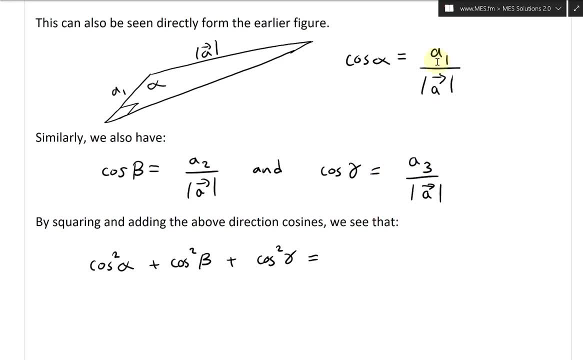 single one. has this one divided by single one? has this one divided by: uh, the length a? then you have this: a1, uh the length a, then you have this a1, uh, the length a, then you have this a1, a2, etc. so this just equals to: a2, etc. so this just equals to a2, etc. so this just equals to one over, and we're going to be squaring one over and we're going to be squaring one over, and we're going to be squaring it all. well, might as well for. 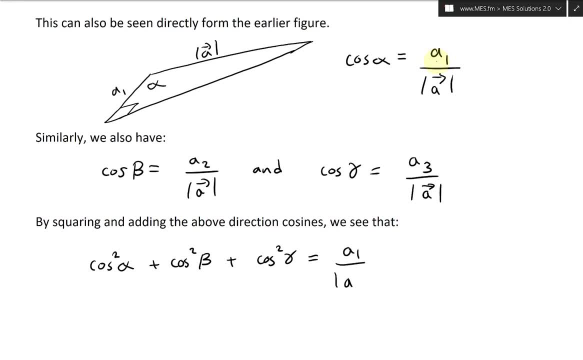 it all. well, might as well for it all. well, might as well for completeness. just write it all together, completeness. just write it all together, completeness. just write it all together. so a1 over, so a1 over, so a1 over. uh, this is going to be a like that. 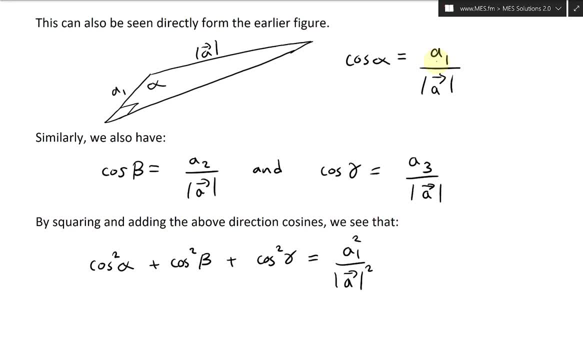 uh, this is going to be a like that. uh, this is going to be a like that: squared, so we're squaring it squared, so we're squaring it squared, so we're squaring it squared, squared, squared, squared, squared, squared, and then plus a, and then plus a. 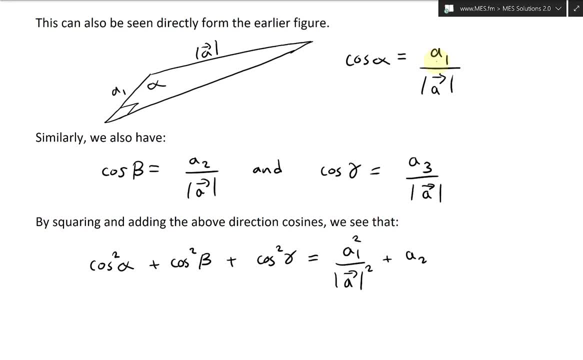 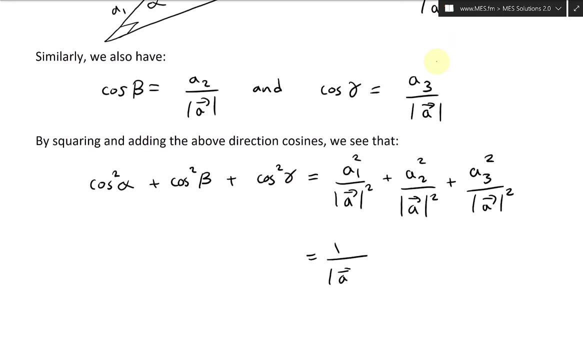 and then plus a uh two, uh two, uh two. a two squared, a two squared, a two squared squared, plus a, plus a three squared, three squared, three squared, like that, like that, like that. factor it out like that, factor it out like that, factor it out like this: 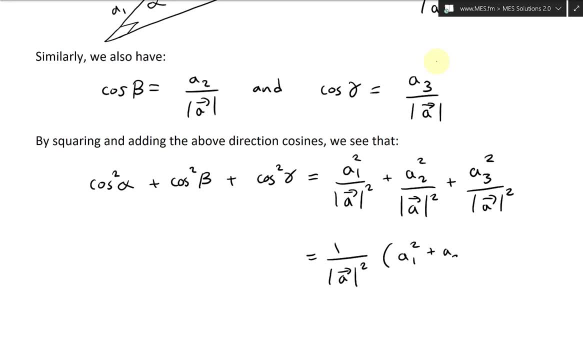 like this, like this: now we're going to get a a1 squared plus. now we're going to get a a1 squared plus. now we're going to get a a1 squared plus a2 squared, plus a2 squared, plus a2 squared plus a3 squared, and this one right here, uh. 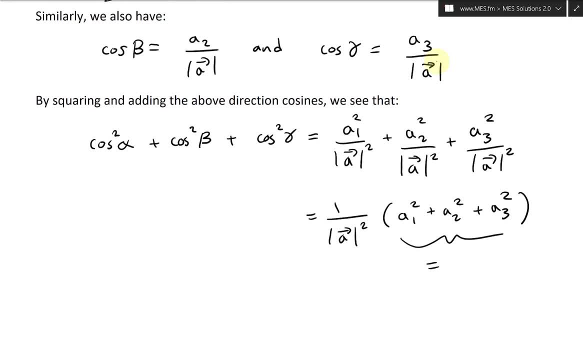 a3 squared, and this one right here. uh, a3 squared, and this one right here. uh, this is just. this is just. this is just. this is equals to again, that's just the uh. this is equals to again, that's just the uh. this is equals to again, that's just the uh. three, three dimensional trigonometric. 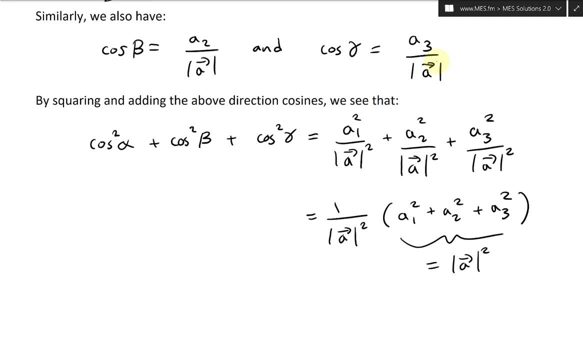 three, three dimensional trigonometric, three, three dimensional trigonometric function, function, function. that's just going to be a squared. that's just going to be a squared. that's just going to be a squared. yeah, in other words, this whole thing. yeah, in other words, this whole thing. 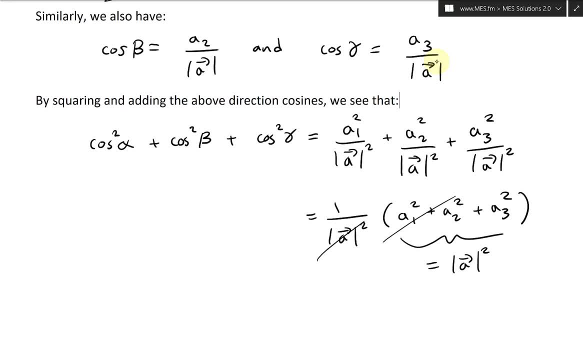 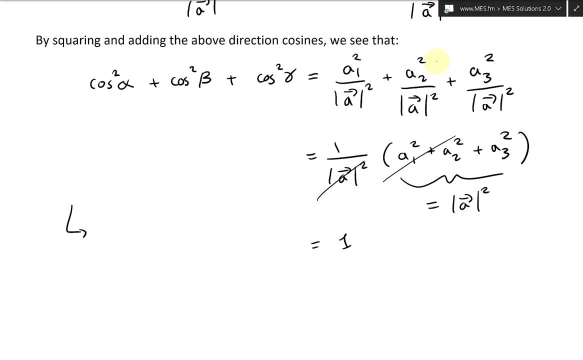 yeah, in other words, this whole thing cancels, cancels, cancels, and this cancel this, and this cancel this, and this cancel this. so this is equals to one, so this is equals to one, so this is equals to one, so this equals to one. in other words, 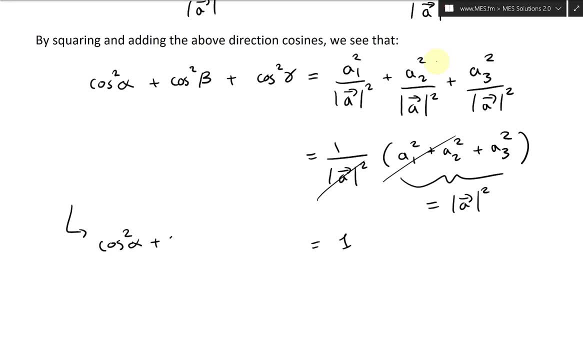 so this equals to one. in other words, so this equals to one. in other words, just down here, cosine squared alpha. just down here, cosine squared alpha. just down here, cosine squared alpha plus cosine plus cosine squared beta plus plus cosine squared beta plus plus cosine squared beta plus cosine squared gamma equals to: 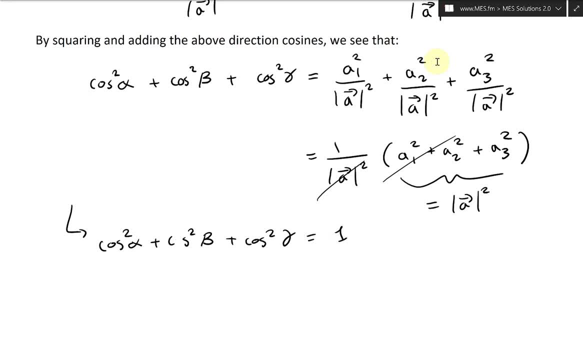 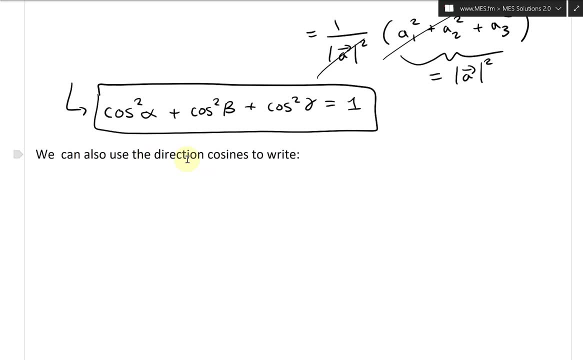 cosine squared gamma equals to cosine squared gamma equals to uh pi. a equals to one, uh pi a equals to one, uh pi. a equals to one. like that, like that, like that, all right going further. we can also use all right, going further. we can also use all right going further. we can also use the direction cosines to. 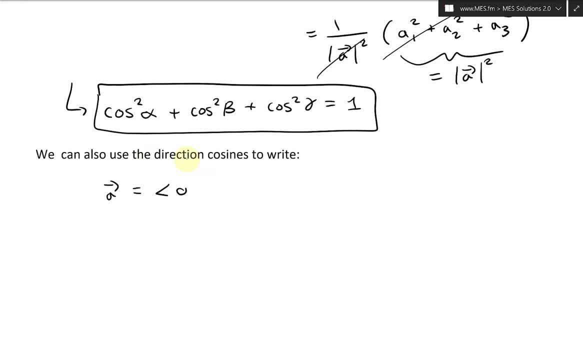 the direction cosines. to the direction cosines. to write. and let's just write our vector a: write. and let's just write our vector a write. and let's just write our vector a with its components a1 with its components a1. with its components a1, a2, a3. this equals: 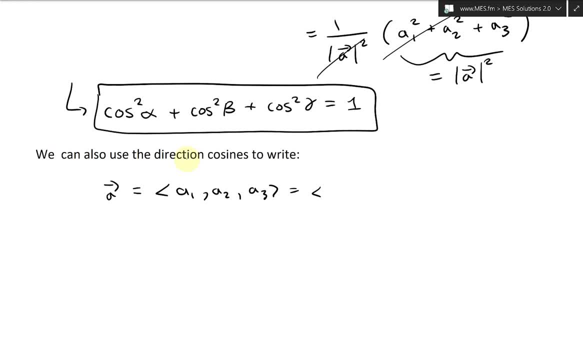 a2- a3- this equals a2- a3- this equals two. and then we could write these all two, and then we could write these all two, and then we could write these all out: uh, using the a1 number: a1 is just out. uh, using the a1 number: a1 is just. 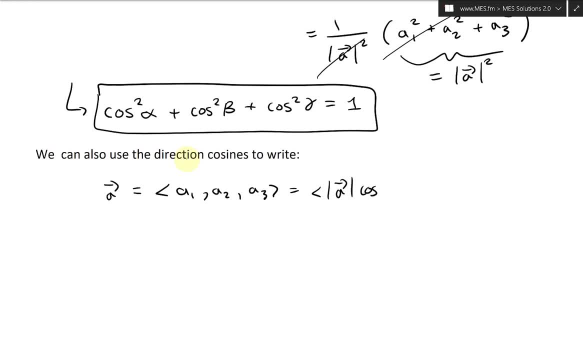 out, uh, using the a1 number. a1 is just going to be the going to be the going to be the length a times by the cosine of the length. a times by the cosine of the length, a times by the cosine of the, i mean the length a. 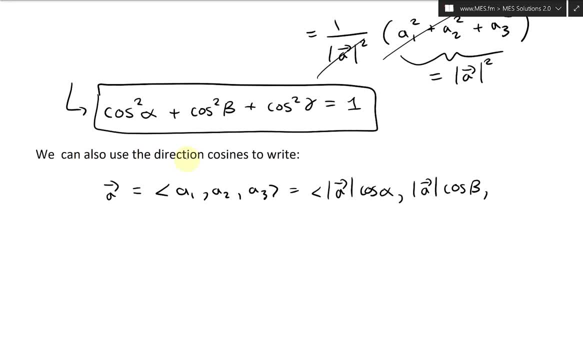 i mean the length a, i mean the length a multiplied by cosine beta, multiplied by cosine beta, multiplied by cosine beta. and then length a multiplied by the, and then length a multiplied by the, and then length a multiplied by the cosine, cosine, cosine, gamma, like that, gamma, like that. 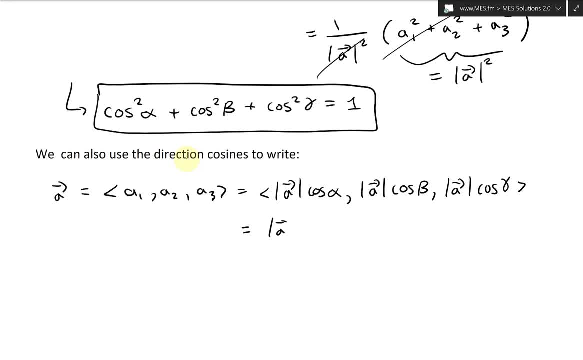 gamma, like that. all right, let's move that over. and now, all right, let's move that over. and now all right, let's move that over. and now just factor out the length, just factor out the length. just factor out the length. a like that cosine, a like that cosine. 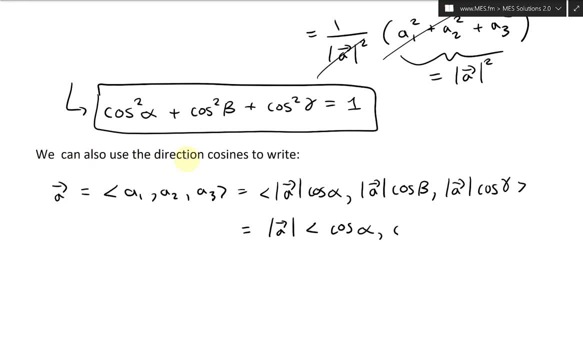 a like that cosine alpha and then cosine beta and then cosine beta and then cosine beta, cosine gamma, cosine gamma, cosine gamma. it's quite, it's quite, it's quite fast, it's quite fast. fascinating. and now just factor out this fascinating. and now just factor out this. 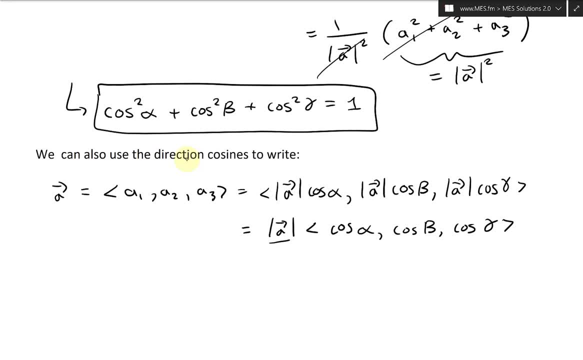 fascinating. and now just factor out this whole thing out, move it over whole thing out. move it over whole thing out. move it over, so, in other words, and move it all the so, in other words, and move it all the so, in other words, and move it all the way to the other side. 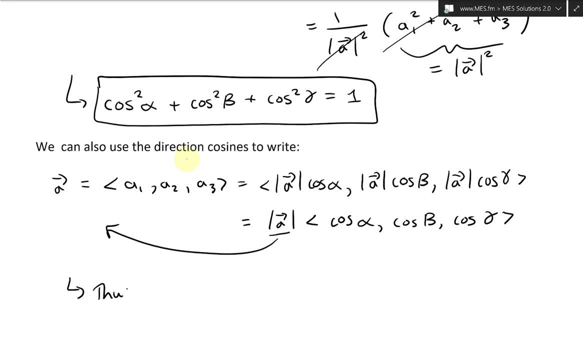 way to the other side, way to the other side. so what we get is thus so. what we get is thus so. what we get is thus: plus. we have one over plus, we have one over plus, we have one over the length. times it by the length, times it by. 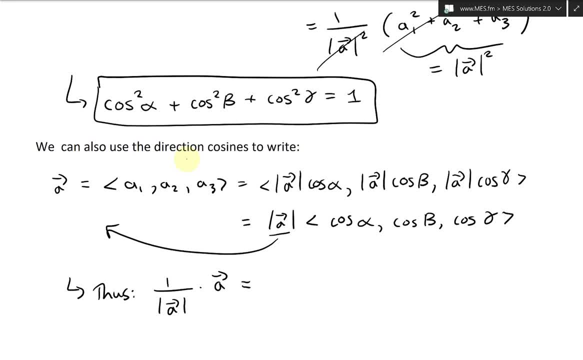 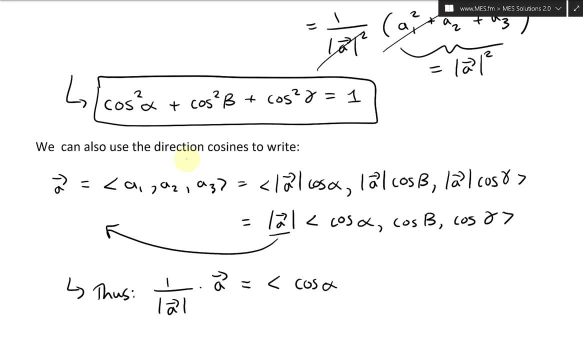 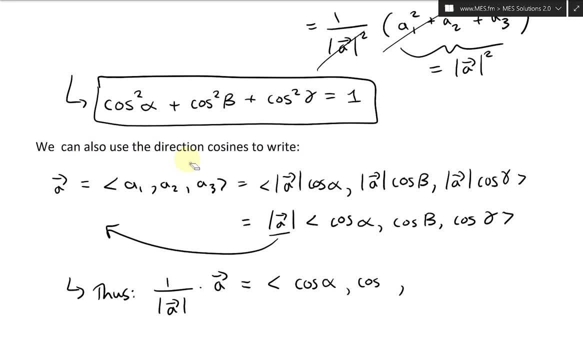 cosine, alpha, cosine, alpha, cosine, beta, cosine, beta, cosine, beta. uh put a better b, uh put a better b, uh put a better b. cosine, cosine, cosine, gamma, gamma, gamma. so this better be like that or better. so this better be like that or better. so this better be like that or better, beta. 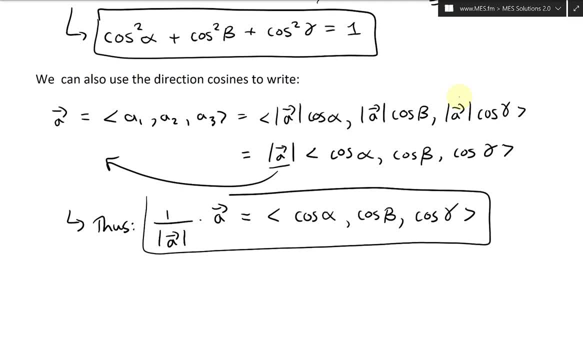 beta, beta. all right. so now let's just box this. all right. so now let's just box this. all right. so now let's just box this whole thing in yes, fascinating stuff, whole thing in yes, fascinating stuff, whole thing in yes, fascinating stuff. and now what this equation says is that 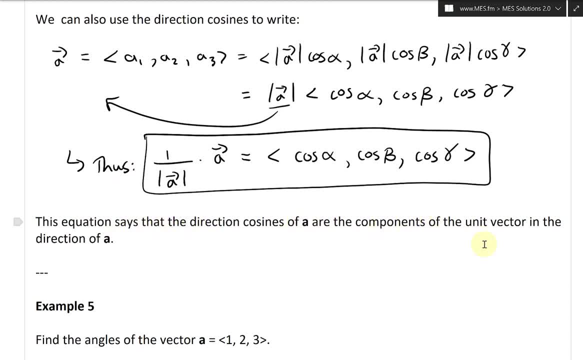 and now what this equation says is that. and now what this equation says is that the direction, the direction, the direction. cosines of a are the components of the cosines of a. are the components of the cosines of a are the components of the unit vector. 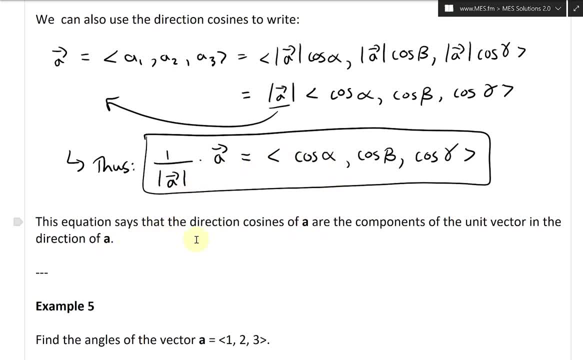 unit vector. unit vector, uh, in the direction of a which is uh, uh in the direction of a, which is uh, uh in the direction of a which is, uh, quite fascinating. this is a unit vector, quite fascinating. this is a unit vector quite fascinating. this is a unit vector, basically. so, if you have length, a, i mean. basically so if you have length a, i mean basically so if you have length a, i mean if you have vector a, if you look at the, if you have vector a, if you look at the, if you have vector a, if you look at the length of it, it's gonna be this: length of it it's gonna be this. length of it, it's gonna be this, but then this is just a scalar number. so, but then this is just a scalar number. so, but then this is just a scalar number, so you're dividing by it. you're dividing by it. 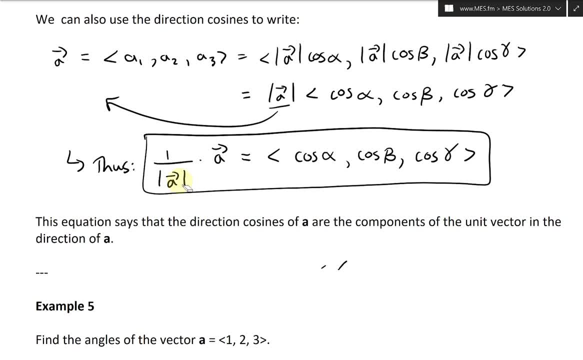 you're dividing by it, so you're going to equal to one, so it's so. you're going to equal to one, so it's so. you're going to equal to one. so it's going to be length one going to be length one, going to be length one, and it's going to be the direction of a. so 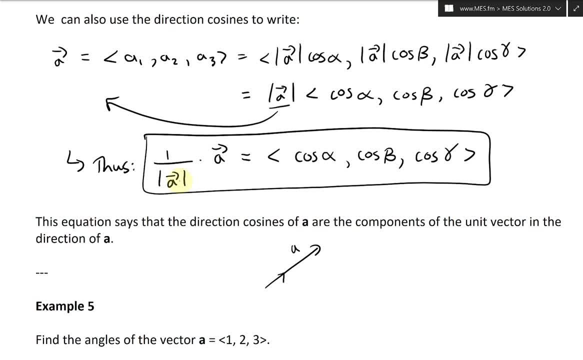 and it's going to be the direction of a. so, and it's going to be the direction of a. so if you have a like this, if you have a like this, if you have a like this, it's going to go in the unit vector. it's going to go in the unit vector. 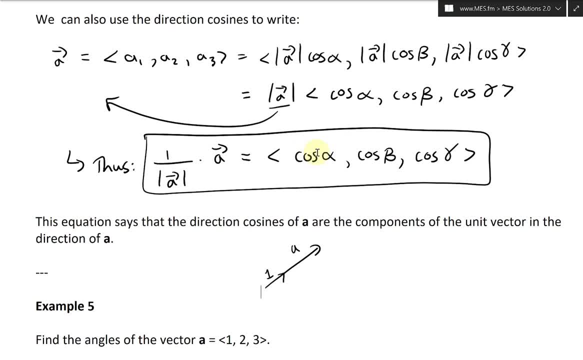 it's going to go in the unit vector. here's going to be length. one of the here's going to be length. one of the here's going to be length. one of the components there, components there, components there, and all these cosines are going to be all. 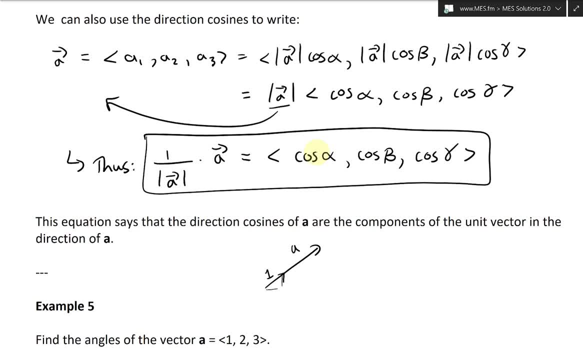 and all these cosines are going to be all, and all these cosines are going to be all of the ratios of the, of the ratios of the, of the ratios of the of that rectangle box, etc. of that rectangle box, etc. of that rectangle box, etc. uh, as before, 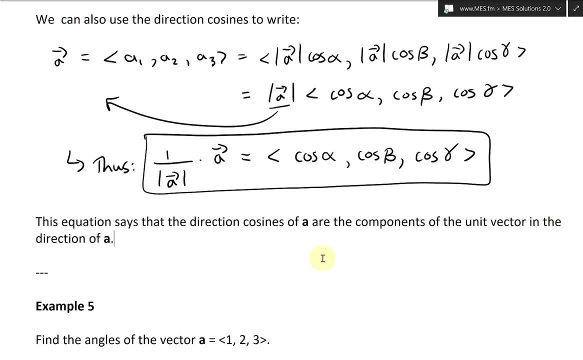 uh, as before. uh, as before. now, here's drew a better rectangle box. now, here's drew a better rectangle box. now, here's drew a better rectangle box, but anyways, it's just the um. but anyways, it's just the um. but anyways, it's just the um. it's just the x, y, z components, or i j. 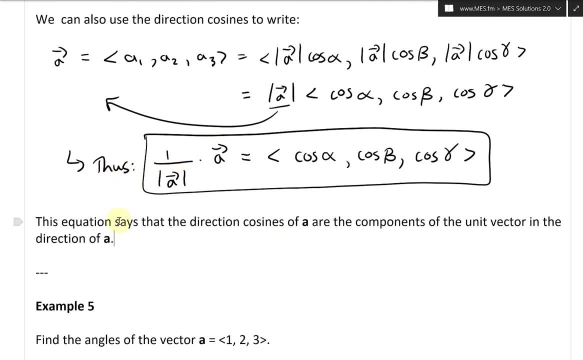 it's just the x, y, z components, or i j it's just the x, y, z components, or i j k components of it. serious fasting stuff. k components of it- serious fasting stuff, k components of it, serious fasting stuff. so, going further, let's take a look at. 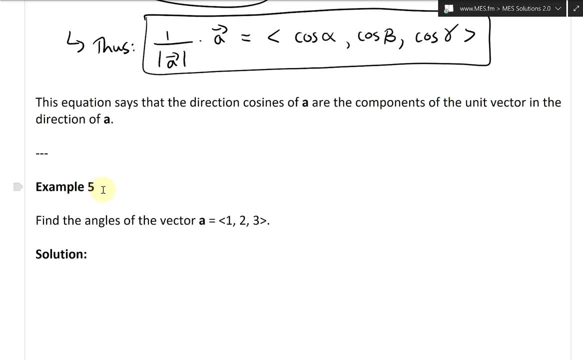 so going further, let's take a look at. so going further, let's take a look at example, example, example five. and this one states: find the five. and this one states: find the five. and this one states: find the direction angles of the vector a. direction angles of the vector a. 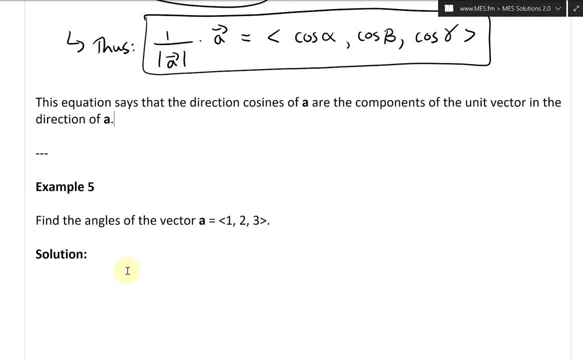 direction angles of the vector a, which is has components one, two and three, which is has components one, two and three, which is has components one, two and three. all right, so now, if we were to solve all right, so now, if we were to solve all right, so now, if we were to solve this. well, we know that, uh, the. 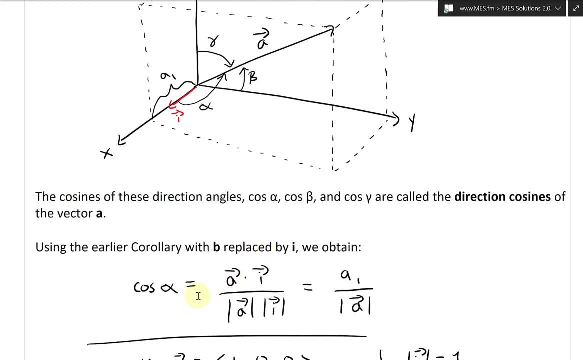 this well, we know that. uh, the this well, we know that. uh, the direction angle, or the direction direction angle, or the direction direction angle, or the direction cosines, uh, if you just go back above cosines, uh, if you just go back above cosines, uh, if you just go back above here, it's just going to be a1 over uh. 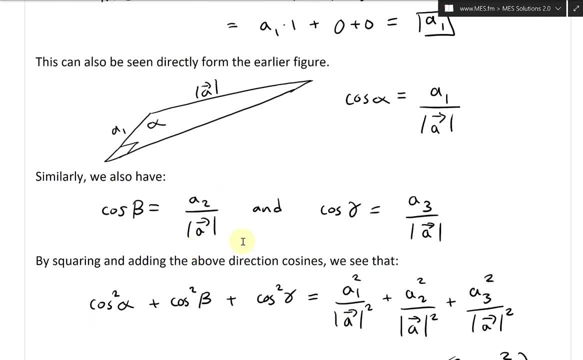 here it's just going to be a1 over uh. here it's just going to be a1 over uh the length. a the length. a the length. a or a2 over length. uh, a or a3 over length or a2 over length, uh, a or a3 over length. 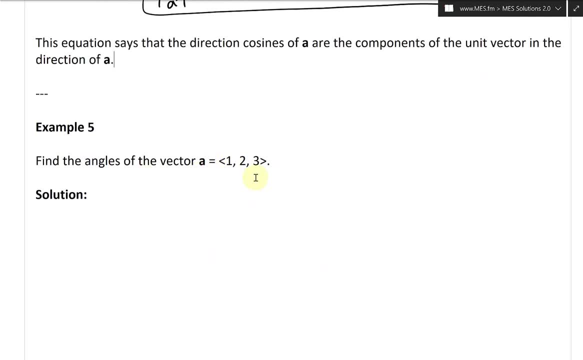 or a2 over length uh, a or a3 over length a. so find the angle. but we're never asked a. so find the angle. but we're never asked a. so find the angle, but we're never asked to find the angles of it. so to find the angles of it. so 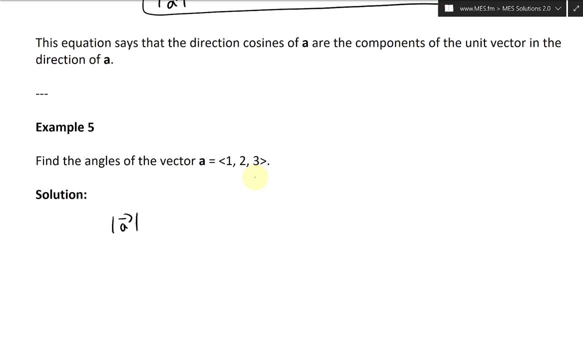 to find the angles of it. so first we're going to need the length, first we're going to need the length first. we're going to need the length first, first. first we're going to need the length. length a is going to equal to length a is going to equal to. 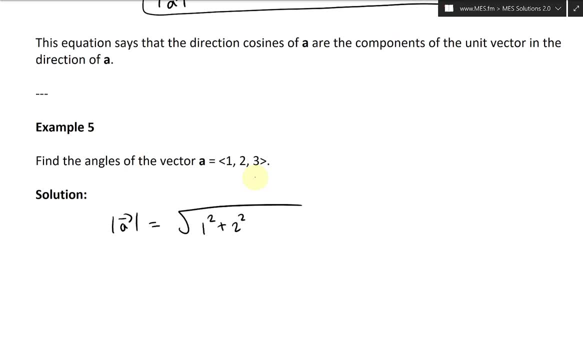 length a is going to equal to square root: uh one squared. all the square root, uh one squared, all the square root, uh one squared. all the components squared: components squared. components squared plus two squared plus three squared. this plus two squared plus three squared. this plus two squared plus three squared, this equals to: 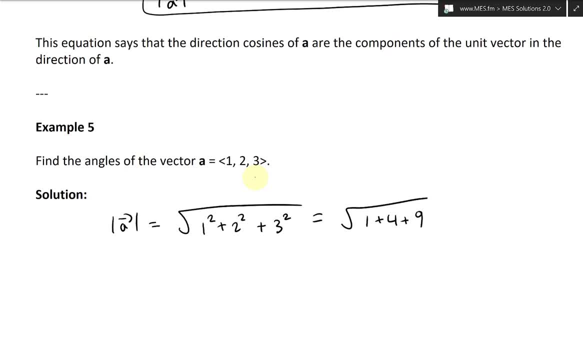 equals to: equals to one plus four plus one plus four plus one plus four plus nine. in other words: nine plus one is nine. in other words, nine plus one is nine. in other words, nine plus one is uh. or the nine plus one is ten plus four, uh. or the nine plus one is ten plus four. 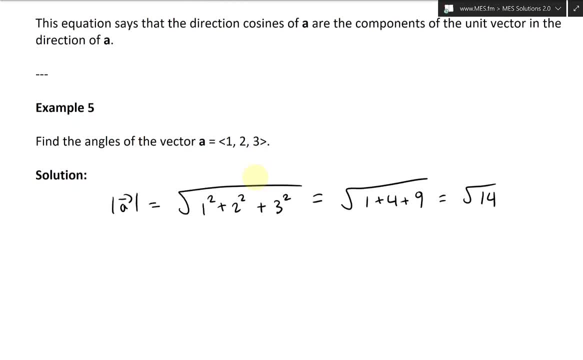 uh, or the nine plus one is ten plus four is fourteen, is fourteen, is fourteen, the square root of fourteen, the square root of fourteen, the square root of fourteen. thus, let's get all the direction. thus, let's get all the direction. thus, let's get all the direction, cosines first, and then we'll, yeah, and. 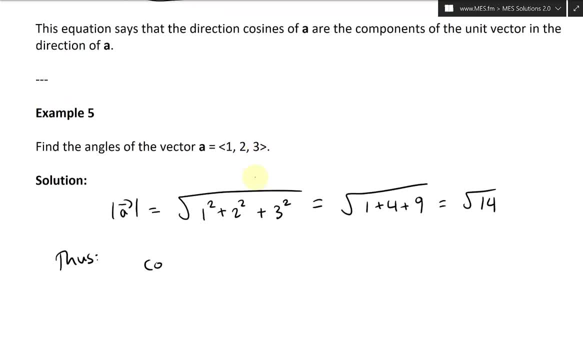 cosines first, and then we'll yeah, and cosines first, and then we'll yeah, and then we'll do the angles after. so let's, then we'll do the angles after. so let's, then we'll do the angles after. so let's get the cosines. 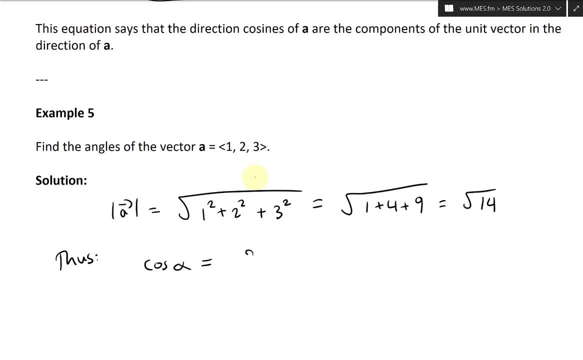 get the cosines, get the cosines. cosine uh. cosine alpha is equal to cosine uh. cosine alpha is equal to cosine uh. cosine alpha is equal to: again, that's just greek letter alpha a1. again, that's just greek letter alpha a1. again, that's just greek letter alpha a1 over the length. 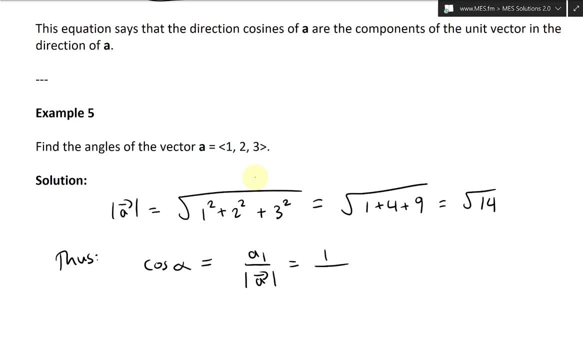 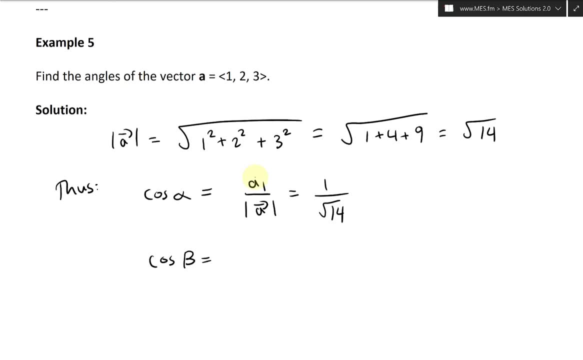 over the length, over the length. a like that, a like that, a like that. this equals to 1 over. this equals to 1 over. this equals to 1 over square root 14.. square root 14.. square root 14.. cosine beta. this equals to a 2. 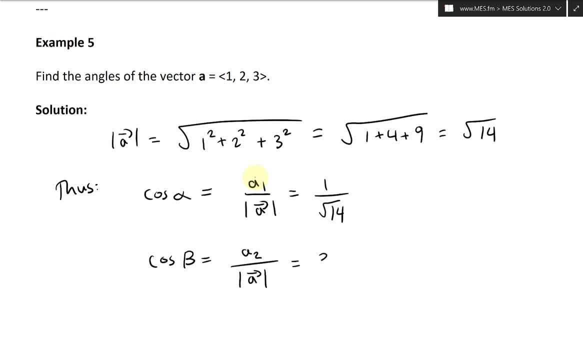 beta. this equals to a 2 beta. this equals to a 2 over the length a. this equals to over the length a. this equals to over the length a. this equals to 2 over 14.. 2 over 14.. 2 over 14.. because, again, that's components two, the 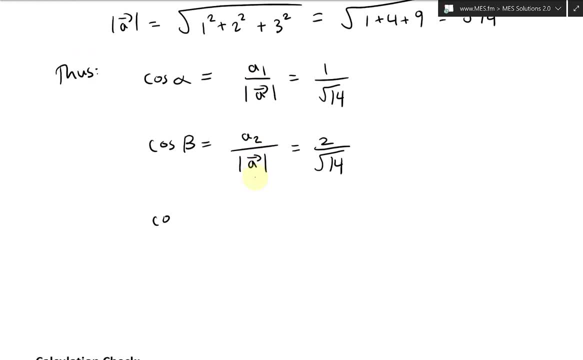 because, again, that's components two. the because, again, that's components two. the next one is going to be three, next one is going to be three, next one is going to be three. and then cosine, and then cosine, and then cosine, uh, cosine, uh, cosine, uh, cosine gamma. this equals to a 3 over. 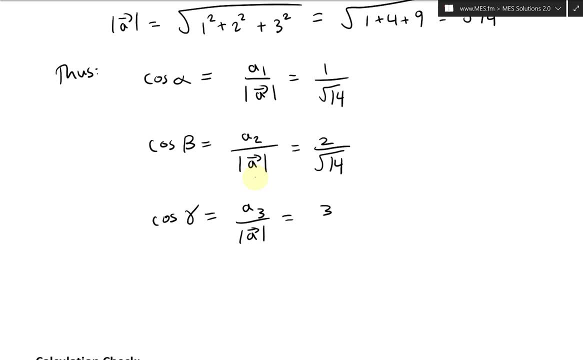 gamma. this equals to a 3 over gamma. this equals to a 3 over unit. in fact, i mean the length a unit. in fact, i mean the length a unit. in fact, i mean the length a equals to 3 over, equals to 3 over, equals to 3 over 14.. 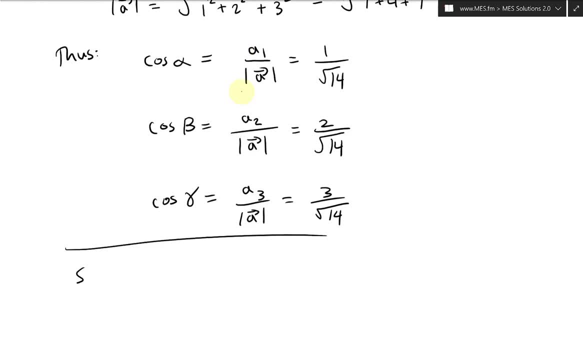 14. 14.. all right, so that's what we have here. so all right, so that's what we have here. so all right, so that's what we have here. so now, oh, instead of saying thus, let's now, oh, instead of saying thus, let's. 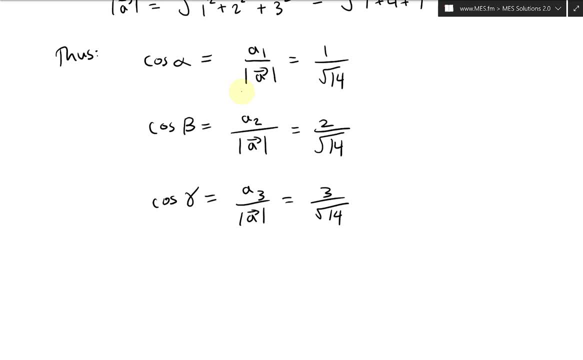 now, oh, instead of saying thus: let's write, so, write, so write. so we already had a thought, so i'll just. we already had a thought, so i'll just. we already had a thought, so i'll just say so, or say so, or say so or um, so we get. now we just take the. 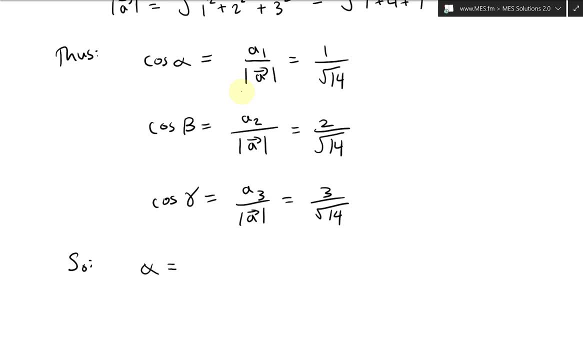 um. so we get. now we just take the um. so we get, now we just take the inverse. so inverse, so inverse. so uh alpha is equal to inverse cosine. uh alpha is equal to inverse cosine. uh alpha is equal to inverse cosine or arc cosine or a cosine 1 over 14. 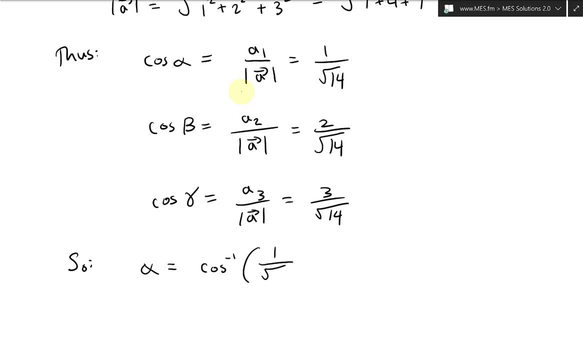 or arc cosine, or a cosine 1 over 14 or arc cosine 1 over 14, 1 over square root 14, and now if you plug this into the, and now if you plug this into the, and now if you plug this into the calculator, you should get around 74. 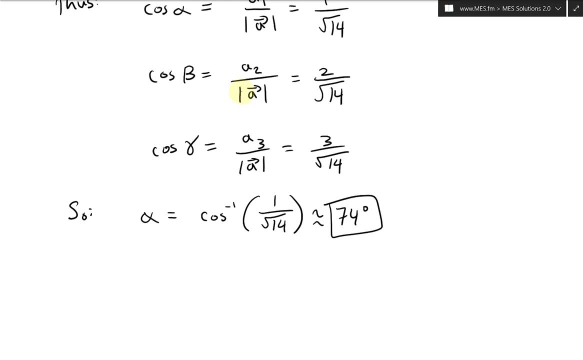 calculator, you should get around 74. calculator, you should get around 74 degrees, degrees, degrees. i'll box this out because that's what i'll box this out, because that's what i'll box this out, because that's what we're asked to. we're asked to: 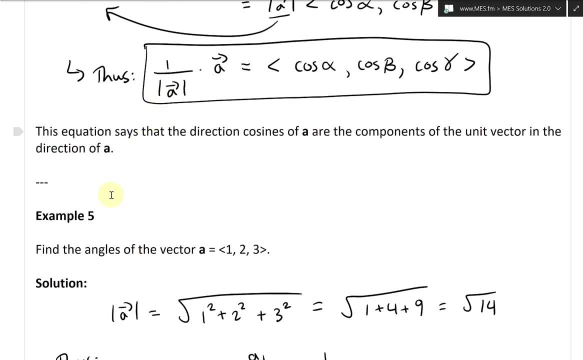 we're asked to find, find, find. we're asked to find all of the angles by. we're asked to find all of the angles by. we're asked to find all of the angles by the angles of this vector, the angles of this vector, the angles of this vector, so 74 degrees. and then the next one is: 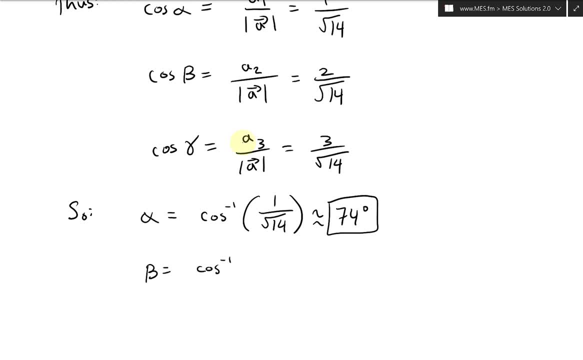 so 74 degrees, and then the next one is so 74 degrees, and then the next one is beta, beta, beta is equal to cosine inverse, is equal to cosine inverse is equal to cosine inverse. in the calculator, you get 58 degrees. in the calculator, you get 58 degrees. 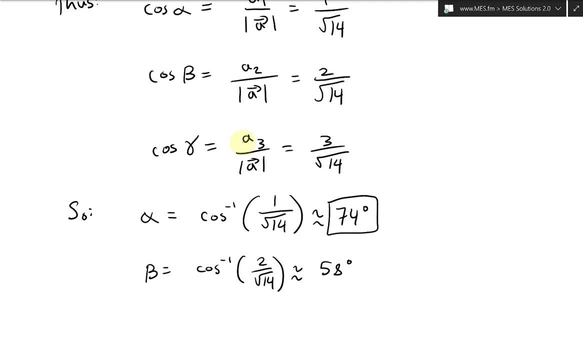 in the calculator you get 58 degrees. just quite, just, quite just, quite interesting. all right, that's 58, all right. the next one now is the um- all right. the next one now is the um- all right. the next one now is the um: gamma, gamma, gamma. this equals to cosine. 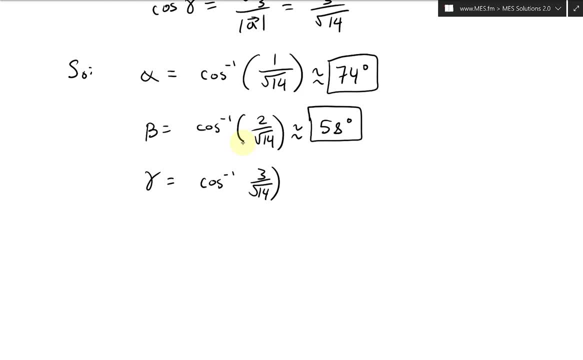 this equals to cosine. this equals to cosine: 3 over square root 14. 3 over square root 14, 3 over square root 14. let's write this bit neater. like this, like this: like this: this equals to plug in the. this equals to plug in the. 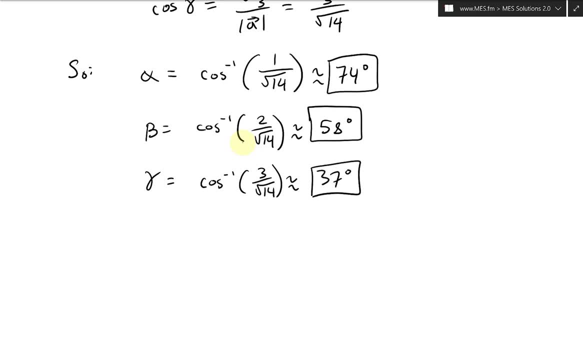 this equals to plug in the calculator, calculator, calculator 37 degrees like that, 37 degrees like that, 37 degrees like that. and uh, now we'll do a quick calculation. and uh, now we'll do a quick calculation. and uh, now we'll do a quick calculation. check as per usual, again this built-in. 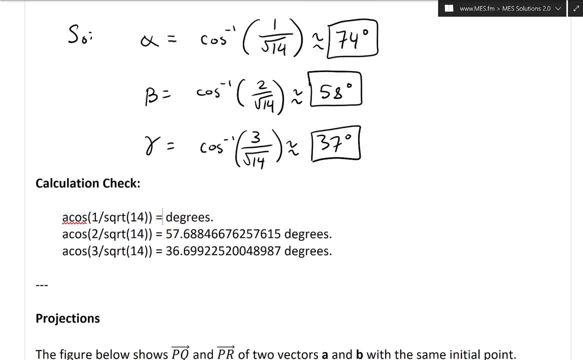 check as per usual, again this built-in. check as per usual, again this built-in. one note calculator. one note calculator. one note calculator. i'll put a, a cos or arc. i'll put a, a cos or arc. i'll put a, a cos or arc. cosine or inverse cosine: 1 divided by 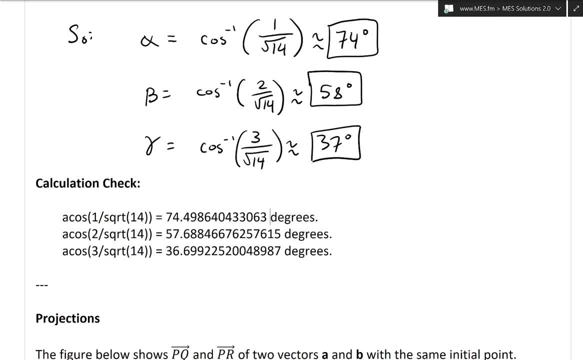 cosine or inverse cosine 1 divided by cosine or inverse cosine 1 divided by square root 14 or sqrt 14, and then square root 14 or sqrt 14, and then square root 14 or sqrt 14, and then press space. auto calculates which is. 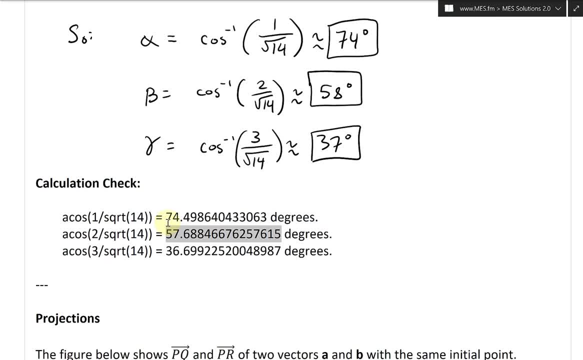 press space auto calculates which is press space auto calculates, which is quite fascinating: 74.49, etc. quite fascinating, 74.49, etc. quite fascinating, 74.49, etc. rounds down to 74.. rounds down to 74.. rounds down to 74.. the next one: 57.68. 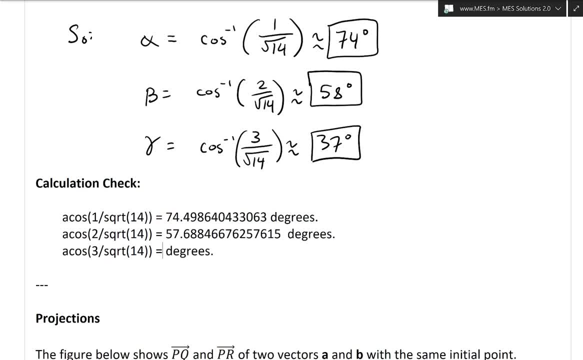 the next one: 57.68. the next one: 57.68. that's right. rounds up to 58. that's right, rounds up to 58. that's right, rounds up to 58. next one: 36 again. this is one, two, three. next one: 36 again. this is one, two, three. 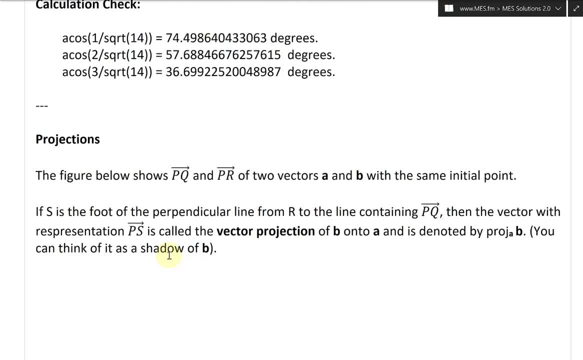 next one: 36 again. this is one, two, three, 36 rounds up to 37- yeah, 36.699, etc. 36 rounds up to 37- yeah, 36.699, etc. 36 rounds up to 37- yeah, 36.699, etc. that's quite fascinating. 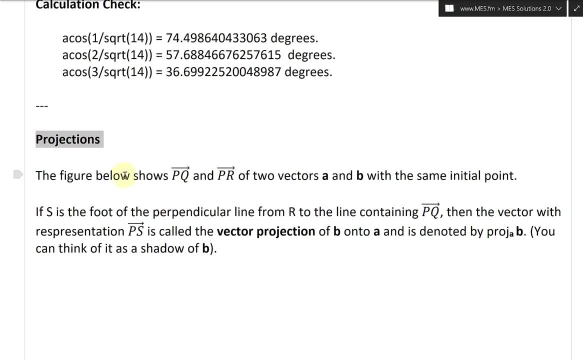 that's quite fascinating. that's quite fascinating. all right, so now let's take a look at. all right, so now let's take a look at. all right, so now let's take a look at projections. the next section, so the projections. the next section, so the projections. the next section. so the figure below shows pq and pr. 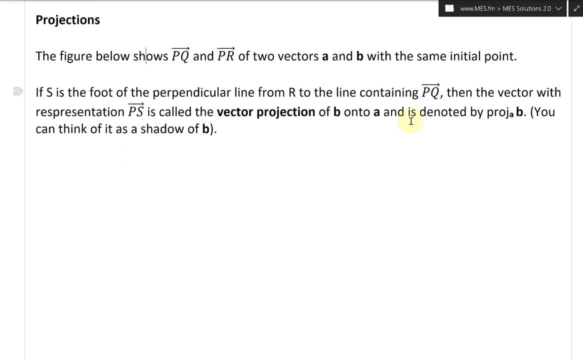 figure below shows pq and pr. figure below shows pq and pr of two vectors, a and b, with the same of two vectors a and b. with the same of two vectors a and b with the same initial, initial, initial point. so let's say we have here these. 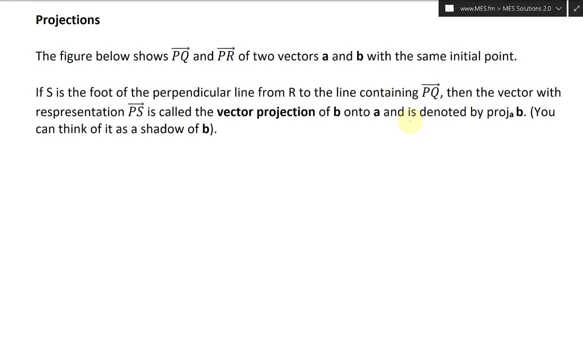 point. so let's say we have here these point. so let's say we have here these two uh, two, uh two uh line segments here. so we have the same line segments here. so we have the same line segments here. so we have the same starting points. let's say it's starting. 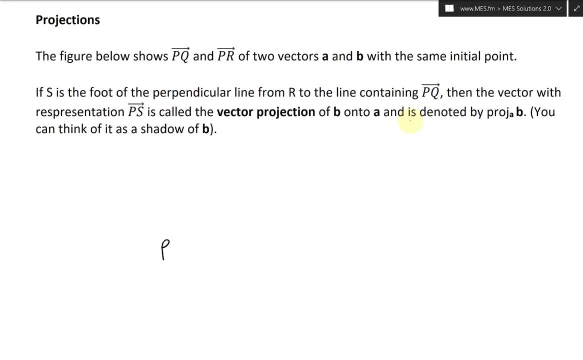 starting points. let's say it's starting starting points. let's say it's starting at p, at p, at p, and it goes over to you have pq, and it goes over to you have pq, and it goes over to you have pq. let's say it goes to pq, like this, this: 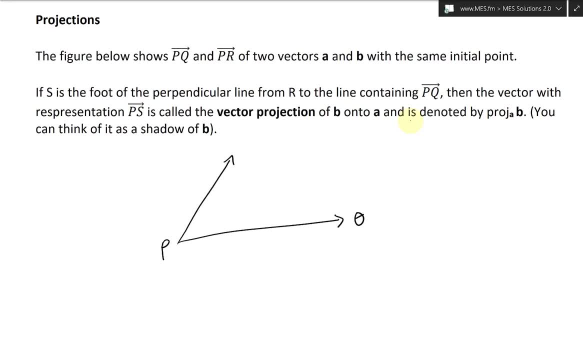 let's say it goes to pq like this. this: let's say it goes to pq like this: this is q is q is q. it has pr. goes to here like that. it has pr. goes to here like that. it has pr. goes to here like that, that's pr. this is a pq. 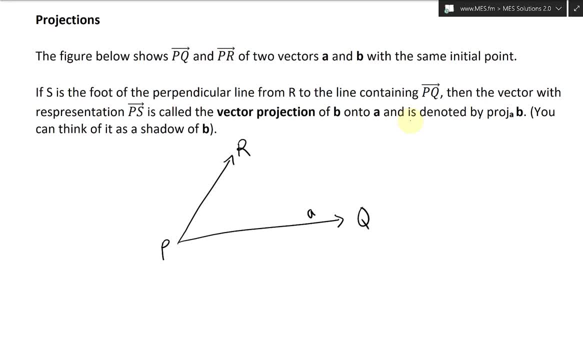 that's pr. this is a pq. that's pr. this is a pq. all right, yeah, just fix that up. and this all right. yeah, just fix that up. and this all right. yeah, just fix that up. and this is the vectors. a is the vectors. a is the vectors a and this is vector b. 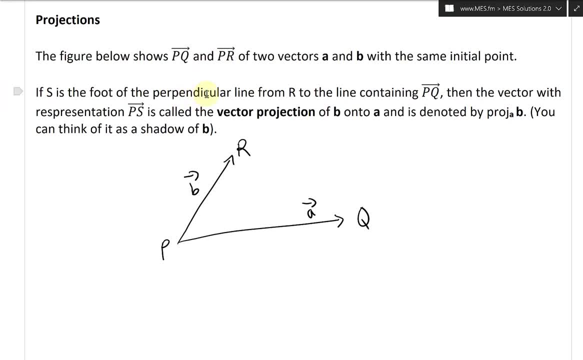 and this is vector b, and this is vector b, all right. so if s is the foot of the, all right, so if s is the foot of the all right, so if s is the foot of the perpendicular line from r to the line pq, so that would be all the. 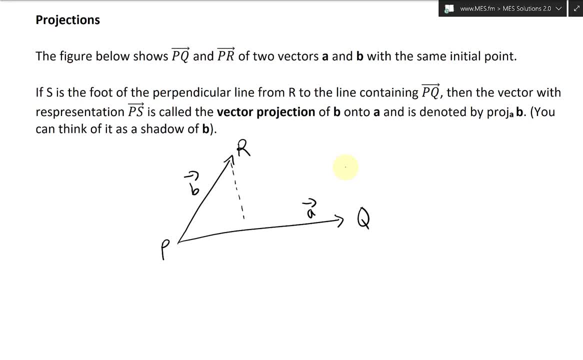 to the line pq, so that would be all the to the line pq, so that would be all the way here. and then you draw a way here, and then you draw a way here, and then you draw a perpendicular line, perpendicular line, perpendicular line, i guess that does. and then there is a 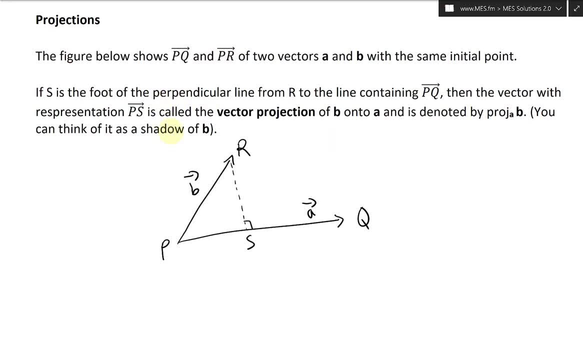 i guess that does. and then there is a- i guess that does. and then there is a perpendicular line, perpendicular line, perpendicular line, and that is s is the foot of it, then the, and that is s is the foot of it, then the, and that is s is the foot of it, then the vector with representation. 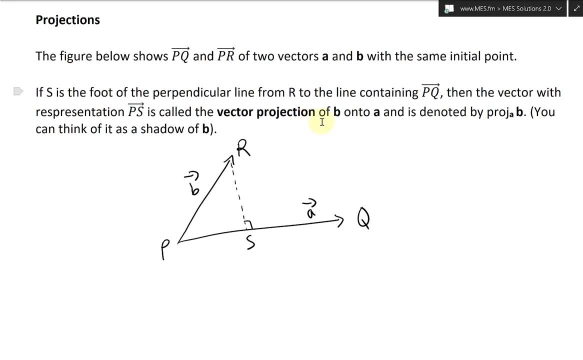 vector with representation. vector with representation- ps is called. the vector projection of ps is called. the vector projection of ps is called the vector projection of, of b, of b, of b. yeah on onto a and it's denoted by yeah on onto a and it's denoted by: 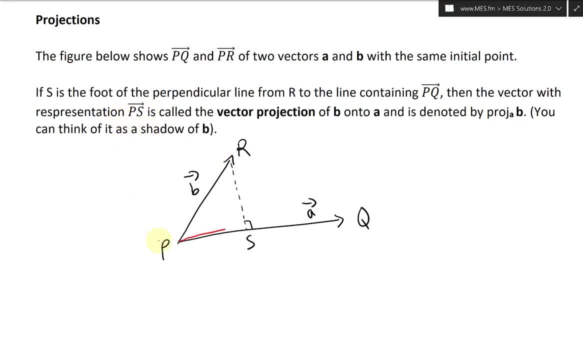 yeah, on onto a and it's denoted by: here's this: ps is so ps is vector. i'm here's this: ps is so ps is vector. i'm here's this: ps is so ps is vector. i'm going to draw this in red. going to draw this in red. 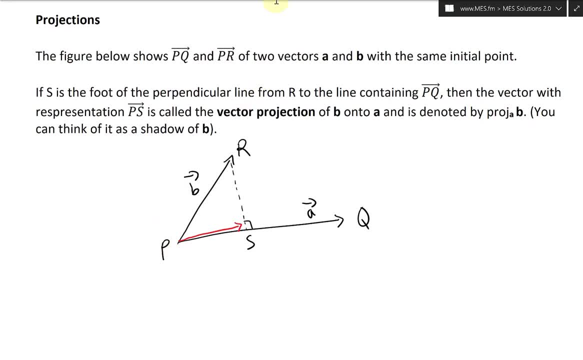 going to draw this in red, like that. so that is this a ps vector, like that. so that is this a ps vector, like that. so that is this a ps vector. and yeah, it's denoted by this and yeah, it's denoted by this and yeah, it's denoted by this projection. uh, subscript a, and and then. 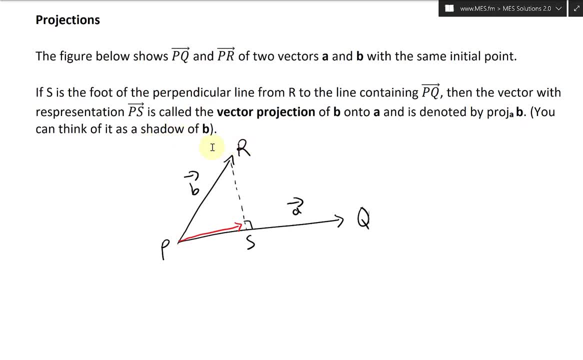 projection uh, subscript a and, and then projection uh, subscript a and, and then b vector and you can think of it as a b vector and you can think of it as a b vector and you can think of it as a shadow of b, so shadow of it onto. 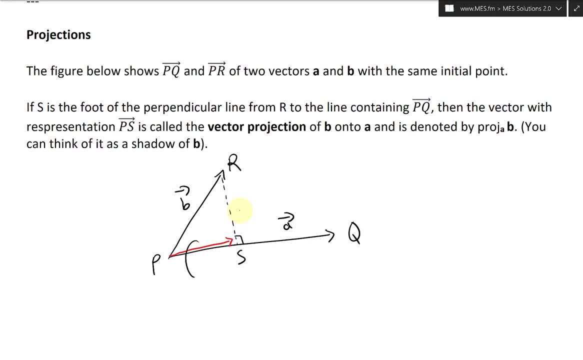 shadow of b. so shadow of it onto shadow of b. so shadow of it onto this setup right here and uh, this arrow, this setup right here and uh, this arrow, this setup right here and uh this arrow right here. uh, this is projection. right here, uh, this is projection. 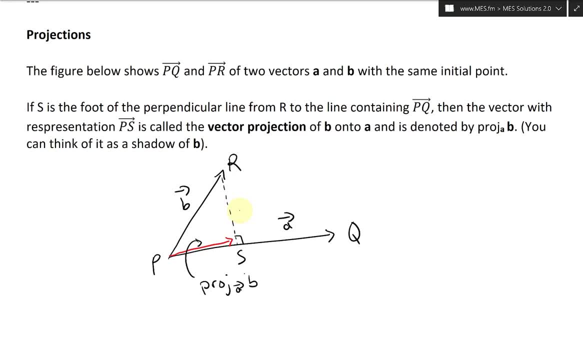 right here. uh, this is projection of a and so it's bold, but it's a bit of a, and so it's bold, but it's a bit of a and so it's bold, but it's a bit smaller than put the ap on top like that. 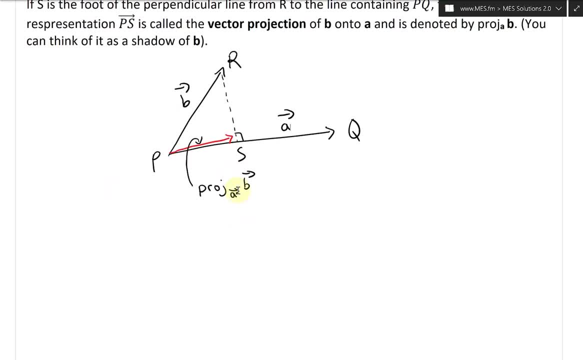 smaller than put the ap on top like that. smaller than put the ap on top, like that. you know, right here, i just uh fixed that. you know right here, i just uh fixed that. you know, right here, i just uh fixed that up and uh, this is a, this is an angle. 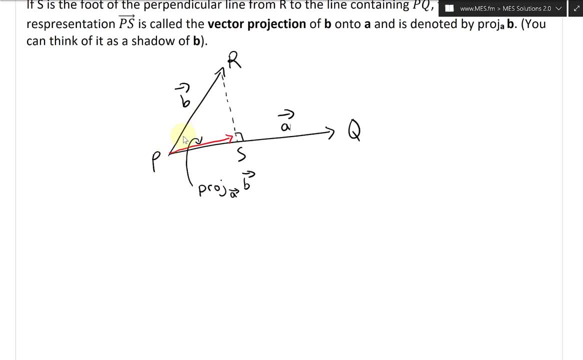 up and uh, this is a, this is an angle. up and uh, this is a, this is an angle that is uh, that is uh, that is uh. uh, that's less than 90 degrees. let's, that's less than 90 degrees. let's, that's less than 90 degrees. let's draw one that's more. so what happens is: 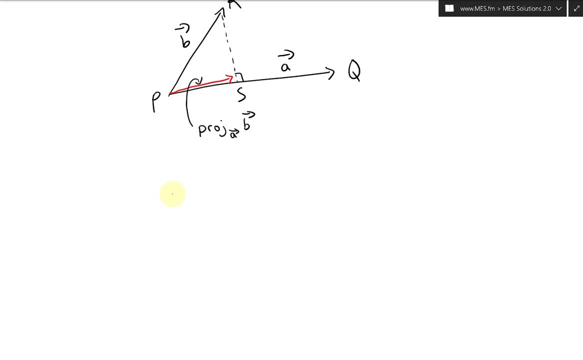 draw one that's more so. what happens is: draw one that's more so. what happens is: if you had one like this, let's say: if you had one like this, let's say: if you had one like this, let's say: same starting point: you go from p. 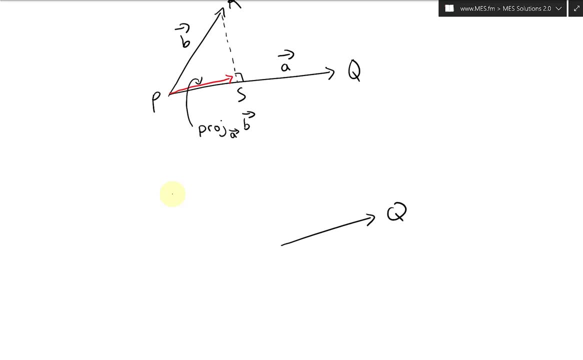 same starting point. you go from p. same starting point. you go from p over here. let's say that's q over here. let's say that's q over here. let's say that's q. so this is p. now you have a vector. so this is p. now you have a vector. 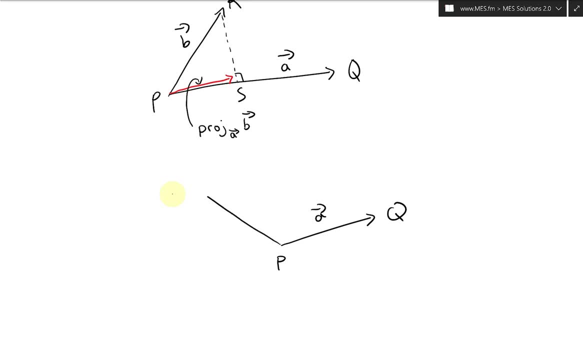 so this is p. now you have a vector a, and then you have the vector b like a, and then you have the vector b like a, and then you have the vector b like this, and then i'm going to r this is, and then i'm going to r this is. 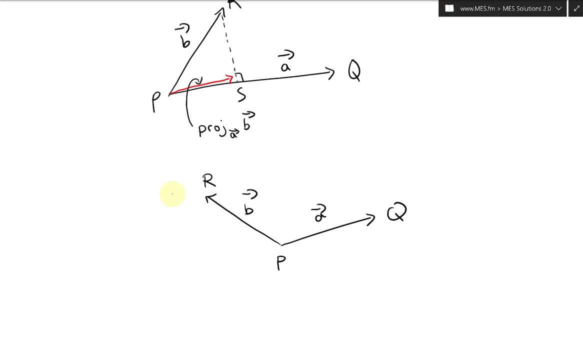 and then i'm going to r: this is b like that, and then going across b like that, and then going across b like that, and then going across. this way is going to be our s set up. this way is going to be our s set up. this way is going to be our s set up here. 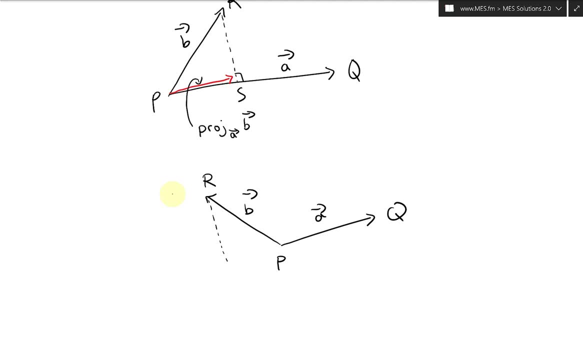 here, here, and this is the yeah. this projection, and this is the yeah. this projection, and this is the yeah. this projection goes all the way down here, goes all the way down here, goes all the way down here, and it's 90 degrees and it's 90 degrees. 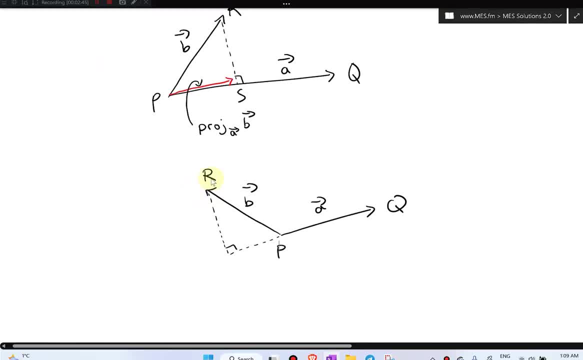 and it's 90 degrees like that, like that, like that, yeah, so that's going, uh, yeah, the shadow: yeah, so that's going, uh, yeah, the shadow, yeah, so that's going. uh, yeah, the shadow of it goes down or the projection goes of it goes down or the projection goes. 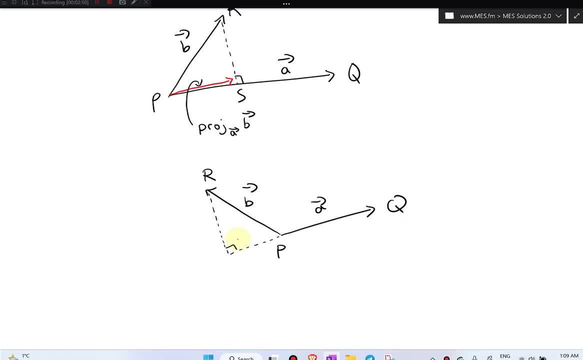 of it goes down, or the projection goes down here, so it's perpendicular, and then down here, so it's perpendicular, and then down here, so it's perpendicular, and then we'll have it going backwards. now this, we'll have it going backwards. now this, we'll have it going backwards. now this uh s set up there and uh, this would be. 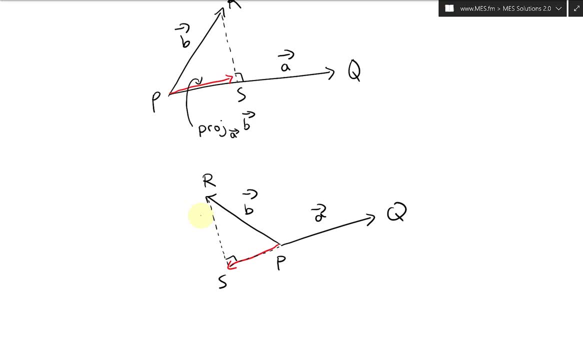 uh s set up there and uh, this would be uh s set up there. and uh, this would be the s, the s, the s. here and here i'll write s. and then this: here and here i'll write s. and then this: here and here i'll write s. and then this, right here is our 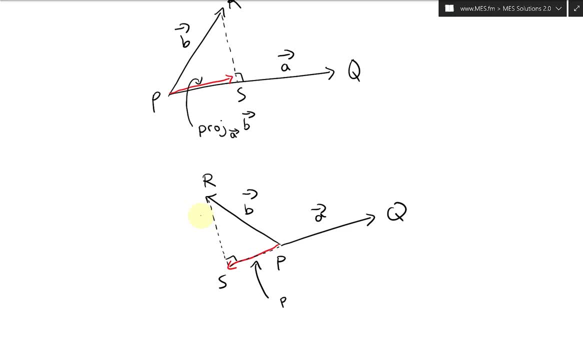 right. here is our right here is our. uh projection: the same same set up there. uh projection: the same same set up there. uh projection: the same same set up there, but different angle, but different angle, but different angle projection. try this, uh nicer projection. try this, uh nicer. 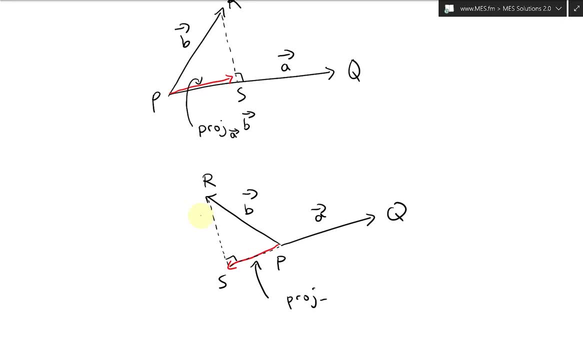 projection. try this: uh, nicer, a bit hard writing it a bit hard, writing it a bit hard. writing it: uh, subscript a and then b subscript. uh, subscript a and then b subscript. uh, subscript a and then b subscript. now i mean air on top, uh. so. now i mean air on top, uh, so. now i mean air on top. uh, so subscript a with air on top, and then b subscript a with air on top, and then b subscript a with air on top and then b air on top, and so on. so yes, air on top, and so on. so yes, 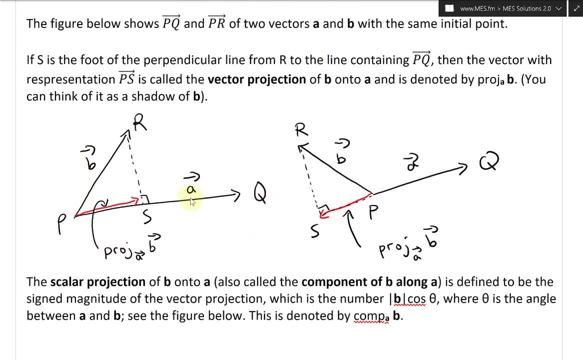 air on top and so on. so, yes, fascinating stuff, all right here. i just fascinating stuff, all right here. i just fascinating stuff all right here. i just moved it over to this uh side by side. so moved it over to this uh side by side. so moved it over to this uh side by side. so a bit neater, all right. so let's go. 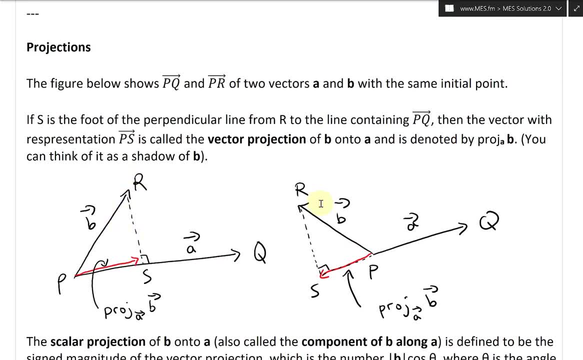 a bit neater, all right. so let's go a bit neater, all right. so let's go further. now, the scalar projections. further now the scalar projections. further now the scalar projections. this is a vector projection. we're this is a vector projection. we're this is a vector projection. we're projecting, projecting the vector onto. 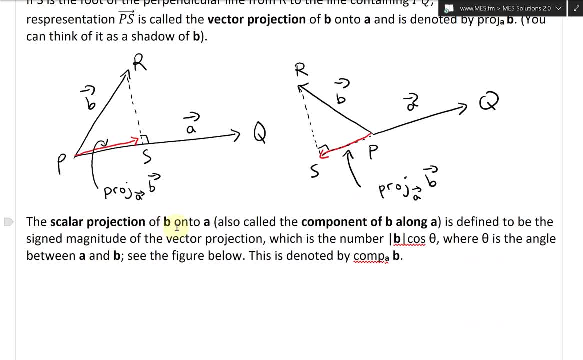 projecting, projecting the vector onto projecting, projecting the vector onto here, and we have this projection there here and we have this projection there here and we have this projection there, like that. so the scalar projection of b, like that. so the scalar projection of b, like that. so the scalar projection of b onto a, also called the component of b. 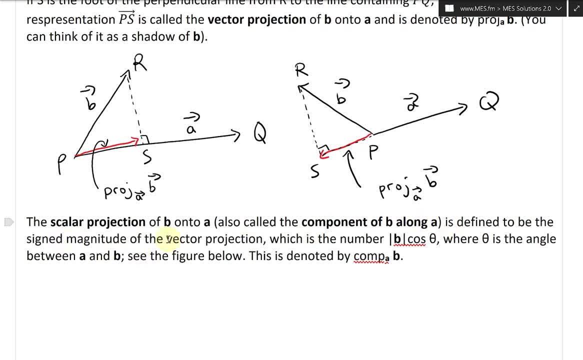 onto a, also called the component of b onto a, also called the component of b along. a is defined to be the signed along. a is defined to be the signed along. a is defined to be the signed. magnitude of the vector projection. so, magnitude of the vector projection, so 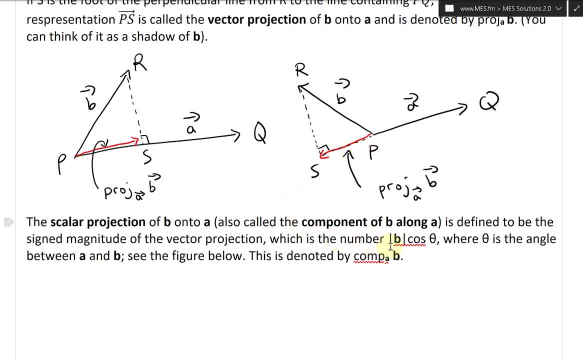 magnitude of the vector projection. so, the actual magnitude of it, the actual magnitude of it, the actual magnitude of it, which is the number, yeah, the number which which is the number, yeah, the number which which is the number, yeah, the number which is the length b is the length b. 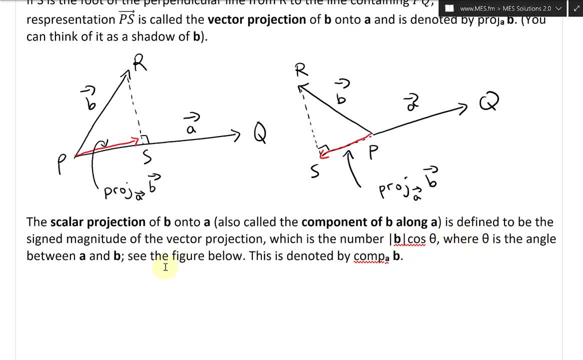 is the length b cosine theta. where theta is the angle cosine theta. where theta is the angle cosine theta. where theta is the angle between a and b. and see the figure below between a and b. and see the figure below between a and b. and see the figure below, and this is denoted by yeah, donated by: 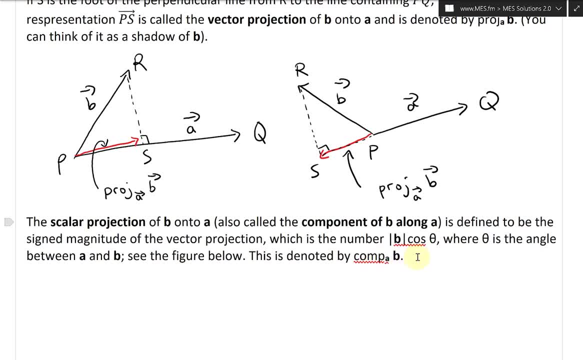 and this is denoted by yeah donated by, and this is denoted by yeah donated by this comb or component, and then this comb or component, and then this comb or component, and then subscript a vector, subscript a vector, subscript a vector, and then a b vector, like that. so let's. 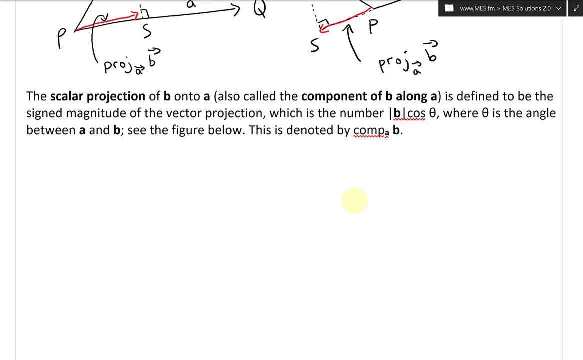 and then a b vector like that, so let's. and then a b vector like that, so let's draw. let's draw this out, and so if you have again similar to the and, so if you have again similar to the and, so if you have again similar to the above one, so you have the p. 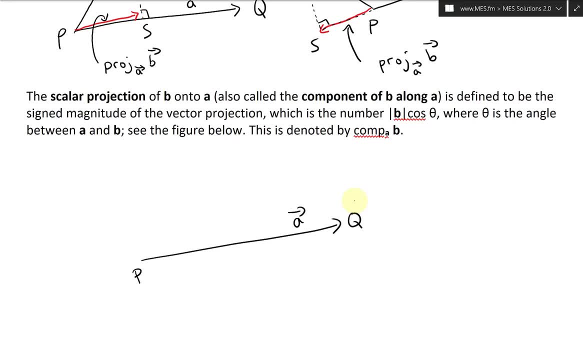 above one. so you have the p above one. so you have the p and it goes to q. this is our a vector. and it goes to q. this is our a vector. and it goes to q. this is our a vector. now you have the r like that. 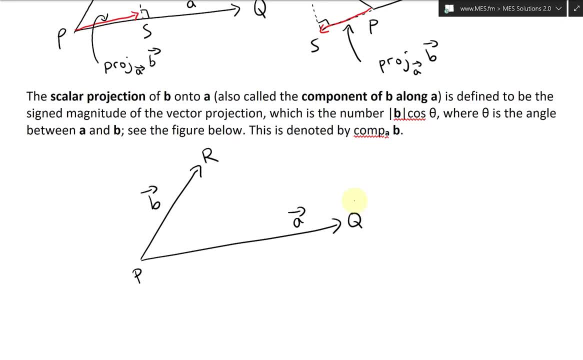 now you have the r like that. now you have the r like that. this is the r, this is the b, this is the r. this is the b, this is the r, this is the b like that, and this goes all the way like that and this goes all the way. 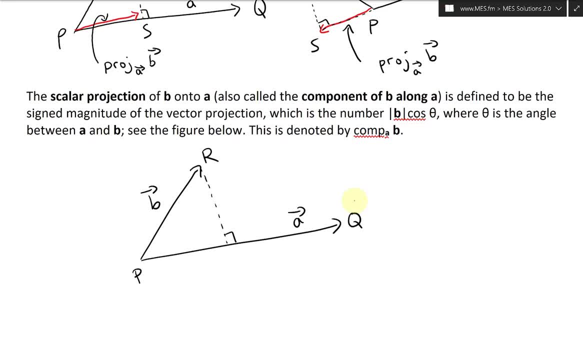 like that and this goes all the way across, like this, across, like this, across, like this, and this is our right angle, this is our and this is our right angle, this is our and this is our right angle. this is our s s, and now, uh, the the magnitude of this, uh, 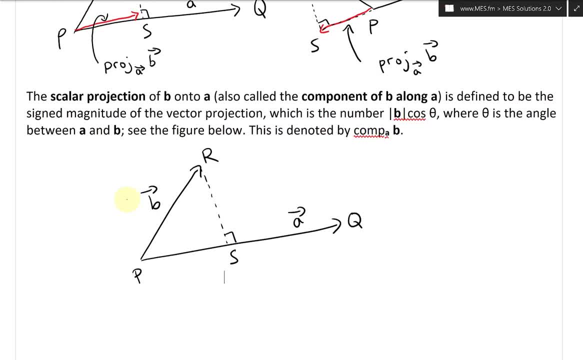 and now, uh, the the magnitude of this, uh, and now, uh, the the magnitude of this, uh. vector projection, vector projection, vector projection is going to be well. this is an angle is going to be well. this is an angle is going to be well. this is an angle, theta. 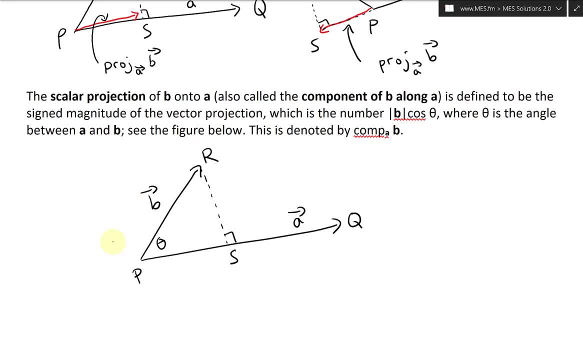 theta, theta. so this right here and this right here, so this right here and this right here. so this right here and this right here. i'm going to draw this in, i'm going to draw this in, i'm going to draw this in red. so this right here, is the magnitude. 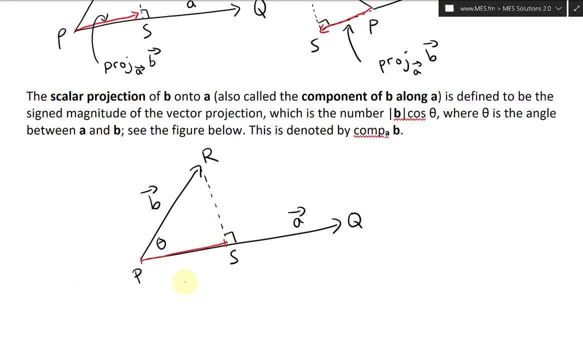 red. so this right here is the magnitude red. so this right here is the magnitude of it and it's a signed magnet. so it of it and it's a signed magnet, so it of it, and it's a signed magnet, so it could be negative or positive, and so on. 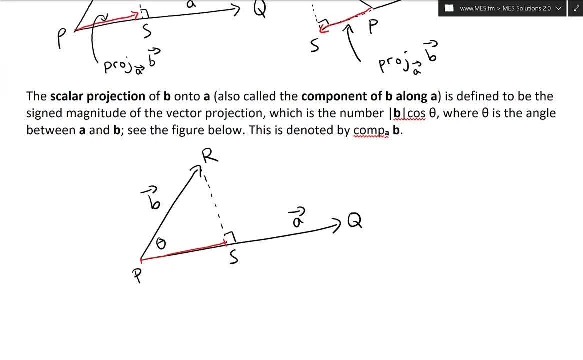 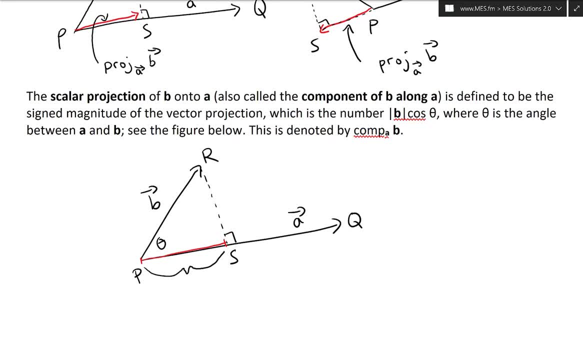 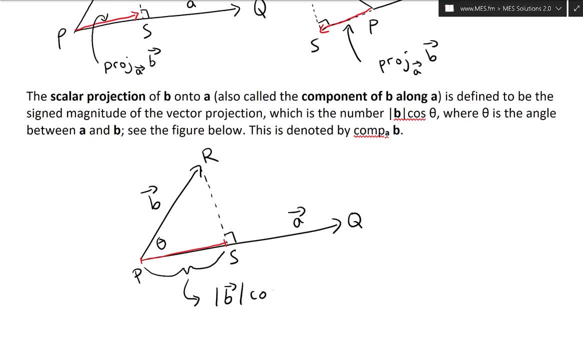 so that's the hypotenuse and there's. so that's the hypotenuse and there's. this is going to be cosine again, like this is going to be cosine again, like this is going to be cosine again, like always, always, always, cosine, theta, cosine, theta. 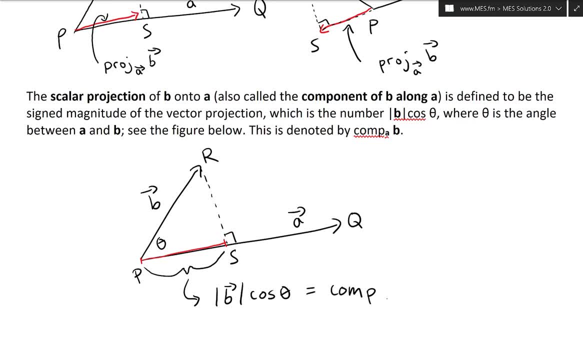 cosine theta. and you can write this as comp is. and you can write this as comp is. and you can write this as comp is denoted by comp. and you can write this as comp is denoted by comp. subscript a of the vector b. so subscript a of the vector b, so. 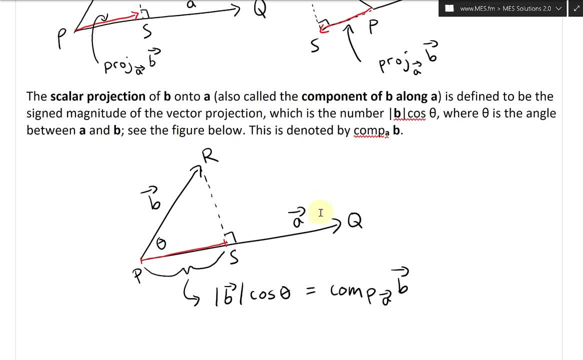 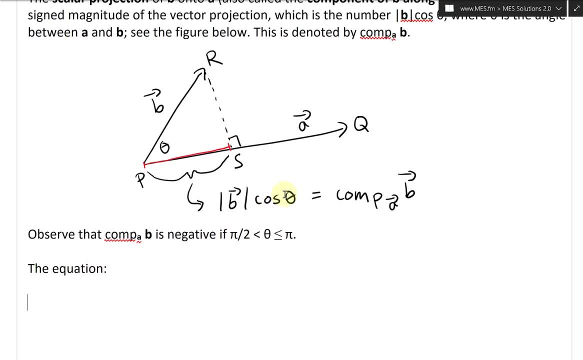 subscript a of the vector b. so the component of b along a, yes, fascinating the component of b along a, yes, fascinating the component of b along a, yes, fascinating stuff, stuff, stuff, yes. and since this is the signed yes, and since this is the signed yes, and since this is the signed magnitude, because notice the cosine theta- 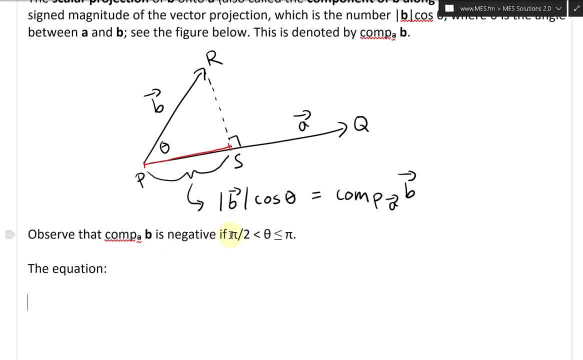 magnitude because notice the cosine theta. magnitude because notice the cosine theta, so observe that the component a b is so. observe that the component a b is so. observe that the component a b is negative. if this angle right here, theta negative. if this angle right here, theta negative. if this angle right here, theta is between pi over two and, uh, pi, so 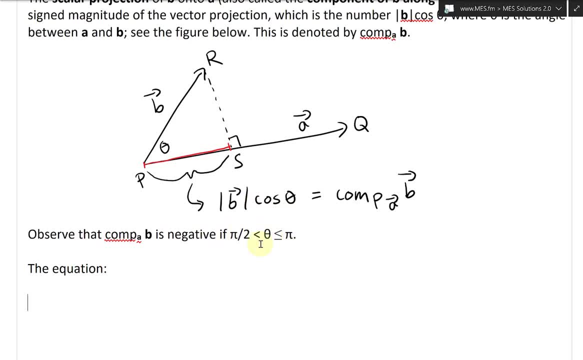 is between pi over two and uh pi. so is between pi over two and uh pi. so it's greater than power two. it's gonna be. it's greater than power two. it's gonna be. it's greater than power two. it's gonna be negative, negative, negative. uh yeah, so it's gonna be negative there. uh, yeah, so it's gonna be negative there. uh, yeah, so it's gonna be negative there, and then, and if it equals to pi, it's, and then. and if it equals to pi, it's, and then. and if it equals to pi, it's gonna be negative one there. so, yes, it's. 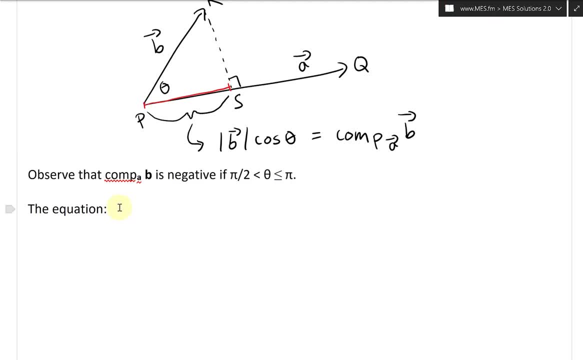 gonna be negative one there. so yes, it's gonna be negative one there. so yes, it's gonna be negative, gonna be negative, gonna be negative. uh angle there, so it's interesting, and uh angle there, so it's interesting, and uh angle there, so it's interesting. and now 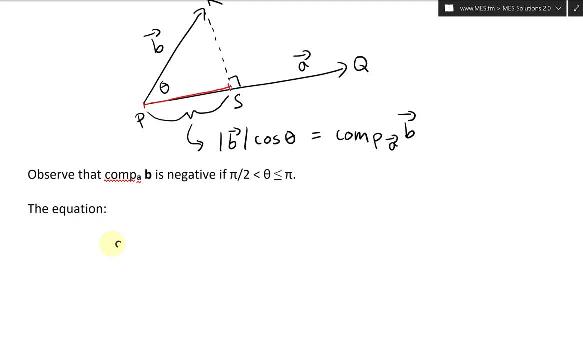 now, now note that the equation. so if we write note that the equation. so if we write note that the equation, so if we write this out, this out, this out, uh, the dot product a, dot b. uh, this equals to all the lengths a. uh, this equals to all the lengths a. 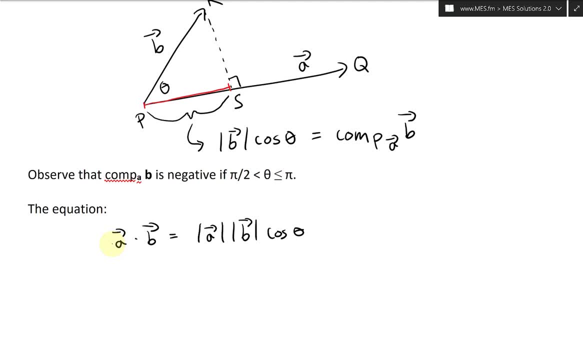 uh. this equals to all the lengths a times by the length b of cosine times by the length b of cosine times by the length b of cosine theta and uh. we know that. the component uh of and uh. we know that the component uh of and uh. we know that the component uh of uh. 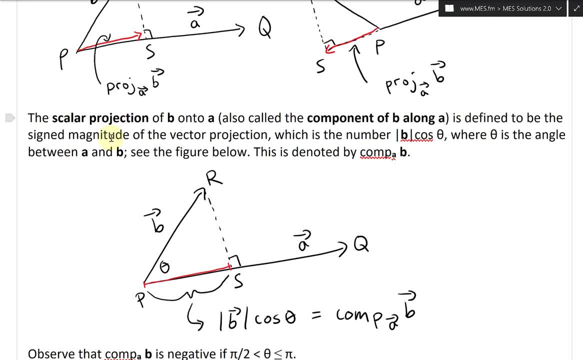 uh uh of b on along a or component of b along a. of b on along a or component of b along a. of b on along a or component of b along a, or the scalar projection of b onto a. or the scalar projection of b onto a. 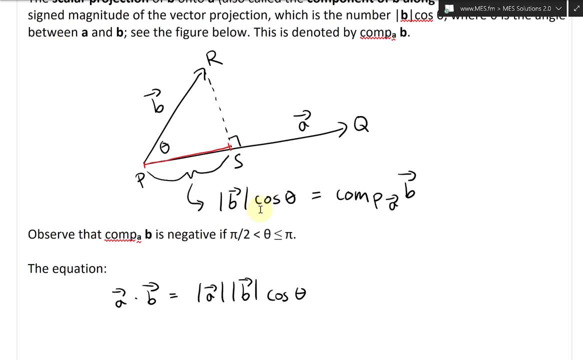 or the scalar projection of b onto a. is just this: b length b times um. is just this b length b times um. is just this b length b times um cosine theta. in other words, we could cosine theta in other words. we could cosine theta. in other words, we could write this as: 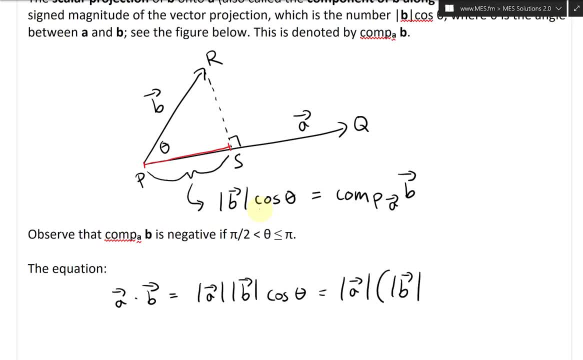 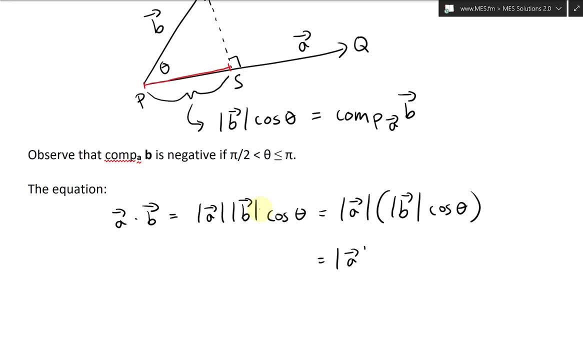 write this as, write this as in a bracket. so this is the component in a bracket, so this is the component in a bracket, so this is the component like this, like this, like this. in other words, this equals to. in other words, this equals to. in other words, this equals to, uh, the length of a times it by. 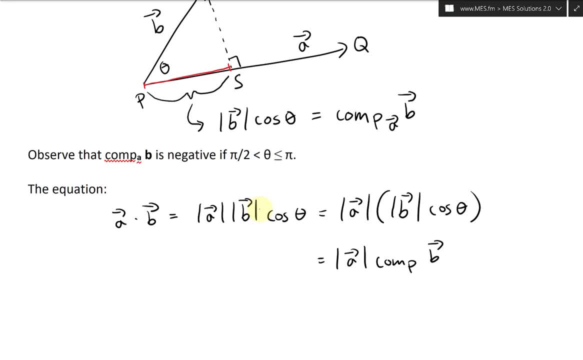 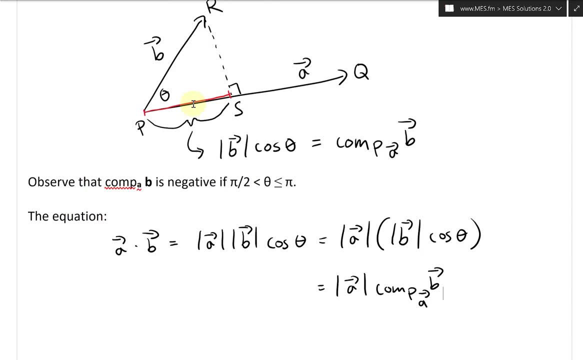 uh, the length of a times it by. uh, the length of a times it by the component, the component, the component of b along a, of the scalar projection of b along a, of the scalar projection of b along a, of the scalar projection of b onto a or of, you have, beyond a. 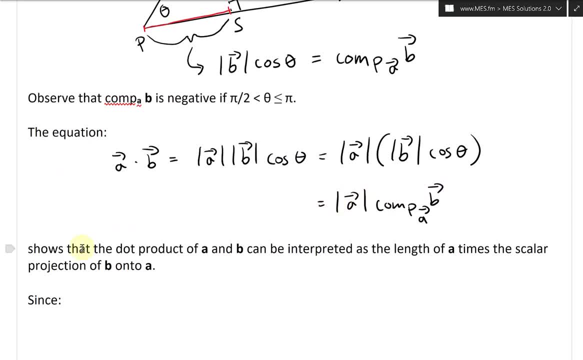 of b onto a, or of you have beyond a, of b onto a, or of you have beyond a. that's fascinating stuff. yeah. so this, that's fascinating stuff. yeah, so this, that's fascinating stuff. yeah. so this equation right here, uh shows that the equation right here, uh shows that the 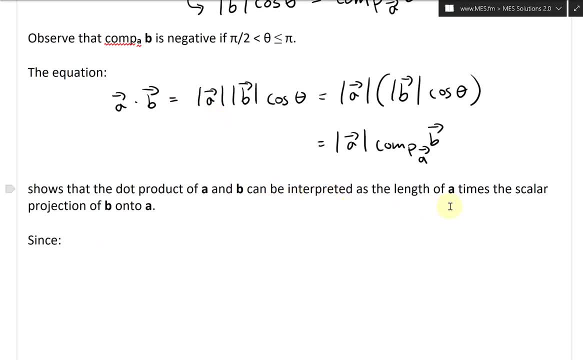 equation right here, uh, shows that the dot, dot, dot product of a and b can be interpreted as product of a and b can be interpreted as product of a and b. can be interpreted as: the length of a, the length of a, the length of a times the scalar projection of b. 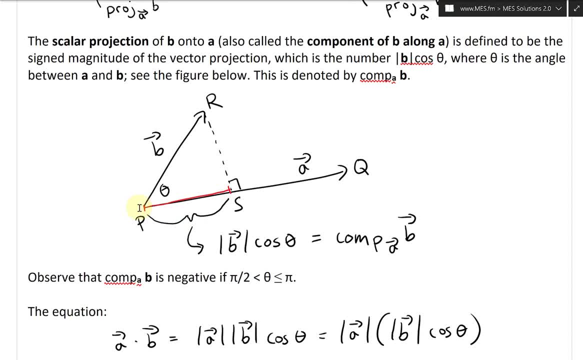 times the scalar projection of b times the scalar projection of b onto a, which is quite interesting. so if onto a, which is quite interesting, so if onto a, which is quite interesting. so if you look at it here, this could be viewed. you look at it here, this could be viewed. 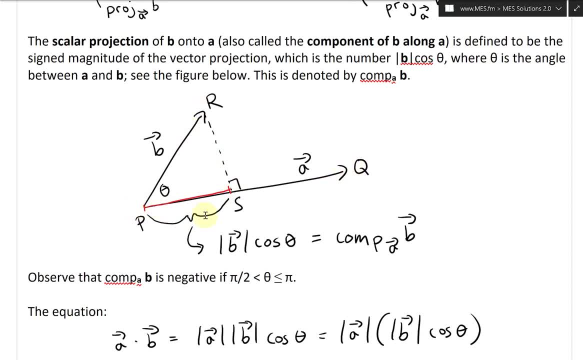 you look at it here, this could be viewed as the length of a, as the length of a as the length of a times it by the projection of b onto a times it by the projection of b onto a times it by the projection of b onto a, such as: uh. so you're multiplying at the. 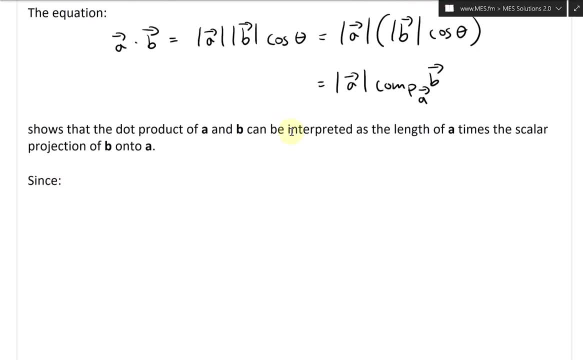 such as uh, so you're multiplying at the such as uh, so you're multiplying at the amount that's actually uh. the shadow is amount. that's actually uh. the shadow is amount. that's actually uh. the shadow is actually hitting here, actually hitting here, actually hitting here, perpendicular, so, which is quite 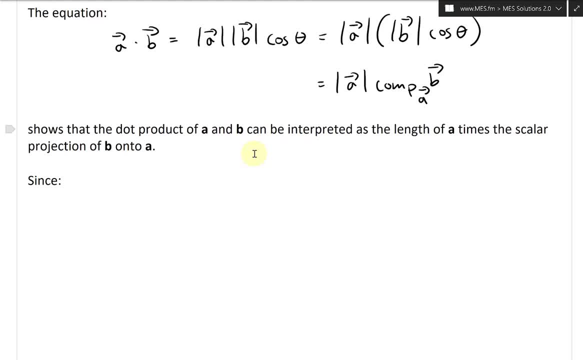 perpendicular, so which is quite perpendicular, so which is quite interesting, interesting, interesting, all right. so now going further, since all right, so now going further, since all right, so now going further, since, so, since we have, so, since we have, so since we have, uh, this right here, the length of b. 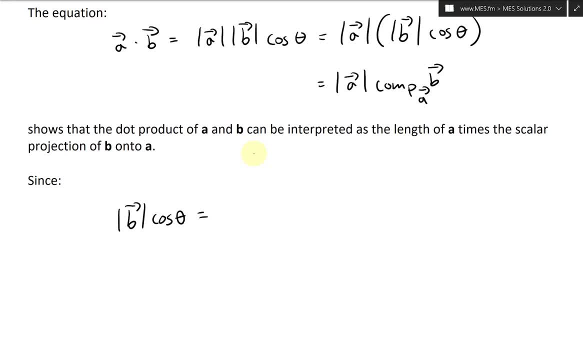 uh, this, right here, the length of b, uh, this, right here, the length of b. cosine, theta, cosine, theta, cosine, theta is equal to uh, is equal to uh, is equal to uh. and here what i've done here is, and here, what i've done here is, and here, what i've done here is is just move this over to this side. 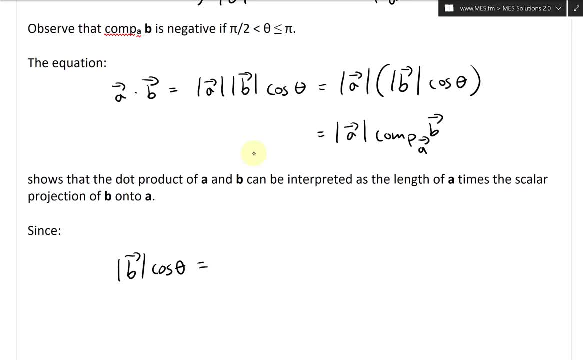 is just move this over to this side, is just move this over to this side, and uh. so all we're left with is the and uh. so all we're left with is the and uh. so all we're left with is the component of uh. b onto a. 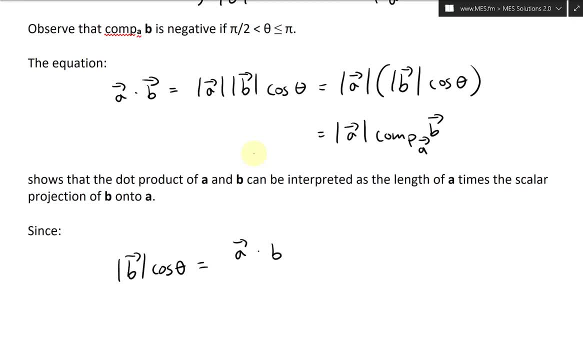 component of uh b onto a. component of uh b onto a. so what we get is this dot product. so what we get is this dot product. so what we get is this dot product: a a dot b over a. a dot b over a. a dot b over uh. the length a. 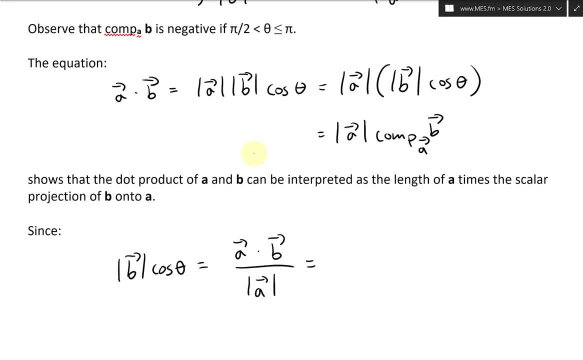 uh the length, a. uh the length, a like that, like that, like that. and then in a unit vector form, just, and then in a unit vector form, just, and then in a unit vector form, just. write these together, write these together, write these together. this can be a over. 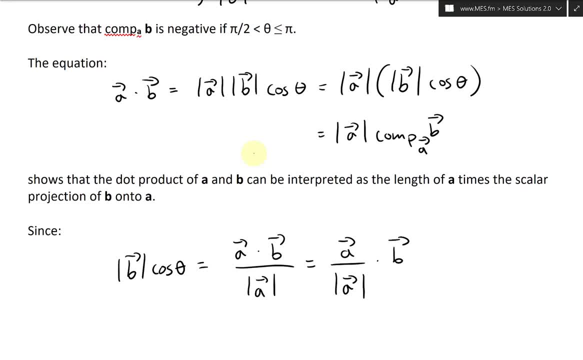 this can be a over. this can be a over length, a length, a length, a dot, dot, dot, b like that b. like that, b like that. so the component or the: yeah, the. so the component or the. yeah, the. so the component or the. yeah, the component of b. 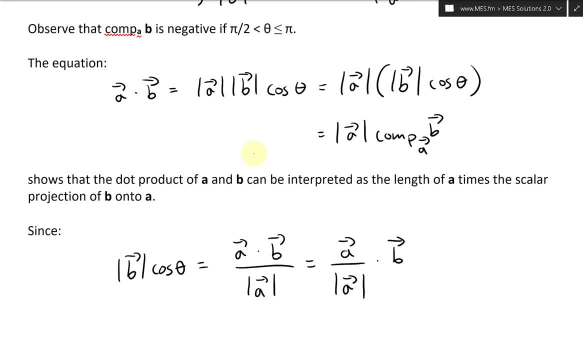 component of b. component of b, or the scalar projection of b onto a, or the scalar projection of b onto a or the scalar projection of b onto a is going to be the unit vector of a dot. is going to be the unit vector of a dot. is going to be the unit vector of a dot product. 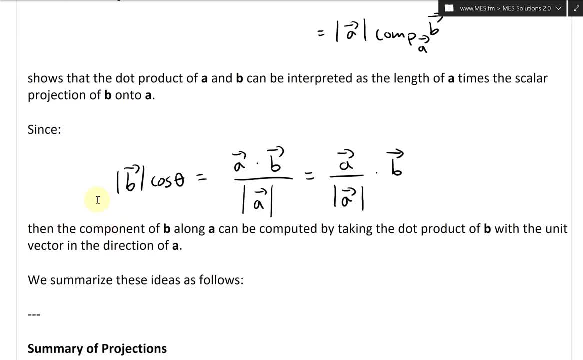 product. product with b. it's quite interesting. yeah, so with b it's quite interesting. yeah, so with b it's quite interesting. yeah, so here i've written it down. so since we here, i've written it down. so since we here i've written it down. so since we have this, uh then the component of 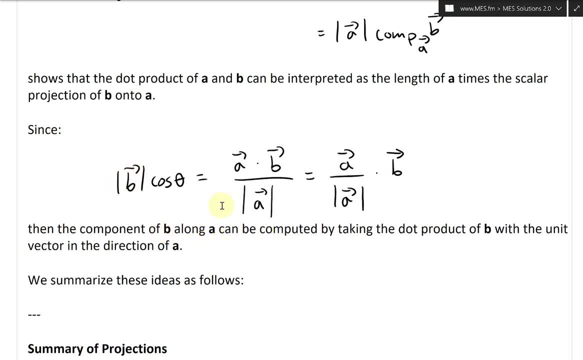 have this, uh, then the component of. have this: uh, then the component of b along a. yes, the component b along a, b along a. yes, the component b along a, b along a. yes, the component b along a can be computed by taking the dot. can be computed by taking the dot. 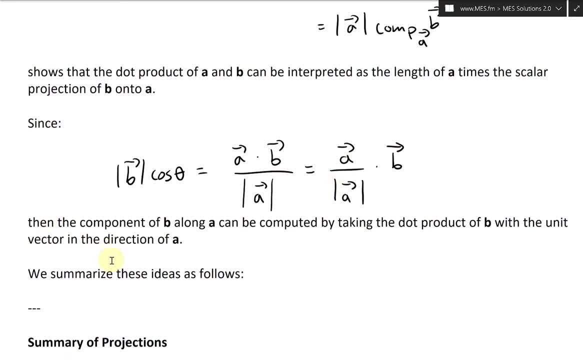 can be computed by taking the dot: number that's the length of one, because number that's the length of one, because number that's the length of one, because you're dividing by the full length. there, you're dividing by the full length, there, you're dividing by the full length there. so we summarize, summarize these ideas as: 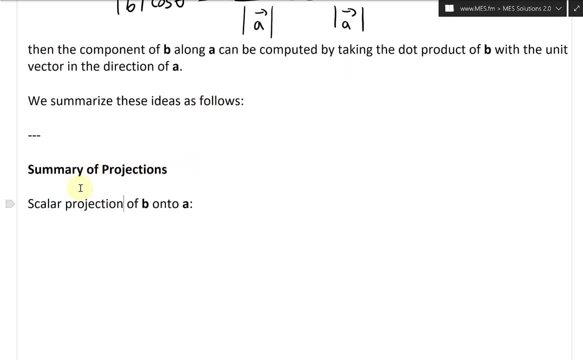 so we summarize, summarize these ideas as. so we summarize, summarize these ideas as follows: so summary of projections. all follows, so summary of projections, all follows. so summary of projections, all right. so the first one is right. so the first one is right. so the first one is scalar projection of b onto a. that's just. 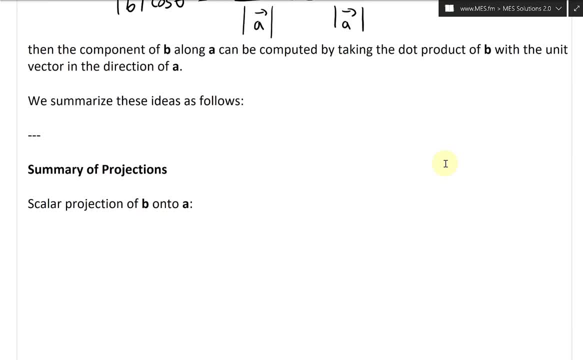 scalar projection of b onto a. that's just scalar projection of b onto a. that's just this comp setup over here, this comp setup over here, this comp setup over here. in other words, uh, comp, i'll write this. in other words, uh, comp, i'll write this. 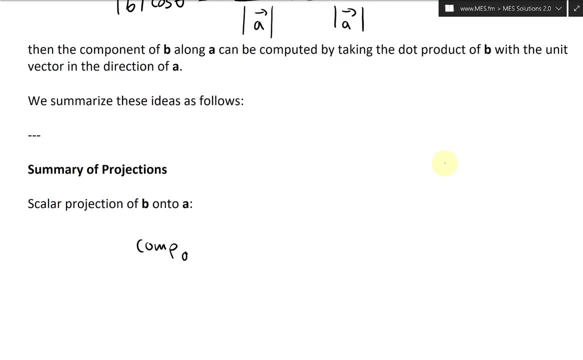 in other words, uh, comp- i'll write this here: comp of um, this is going to be here. comp of um, this is going to be here. comp of um. this is going to be b along a. the subscript a: b along a. the subscript a: b along a. the subscript a is equal to. 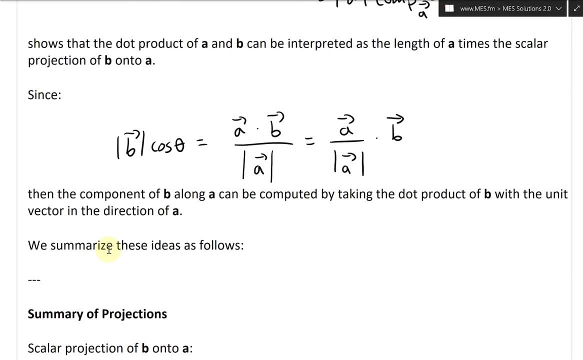 is equal to is equal to, and that is just here. move this over a, and that is just here. move this over a, and that is just here. move this over a to this other side. so dot product to this other side. so dot product to this other side. so dot product divided by the length. 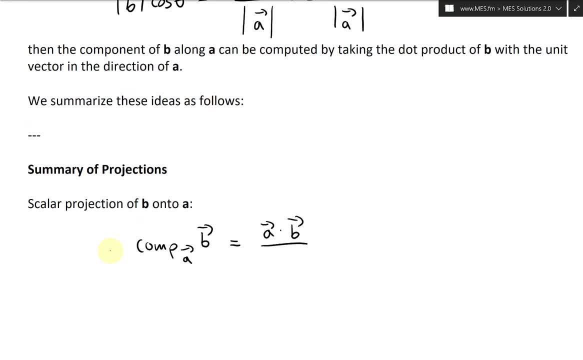 divided by the length divided by the length, so dot product, so dot product, so dot product of a dot b divided by the length of a of a dot b divided by the length of a of a dot b divided by the length of a, like this, like this: 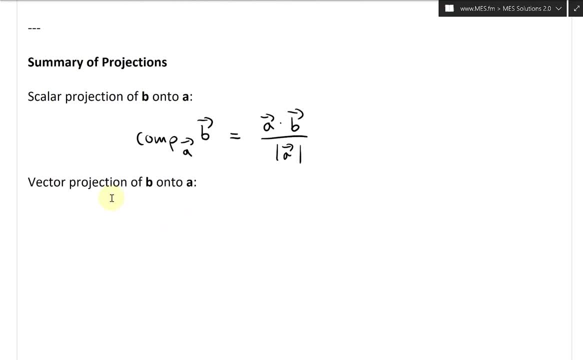 like this. all right, so that's the scalar. all right, so that's the scalar. all right, so that's the scalar projection. and now let's look at the projection. and now let's look at the projection. and now let's look at the vector projection of b onto a. 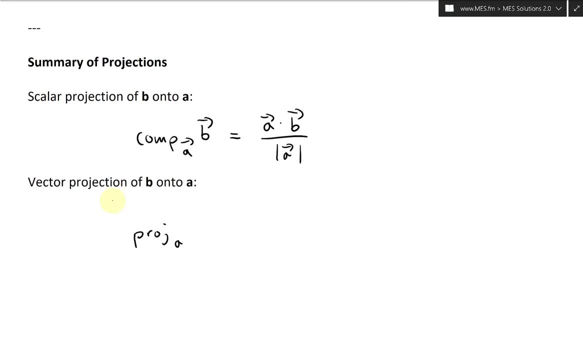 vector projection of b onto a, vector projection of b onto a. so the projection approach like that, so the projection approach like that, so the projection approach like that: uh, subscript a of uh, subscript a of uh subscript a of b, sub b is projection of b onto a in. 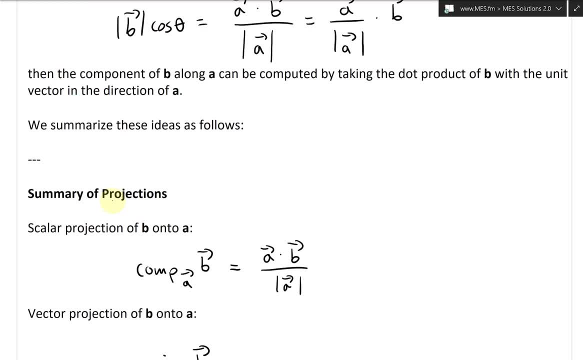 b. sub b is projection of b onto a in b. sub b is projection of b onto a in vector format. vector format. vector format: yeah, this equals two, so scroll, scroll. yeah, this equals two, so scroll, scroll. yeah, this equals two, so scroll, scroll. back to our projections. 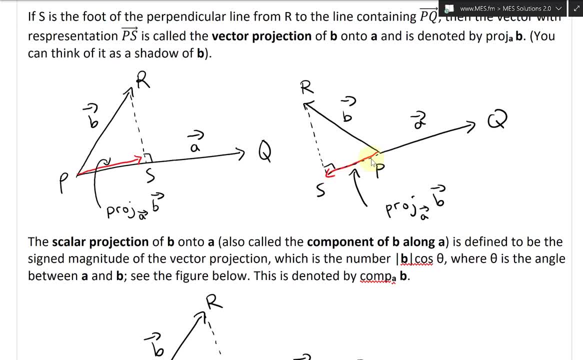 back to our projections, back to our projections. yeah, this projection, so that's a vector. yeah, this projection, so that's a vector. yeah, this projection, so that's a vector format. so basically, uh, we need to know format. so basically, uh, we need to know format. so basically, uh, we need to know the direction of this. 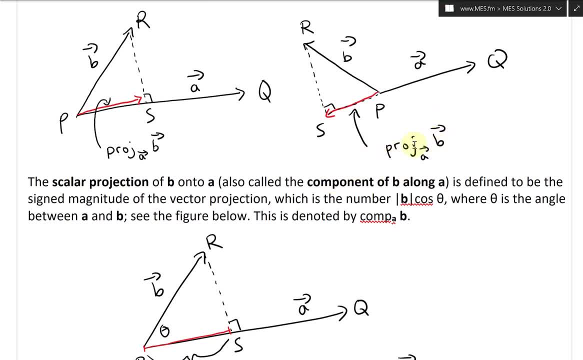 the direction of this. the direction of this, uh yeah. so the direction of this, uh yeah. so the direction of this, uh yeah. so the direction of this approach, uh, projection of b onto a approach, uh, projection of b onto a approach, uh, projection of b onto a. but- and we know the out of the magnitude- 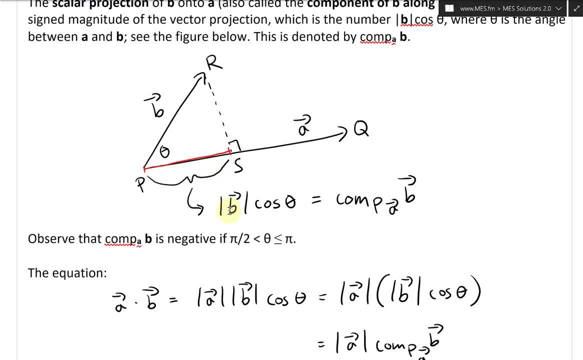 but, and we know the out of the magnitude, but, and we know the out of the magnitude of it, that's the full size, it's a signed of it, that's the full size, it's a signed of it, that's the full size, it's a signed size. and that, whether it's negative or 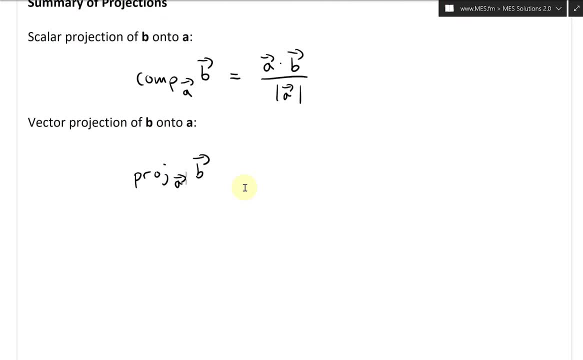 size, and that, whether it's negative or size, and that, whether it's negative or positive, will positive, will positive will determine the direction. so, in other, determine the direction, so in other, determine the direction. so, in other words, we could write this as projection words, we could write this as projection. 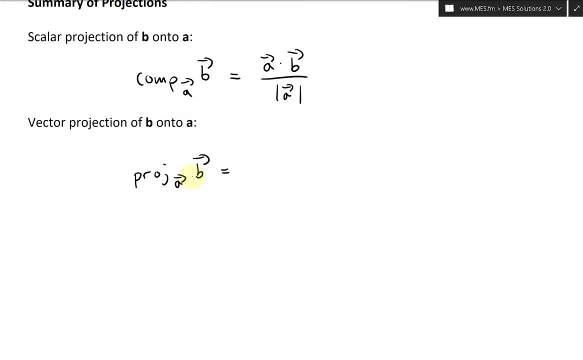 words. we could write this as: projection of b onto a is equal to of b. onto a is equal to of b onto a is equal to the component of b, the component of b, the component of b onto a. i'll just write this: yeah, so onto a. i'll just write this: yeah so. 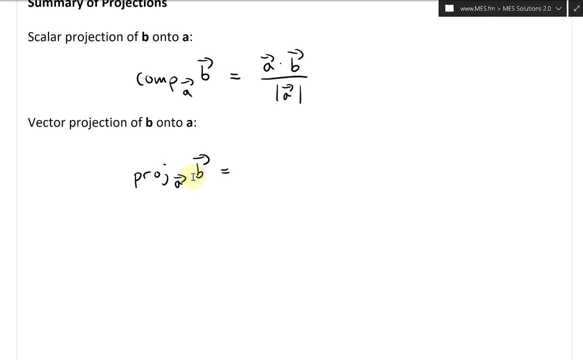 onto a. i'll just write this: yeah, so that's equals to that's, equals to, that's equals to this part right here, and write this as a dot b over a dot b over a dot b over: uh, the length a, uh, the length a, uh, the length a, and then multiply this by well, the direct. 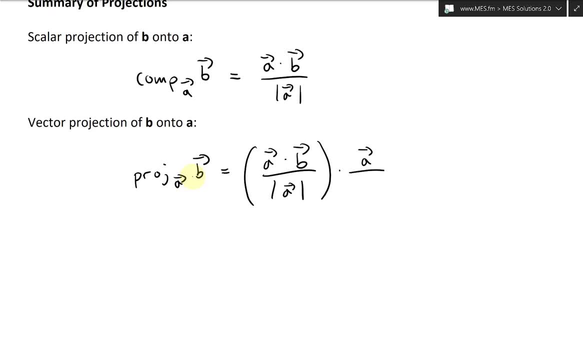 and then multiply this by well the direct, and then multiply this by well the direct: the unit vector in the direction of a. the unit vector in the direction of a. the unit vector in the direction of a. like that. so it's gonna be the direction, like that. so it's gonna be the direction. 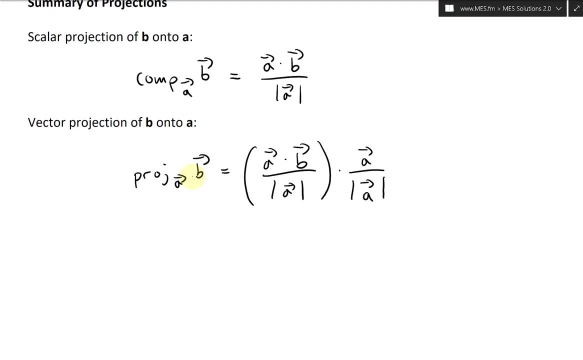 like that. so it's gonna be the direction of a there, because that's where the of a there, because that's where the of a there, because that's where the component is, and this sign is whether component is, and this sign is whether component is, and this sign is whether it's negative or positive, depending on 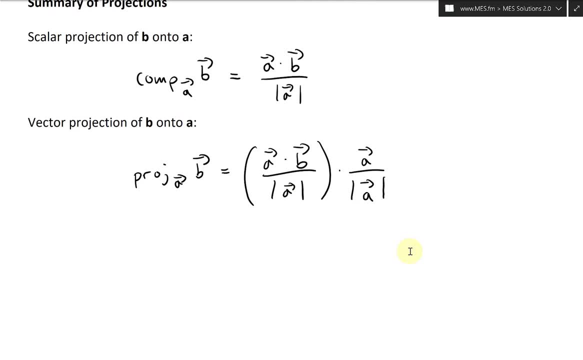 it's negative or positive, depending on it's negative or positive, depending on the angle: the angle, the angle of the uh, of the of the uh of the of the uh of the of the vector b, of the vector b of the uh of the of the vector b relative to a. so, yes, that's fast. so in. 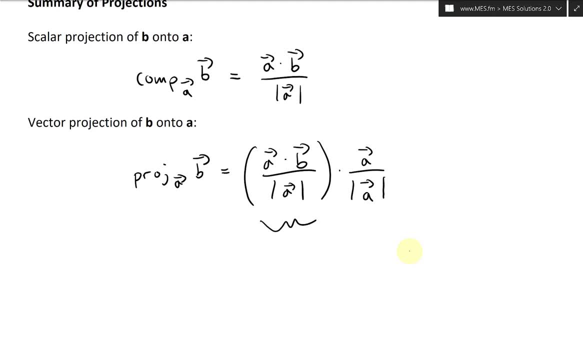 relative to a: so, yes, that's fast. so in relative to a: so, yes, that's fast. so, in other words, this right here, i'll put other words. this right here, i'll put other words. this right here, i'll put this: this is the component, component, component. 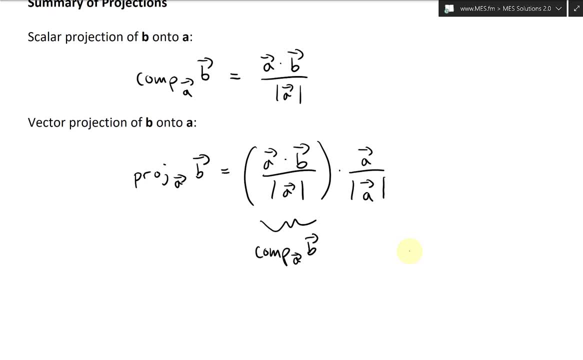 component onto a of b, onto a of b, onto a of b. and this right here and this right here and this right here is the unit vector, is the unit vector, is the unit vector. this is a unit vector along the direction of a, so that's along the direction of a, so that's. 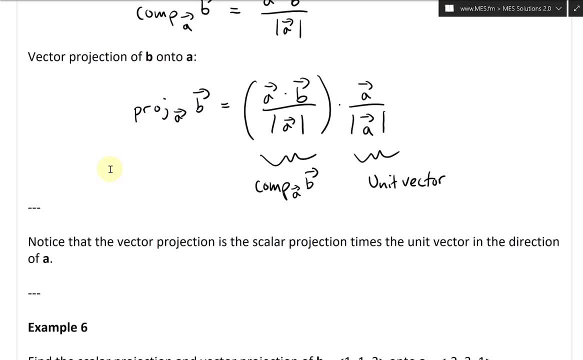 along the direction of a. so that's fascinating stuff, fascinating stuff, fascinating stuff. all right, let's continue further. all all right, let's continue further. all all right, let's continue further. all right, so now i continue for this notice. right, so now i continue for this notice. 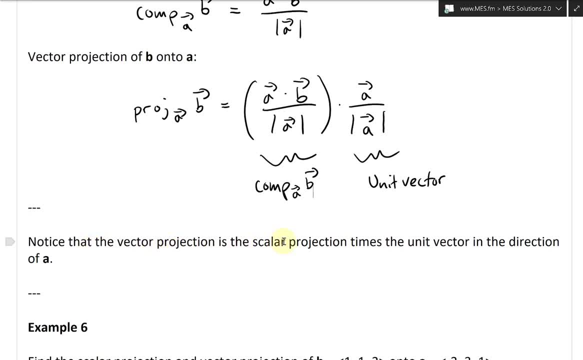 right. so now i continue for this. notice again, as i said here. notice that again, as i said here. notice that again, as i said here. notice that the, the, the vector projection, is just a scalar vector projection is just a scalar vector projection is just a scalar projection times or multiplied. 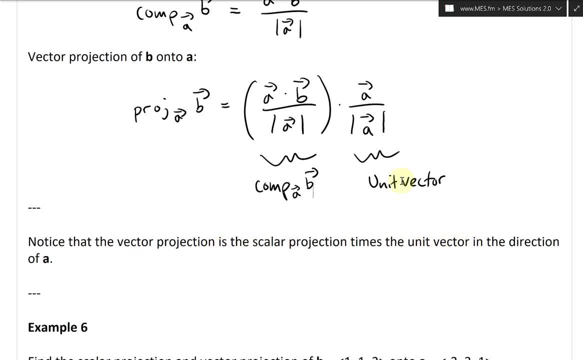 projection times or multiplied projection times or multiplied: uh the unit multiplied by the unit. uh the unit multiplied by the unit. uh the unit multiplied by the unit. vector in the direction of a. so that's vector in the direction of a. so that's vector in the direction of a. so that's the unit vector. 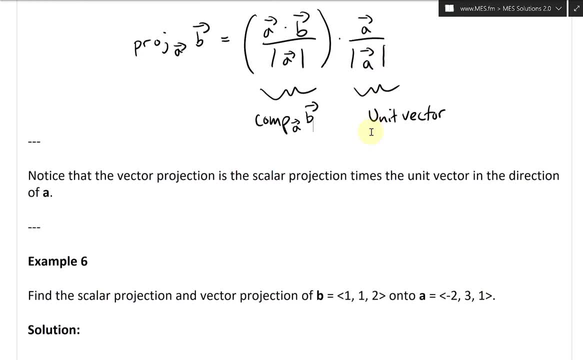 the unit vector, the unit vector, unit vector in a direction of a, hence this unit vector in a direction of a. hence this unit vector in a direction of a. hence this vector, and there's the length of it, vector, and there's the length of it, vector, and there's the length of it. all, right, very interesting. so now let's. 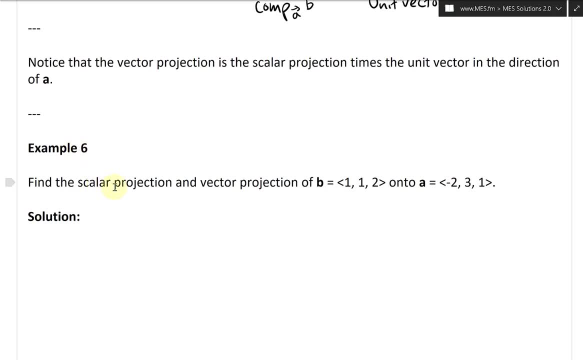 all right, very interesting, so now let's. all right, very interesting, so now let's continue further. and look at example. continue further. and look at example. continue further. and look at example six. and this one states: uh, find the six. and this one states: uh, find the six. and this one states: uh, find the scalar projection and vector projection. 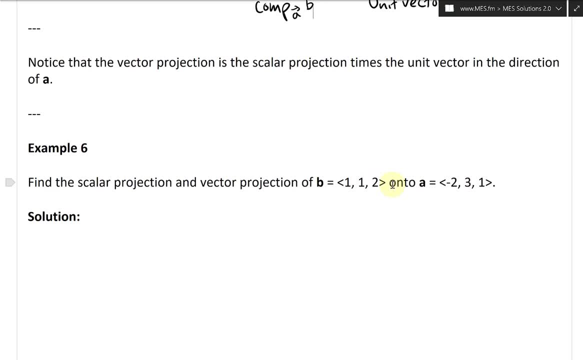 scalar projection and vector projection. scalar projection and vector projection of the vector b with components one. one of the vector b with components one. one of the vector b with components one. one, two onto a, which has components. two onto a, which has components. two onto a, which has components. negative. two, three and one. 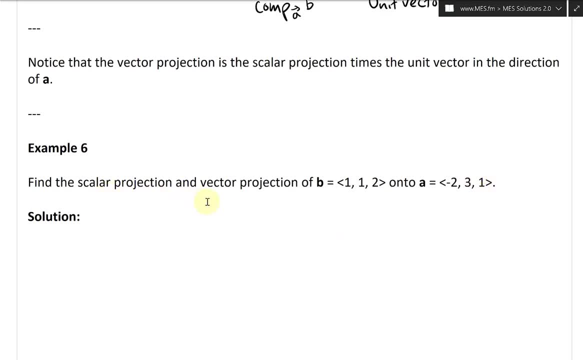 negative, two, three and one. negative, two, three and one, all right. so let's get the scalar which, all right. so let's get the scalar which, all right. so let's get the scalar which is the component one, and then we'll do. is the component one, and then we'll do. 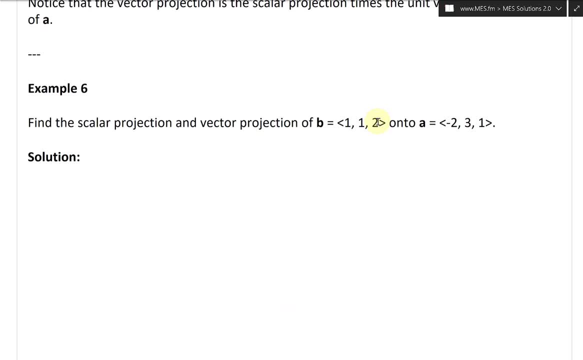 is the component one, and then we'll do the vector projection. because we multiply the vector projection, because we multiply the vector projection, because we multiply the unit vector. so let's take a look at the vector projection, because we multiply the unit vector. so let's take a look at. 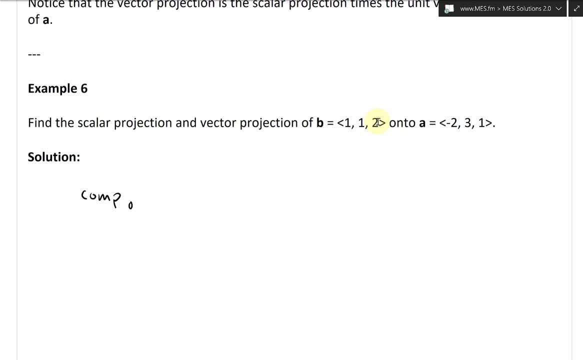 the vector projection, because we multiply the unit vector. so let's take a look at this so component, this so component, this so component. onto a of b, so b onto a. onto a of b, so b onto a. onto a of b, so b onto a. oops, 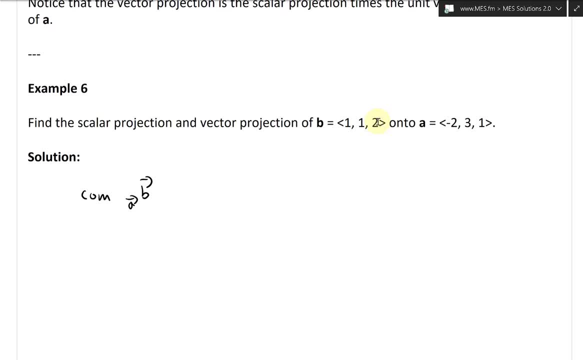 oops, oops, um, um, um. raise this better, raise this better, raise this better. component, component, component. uh, this right here, this equals two. and uh, this right here, this equals two. and uh, this right here, this equals two. and this is just again. this is just again. 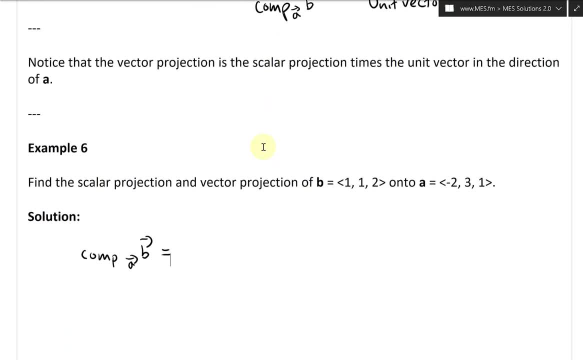 this is just again: uh, the vector on the dot product divided, uh, the vector on the dot product divided, uh, the vector on the dot product divided by the length, by the length, by the length. so this is going to be so. this is going to be so. this is going to be a dot b. 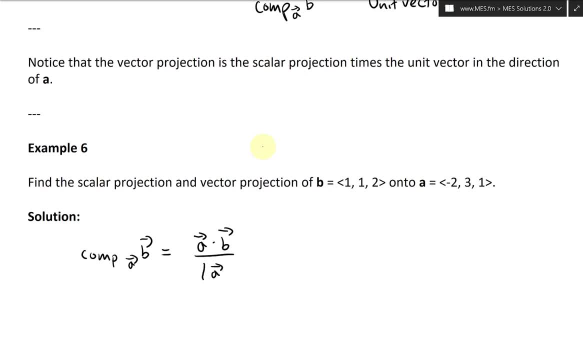 dot b over length a. dot b over length a, dot b over length a. this equals two. let's put this. all this equals two. let's put this, all this equals two. let's put this all together, so the dot product will have. together, so the dot product will have. 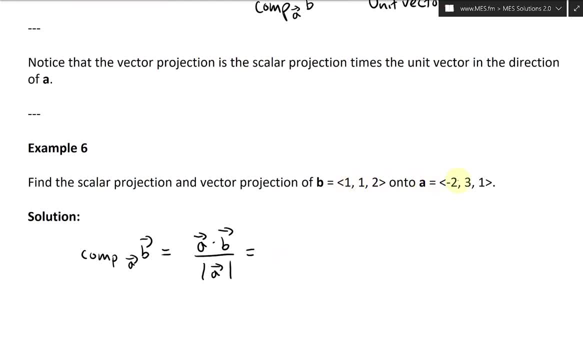 together, so the dot product will have this one, this one, this one times negative, one times negative, one times negative one. or we'll go a here first, so negative, or we'll go a here first, so negative. or we'll go a here first, so negative, negative, two. 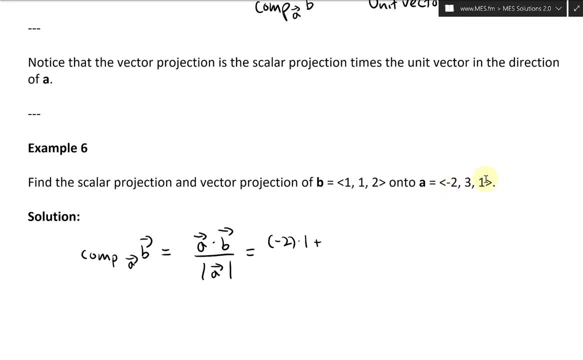 negative two negative two times by one times by one times by one plus three times one plus three times one plus three times one plus one times two plus one times two plus one times two, and then divided by, and now we're going. and then divided by, and now we're going. 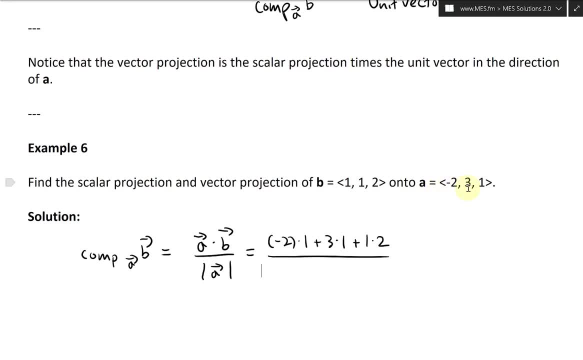 and then divided by. and now we're going to look at the length of a, to look at the length of a, to look at the length of a. here that's going to be square root, the here that's going to be square root, the here that's going to be square root, the positive square root. 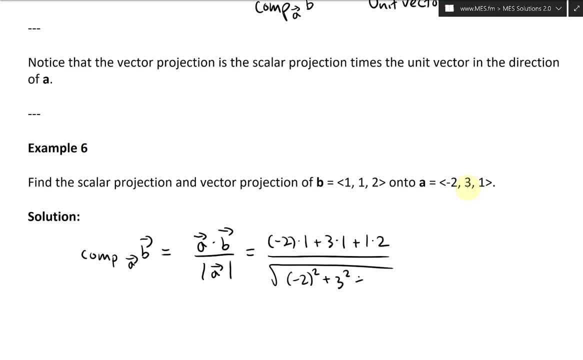 positive square root: positive square root negative. two squared plus three squared negative. two squared plus three squared negative. two squared plus three squared plus one plus one plus one squared which equals two squared which equals two squared, which equals two. this equals two. well negative two. this equals two. well negative two. 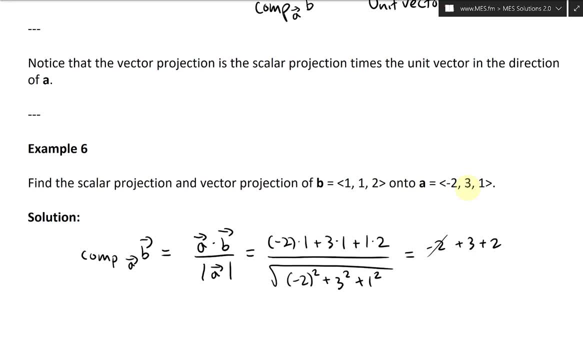 this equals two, well, negative two plus three plus three plus three plus two. this cancels plus two, this cancels plus two, this cancels. we're left with three. we're left with three, we're left with three, and then the bottom is going to be, and then the bottom is going to be. 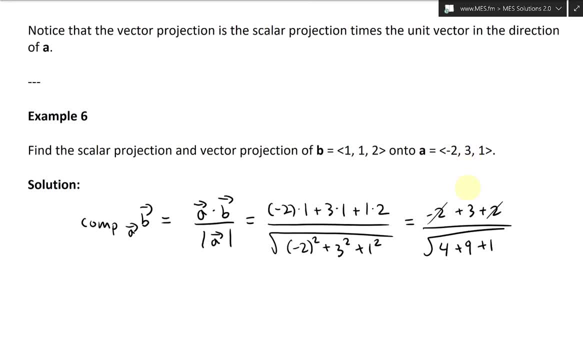 and then the bottom is going to be four plus nine plus one. that's a square four plus nine plus one. that's a square four plus nine plus one. that's a square root 14. because it's four plus one is root 14, because it's four plus one is. 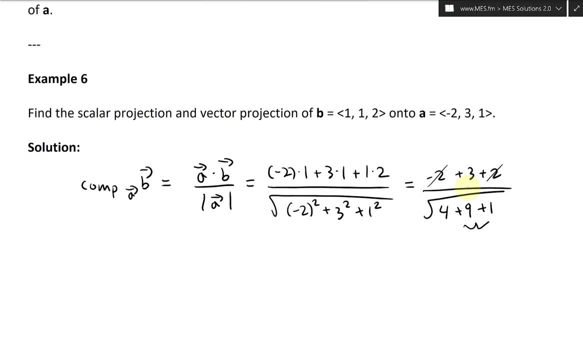 root 14, because it's four plus one is five or nine plus one is ten. five or nine plus one is ten, five or nine plus one is ten. yeah, this is 10, yeah, this is 10, yeah, this is 10, right here, right here, right here. and then 4 plus 10 is 14.. 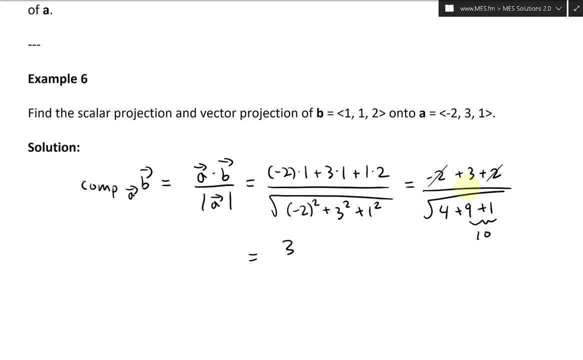 and then 4 plus 10 is 14.. and then 4 plus 10 is 14.. so this equals to, so this equals to. so this equals to: uh three over, or i'll just move it over. uh three over, or i'll just move it over. 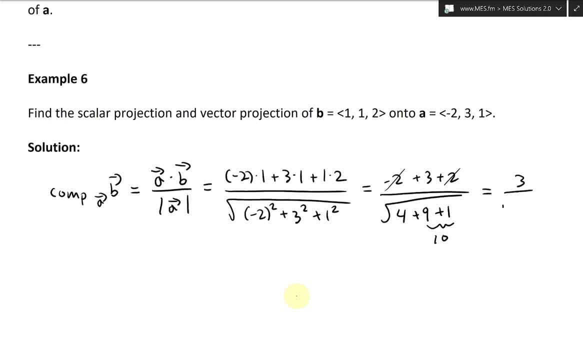 uh, three over, or i'll just move it over here. i moved everything over there, fit it here. i moved everything over there. fit it here. i moved everything over there, fit it all in there. so three over, all in there. so three over here. square root 14 is the. 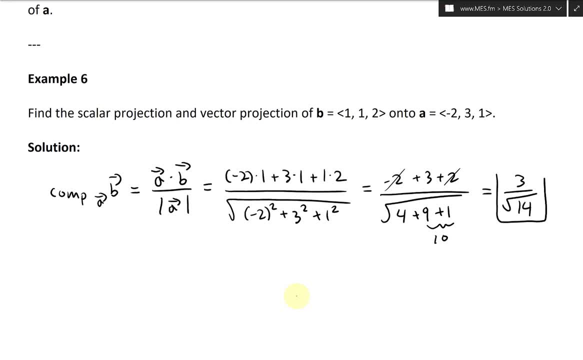 square root. 14 is the square root. 14 is the component of b. the magnitude of the component of b, the magnitude of the component of b, the magnitude of the projection onto it, projection onto it, projection onto it. now, we just got to multiply by the unit. 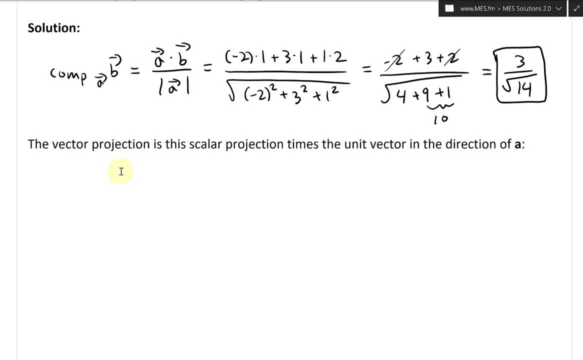 now we just got to multiply by the unit. now we just got to multiply by the unit: vector along a vector along a vector along a, and we'll do that here, so the vector, and we'll do that here, so the vector, and we'll do that here, so the vector. projection is: 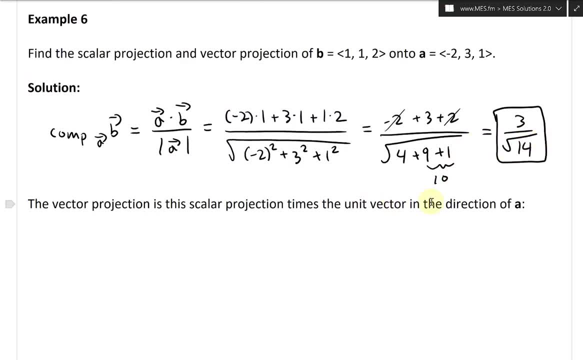 projection is, projection is. is this scalar projection of above here. is this scalar projection of above? here. is this scalar projection of above here: times the unit vector in the direction. times the unit vector in the direction. times the unit vector in the direction of a. so let's write it down. 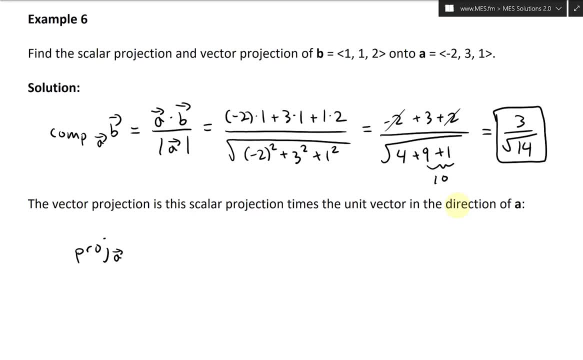 of a, so let's write it down. of a. so let's write it down. projection of a unit vector. projection of a unit vector. projection of a unit vector of b onto a is equal to the component of b onto a is equal to the component of b onto a is equal to the component or the scalar projection. 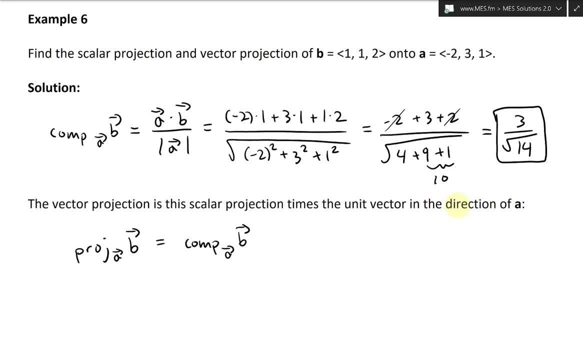 or the scalar projection, or the scalar projection, this is along a of b along a. this is along a of b along a. this is along a of b along a. multiplied by, multiplied by, multiplied by uh, this is going to be the uh, this is going to be the. 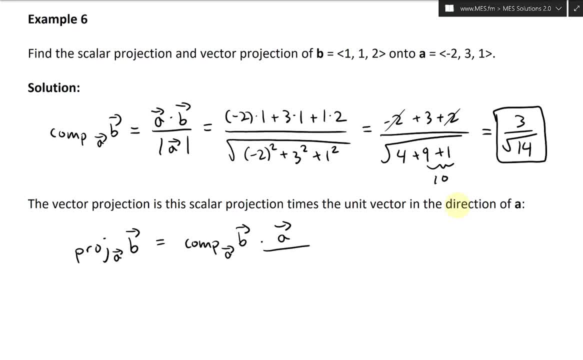 uh, this is going to be the yeah, the a vector unit vector along a. yeah, the a vector unit vector along a. yeah, the a vector unit vector along a. in other words, divide this by, in other words, divide this by, in other words, divide this by its length. so, 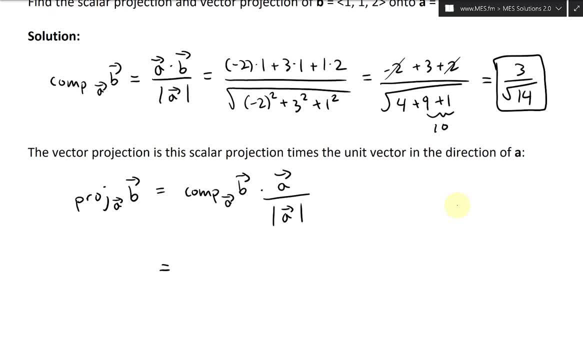 its length, so its length. so this all equals two, and let's put it: this all equals two. and let's put it: this all equals two, and let's put it together here, just put it on top there, together here. just put it on top there, together here. just put it on top there, and- and we know that this is just uh- 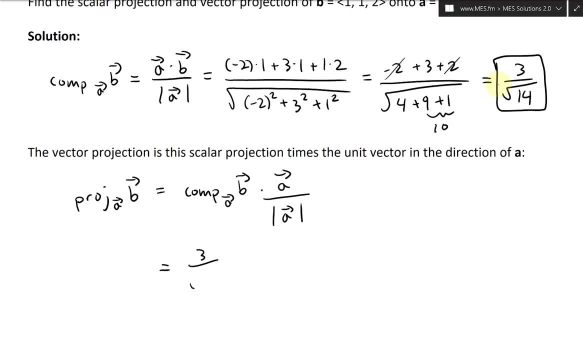 and, and we know that this is just uh, and, and we know that this is just uh, three over squared 14, three over squared 14, three over squared 14. is the component, is the component, is the component. and then multiply by a, and then multiply by a. 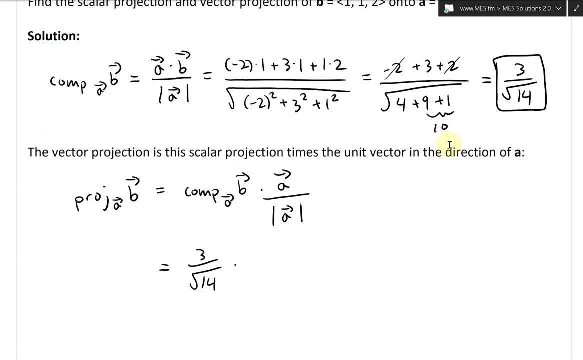 and then multiply by a. well, let's plug in a. is the vectors? well, let's plug in a. is the vectors? well, let's plug in a. is the vectors: here's negative: two, three and one. here's negative: two, three and one. here's negative: two, three and one. negative two, three and one. and the length. 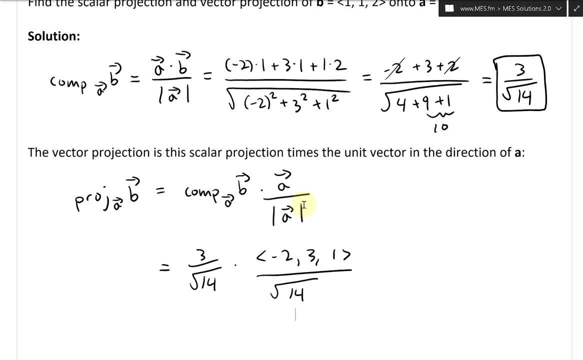 negative two, three and one and the length. negative two, three and one and the length is we know a is 14, is. we know a is 14, is we know a is 14, like that. and uh, yeah, yeah, notice there's like that. and uh, yeah, yeah, notice there's. 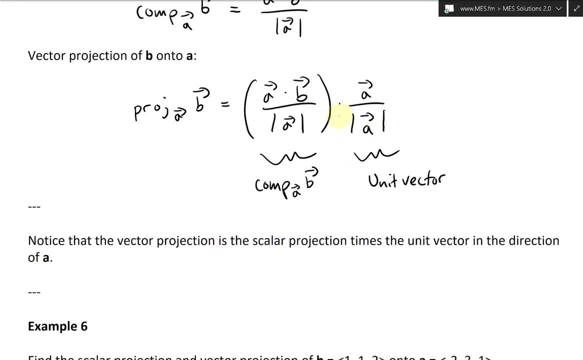 like that, and uh, yeah, yeah, notice, there's gonna be a square there, and actually i gonna be a square there and actually i gonna be a square there, and actually i hear this part, you can uh simplify this. hear this part, you can uh simplify this. hear this part, you can uh simplify this further. actually, i forgot to do this. 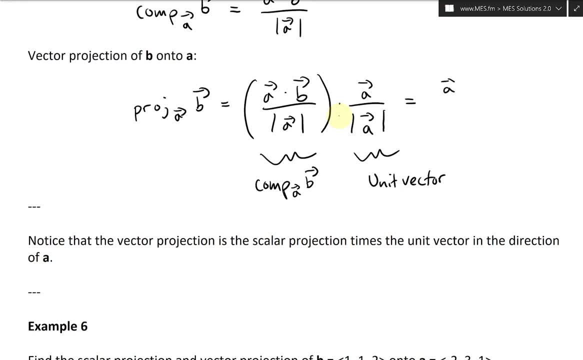 further. actually, i forgot to do this further. actually, i forgot to do this. this is just going to be. this is just going to be. this is just going to be: a dot, a dot, a dot, b over b, over b over a squared, a squared, a squared, and then a dot, i mean, uh, a like that. 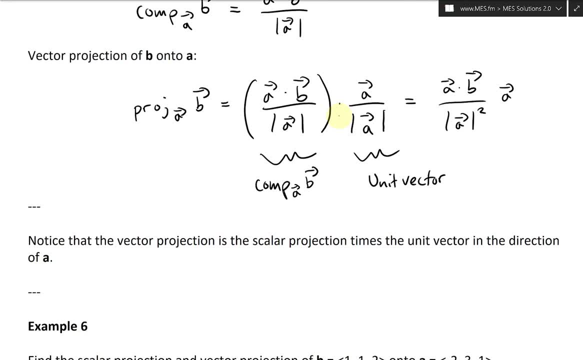 and then a dot, i mean uh, a like that, and then a dot, i mean uh, a like that, so dot product there, and then yeah, so dot product there. and then yeah, so dot product there. and then yeah, it's length a times by length, a that's. 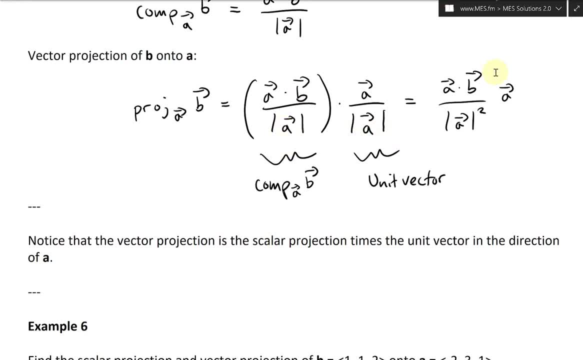 it's length a times by length: a. that's it's length a times by length. a. that's gonna be length a squared gonna be length a squared gonna be length a squared. that's fascinating stuff. and then there's. that's fascinating stuff, and then there's. 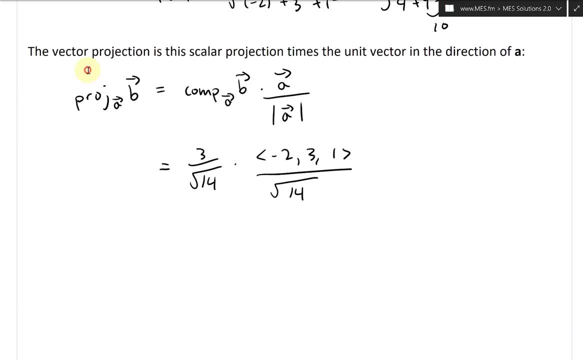 that's fascinating stuff. and then there's the dot product. the dot product, the dot product. all right, continue further. all right, continue further. all right, continue further, all right. so we have this part right. all right, so we have this part right. all right, so we have this part right here, and now we're gonna do is: i'm gonna 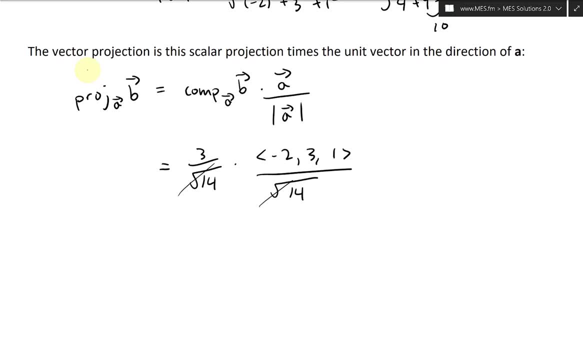 here and now we're gonna do is i'm gonna here and now we're gonna do is i'm gonna uh multiply these out. so yeah, just uh multiply these out. so yeah, just uh multiply these out. so yeah, just squaring that the square roots cancel. squaring that the square roots cancel. 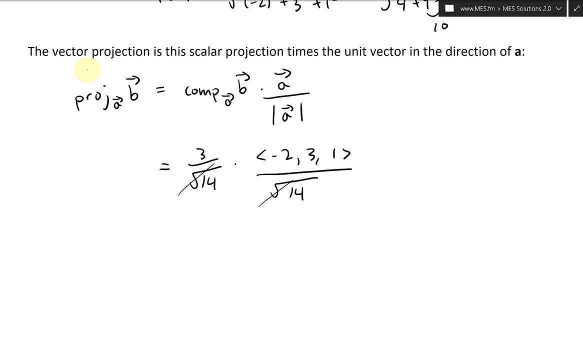 squaring that the square roots cancel. square root 14 times square root 14. square root 14 times square root 14. square root 14 times square root 14. that's gross cancel and we're just going. that's gross cancel and we're just going. 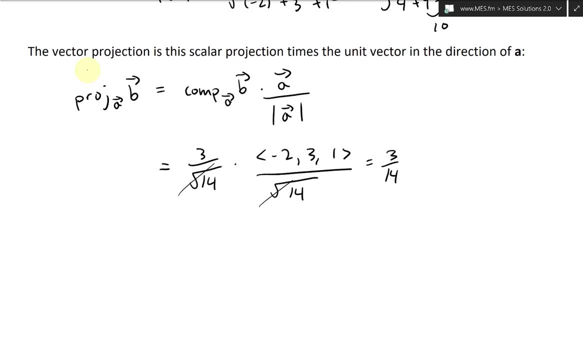 that's gross cancel, and we're just going to be left with 3 over 14, to be left with 3 over 14, to be left with 3 over 14, and then we're going to have this um, and then we're going to have this um. 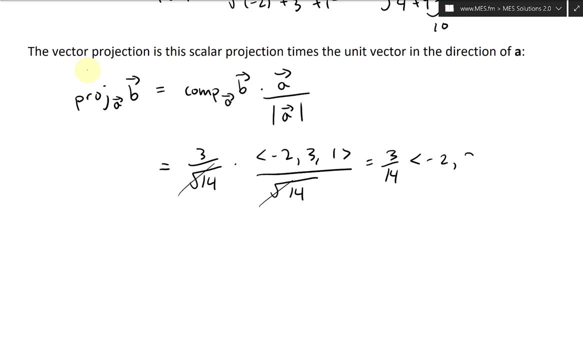 and then we're going to have this: um, this is the a vector, this is the a vector, this is the a vector: negative two, three, negative two, three. negative two, three, one, one, one like that, like that. like that, all right, and now, all right, and now, all right, and now what we'll do is multiply this inside. 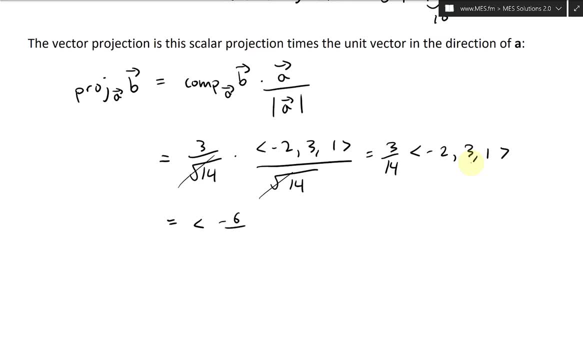 what we'll do is multiply this inside. what we'll do is multiply this inside uh three times negative. two is gonna be a uh three times negative. two is gonna be a uh three times negative. two is gonna be a well negative six. well negative six, well negative six over fourteen. 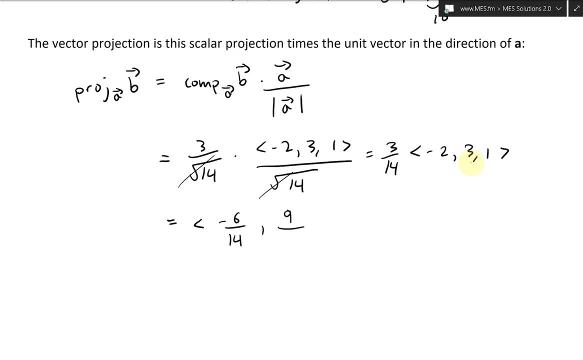 over fourteen over fourteen, and then we're gonna have a nine, and then we're gonna have a nine, and then we're gonna have a nine over fourteen, and then a one over fourteen over fourteen, and then a one over fourteen over fourteen, and then a one over fourteen, i mean a three over fourteen. 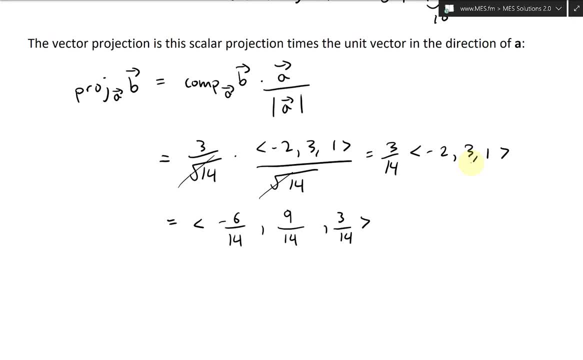 i mean a three over fourteen. i mean a three over fourteen because they have three times. one is because they have three times. one is because they have three times. one is three. yeah, it's just one. three, yeah, it's just one. three, yeah, it's just one and this one. here we could simplify this. 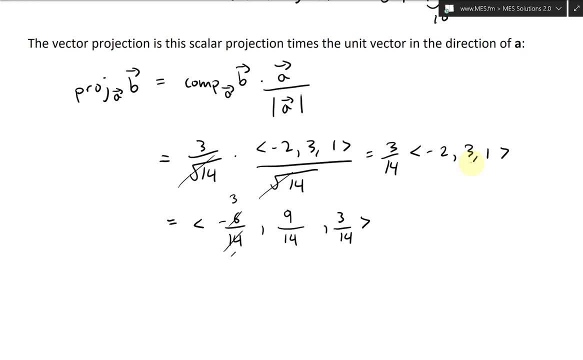 and this one- here we could simplify this. and this one- here we could simplify this- divided by two- and this one- here we could simplify this- divided by two, we have three divided by, we have three divided by, we have three divided by two is going to be a seven. 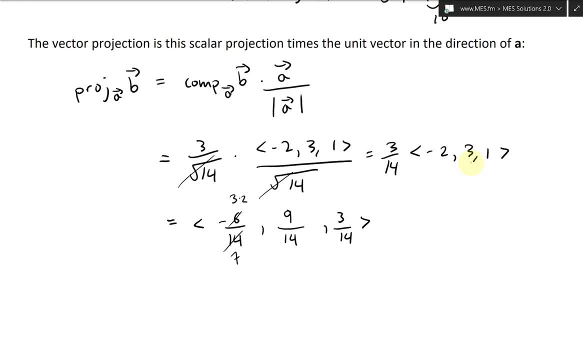 two is going to be a seven. two is going to be a seven, like that, like that, like that. all right. or you just write it as three, all right. or you just write it as three, all right. or you just write it as three times two. this is two times two and this. 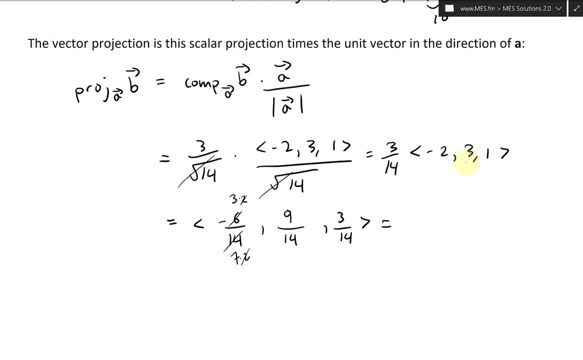 times two. this is two times two, and this times two. this is two times two, and this cancels, cancels, cancels. all right, so we're going to be left with. all right, so we're going to be left with all right. so we're going to be left with this, simplified even further. 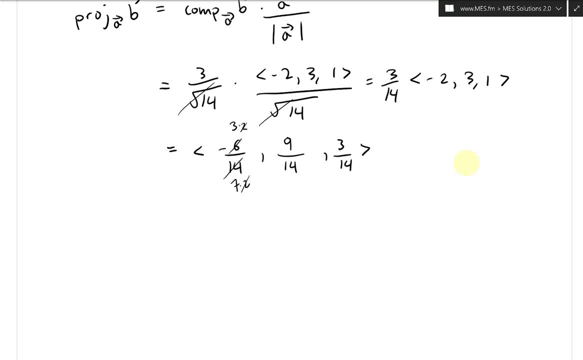 this simplified even further. this simplified even further, and this is all i'll put it all over, and this is all i'll put it all over, and this is all i'll put it all over here. actually, this equals to here. actually, this equals to here. actually, this equals to negative. 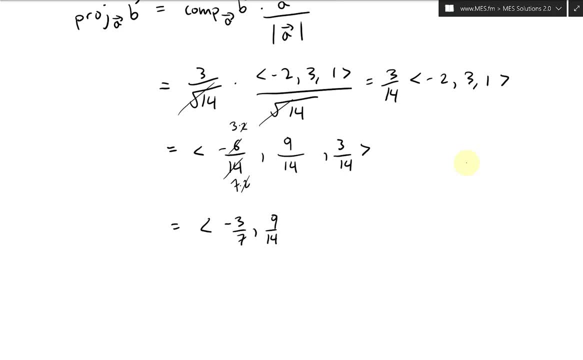 negative: negative: three over seven, three over seven, three over seven, nine over fourteen, nine over fourteen, nine over fourteen and three over fourteen, and this is our, and three over fourteen, and this is our, and three over fourteen, and this is our projection of b, of b, of b onto a. 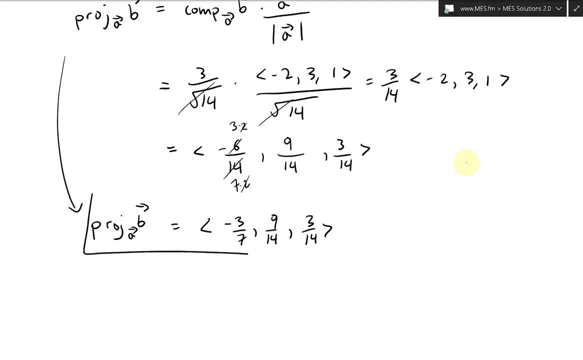 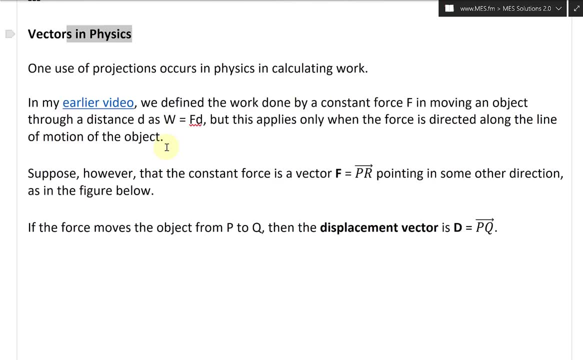 onto a, onto a, and yeah, this is our vector projection and yeah, this is our vector projection and yeah, this is our vector projection. all right, so now we solve that, and let's all right, so now we solve that, and let's all right, so now we solve that, and let's go over the last section of this, uh. 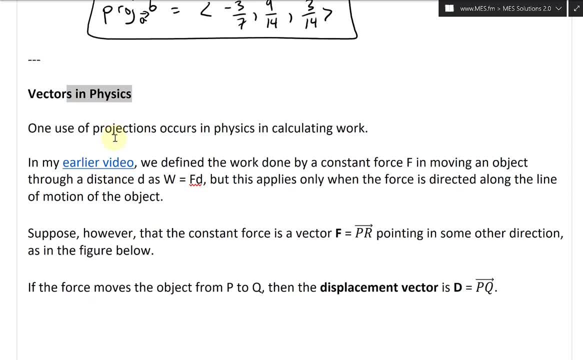 go over the last section of this. uh go over the last section of this. uh, extensive video. uh so vectors in physics- extensive video. uh so vectors in physics- extensive video. uh so vectors in physics. so one use of projections occurs in. so one use of projections occurs in. 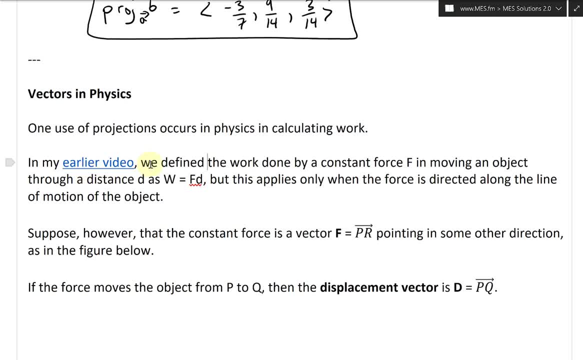 so one use of projections occurs in physics, in calculating physics, in calculating physics, in calculating work. so in my earlier video we defined work. so in my earlier video we defined work. so in my earlier video we defined the work done by constant force, the work done by constant force. 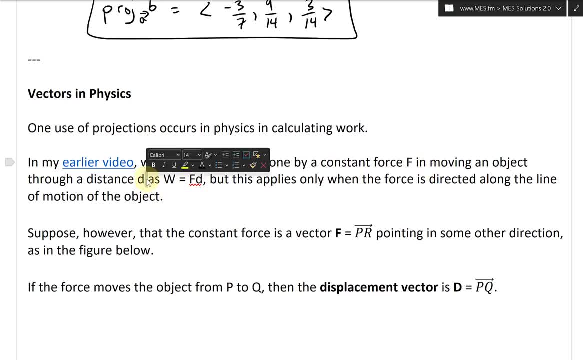 the work done by constant force f and moving an object through a f and moving an object through a f and moving an object through a distance d as distance d as distance d as work equals to force times distance, but work equals to force times distance. but work equals to force times distance, but this applies 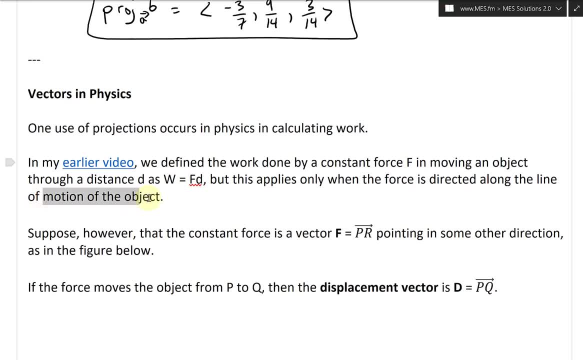 this applies. this applies only when the force is directed along, only when the force is directed along, only when the force is directed along the line of motion, the line of motion, the line of motion. suppose, however, that the constant force, suppose, however, that the constant force, suppose, however, that the constant force is a vector. 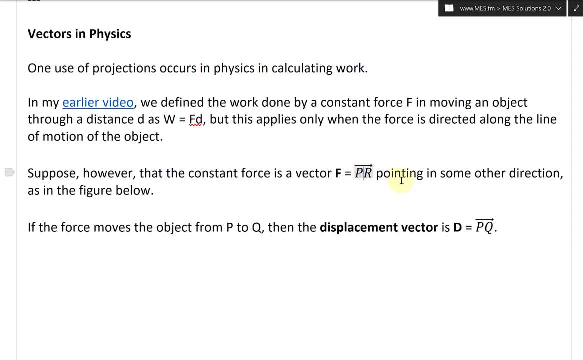 is a vector is a vector. i would call this f equals to pr. i would call this f equals to pr. i would call this f equals to pr. uh, so it pointing in some other uh. so it pointing in some other uh, so it pointing in some other direction, as in the figure. 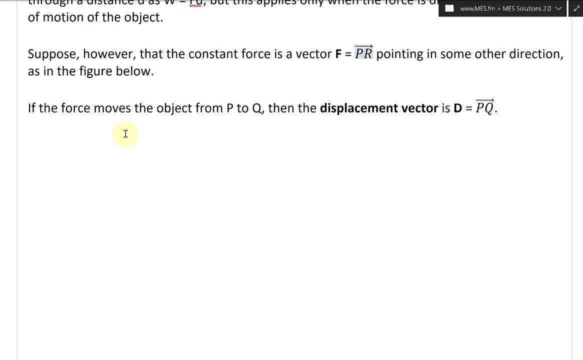 direction, as in the figure direction, as in the figure below, and i'll draw this in a bit so below. and i'll draw this in a bit so below, and i'll draw this in a bit. so if yeah, i'll draw this right here. so if yeah, i'll draw this right here. so 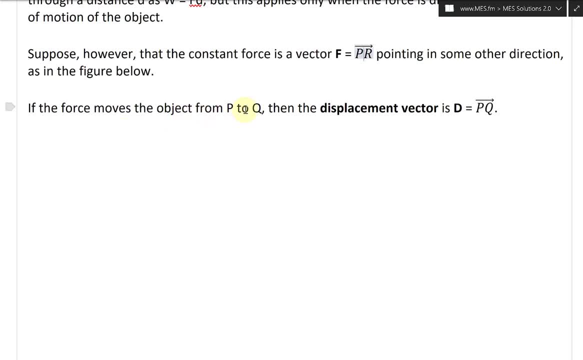 if yeah, i'll draw this right here. so let's say you had, let's say you had, let's say you had: yeah. so if the force moves object from p, yeah. so if the force moves object from p, yeah. so if the force moves object from p to q, then the displacement vector 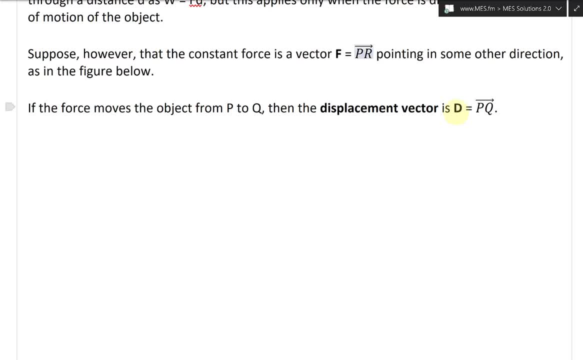 to q, then the displacement vector to q, then the displacement vector is d equals to pq. so in other words is d equals to pq. so in other words is d equals to pq. so in other words, let's say you had, let's say you had, let's say you had a: uh, here's a displacement here, so it. 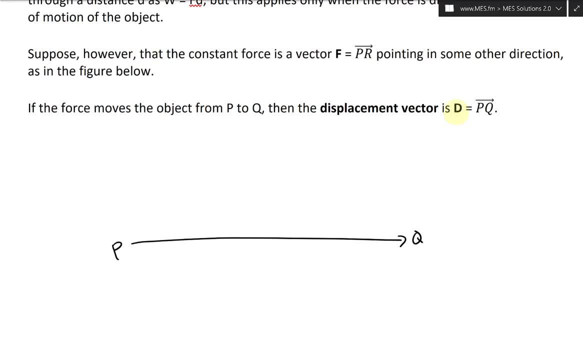 a uh, here's a displacement here. so it a uh, here's a displacement here, so it moves along, this, moves along this, moves along this, this direction from p to q, but the this direction from p to q, but the this direction from p to q, but the force is at some angle across there. this, 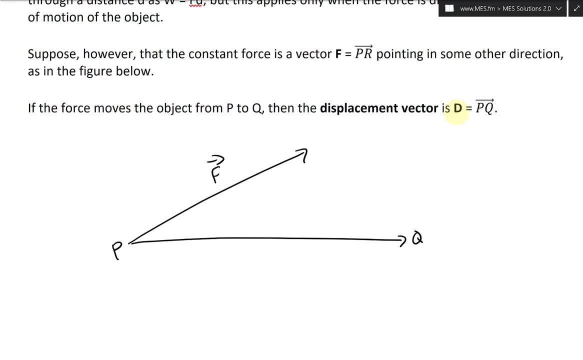 force is at some angle across there. this force is at some angle across there. this is the is the is the vector f and this right here, vector f, and this right here, vector f, and this right here is a displacement vector d is a displacement vector d is a displacement vector d and then this right here is per dash. 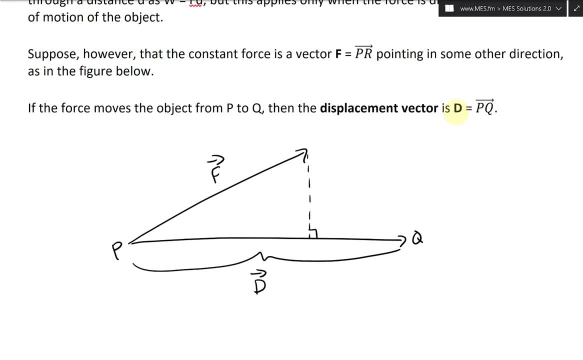 and then this, right here is per dash, and then this, right here is per dash, line, line, line, this perpendicular, and this is going to this perpendicular, and this is going to this perpendicular and this is going to be our s, be our s, be our s, this is going to be our r and then we're. 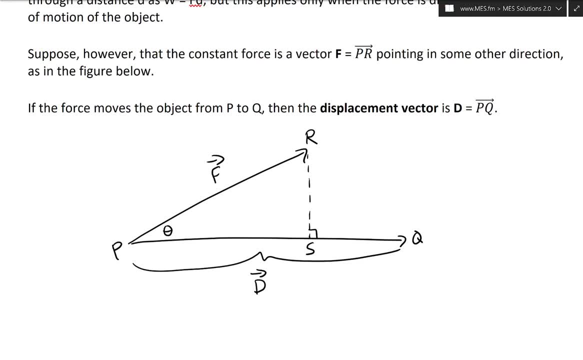 this is going to be our r, and then we're this is going to be our r and then we're going to have our going to have our going to have our other angle- well, this can be our angle. other angle: well, this can be our angle. other angle: well, this can be our angle. like that. 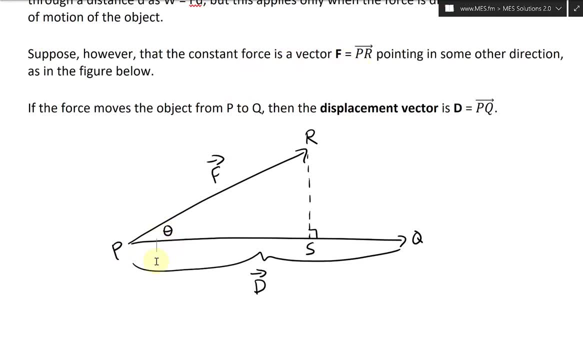 like that, like that. so this is a. this is the pr, so this is so. this is a. this is the pr, so this is. so. this is a. this is the pr, so this is the force f- the displacement from p to the force f- the displacement from p to. 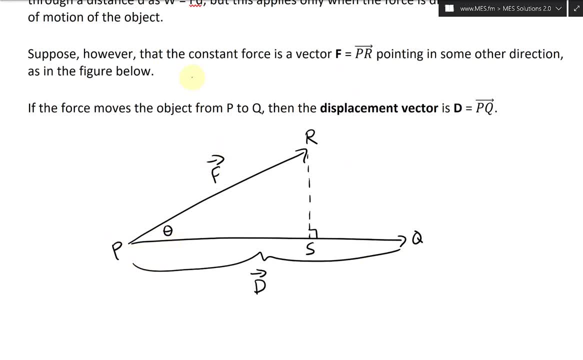 the force f, the displacement from p to q. but yeah, again, this is, this force is at q. but yeah, again, this is, this force is at q. but yeah, again, this is this force is at a different angle. yeah, so our net, uh, a different angle. yeah, so our net uh. 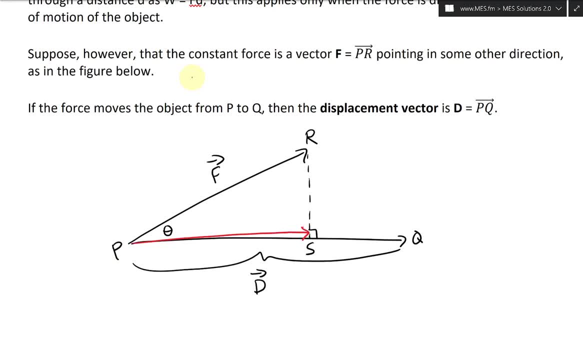 a different angle. yeah, so our net uh force in the direction along the force in the direction along the force in the direction along the displacement is going to be this red one displacement is going to be this red one displacement is going to be this red one again. it's a projection of f onto this. 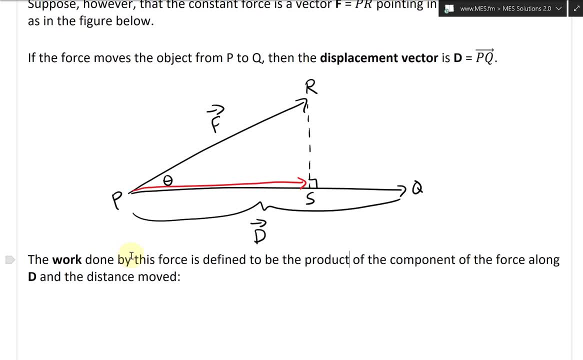 again, it's a projection of f onto this. again, it's a projection of f onto this, right here, right here, right here, all right going further. so now, uh, the all right going further. so now, uh, the all right going further. so now, uh, the work done by this force is defined to be: 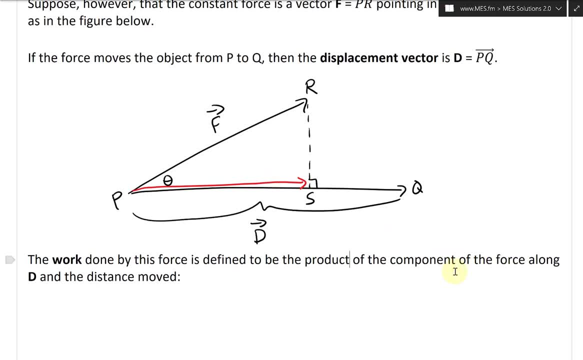 work done by this force is defined to be, work done by this force is defined to be the product of the component. so this, the product of the component. so this, the product of the component. so this right here of the force along, right here of the force along. 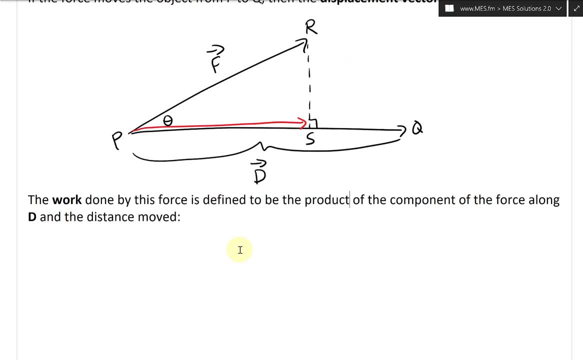 right here of the force along along d and the distance moved so in along d and the distance moved, so in along d and the distance moved so in other words, other words, other words, work is e is defined as work is e is defined as work is e is defined as uh, equaling right here. so this is going. 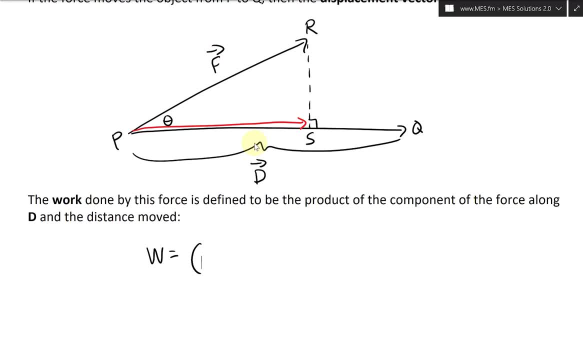 uh, equaling right here. so this is going, uh, equaling right here. so this is going to be the component onto this, this, this to be the component onto this, this, this to be the component onto this, this, this, projection onto here, projection onto here, projection onto here, the component of it. so, in other words, 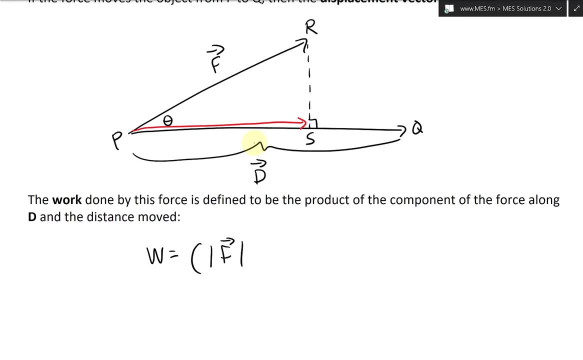 the component of it. so in other words, the component of it. so in other words, the. the magnitude of that, the. the magnitude of that, the, the magnitude of that. force vector times by cosine: to get the force vector times by cosine. to get the force vector times by cosine, to get the cosine direction of it. 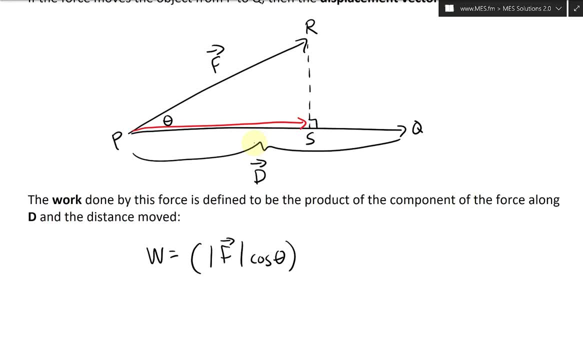 cosine direction of it. cosine direction of it, in other words, uh along q along this pq. in other words, uh along q along this pq. in other words, uh along q along this pq. and then multiply the distance travel, and then multiply the distance travel and then multiply the distance travel, like that. all right, yeah, so that is the. 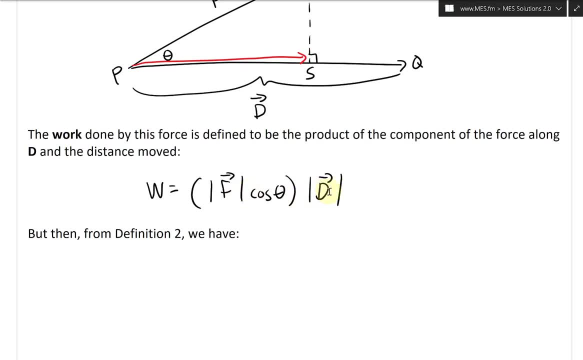 like that: all right, yeah, so that is the like that. all right, yeah, so that is the work. all right, so that is the work. but work all right, so that is the work, but work all right, so that is the work. but notice here, uh, if you just move this, uh, 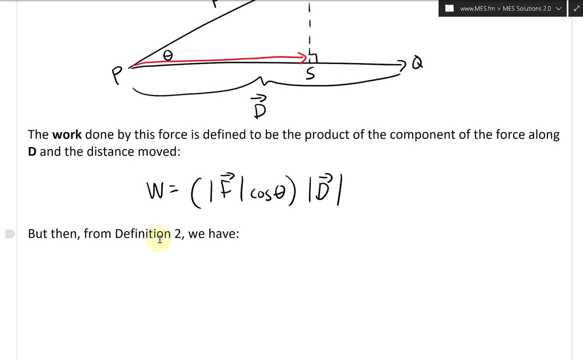 notice here, uh, if you just move this, uh. notice here, uh, if you just move this, uh, distance d over in the front, distance d over in the front, distance d over in the front. and uh, but then from definition two of. and uh, but then from definition two of. 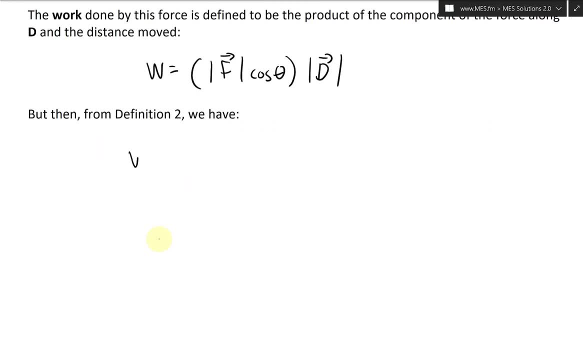 and uh, but then from definition two of the dot product, we have the dot product, we have the dot product we have. so we have: w is equal to, let's move, so we have. w is equal to, let's move, so we have. w is equal to: let's move this over. 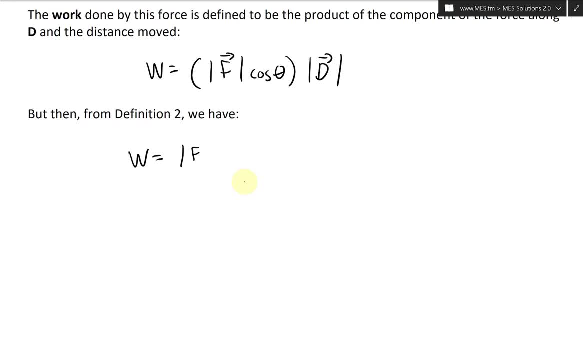 this, over this, over here, and that just becomes, um, the force magnitude times by the distance, the force magnitude times by the distance, the force magnitude times by the distance, traveled, traveled, traveled, and then times by cosine theta in other, and then times by cosine theta in other, and then times by cosine theta in other words, this is the dot product. 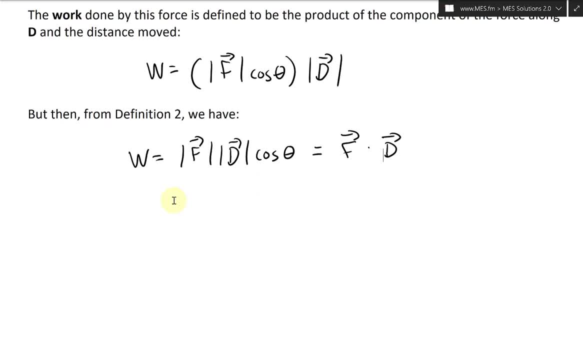 words: this is the dot product. words: this is the dot product. a force times the displacement vector. a force times the displacement vector. a force times the displacement vector, but this. or the distance vector, though, but this, or the distance vector though, but this, or the distance vector though. yeah, so, uh, thus the work done by. 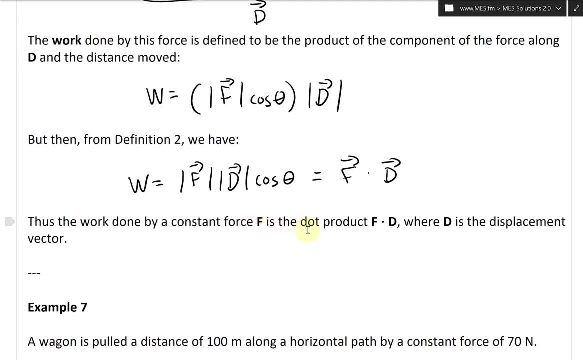 yeah, so uh. thus the work done by. yeah, so uh, thus the work done by. constant force, uh f. constant force, uh f. constant force, uh f. uh vector. f is the dot product of the uh vector. f is the dot product of the uh vector. f is the dot product of the force vector. 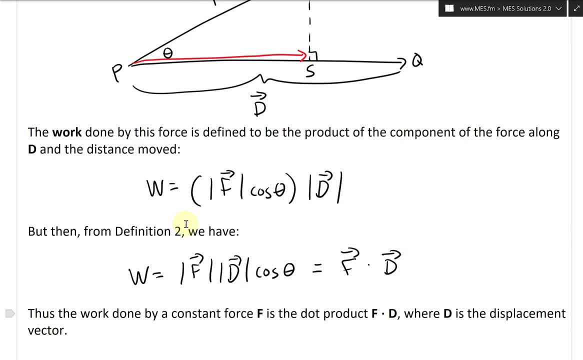 force vector. force vector- oh yeah, dot uh. displacement vector: oh yeah, dot uh. displacement vector, oh yeah, dot uh. displacement vector where d is a displacement vector, which is where d is a displacement vector, which is where d is a displacement vector, which is quite fascinating. so, yes, we define a dot. 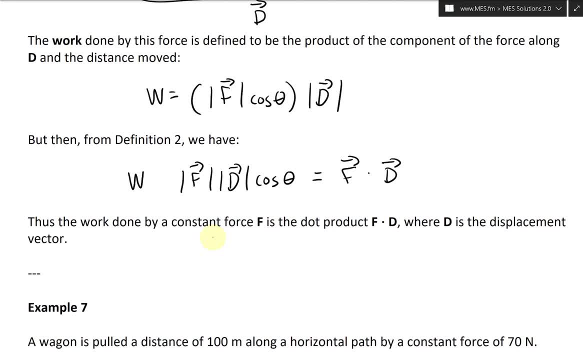 quite fascinating. so, yes, we define a dot. quite fascinating. so, yes, we define a dot, product, product, product. and then we somehow manage to link it. and then we somehow manage to link it, and then we somehow manage to link it all to physics, all to physics, all to physics. and how work is defined. so you just use. 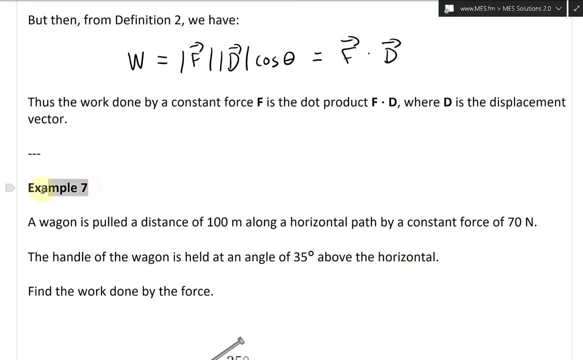 and how work is defined, so you just use, and how work is defined so you just use: the dot product, the dot product, the dot product. interesting, so, continuing further, so interesting, so, continuing further, so interesting, so, continuing further. so let's take a look at, let's take a look at. 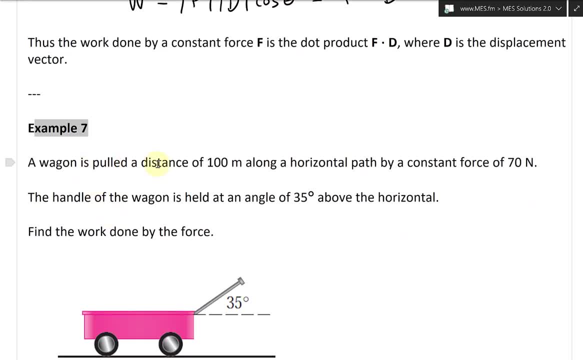 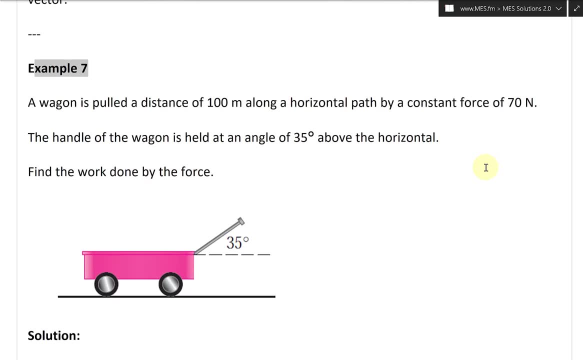 let's take a look at example seven. so a wagon is pulled. example seven: so a wagon is pulled. example seven: so a wagon is pulled. assuming it's being pulled like that: 70. assuming it's being pulled like that: 70. assuming it's being pulled like that, 70 newtons like that. 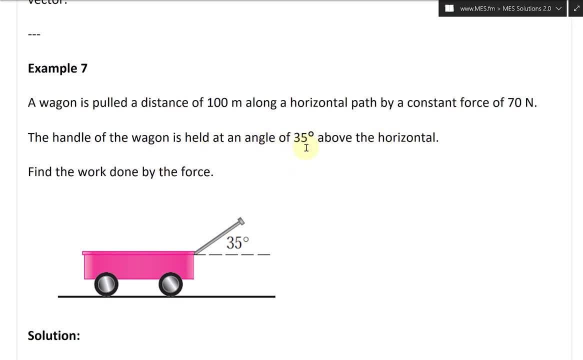 newtons like that. newtons like that. the handle of the wagon is held at an. the handle of the wagon is held at an. the handle of the wagon is held at an angle of 35 degrees above the horizontal, angle of 35 degrees above the horizontal. 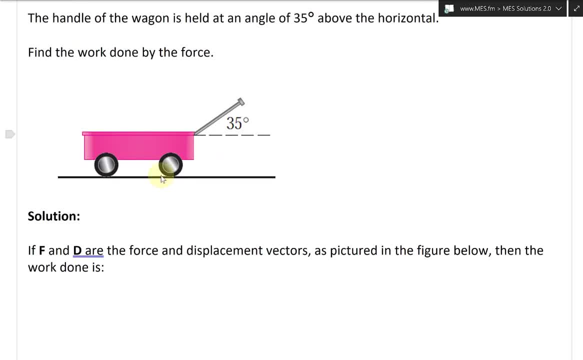 angle of 35 degrees above the horizontal, and it arrests. find the work done by the and it arrests. find the work done by the and it arrests. find the work done by the force, force, force, and let's take a look at the solution. and let's take a look at the solution. 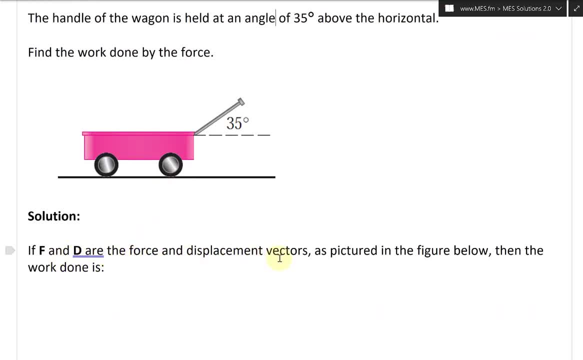 and let's take a look at the solution. all right. so if f and d are the force, all right. so if f and d are the force, all right. so if f and d are the force and displacement vectors as pictured in, and displacement vectors as pictured in. 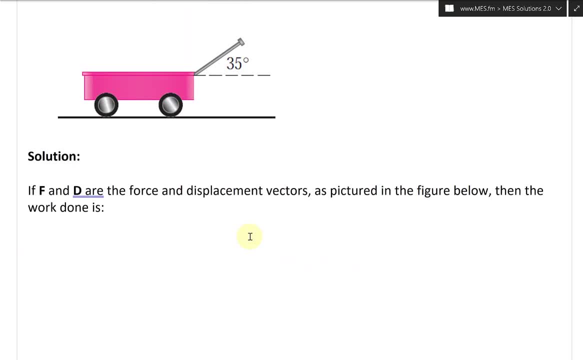 and displacement vectors, as pictured in the figure below, then the work done is the figure below. then the work done is the figure below. then the work done is: unless this- well, this is a. unless this- well, this is a. unless this- well, this is a straightforward one. it goes horizontal. 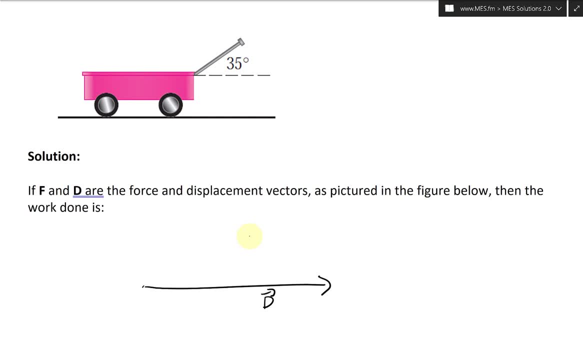 straightforward one: it goes horizontal. straightforward one: it goes horizontal. so you have d, so you have d, so you have d, like that, like that, like that, you have the force here and angles 35. you have the force here and angles 35. you have the force here and angles 35 degrees. 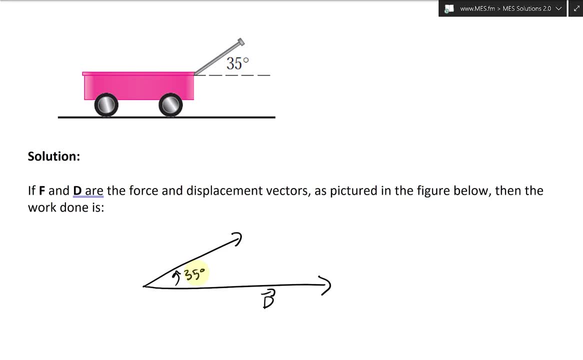 degrees, degrees. let's draw like that. let's draw like that. let's draw like that: 35 degrees. this projection onto here. 35 degrees. this projection onto here, 35 degrees. this projection onto here. this is the right angle, this is our. this is the right angle, this is our. 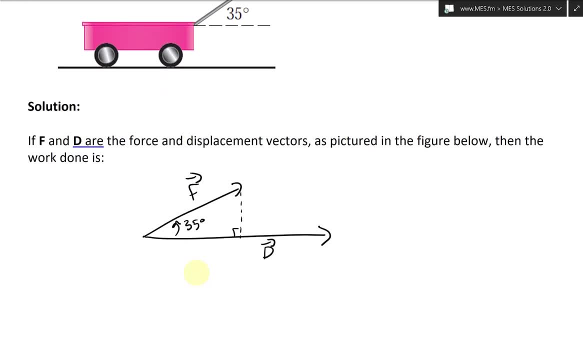 this is the right angle. this is our force vector, force vector, force vector, and what we get is, and what we get is and what we get is. i'll smooth this over, i'll smooth this over, i'll smooth this over to here on the left side, to here on the left side. 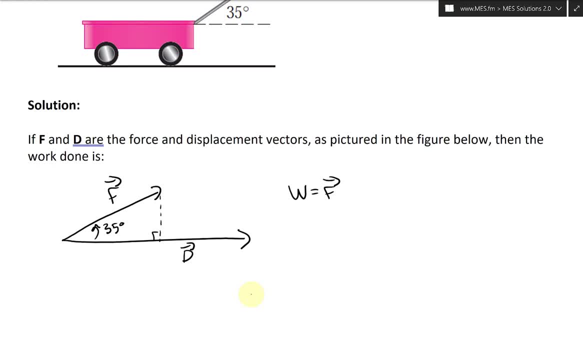 to here on the left side. so we get work, so we get work, so we get work. it goes well. just a dot product: uh f times d, but we're given the angle. uh f times d, but we're given the angle. uh f times d, but we're given the angle, so we know angle. 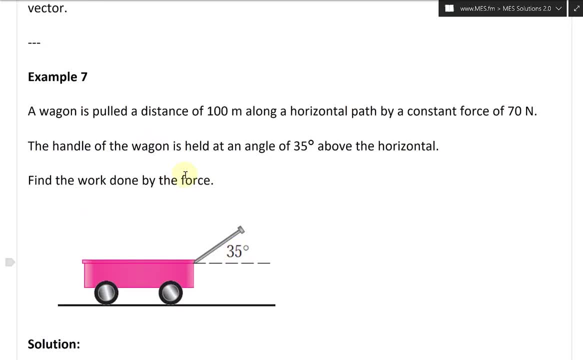 so we know angle. so we know angle. uh, we know the magnitudes of both. uh, we know the magnitudes of both. uh, we know the magnitudes of both. this number, right here, this goes 100. this number right here, this goes 100. this number right here, this goes 100 meters. 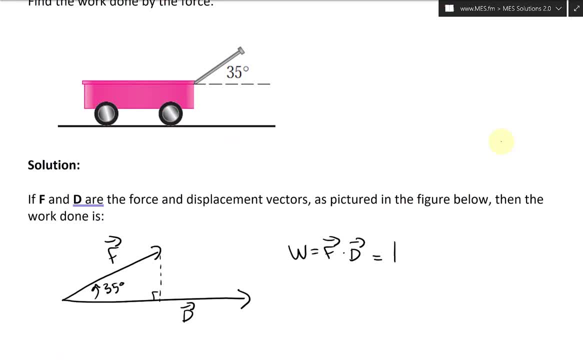 meters. meters. the magnitude of the force times by the. the magnitude of the force times by the. the magnitude of the force times by the distance traveled or the displacement distance traveled, or the displacement distance traveled, or the displacement, and then cosine of the angle. and then cosine of the angle. 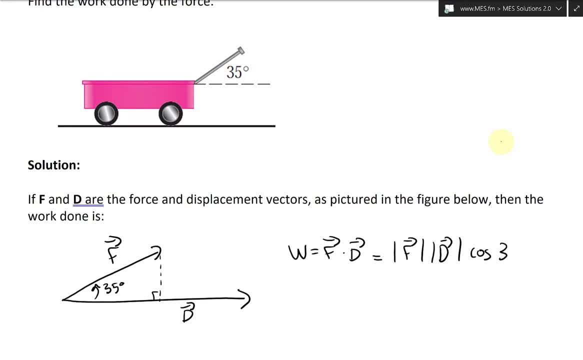 and then cosine of the angle- uh, this is going to be cosine theta, or uh, this is going to be cosine theta, or uh, this is going to be cosine theta. or cosine 35, cosine 35, cosine 35, like that, or better. yes, but cosine theta, like that, or better. yes, but cosine theta. 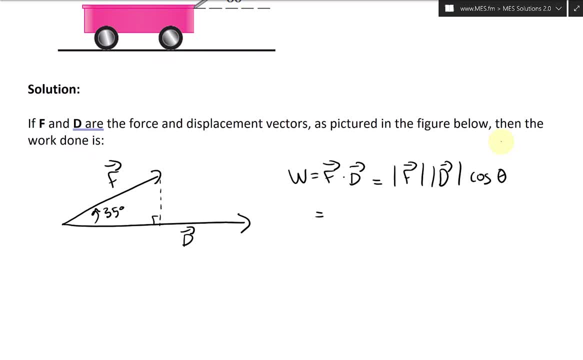 like that, or better, yes, but cosine theta, and then we'll put in all of our, and then we'll put in all of our, and then we'll put in all of our. figures in this equals to figures in this equals to. figures in this equals to, or put it here, equals to 70 newtons. 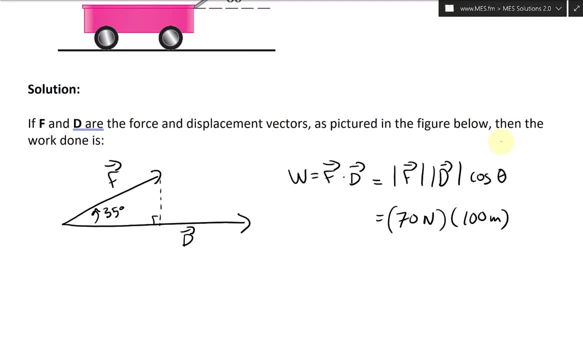 or put it here: equals to 70 newtons. or put it here: equals to 70 newtons times by 100 meters, times by 100 meters. times by 100 meters. yeah, like that: 70 newtons on 100 meters. yeah, like that: 70 newtons on 100 meters. 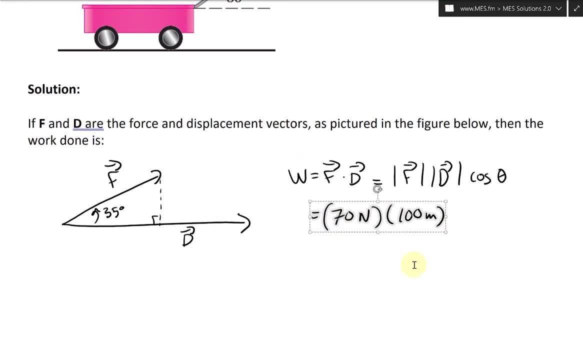 yeah, like that, 70 newtons on 100 meters, and i'm going to move this here to have, and i'm going to move this here to have, and i'm going to move this here to have, some more space, some more space, some more space, and then times by cosine. 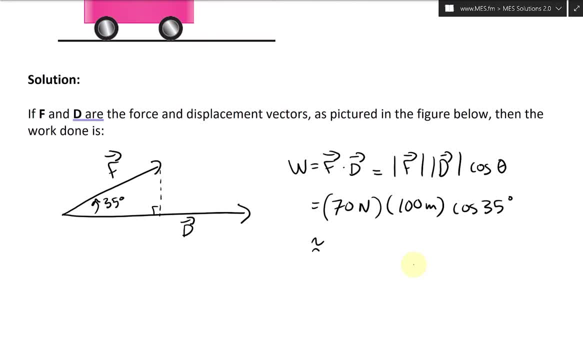 and then times by cosine and then times by cosine, 35 degrees, 35 degrees, 35 degrees, and if you plug this into the calculator, and if you plug this into the calculator, and if you plug this into the calculator, you get about, you get about, you get about five, seven, three, four newton meters. 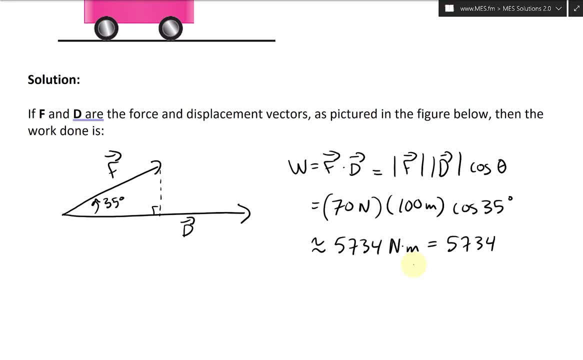 five, seven, three, four newton meters. five, seven, three, four newton meters. uh which equals to five, seven, uh which equals to five, seven, uh which equals to five, seven, three, four joules, or j three, four joules, or j three, four joules or j like that, so joules or newton meters. 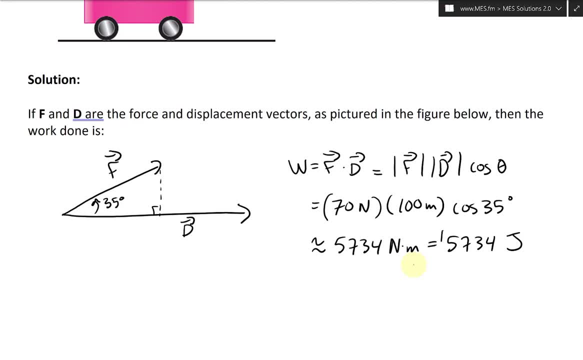 like that. so joules or newton meters like that. so joules or newton meters, yeah, so unit of energy is just a unit of. yeah, so unit of energy is just a unit of. yeah, so unit of energy is just a unit of work there, work there. 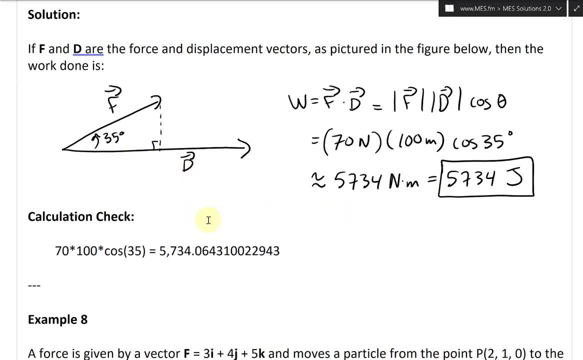 work there. very fascinating stuff, all right now. very fascinating stuff, all right now. very fascinating stuff, all right now. that we have that, let's do a quick that. we have that, let's do a quick. that we have that, let's do a quick calculation. check so: 70 times, 100 times, 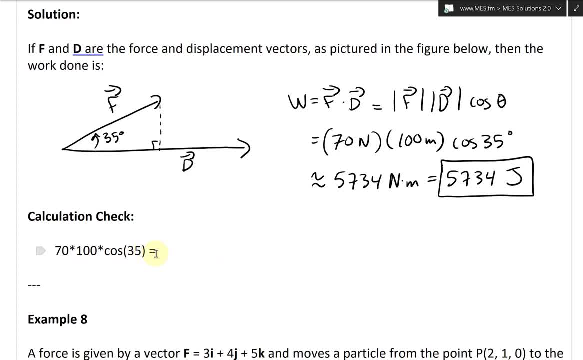 calculation check: so 70 times 100 times. calculation check: so 70 times 100 times cosine 35, cosine 35, cosine 35, and if you just plug this and this gets, and if you just plug this and this gets, and if you just plug this and this gets into joules there, which is fascinating, so 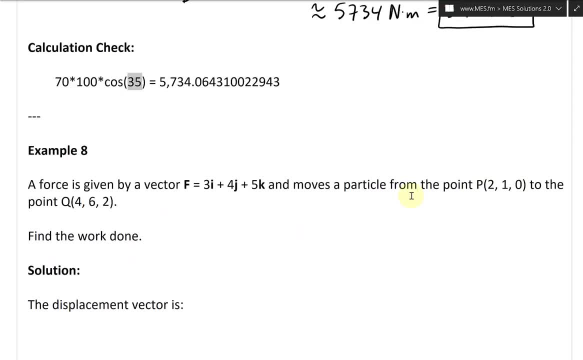 into joules there, which is fascinating. so into joules there, which is fascinating. so, yes, i think, yeah, this uses degrees. so, yes, i think, yeah, this uses degrees. so, yes, i think, yeah, this uses degrees. so, yes, that is correct there. yes, that is correct there. yes, that is correct there. all right, continuing further. so. 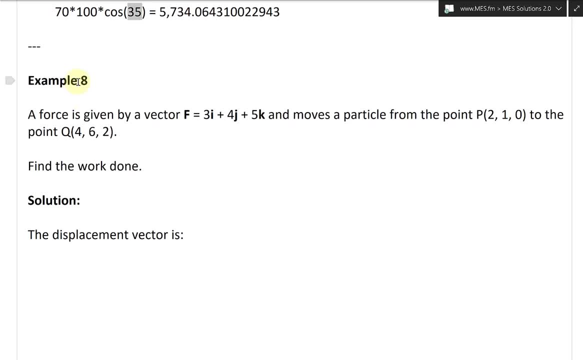 all right, continuing further. so all right, continuing further. so example is the last part of the last. example is the last part of the last. example is the last part of the last question in the question, in the question in the in this video. so a force is given by a 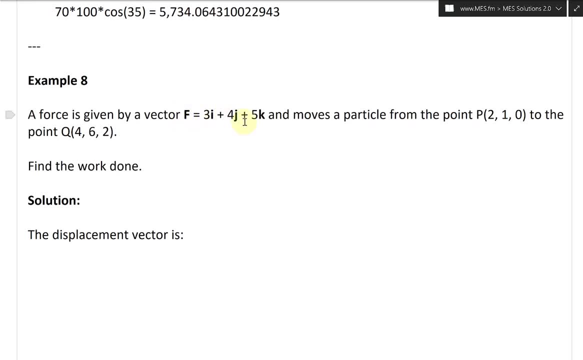 in this video. so a force is given by a in this video. so a force is given by a. vector f equals to 3i plus 4j plus 5k. so vector f equals to 3i plus 4j plus 5k. so 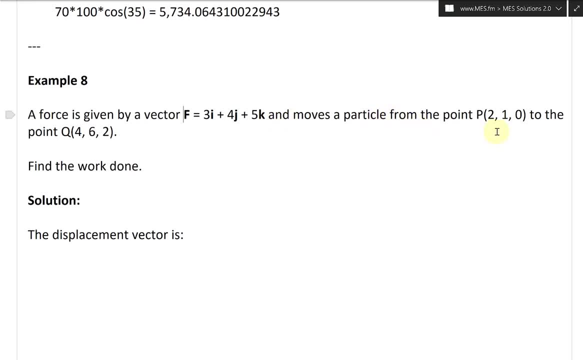 vector f equals to 3i plus 5k. so this is the standard basis vectors and this is the standard basis vectors, and this is the standard basis vectors. and moves a particle from the point p. moves a particle from the point p. moves a particle from the point p, uh, which is 2 1, 0, to the uh, point q. 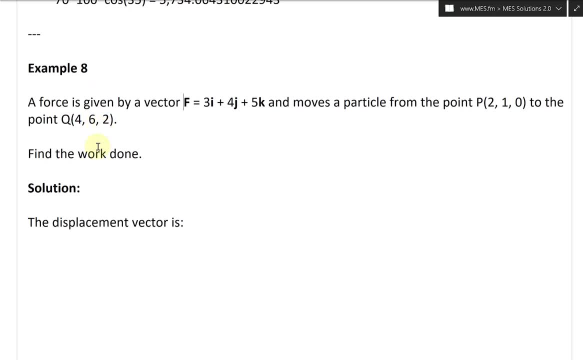 uh, which is 2 1 0 to the uh point q, uh, which is 2 1 0 to the uh point q, uh, with with the coordinates 462 and uh with with the coordinates 462 and uh with with the coordinates 462, and we're asked to find the work done and 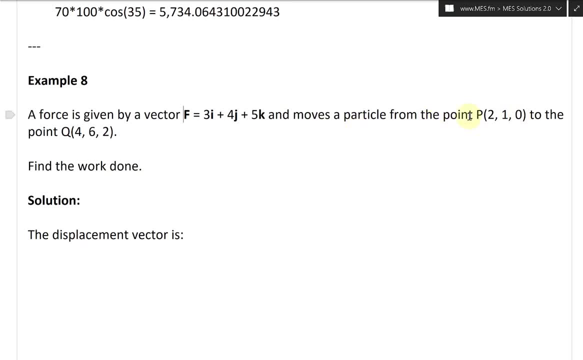 we're asked to find the work done. and we're asked to find the work done and, and, and, and. yeah, so find the work done. and moving: yeah, so find the work done. and moving- yeah, so find the work done. and moving this particle from there using this. 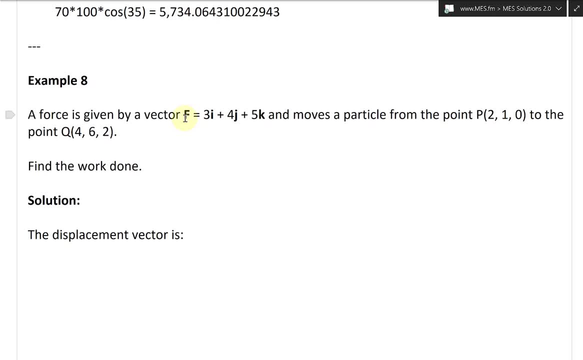 this particle from there, using this, this particle from there, using this force, we have the distance or force, we have the distance or force, we have the distance or displacement, we can calculate and we displacement, we can calculate and we displacement, we can calculate and we have the force and we can just find the. 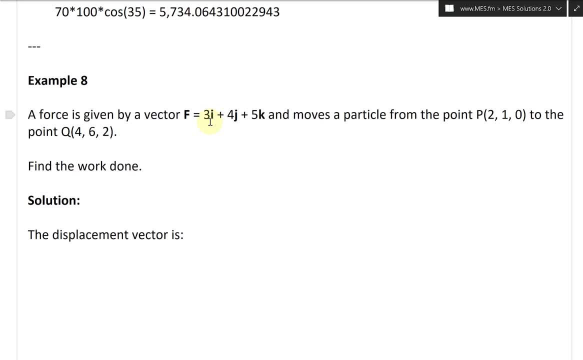 have the force and we can just find the have the force and we can just find the work done all right. so the displacement work done all right. so the displacement work done all right. so the displacement vector is well, we're given uh. vector is well, we're given uh. 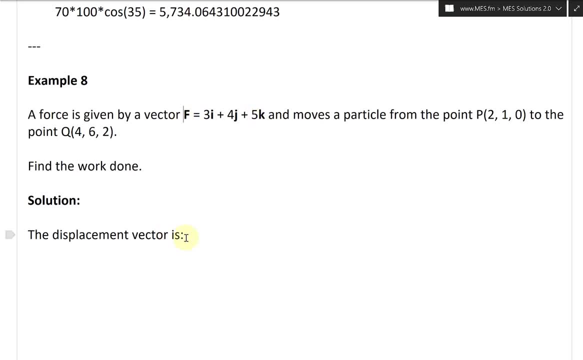 vector is. well, we're given: uh, we can solve the displacement vector, we can solve the displacement vector, we can solve the displacement vector, let's just solve this one, let's just solve this one, let's just solve this one first, so, and then we can do the dot. 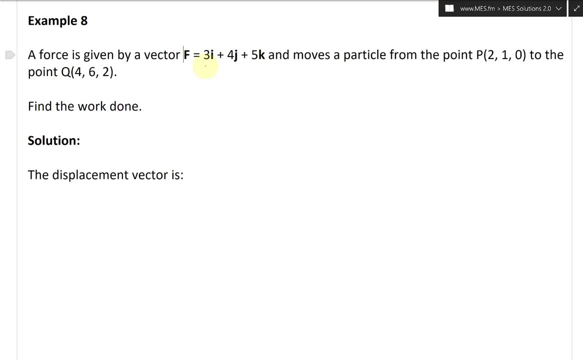 first so, and then we can do the dot first so, and then we can do the dot product and solve it. but i want to product and solve it, but i want to product and solve it, but i want to graph it in a bit, so let's go to the. 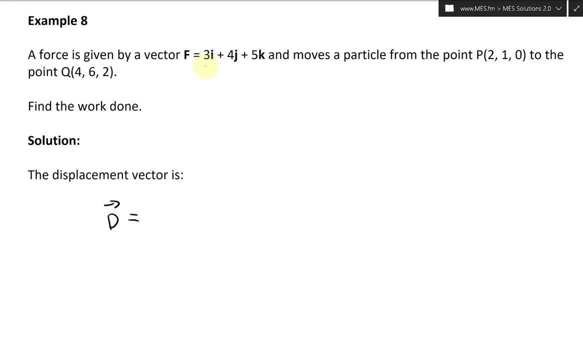 graph it in a bit. so let's go to the graph it in a bit. so let's go to the displacement vector d. displacement vector d. displacement vector d. this equals two well distance. or the this equals two well distance. or the this equals two well distance. or the vector from p to q. 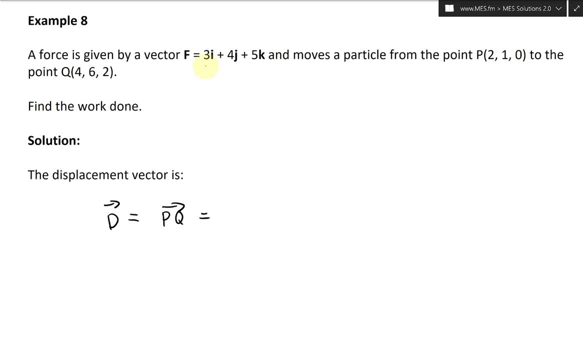 vector from p to q. vector from p to q. or the displacement there i'm going to, or the displacement there i'm going to, or the displacement there, i'm going to write this as, write this as. write this as: uh equals two, uh equals two, uh equals two. well, it's going to be the difference. so 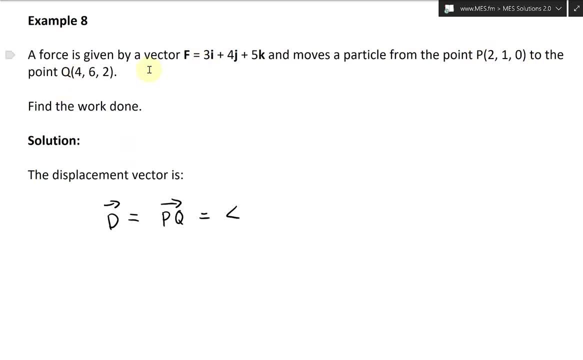 well, it's going to be the difference, so well, it's going to be the difference. so, difference from p to q, so q. difference from p to q, so q. difference from p to q, so q. you're moving from p to q, so the you're moving from p to q, so the. 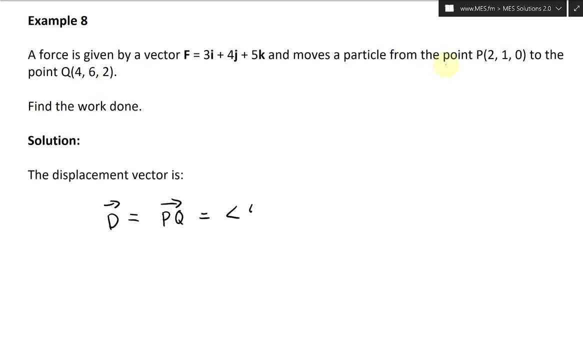 you're moving from p to q. so the displacement is the distance between it. displacement is the distance between it, displacement is the distance between it. so four minus two subtract all the so four minus two subtract all the so four minus two subtract all the components, components, components: four minus two, six minus one, and then 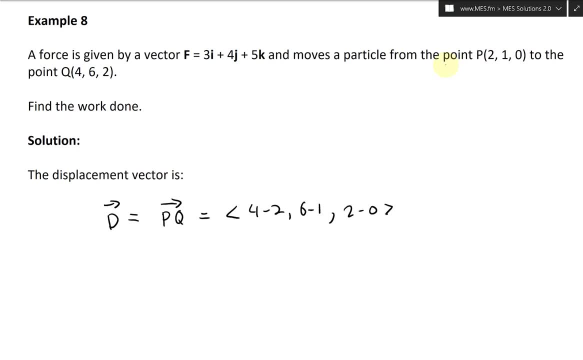 four minus two, six minus one, and then four minus two, six minus one, and then two minus zero, two minus zero, two minus zero. like this. so this equals two well, two. like this. so this equals two well, two. like this. so this equals two well two. five, two like that. 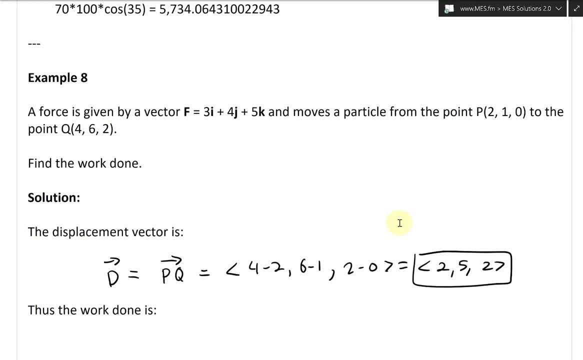 five, two like that, five, two like that. that's the displacement vector and this, that's the displacement vector and this, that's the displacement vector and this displacement vector is again. is the displacement vector, is again. is the displacement vector is again. is the relative distance from uh, from p to q. 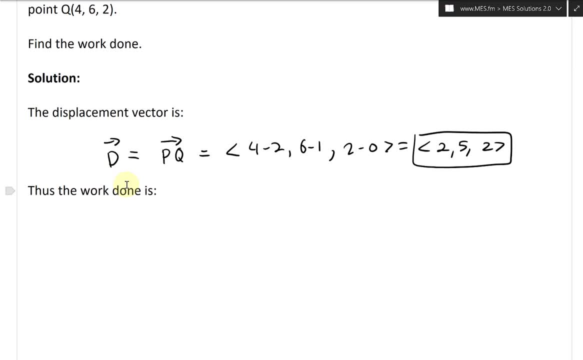 relative distance from uh from p to q. relative distance from uh from p to q. all right, so thus the work done is, and all right, so thus the work done is, and all right, so thus the work done is. and before i do that, i just want to 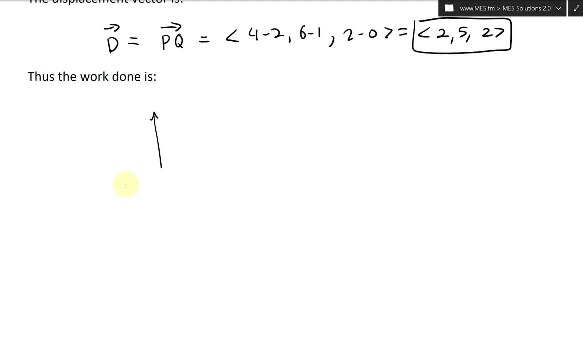 before i do that, i just want to, before i do that, i just want to graph all of this in 3d. just to graph all of this in 3d. just to graph all of this in 3d, just to illustrate what we're doing. 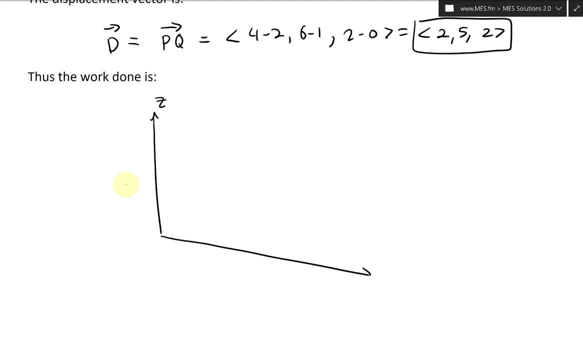 illustrate what we're doing. illustrate what we're doing and this is going to be our z components, and this is going to be our z components, and this is going to be our z components. this is going to be our y. this is going to be our y. 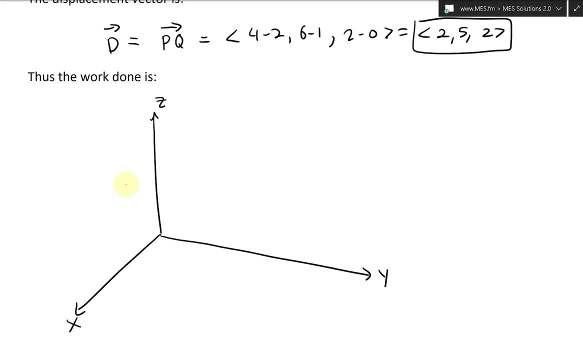 this is going to be our y and this is going to be our x, and this is going to be our x and this is going to be our y. like that, this is going to be our zero. like that, this is going to be our zero. like that, this is going to be our zero. uh, origin. 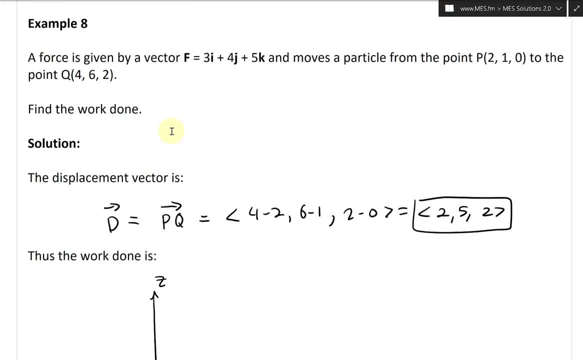 uh origin, uh origin, and we are going with a, and we are going with a, and we are going with a. let's get some uh points here. so we, let's get some uh points here. so we, let's get some uh points here. so we are going to be: uh, the force is going to. 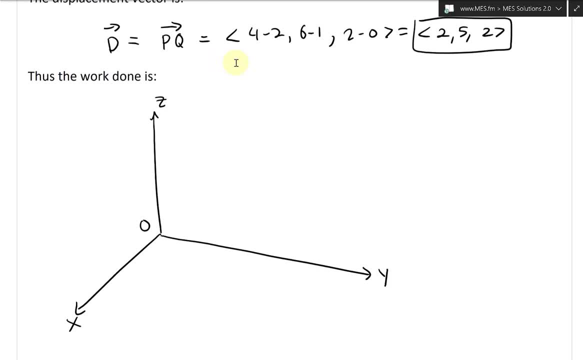 are going to be, uh, the force is going to. are going to be, uh, the force is going to be in this direction. be in this direction, be in this direction. three i four j, five k, so three i so one. three i four j, five k, so three, i so one. 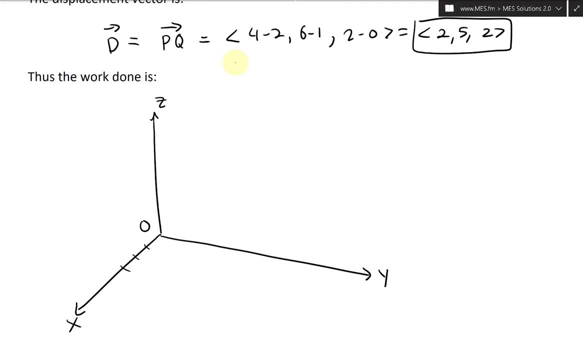 three, i four, j, five, k, so three. i so one, two, two, two, three, then four, j that's gonna be three, then four, j that's gonna be three, then four, j that's gonna be: uh, one, two, three, four, put it here. uh, one, two, three, four, put it here. 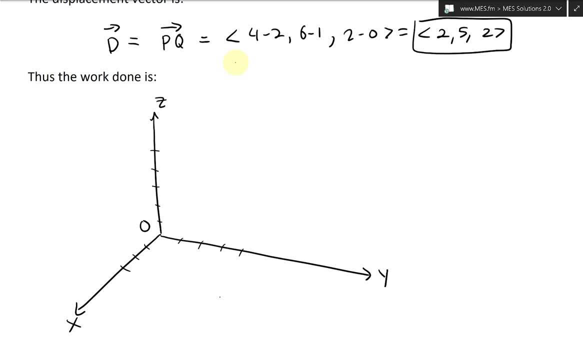 uh, one, two, three, four, put it here- and then five: one, two, three, four, five, and then five. one, two, three, four, five, and then five. one, two, three, four, five, all the way up across on top, all the way up across on top, all the way up across on top there, and i'll just draw this in, uh, 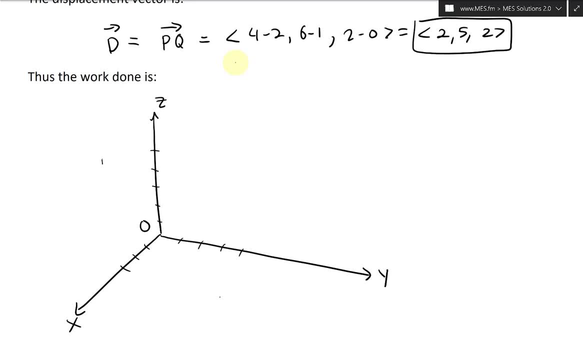 there and i'll just draw this in: uh there and i'll just draw this in: uh 3d here. this one projected is gonna be 3d here. this one projected is gonna be 3d here. this one projected is gonna be across here, across here. 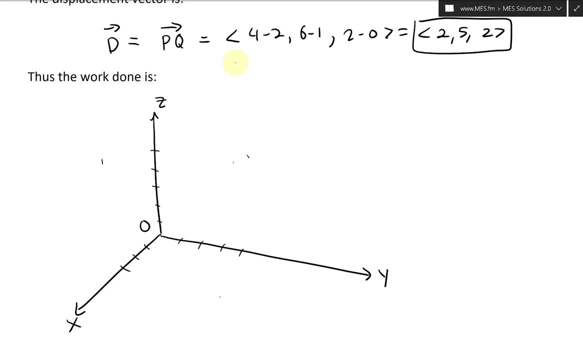 across here. uh, this one's going to be across here. uh, this one's going to be across here. uh, this one's going to be across here and it's going to look somewhere like, and it's going to look somewhere like, and it's going to look somewhere like this. so this is our force. 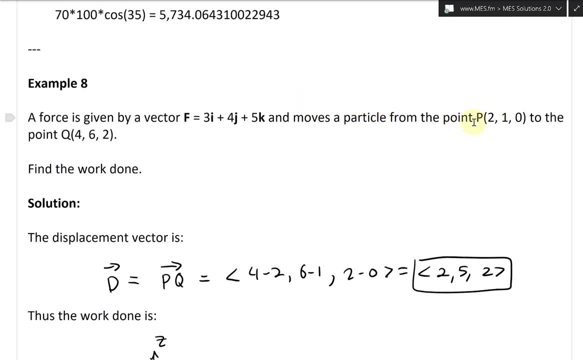 this, so this is our force, this, so this is our force: f and then our particles can be moved. f and then our particles can be moved, f. and then our particles can be moved from q from point p two one zero. from q from point p two, one zero. 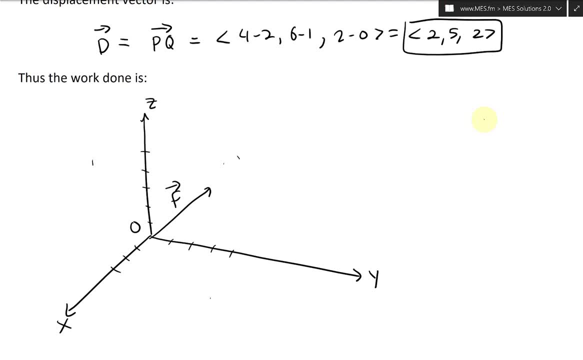 from q, from point p: two, one, zero. this is gonna be one, two, oh yes, two. this is gonna be one, two, oh yes, two. this is gonna be one, two, oh yes two. one and zero, so it starts from here. one and zero, so it starts from here. 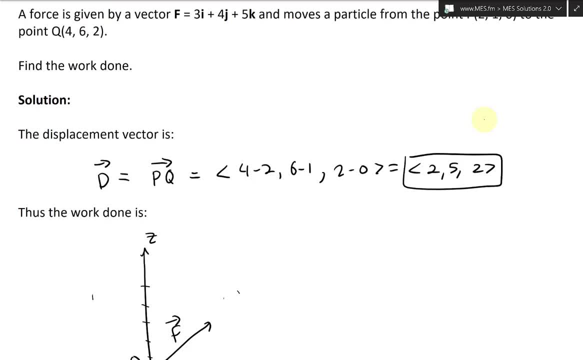 one and zero. so it starts from here. that's our point p, that's our point p, that's our point p, and it's going to go all the way into, and it's going to go all the way into, and it's going to go all the way into. well, let's see where q is. 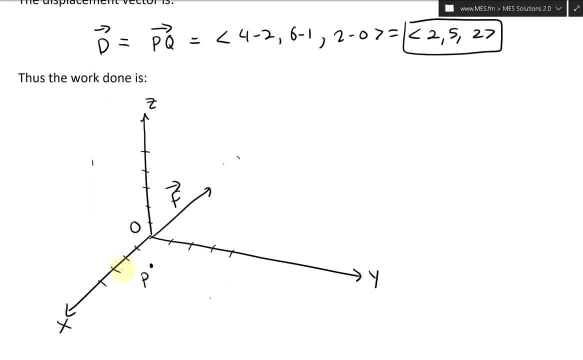 well, let's see where q is. well, let's see where q is. is four six two, it's gonna go to one. is four six two, it's gonna go to one. is four six two, it's gonna go to one. two, three, four, two, three, four, two, three, four. and then this is going to be, if this is, 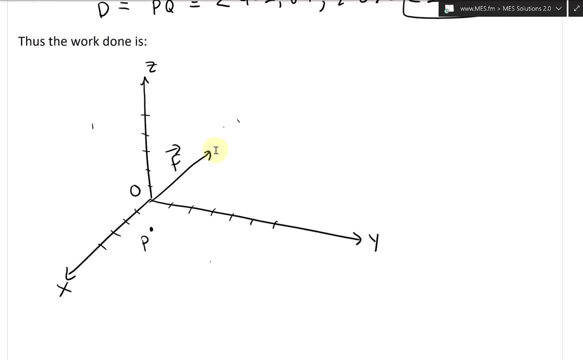 and then this is going to be, if this is, and then this is going to be, if this is: four right here, five, four, right here. five, four right here, five. six and then two, i'm gonna go rise up. six and then two, i'm gonna go rise up. 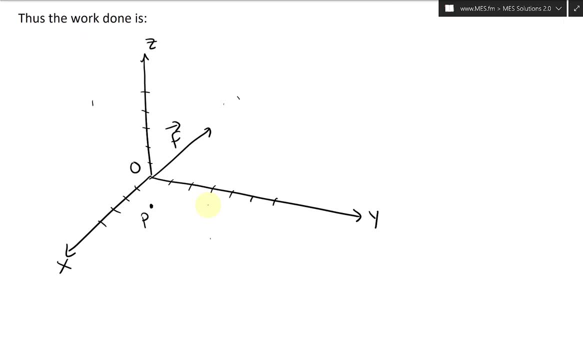 six and then two. i'm gonna go rise up twice, twice, twice. this is going to be somewhere across. this is going to be somewhere across. this is going to be somewhere across. uh, here one, two, uh, here, one, two, uh, here one, two. it's somewhere above here, so it's uh. 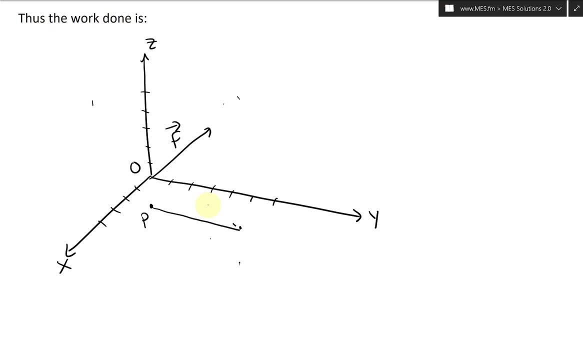 it's somewhere above here, so it's uh. it's somewhere above here, so it's uh, maybe a bit in 3d, maybe a bit in 3d, maybe a bit in 3d, it'll be somewhere like that. so that is the display, the distance here. 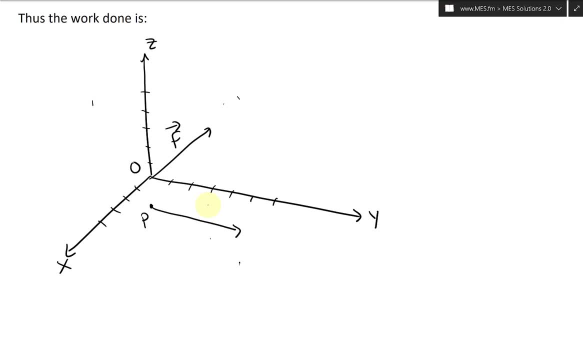 so that is the display, the distance here. so that is the display, the distance here. let's move it like that just a bit hard. let's move it like that just a bit hard. let's move it like that just a bit hard to to, to. that is our q. 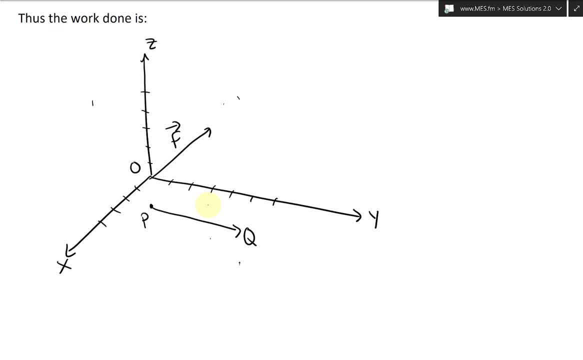 that is our q, that is our q, and this thing is uh pushing it there and this thing is uh pushing it there and this thing is uh pushing it there, and yeah, that's what we have. so this is, and yeah, that's what we have, so this is. 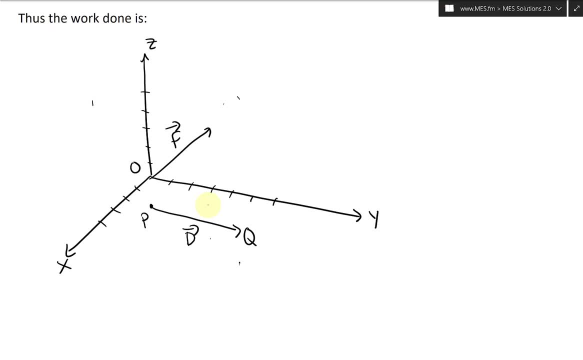 and yeah, that's what we have. so this is a displacement vector, a displacement factor, a displacement factor and, uh, i believe we did, yeah, we do here, and yeah, that's what we have. so this is a displacement vector and yeah, that's what we have. so this is a displacement factor here. this force again, i 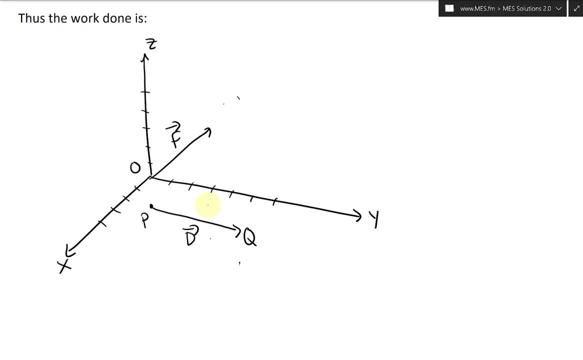 here this force again. i here this force again. i assume it just in the general direction, assume it just in the general direction, assume it just in the general direction, like that, so you just move it across, like that, so you just move it across, like that, so you just move it across here. 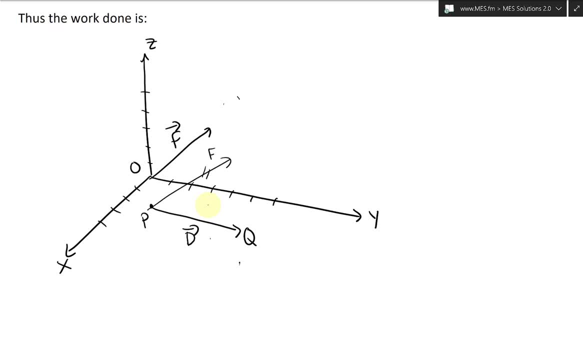 here, here, and this is going to be just f- just move it across there. so there's a, just move it across there. so there's a, just move it across there. so there's a force pushing in, that, force pushing in that force pushing in that uh direction, like that. and 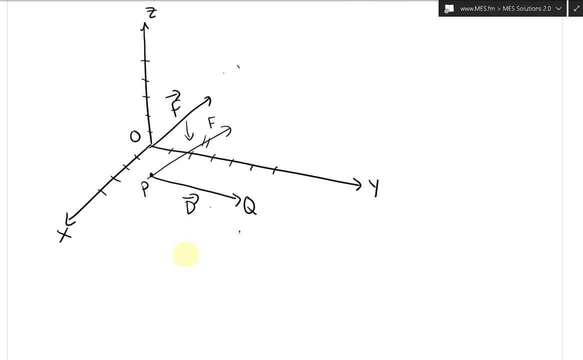 uh direction like that and uh direction like that. and yeah, i just wanted to show that anyway. yeah, i just wanted to show that anyway. yeah, i just wanted to show that anyway. so now we could just solve our. so now we could just solve our. so now we could just solve our uh product, i mean our dog product. 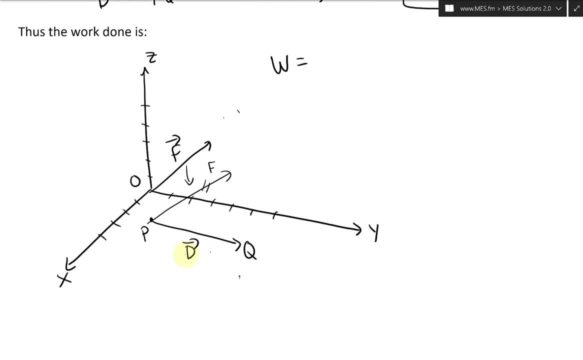 uh product, i mean our dog product. uh product, i mean our dog product. so we can do that right here w. so we can do that right here w. so we can do that right here w. equals to equals to equals to uh uh uh. the force vector times displacement. 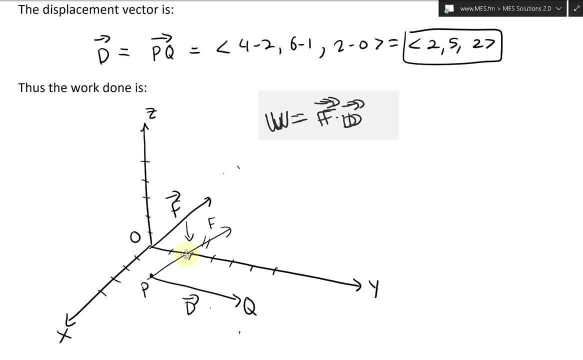 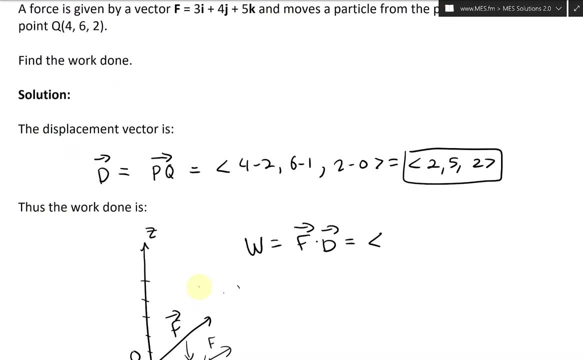 the force vector times displacement, the force vector times displacement vector which equals two, which equals two, which equals two, and this is going to be um the force and this is going to be um the force and this is going to be um the force vector vector. vector is 3i, 4j. 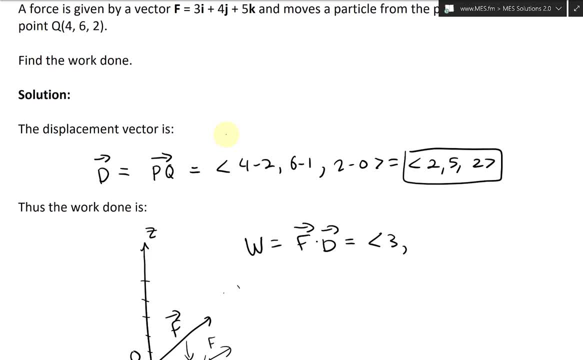 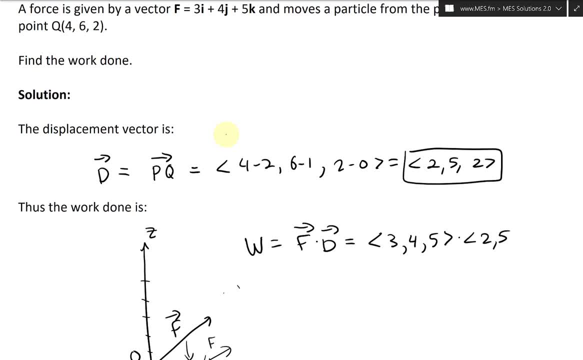 four, five, four, five, and then, and then, and then, dot it with two, five, dot it with two, five, dot it with two, five, two, two, two, two, five, two, two, five, two, two, five, two, and this equals two, and this equals two and this equals two. well, three times two. 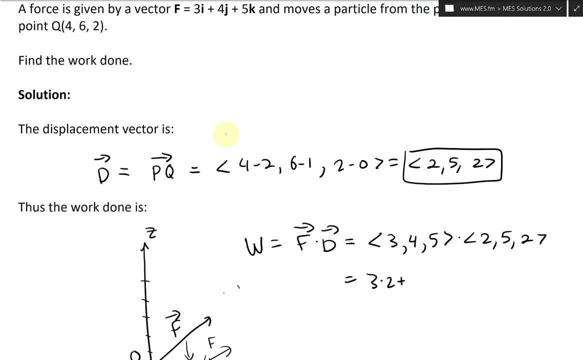 well, three times two. well, three times two. i'll just put it all together three. i'll just put it all together three. i'll just put it all together three times two times two times two plus four times five plus four times five plus four times five plus. 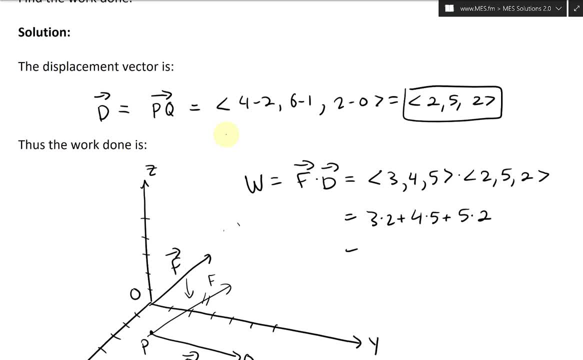 plus plus four times five times two times two times two. this equals two six plus 20. this equals two six plus 20. this equals two six plus 20 plus 10. so equals 36 plus 10. so equals 36 plus 10. so equals 36. all right, so that's 36, and it depends on. 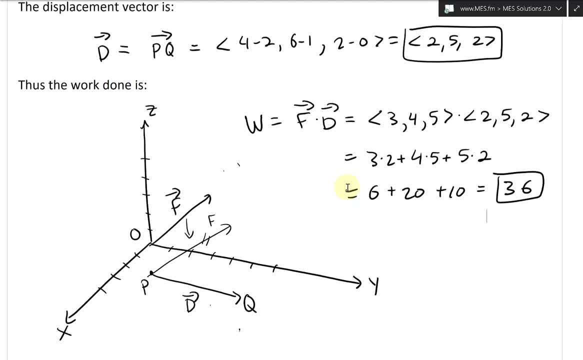 all right, so that's 36 and it depends on all right. so that's 36 and it depends on the units, the units, the units, and we're not giving in units here, but and we're not giving in units here, but and we're not giving in units here, but if i assume it's newtons and meters. 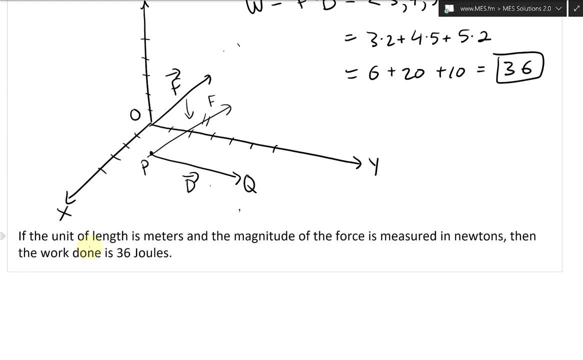 if i assume it's newtons and meters, if i assume it's newtons and meters, we'll get joules. all right, we'll get joules. all right, we'll get joules all right. all right, in here i'm just going to draw. all right, in here, i'm just going to draw. 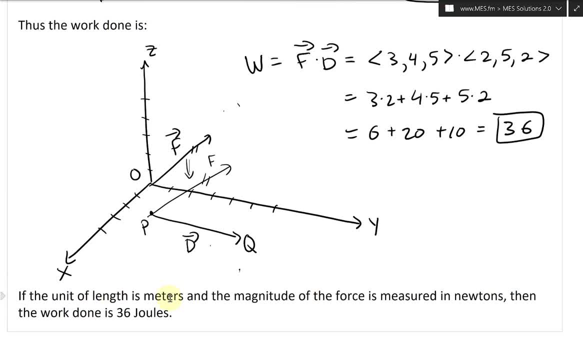 all right in here i'm just going to draw this parallel. so yeah. so if the unit this parallel, so yeah. so if the unit this parallel, so yeah. so if the unit of length is meters and the magnitude of of length is meters and the magnitude of of length is meters and the magnitude of the force is measured in newtons, 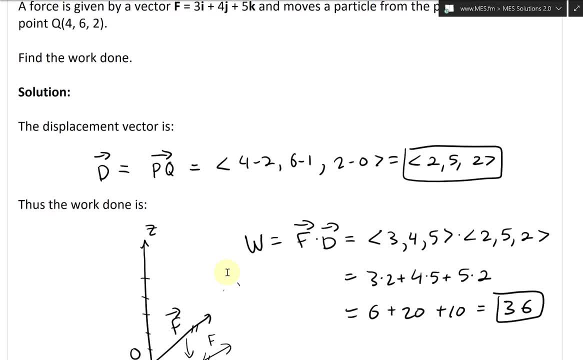 the force is measured in newtons. the force is measured in newtons and the work done is 36 joules again, and the work done is 36 joules again, and the work done is 36 joules again. that's just the. that's just the. 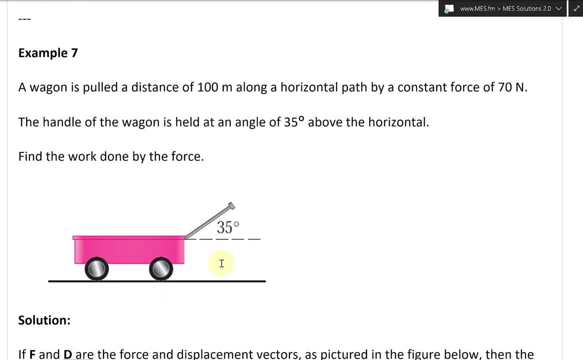 that's just the basic physics units anyways. that is all basic physics units anyways. that is all basic physics units anyways. that is all for today. hopefully you uh for today. hopefully you uh for today. hopefully you uh. follow along another epic long deep dive. follow along another epic long deep dive. 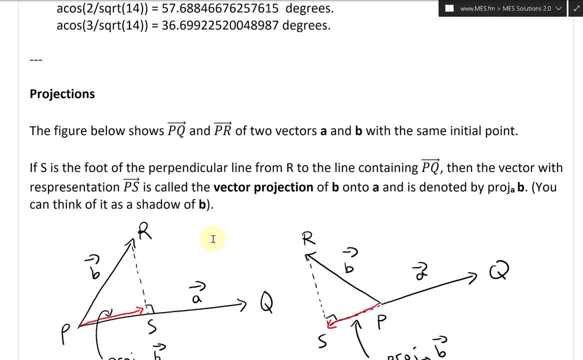 follow along another epic long, deep dive journey into mathematics, journey into mathematics, journey into mathematics anyways. and yes, it helps uh learn it anyways. and yes, it helps uh learn it anyways. and yes, it helps uh learn. it helps me to learn big time, just follow. helps me to learn big time, just follow. 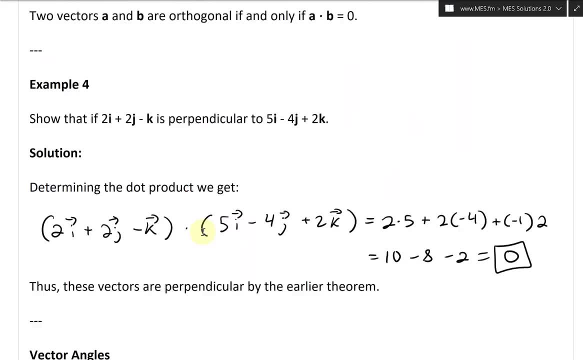 helps me to learn big time. just follow: this is how i learned. i just go through. this is how i learned. i just go through. this is how i learned. i just go through it. make videos and so on. yeah, that's all. it make videos and so on. yeah, that's all. 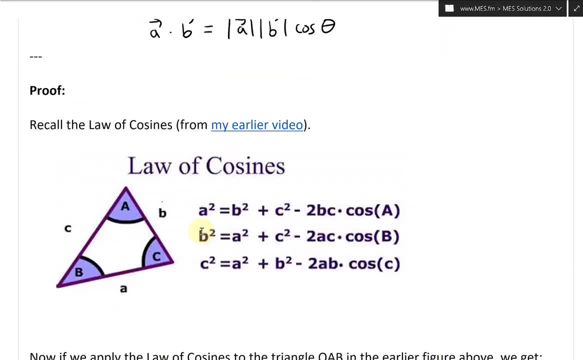 it make videos and so on. yeah, that's all for today. let me just scroll all the way for today. let me just scroll all the way for today. let me just scroll all the way up and i'll update the uh topics that up and i'll update the uh topics that. 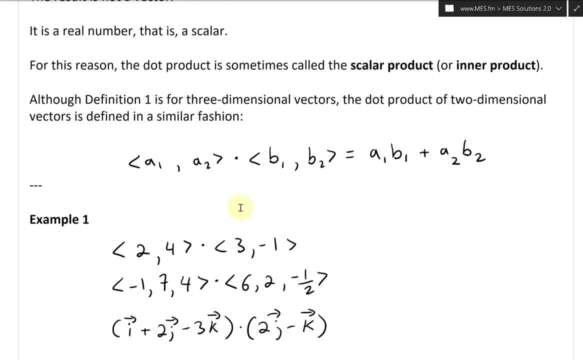 up and i'll update the uh topics that cover and timestamps because i added cover and timestamps, because i added cover and timestamps, because i added more headings as i went through the more headings as i went through the more headings as i went through the video. anyway, that's all for today and 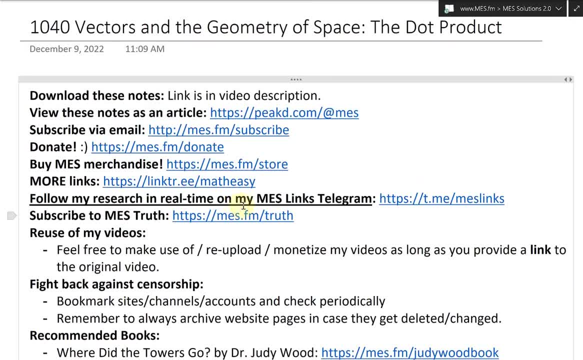 video, anyway, that's all for today. and video, anyway, that's all for today. and, like always, you can download these exact like always. you can download these exact like always. you can download these exact notes in the link in the description. notes in the link in the description. 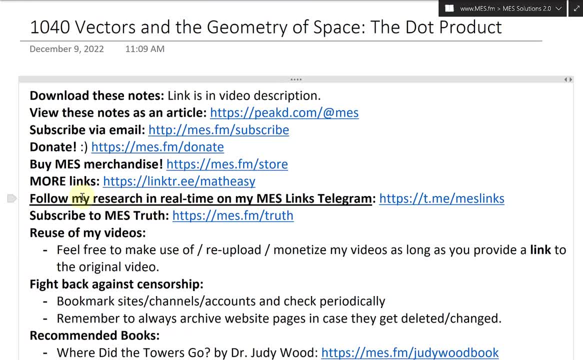 notes in the link, in the description below, below, below. and uh yeah, and that's all for today. and and uh yeah, and that's all for today. and and uh yeah, and that's all for today. and also, you make sure to watch. also, you make sure to watch. 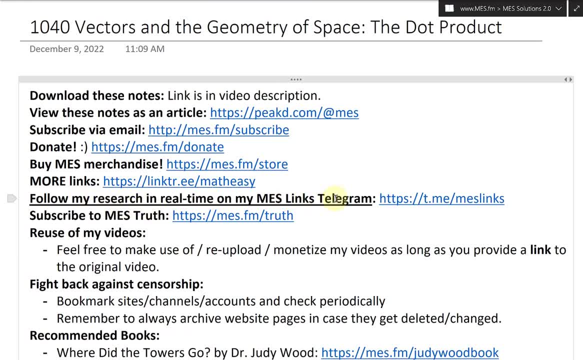 also you make sure to watch. check out my mes links: telegram. check out my mes links telegram. check out my mes links: telegram at tme slash ms links and i at tme slash ms links and i at tme slash ms links, and i basically go through all my research. 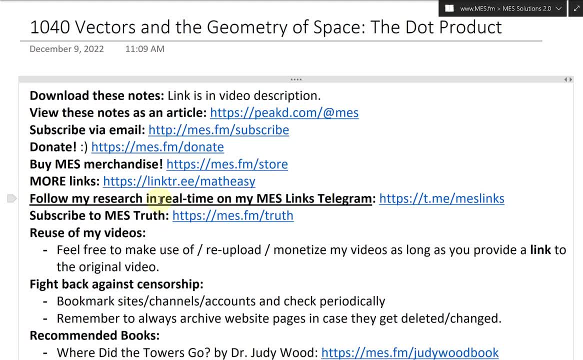 basically go through all my research. basically go through all my research in real time. a lot of funny stuff, a lot in real time, a lot of funny stuff, a lot in real time, a lot of funny stuff, a lot of conspiracy stuff, a lot of of conspiracy stuff, a lot of.